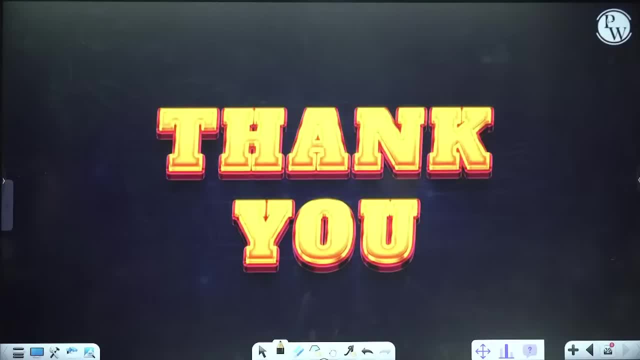 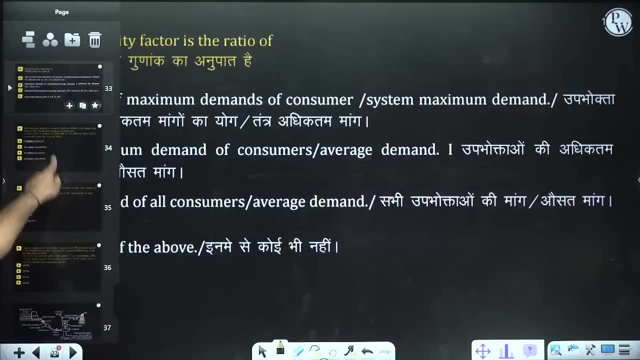 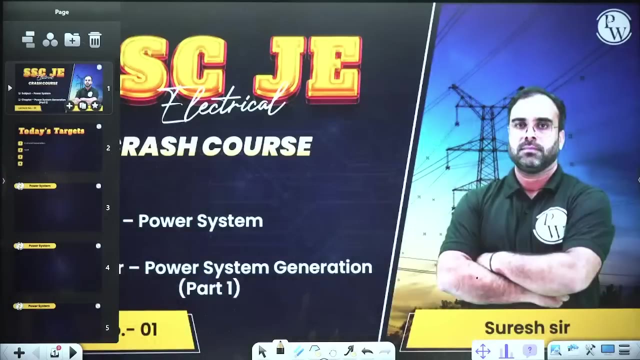 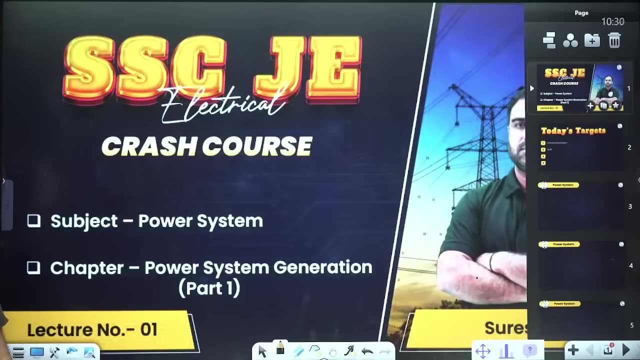 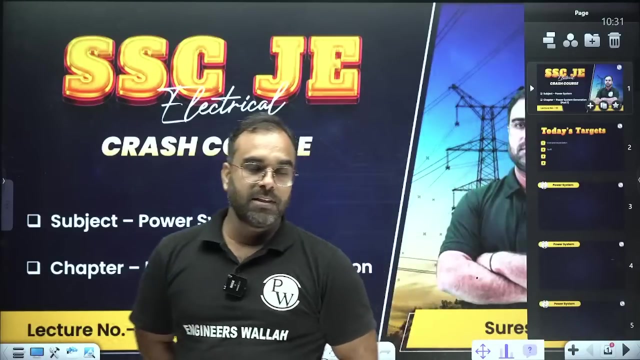 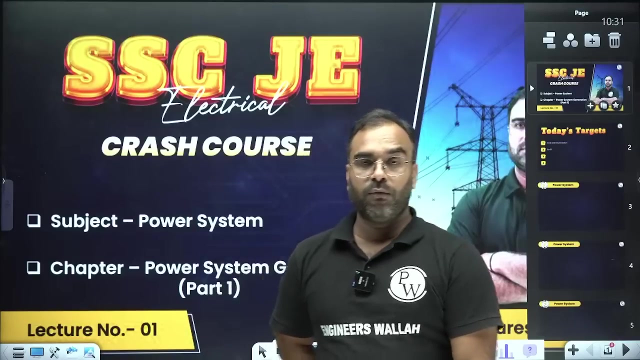 Hello, dear student, good morning Sabiko, very good morning. So how are you all? And we will quickly confirm once it is audible to everyone, clearly, And as you all know that today's subject is going to start, which is the power system. 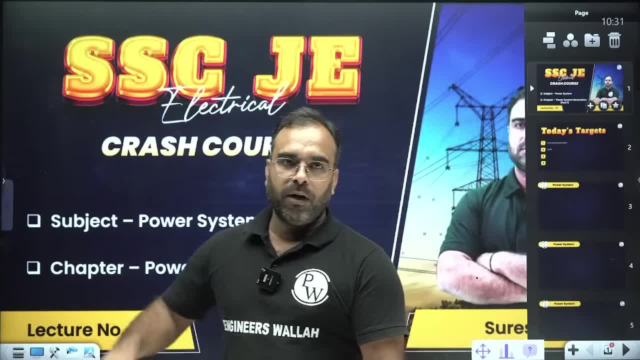 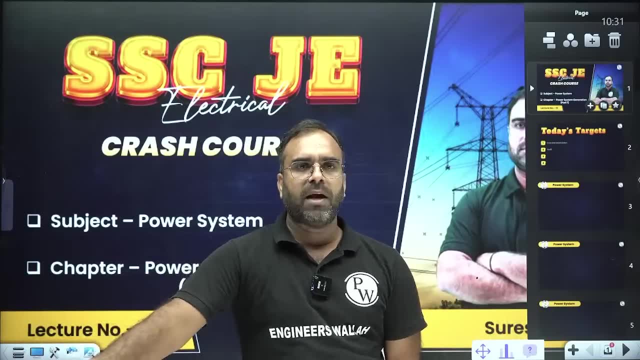 And the power system. you all know that, how important it is. I don't have to say that In every exam, whether it is a state JEE exam, whether it is an AE exam or your SSC JEE, if you are pointing out any exam, if you are studying, if your target, then the power system. 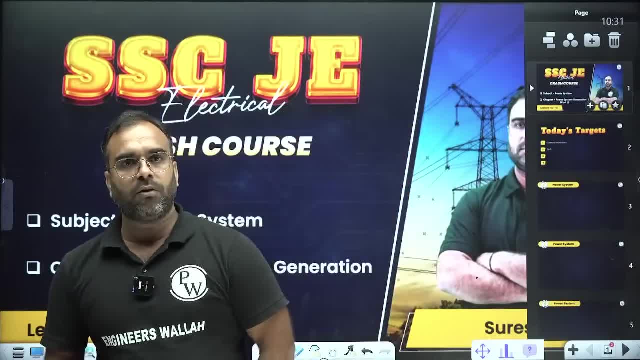 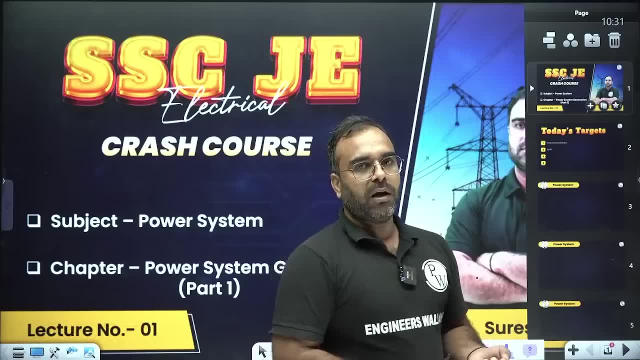 there is about 15-20% normally weightage and 20% weightage is not less. So the way we have studied the machine and we have covered every point one by one, in the same way we will try here in the power system as well, that 80-90%, all the important points. 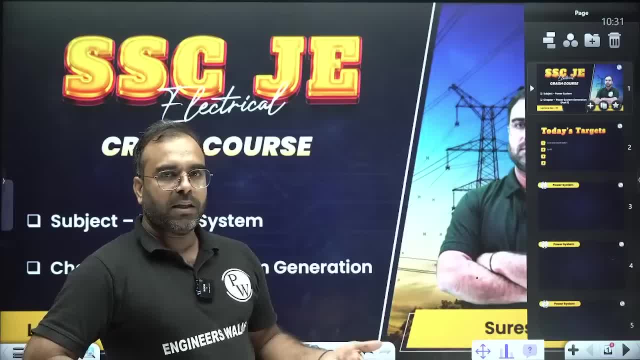 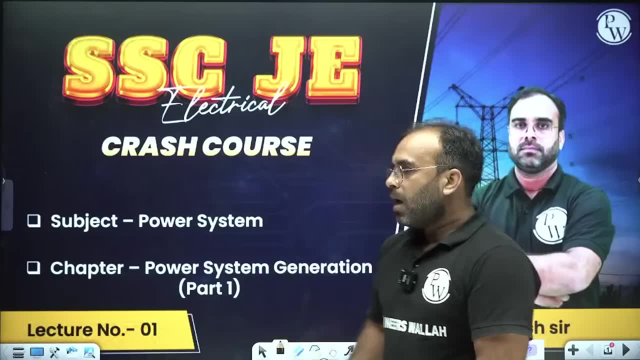 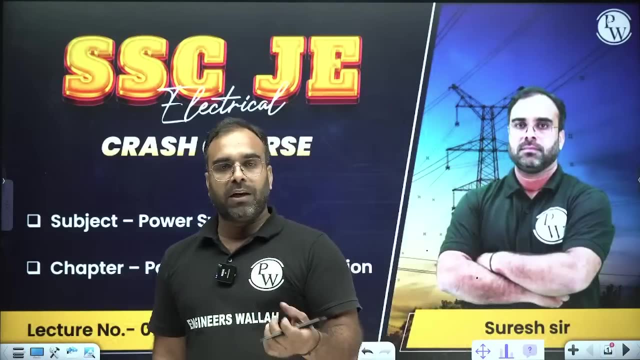 which can be asked in the exams. plus, we will also practice some questions. So, look, if you are watching today, then the first topic I have chosen today is generation. Right, That topic, look for now, because the subject we study in the class, that method, is different. 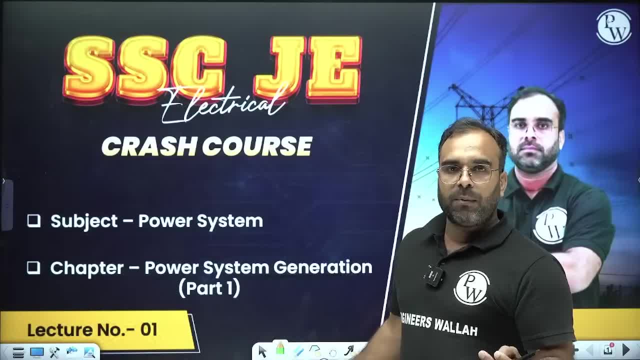 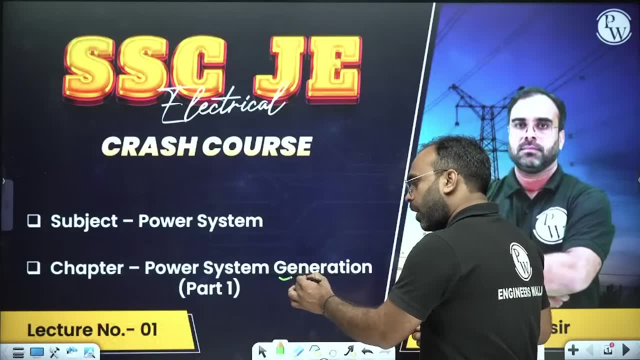 But this crash course everyone knows, And in the crash course we will cover the same topic first, which will be more important in the exam where more questions will come. So now everyone will know that this generation part. once you comment yourself and tell that. 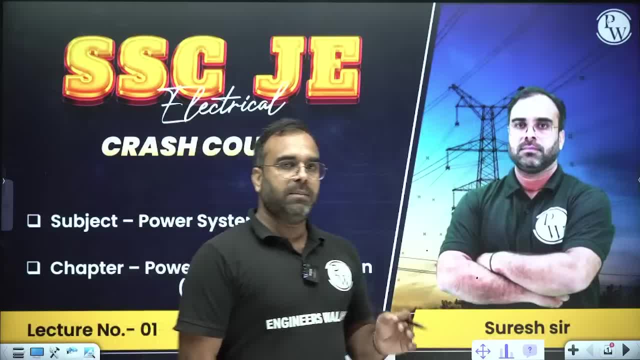 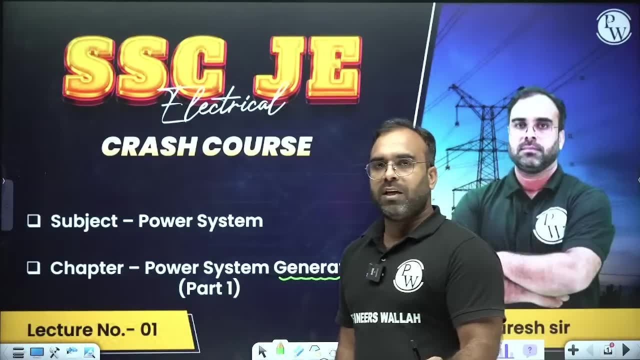 in SSC JEE exams every year, from the generation, how many questions do you get to see minimum? And now recently, if you have given an exam of NHPC or any state JEE exam, then there from the generation, how many questions will you get to see minimum? 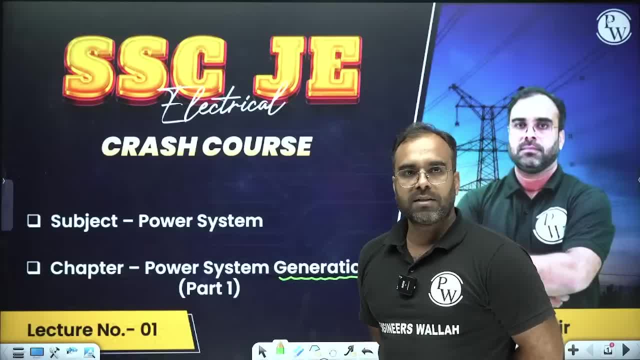 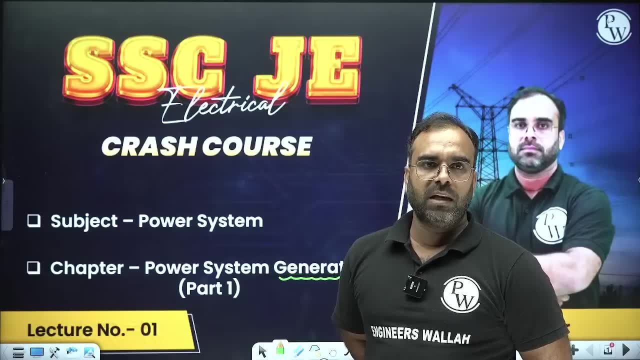 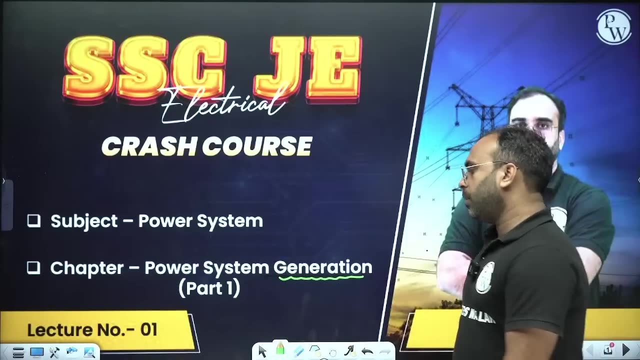 Yes, definitely you can clear it. If you can read all these points, if you know, then you can do it. Whether it is for UKPSC, JEE or for anyone you can prepare for it. So let's assume, if I talk about generation, then at least in SSC JEE exams. 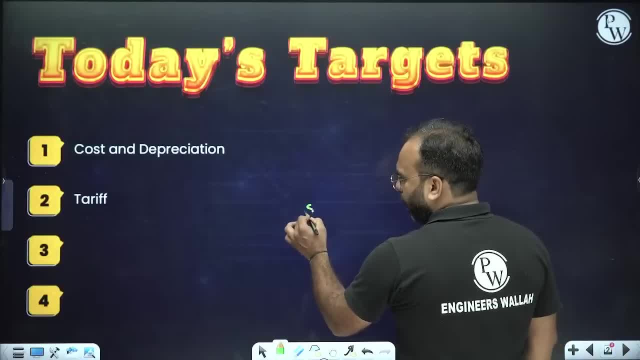 you have to keep in mind at least 5 or 6 questions, That is, 5 to 6 marks only. you will be asked from the generation. then 4,, 5 marks, 5 marks minimum, I mean I will assume the average 5 marks. 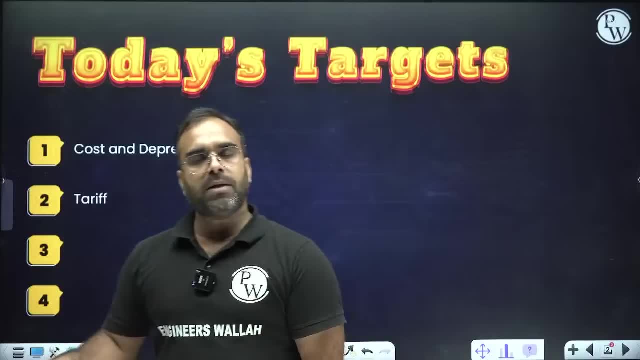 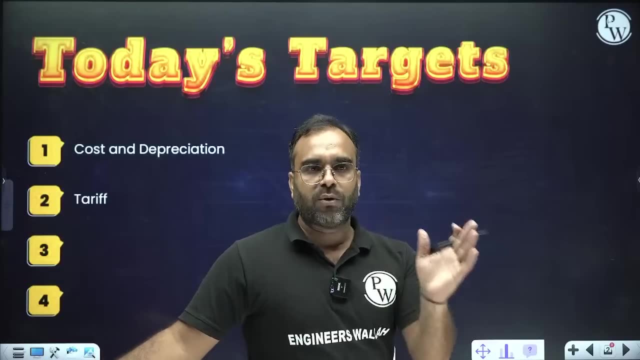 Last year also, in every paper 5 marks came from the generation. See what will we cover in the generation. We will cover tariff plans here. Fix in some set. the question of tariff is in the exams. it is going to come. 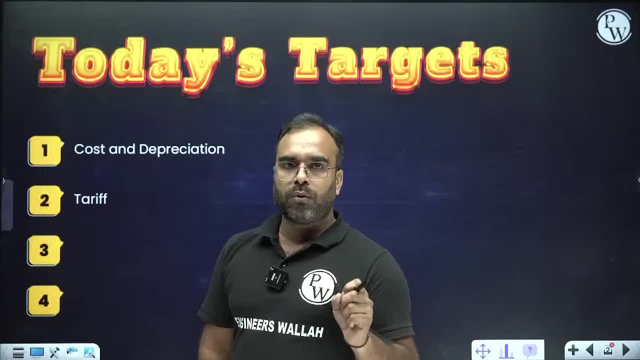 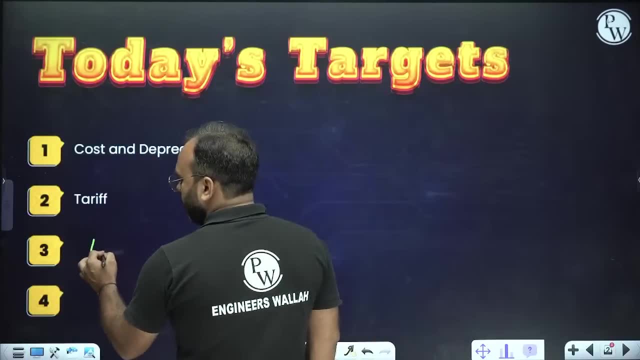 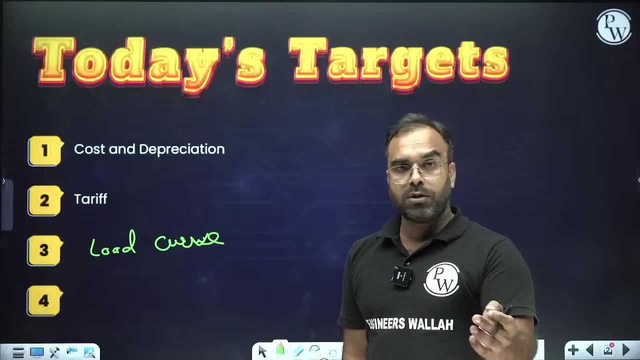 Plus, here we will talk about cost and depreciation. So today, which topics are we going to read? So there is a cost and depreciation. A tariff will be with you. after that we will have a load curve, Load curve. we will read three, four types of load curve. here we are going to read chronological load curve. 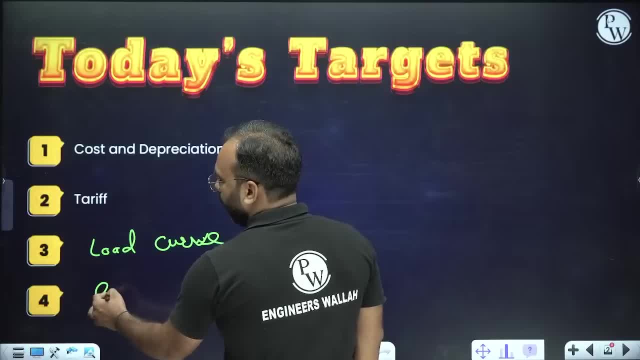 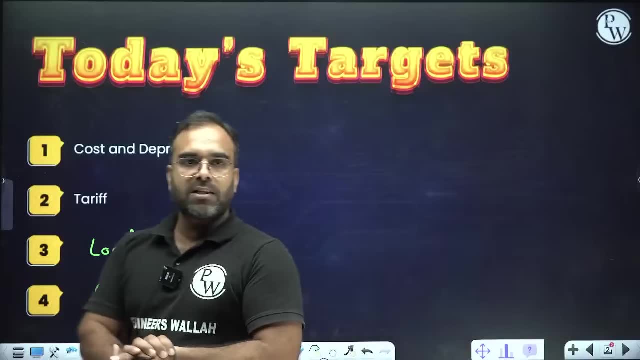 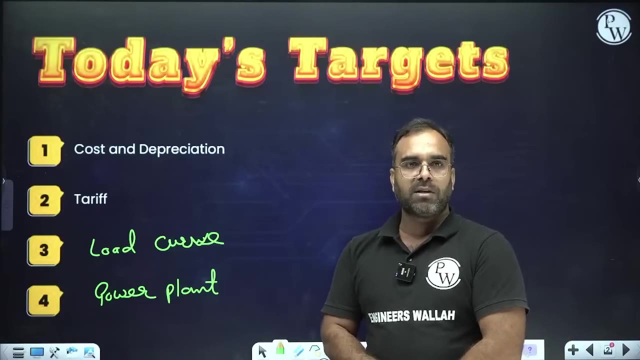 whose name you must have heard. Then we will come here in power plants, which power plants we use. So I will quickly tell you how much excited you are about the power system, because there were a lot of messages, sir, get the power system done. so let's finally power system. 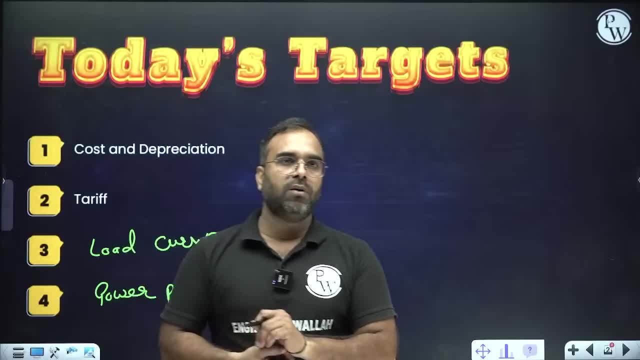 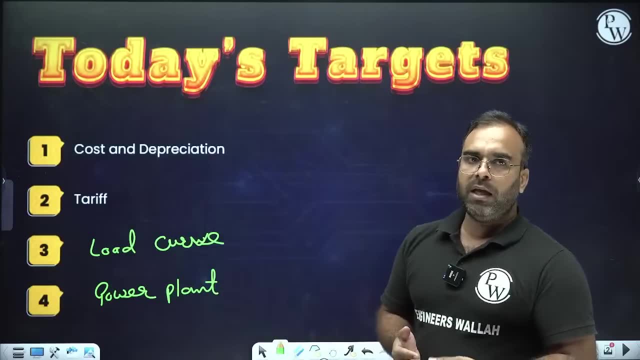 It has started. What will be special about RSE'B against JEE? Let's talk about RSE'B and JEE subject-technical, or you can talk about any exam, Whether you are taking state JEE, AE or any exam you talk about. 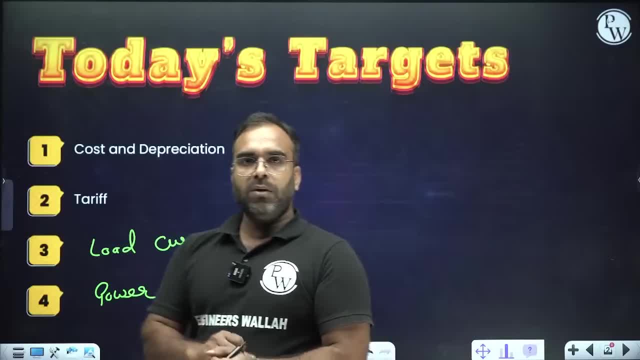 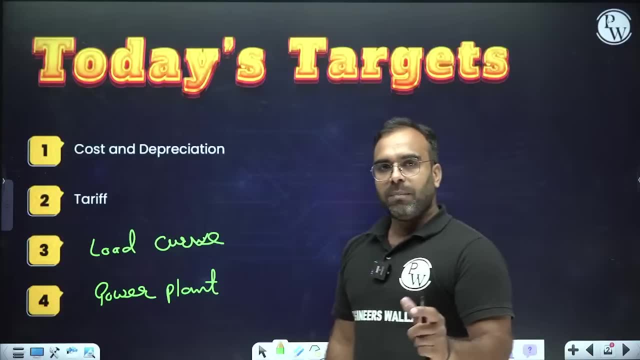 then technical remains the same. there is no change in technical. It will not happen so that for UPPSIL, JEE's power system will be made separately and forjEE, JEE accessor, LG will be different Power which will be same. 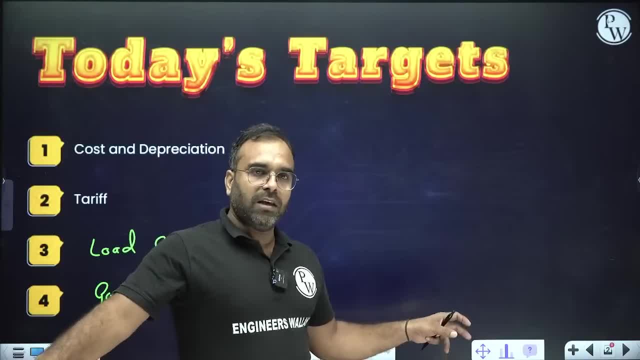 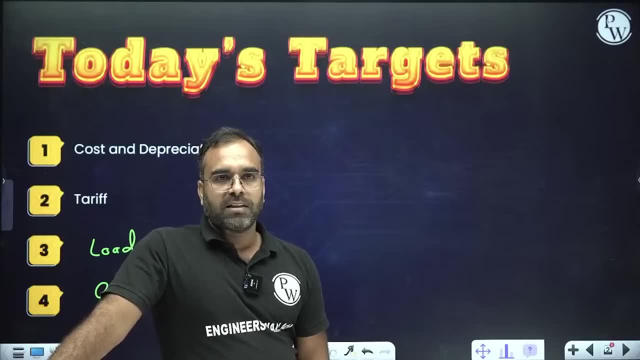 power will be the same and a power stem is covered in the same way that you Have any state. If you have a, If you are preparing for the exam, then your exam should be done. it will be our year, So we are very excited. 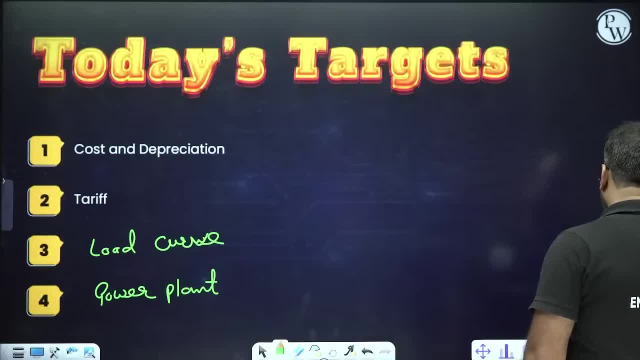 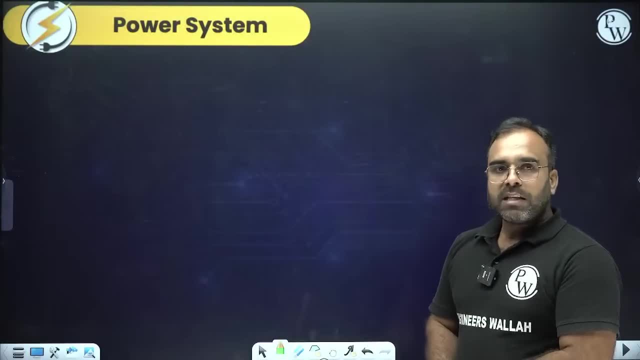 So now, let's not waste time, because I know you all have come to learn something, So we will learn and we will not waste time. So let's start our train, And here we are going to talk about the first topic. First we will have cost and depreciation. 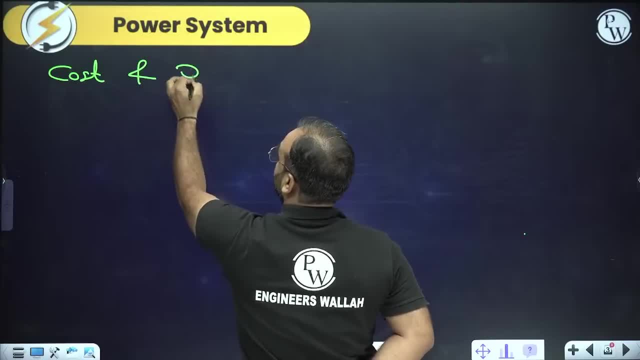 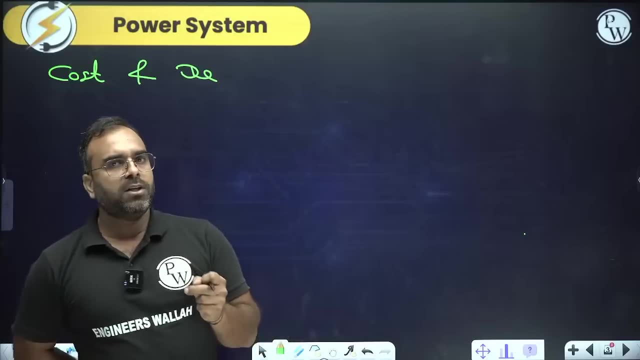 Cost and depreciation. So we will write the heading here. I will take a pen copy with me Because you know that Pavasthan is a very big subject. We will try to cover all the short notes in 50 pages or 60 pages. 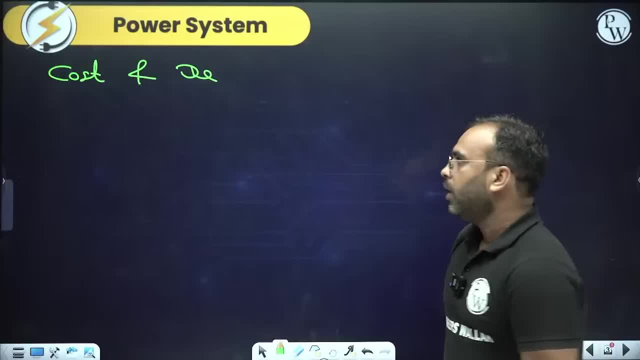 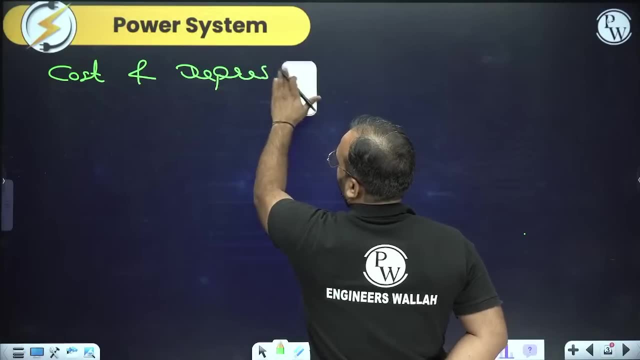 You can easily revise 50-60 pages in the last time, So we will take a pen copy. We are talking about cost and depreciation, So write the heading cost and depreciation. Now here, if we talk in Hindi, then what do we call it? 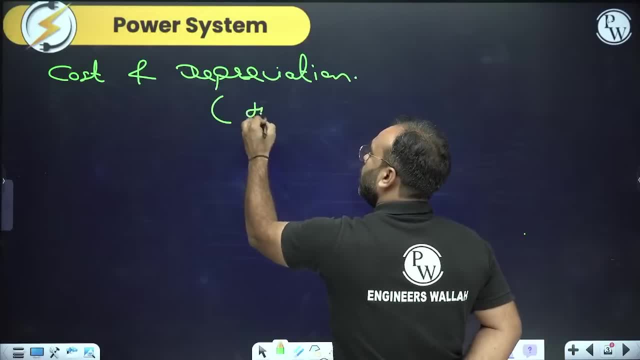 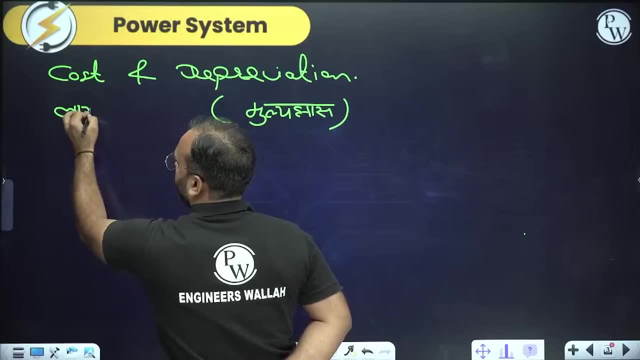 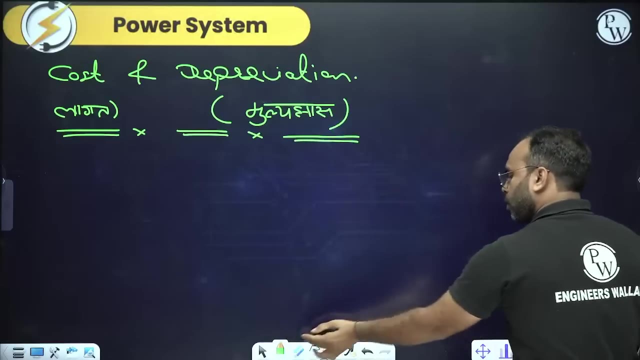 In Hindi we call it depreciation. What do we call it? We call it Mulyahas, We call it Mulyahas, So we call it Mulyahas, So we call it Mulyahas. So here, the first question is the same question that you get in the exam, that how many types of costs do we have in the power stomp? 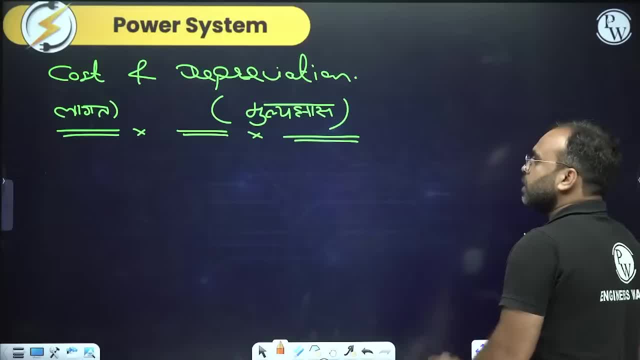 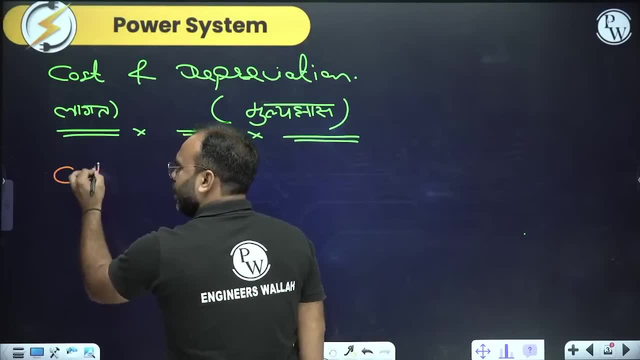 You will also quickly comment once: How many types of costs do we have? So first of all I am talking about the cost, Then I will talk about depreciation. So what are the costs here? Now see, no one will ask. you tell me what is the cost. 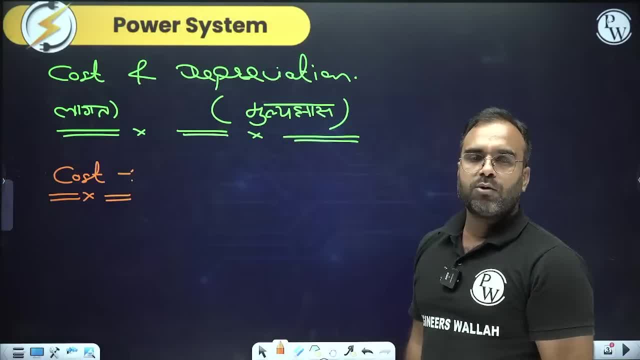 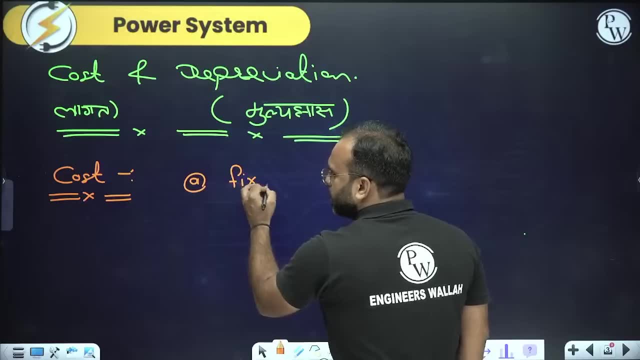 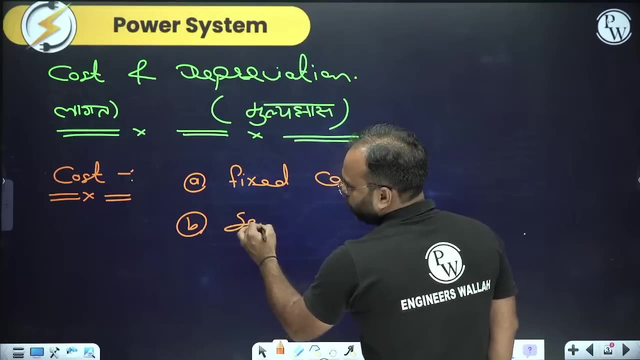 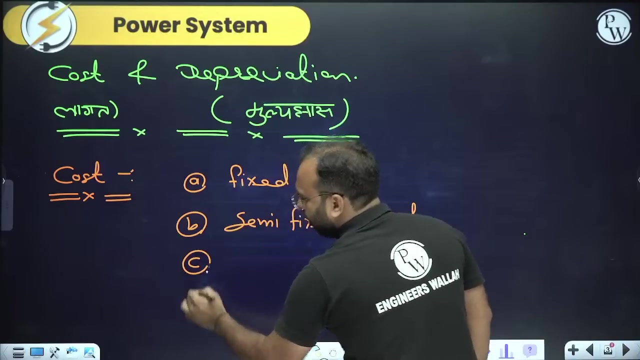 What are the costs? The amount we have to pay to purchase any equipment. what do we call it? It is cost. So cost will be of three types. First we will have fixed cost. Next we will have B semi-fixed cost And after that we will have third, running cost. 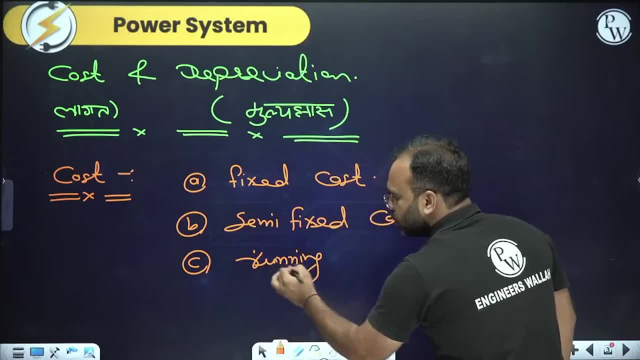 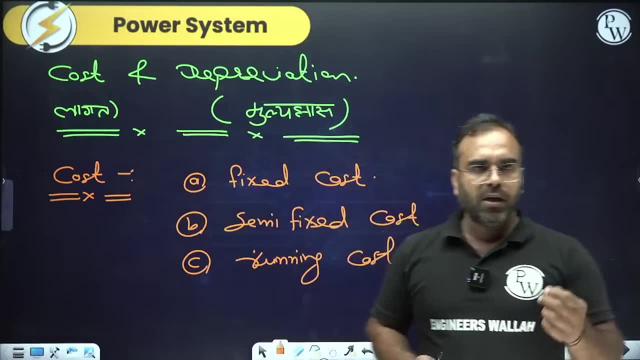 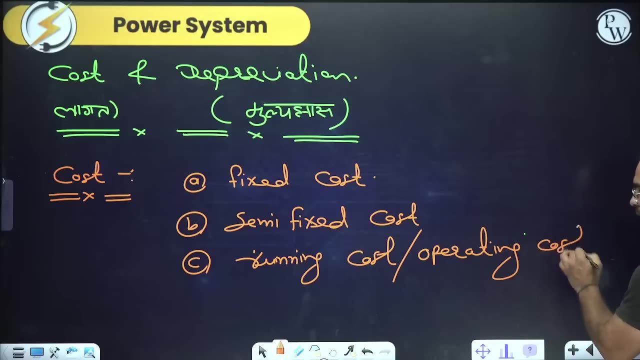 Next we will have running cost, So we will have three types of cost. The correct answer is fixed, semi-fixed and running cost. Running cost is also called operating cost. So the correct answer is of three types of cost. 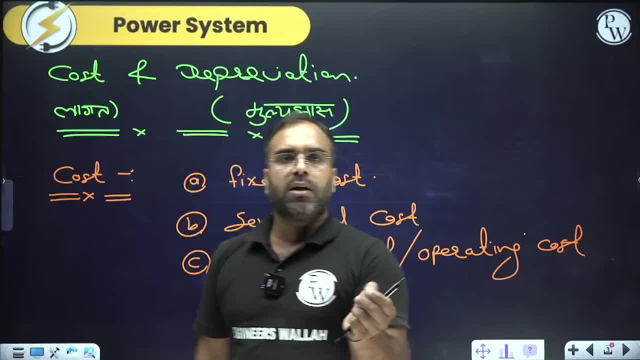 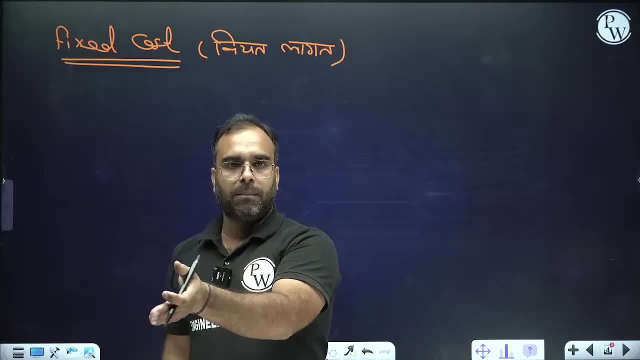 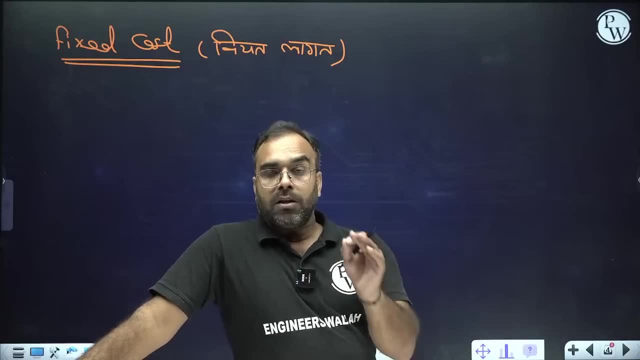 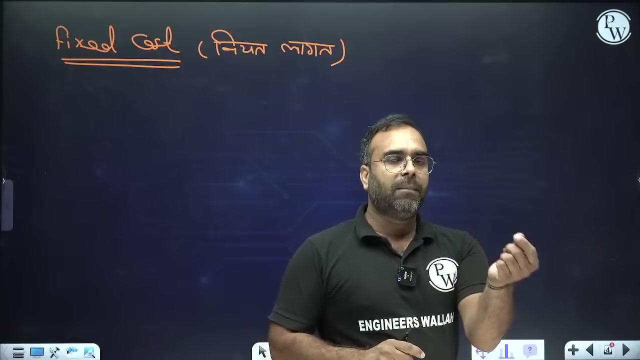 If you go to the bank, then what does the bank say? first, if you want to build a house for that, if you go to take money, then the bank will say that I will take interest from you according to 8%, 10%, 12%. 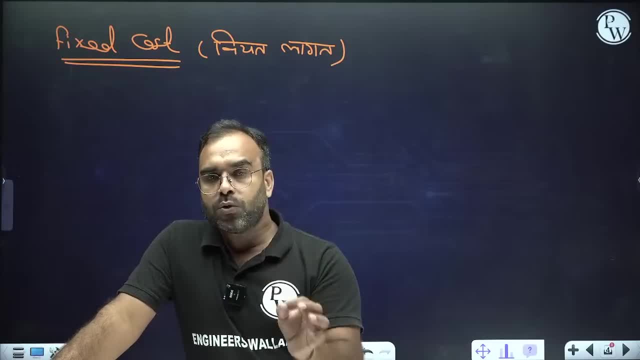 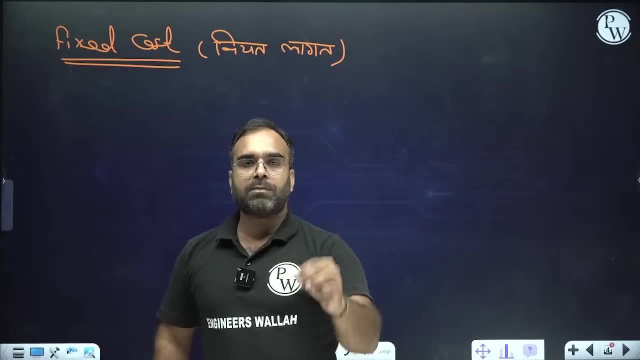 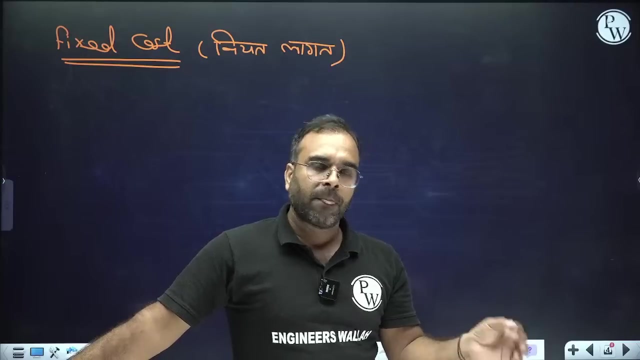 It means that as soon as you thought, as soon as you thought that I have to do what I have to make a power plan, then you went to the bank and you said to the bank that I want money. then the bank will say that take the money, but I will take interest from you. it means that as soon as he transferred the money to your bank account and got to know that your interest is from here, then it started to look. 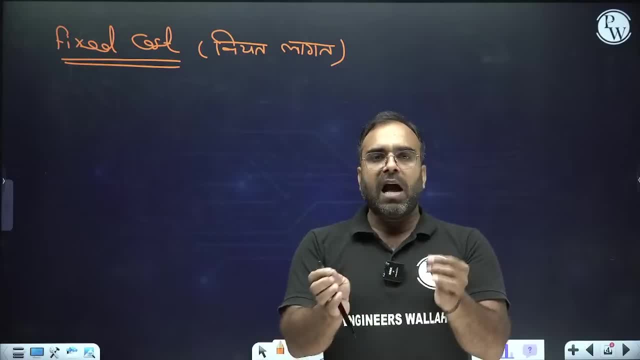 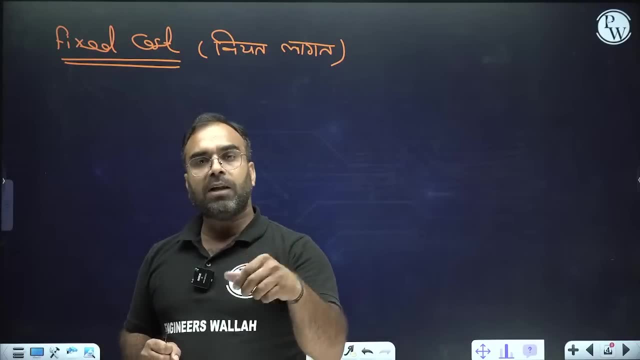 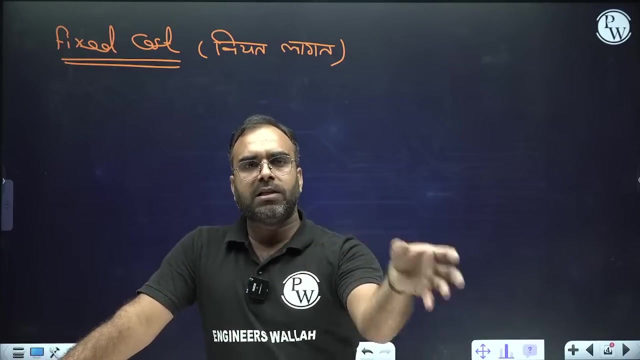 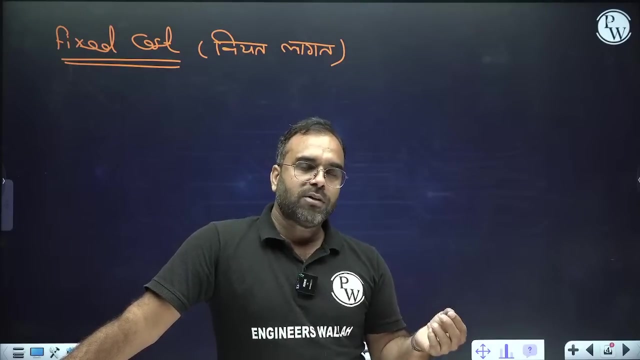 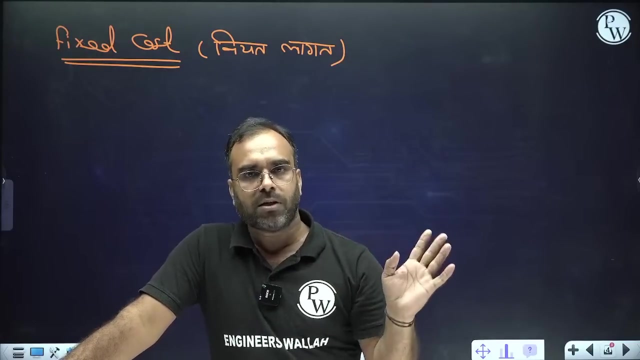 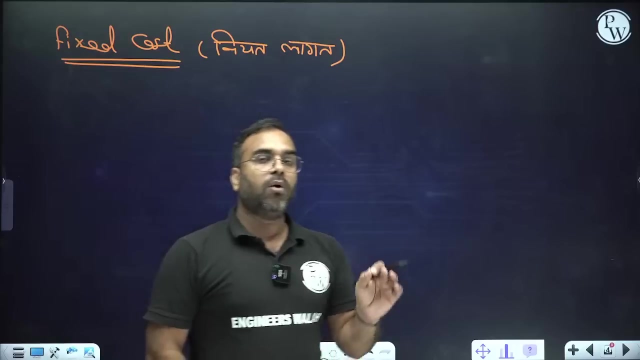 Now, the money you have kept in the bank, whether you use it or not, you have to give interest to the bank. what does this mean? It means that as soon as you thought So, you have taken money, then you will have to give interest on it, whether the plant has run now or not. the plant has not run the amount. you have taken 1000 crores, 2000 crores. we are talking a lot because in the future you will also take the same project. you will work on the project. so see, if you have taken 1000 crores, suppose to make any project, then you will have to give its interest. it is fixed that every month you have to go so much interest. it means what will come in the fixed cost? then in the fixed cost that thing will come which will be constant after making the plant once. 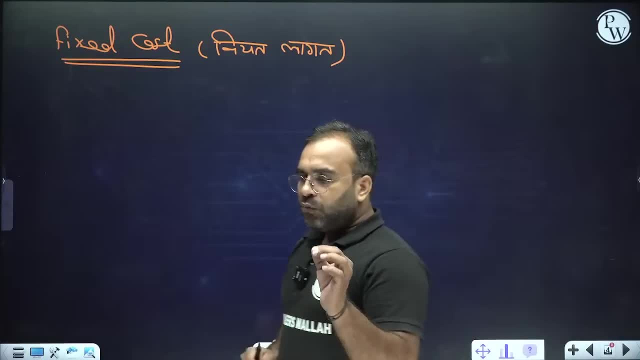 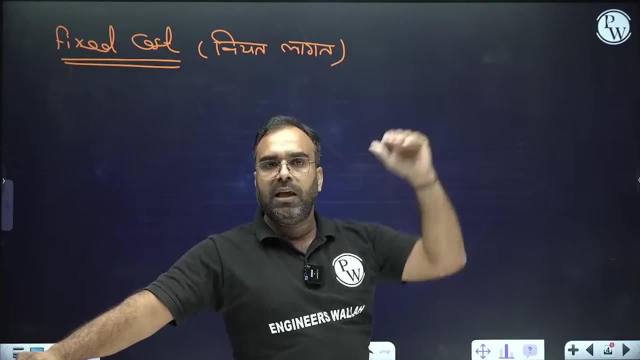 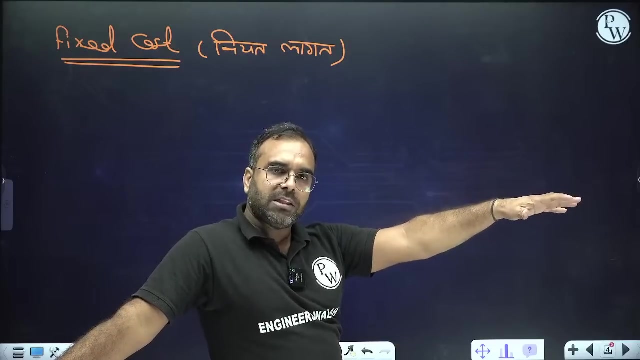 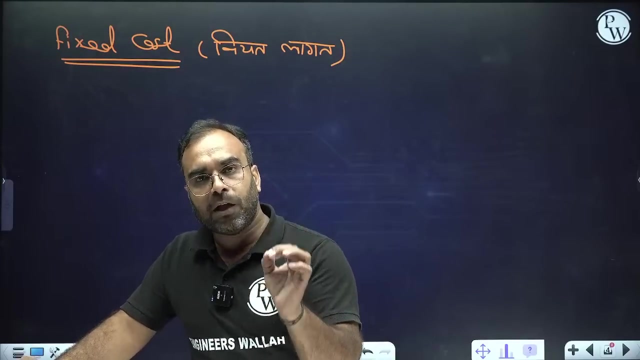 so we will quickly comment once and tell you that the fixed cost is that your plant has been made. is it depending on it? how much is the maximum demand of your plant? is it depending on it? it is not doing it. your plant has not even run. you have just bought the land. and by buying the land, what did you say that? okay, what do I have to do? I have to make a project here, but I have to give interest there. it means that whatever your generating station is, whatever the fixed cost is neither the maximum cost of your plant 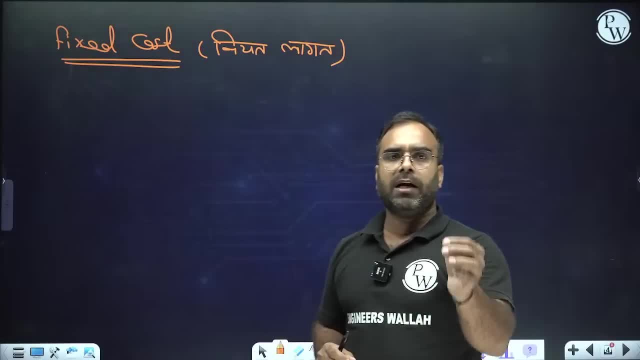 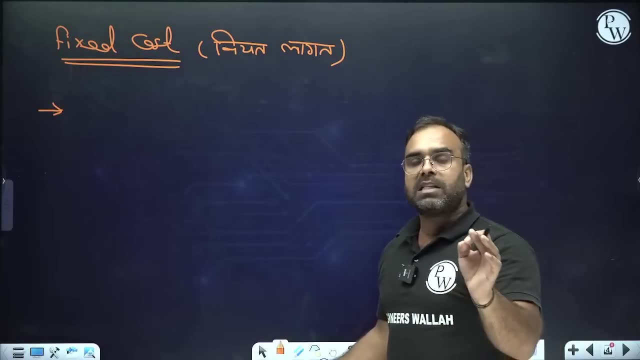 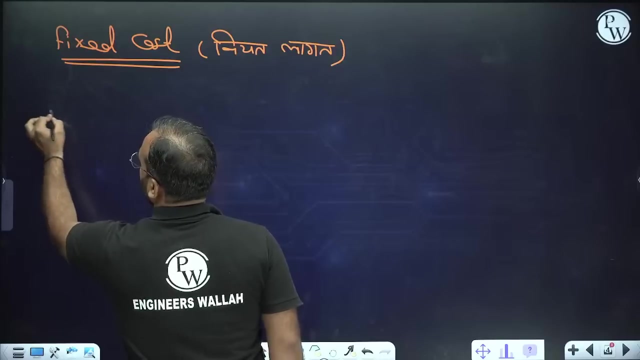 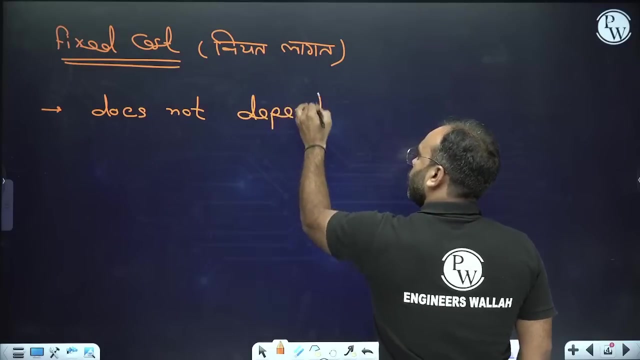 it will depend on the maximum demand and you do not have generated capacity. that is, keep in mind. the first question will ask you that the fixed cost depends on which? so keep in mind neither it depends on the maximum demand and neither it will depend on the KVA generated. that is, you can write a kilowatt hour. so write here, write the first point here. does not depends on, does not depends on, does not depends on where to keep in mind: maximum demand, maximum demand. 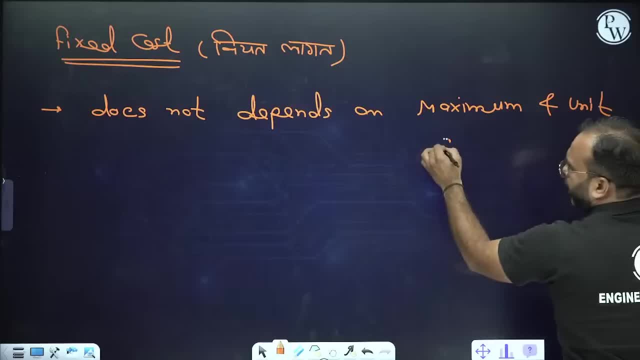 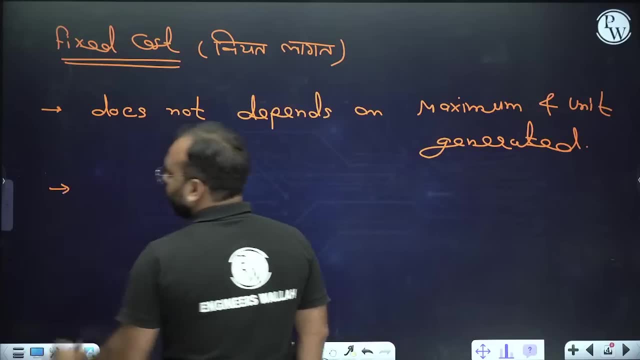 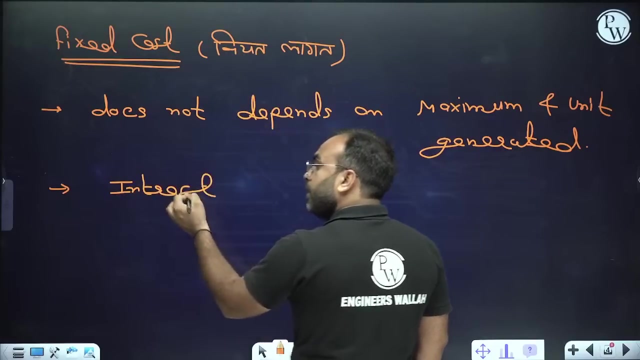 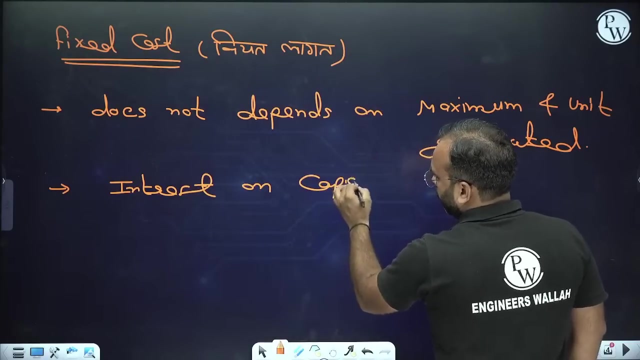 and unit generated, unit generated. so it will not depend on both. you have a question. you must have got this question in the exam many times. you must have seen talking about the second important point. so what will come here in the fixed cost? so interest on capital. what will happen here? so interest means what will happen? you will have to give interest on capital cost, capital cost, capital cost. so on capital cost you will give interest here. that will come second. 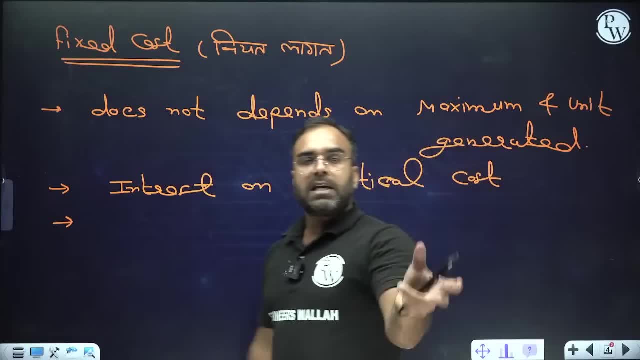 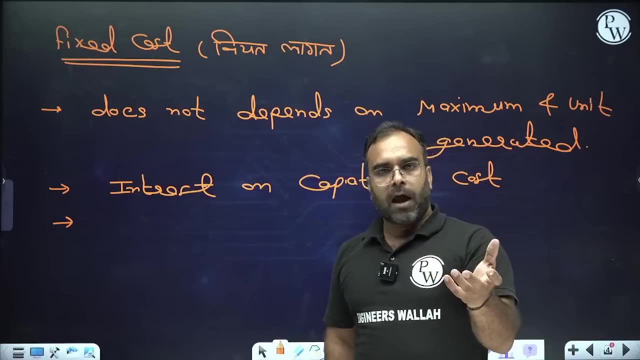 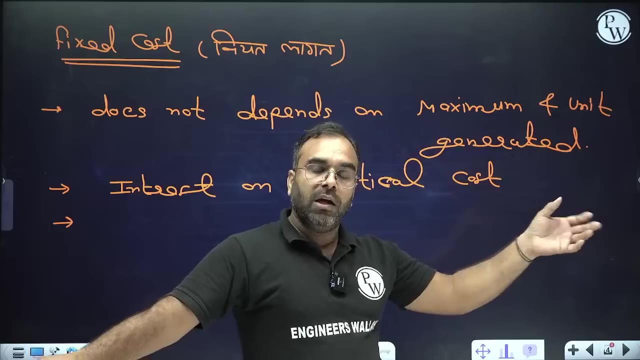 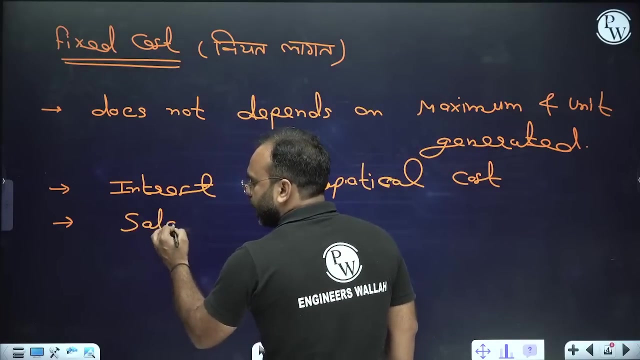 you all know that when you are running a project, then you go to take money. you are a businessman. what, what project do you have to make? what is needed? for that? a skillful, knowledgeful person is required and you all know that. who comes in? that? the big hire officials. ok, the big hire officials, their money will also go and who will go? that will also come in the same fixed cost. so here, keep in mind salary of, salaries of of higher officials, right, salary of higher officials. 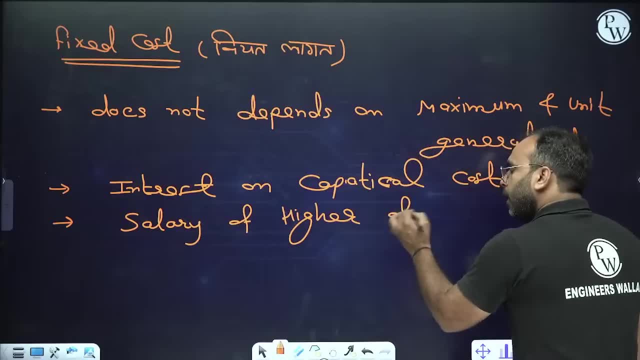 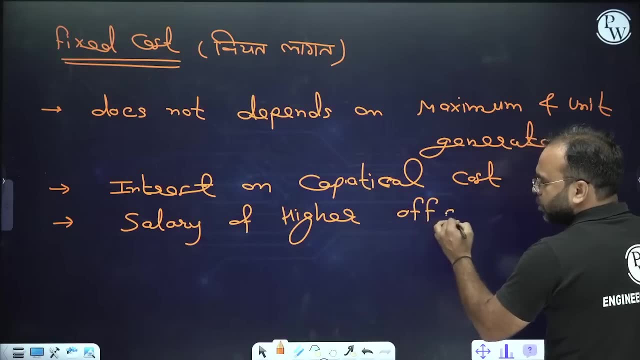 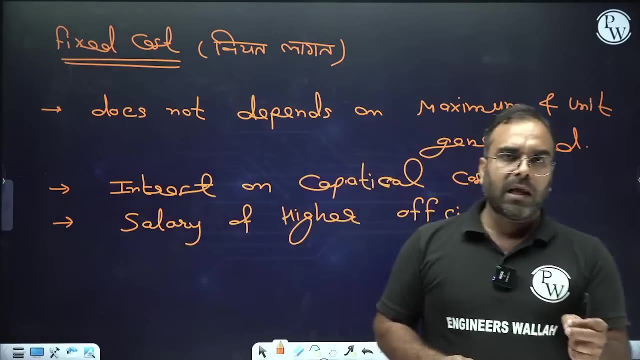 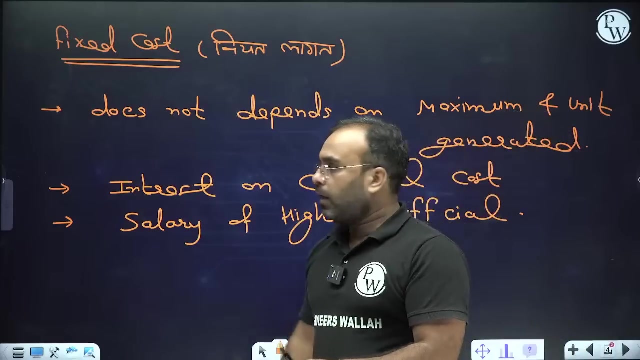 All the higher officials that we have will only come there to see. they will not do that work, they will just give you instructions. so the salary of higher officials will also be included in this. so one is the interest money, one is the salary and one is that the government also gets some money. so all that will come in fixed cost. what did I say? what will come in fixed cost? 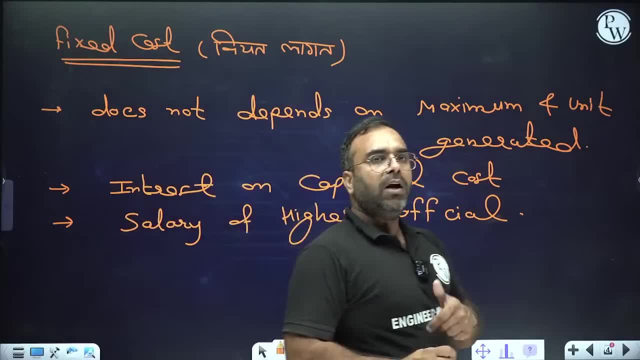 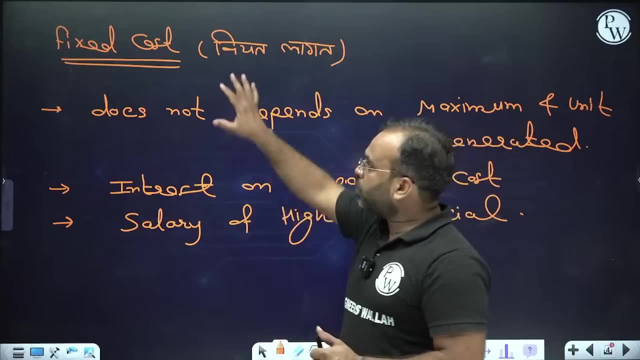 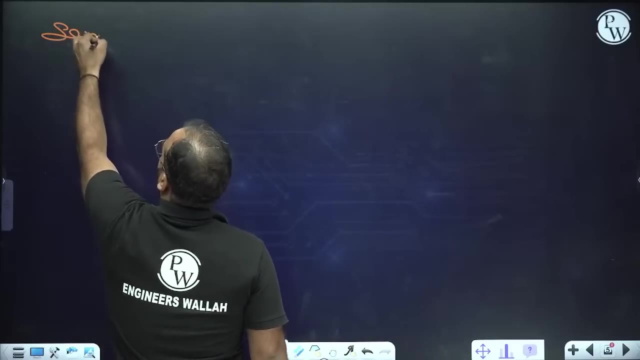 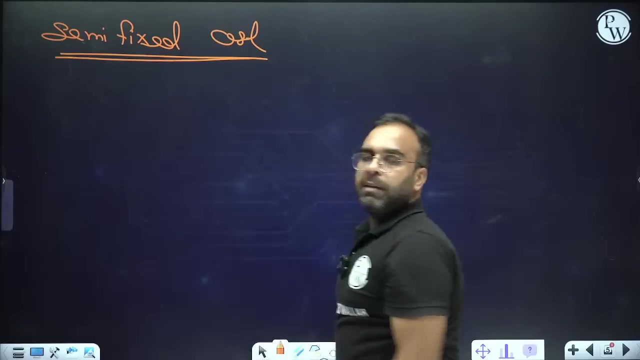 the interest will come, salary of higher officials will come and some money will go to the government. that will be included in it. so now we will quickly tell you what will come in fixed cost. if I talk about fixed cost, then we will come to semi fixed cost. next will come semi fixed cost. if I talk about semi fixed cost, then what will be included in it? so see, if we talk about semi fixed cost, then here the thing that will be included will be there. 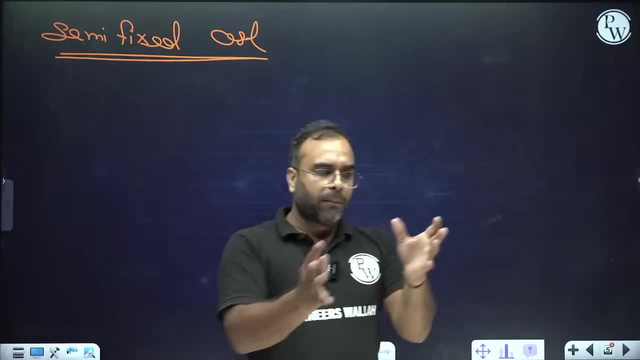 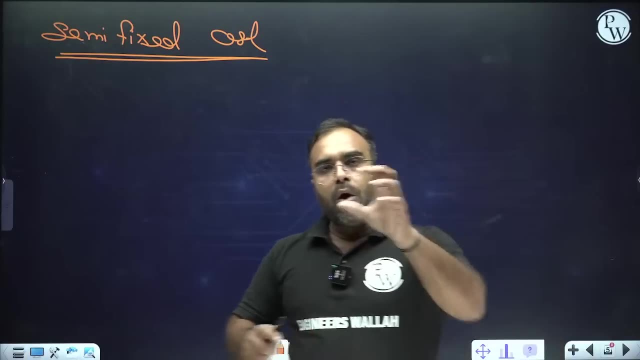 Now you have done the survey for the plant, everything is done. now what do you have to do there? You have to make a plant. you have to make a generating station. then you have to buy equipment to make a generating station. And from where will the money come for that equipment? That too will come from the bank. 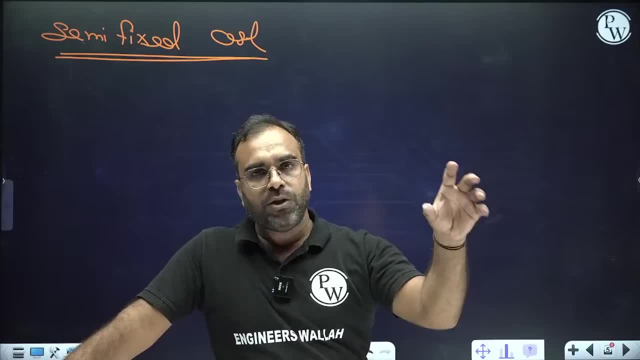 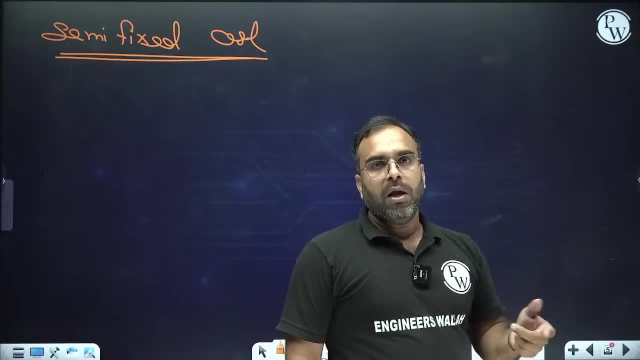 So the interest that is going on the equipment, the interest that is going on the equipment of the generating unit, that will come to you at a semi-fixed cost because that plant has started to be made. So what will come at a semi-fixed cost? The interest will come on the equipment of the generating unit. 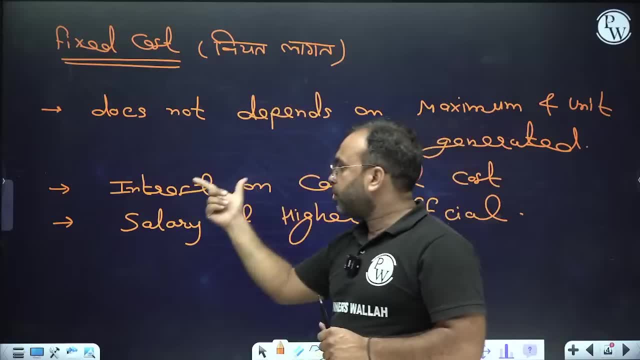 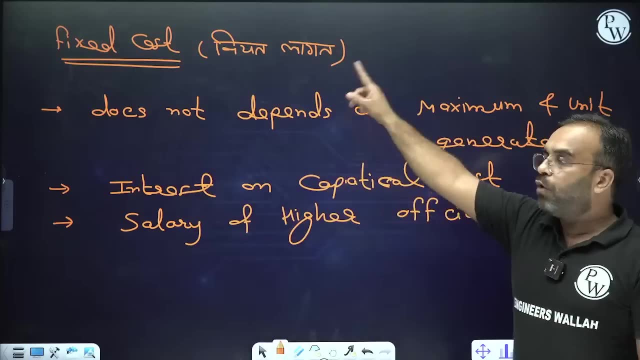 Keep in mind that the interest that is going on, the fixed cost is on the land. The interest that is going on the land that you have bought, where will it come? It will come in fixed, But now you have to make a generating unit. If you are making a generating unit, then see what will come in your mind. 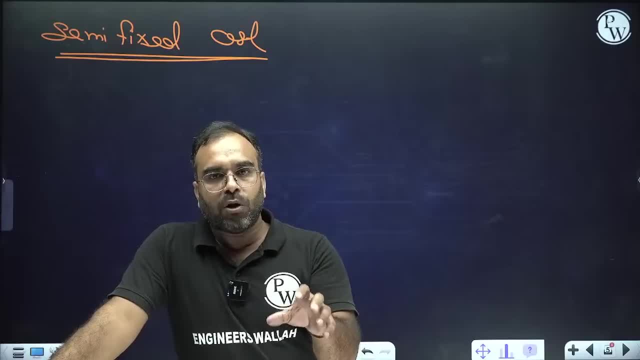 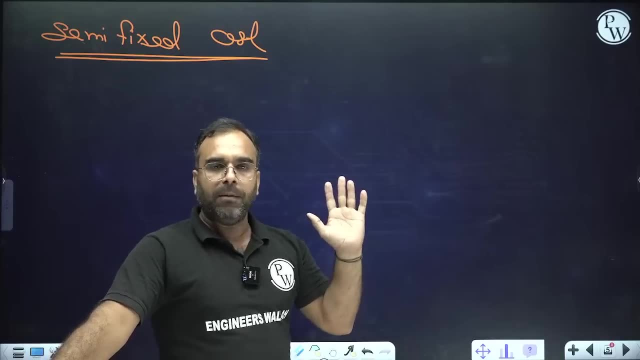 If you want to make a generating power plant, then you will say that I want 100 megawatt, 200 megawatt, 500 megawatt. How many capacity plants will you make? That is when you make a plant. you will not make it in this way. 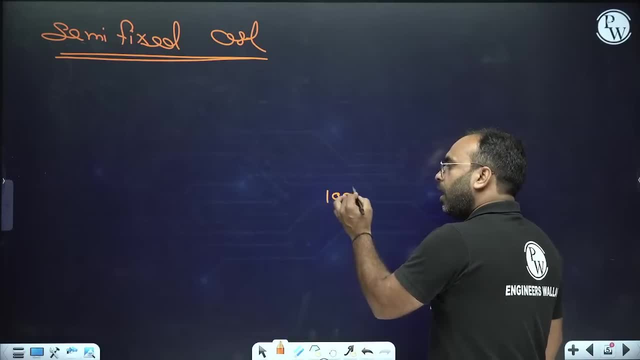 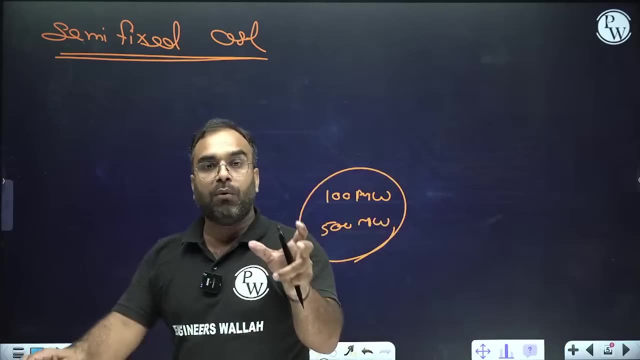 You will first do a survey that. what do I have to do? I have to make a 100 megawatt capacity plant. I have to make a 500 megawatt capacity plant. How many capacity plants do you have to make? You will depend on that. 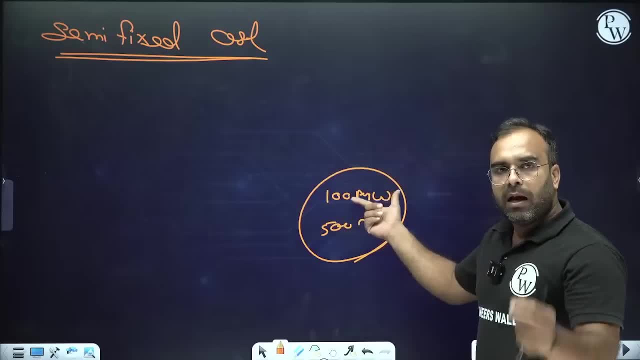 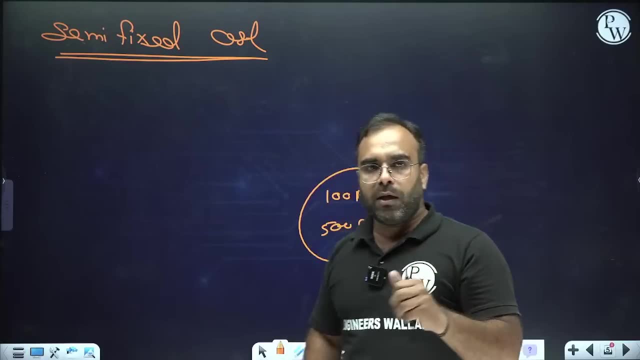 What does this mean? What is this thing? What is 100 megawatt, 500 megawatt? So this is the maximum demand that when you make a plant there, then you will see that how much maximum demand can come on my plant here. 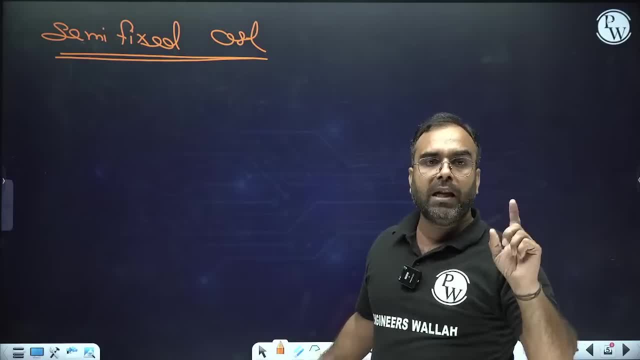 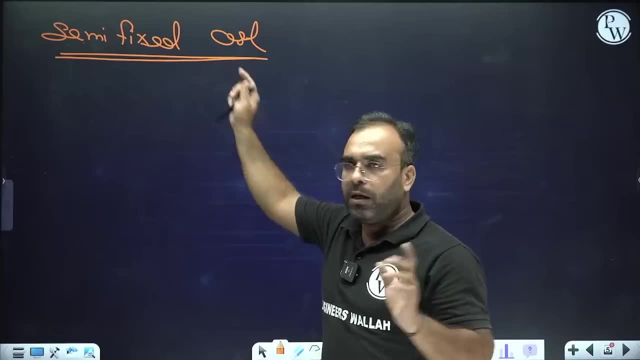 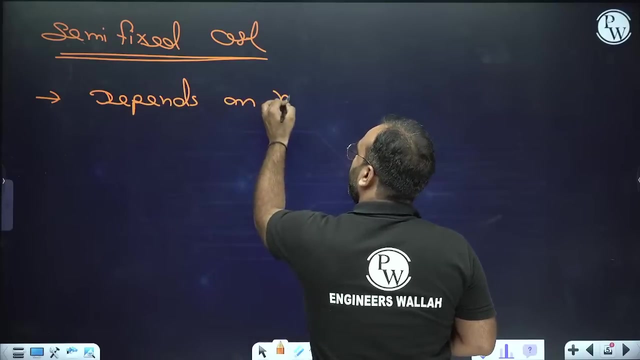 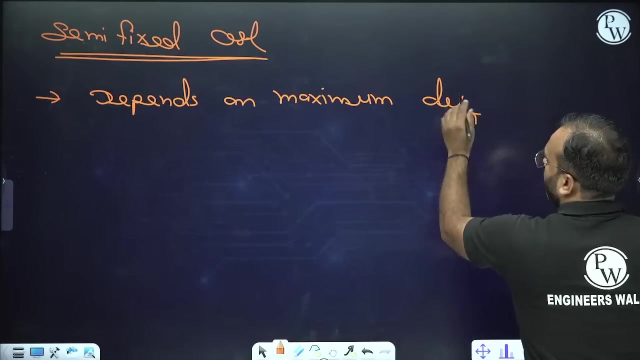 So, according to the demand, I will have to put a high rating generator there. This means that the semi-fixed cost will depend on the maximum demand. So what will be the important point here? So it will depend on the maximum demand. So this thing will depend on the maximum demand. 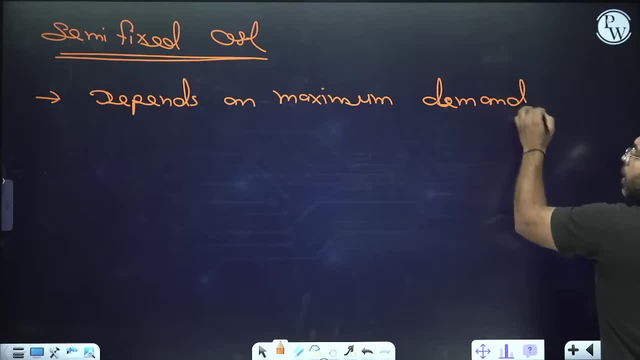 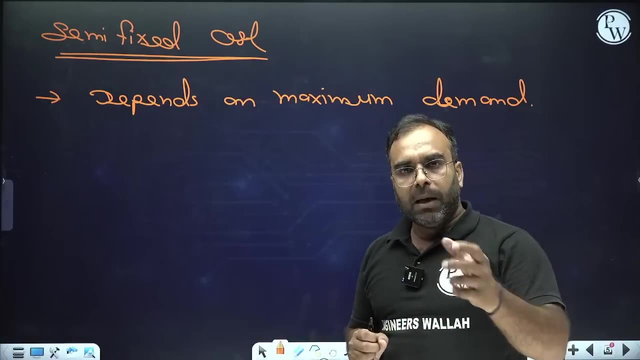 So write here depends on maximum demand, But keep in mind that it does not depend on the unit generated, that it has not started generating yet. Our plant is still being made. Now we have taken the land, we are bringing equipment on the land. 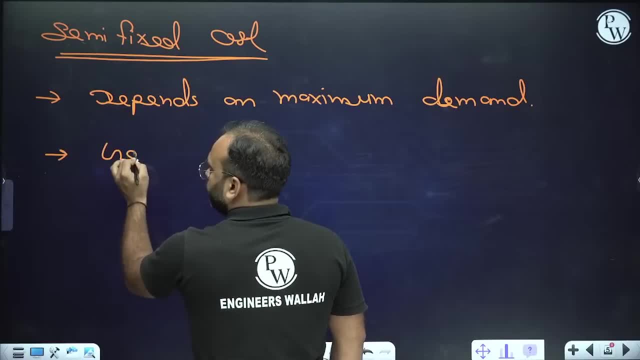 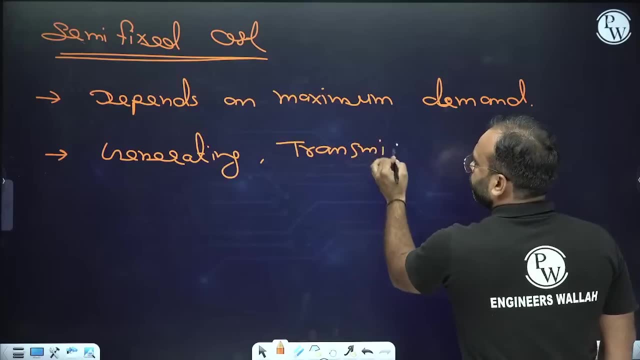 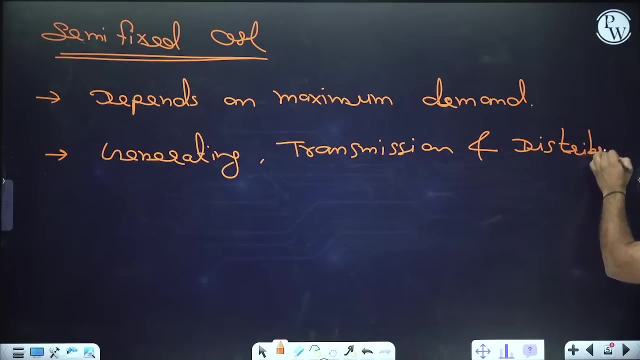 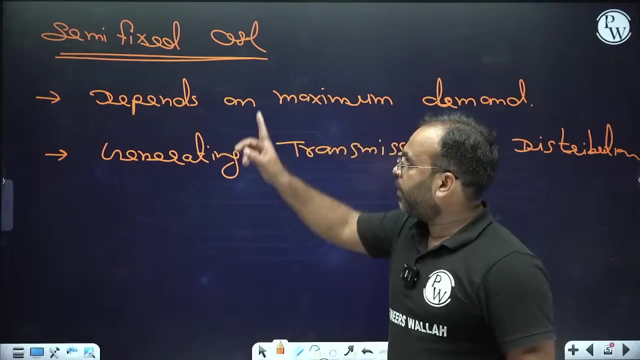 So what will we bring in the equipment, Generation, generating cost. keep in mind generating transmission, generating transmission and distribution network. You will also have to put the transmission line. So here is the generation, transmission, distribution. Whatever transmission line you will put, all the equipment you will put, the cost of all of them will come in the semi-fixed. 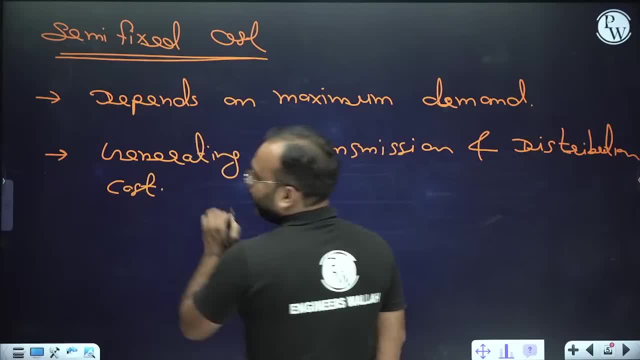 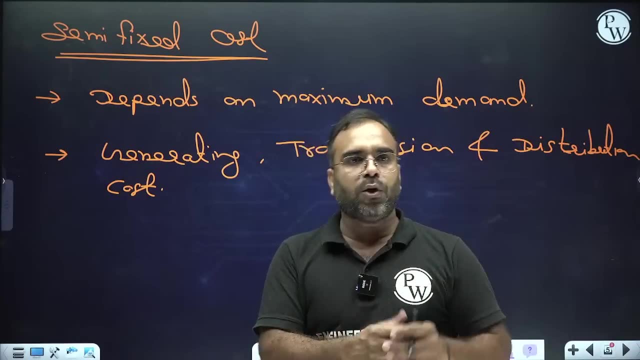 So here the distribution cost will come to us in the semi-fixed cost. Now this plant is just being made. In this you will put a circuit breaker for switch gear and protection, All the equipment you will put. then its cost will also be included in it. 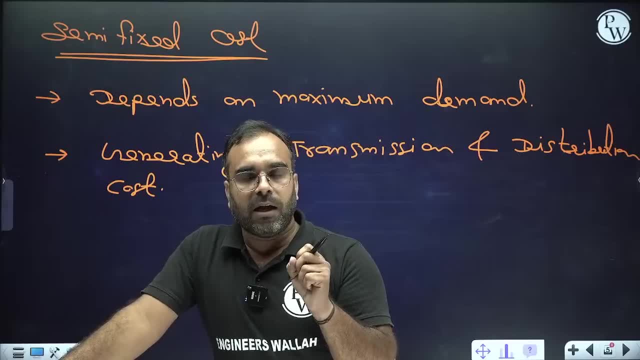 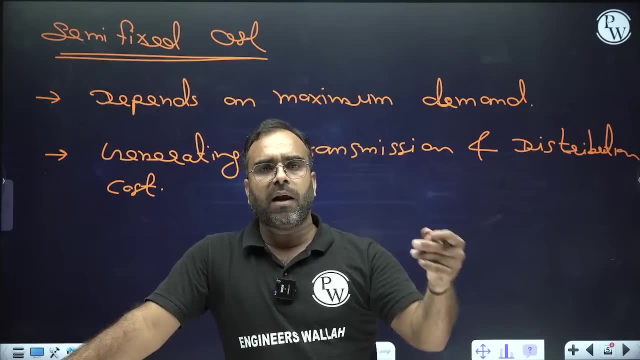 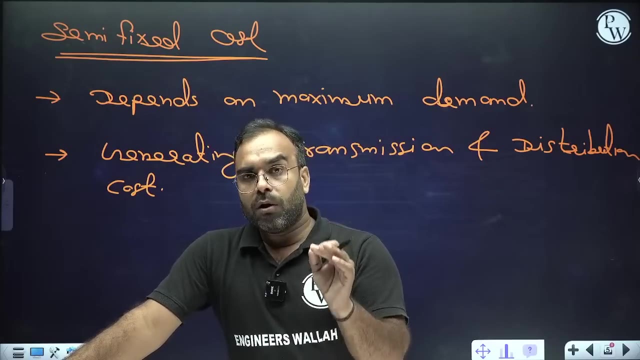 But you tell me if you have started making a plant, then there will be some clerical staff there. Will there be clean workers or not? It is not that the plant is being made there. there is no filth there. All the clerical staff there, their salary, their salary and there is insurance for all of them. 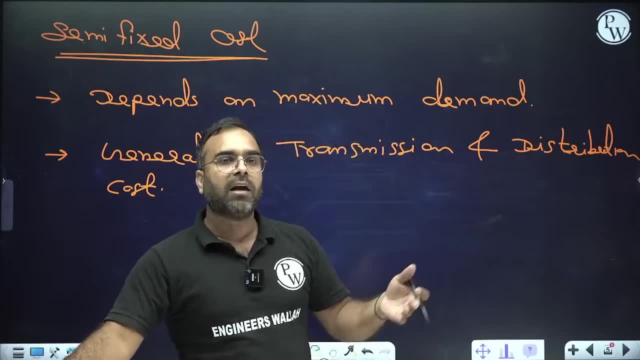 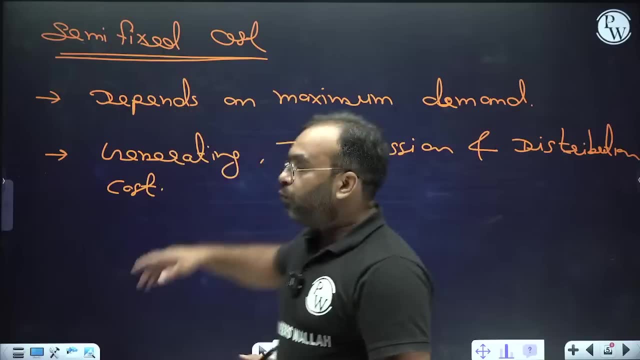 The money of their insurance. suppose if it turns out that a few of them fell in construction, then their insurance money will also have to be given. So all of them have insurance money that will also come in it. This means what will come in our semi-fixed cost. 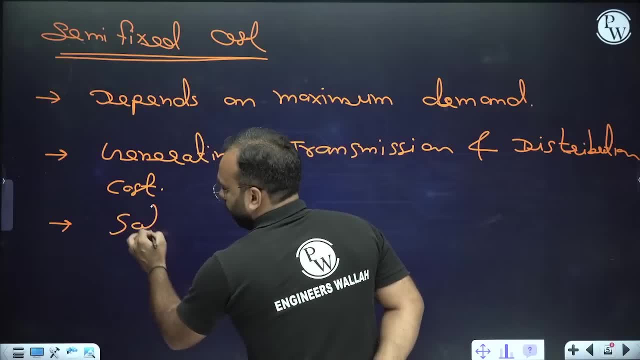 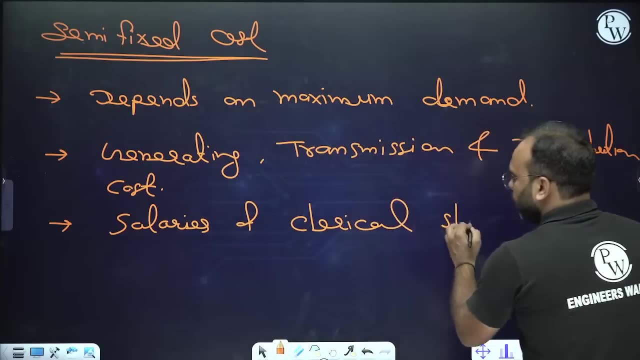 So here the salary will come. So here the salaries of who will be with us. Salaries of clerical staff. What will happen? The salary of the clerical staff will be there Next. after that, if we talk, then all the insurance money will be invested here. 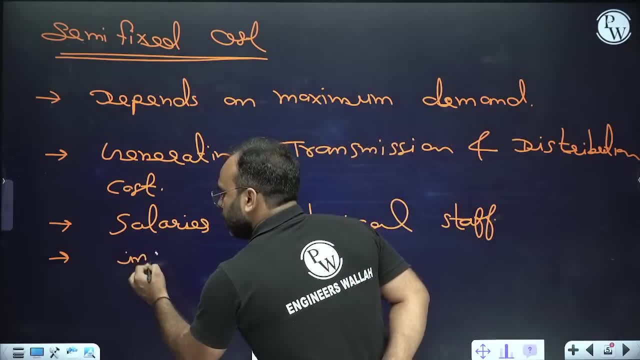 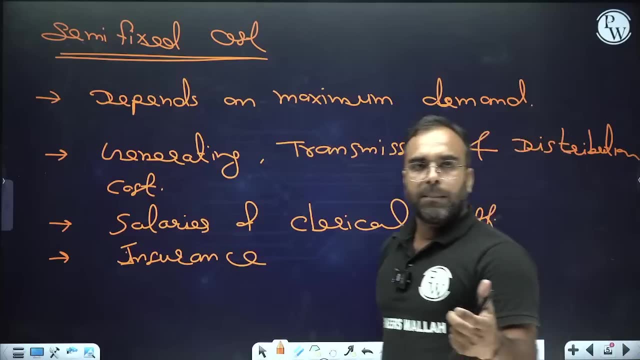 Insurance will be with us Insurance. you also get it done Insurance, so its money will also go. You will also have to pay for it. What does this mean? That is also in our semi-fixed cost. So all these things have to be taken care of. 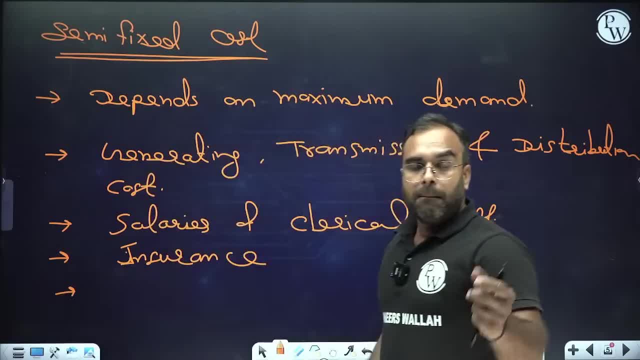 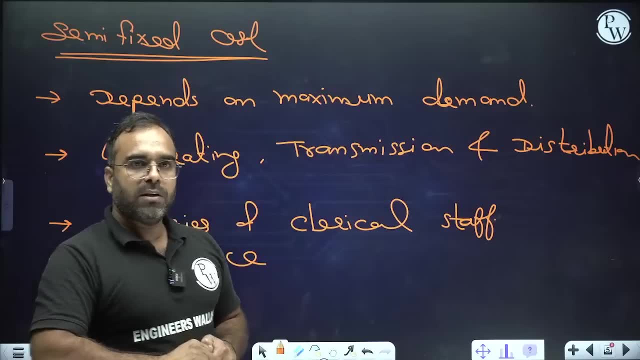 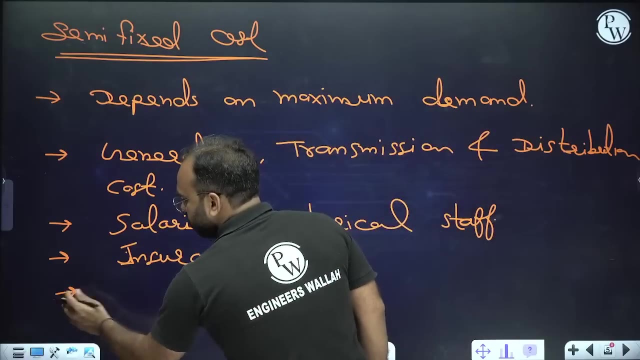 It will be included in it. Plus, all the management there who will manage their salary is with us. Yes, Ajit will definitely read it in the same way. We will read it in the same way. Come here. So this is a crash course. 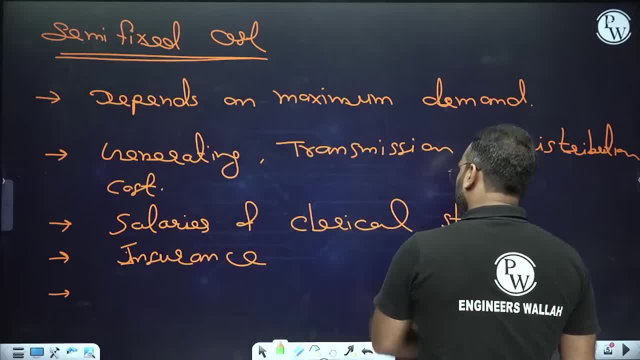 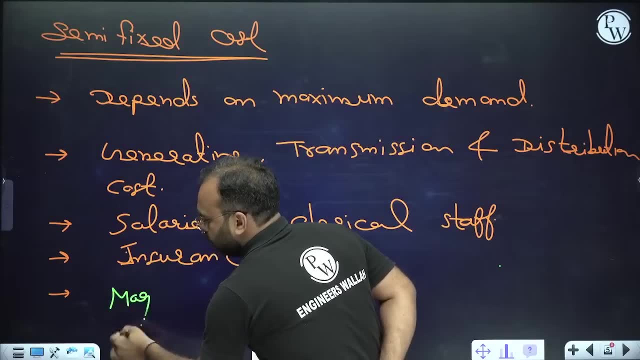 It is a crash course, So we will try in it, We can try our best to cover it completely. So all the managers and officers are there. You can say management, You can say officer. So what will happen here? The salary of management. 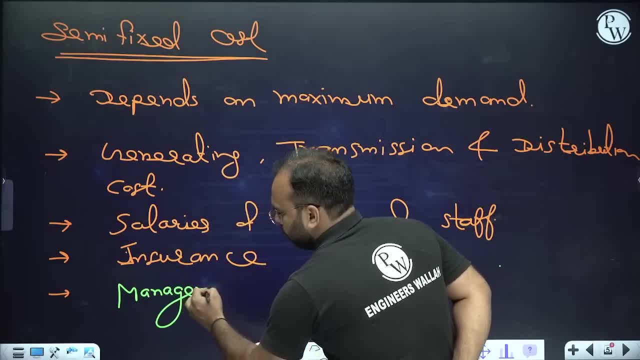 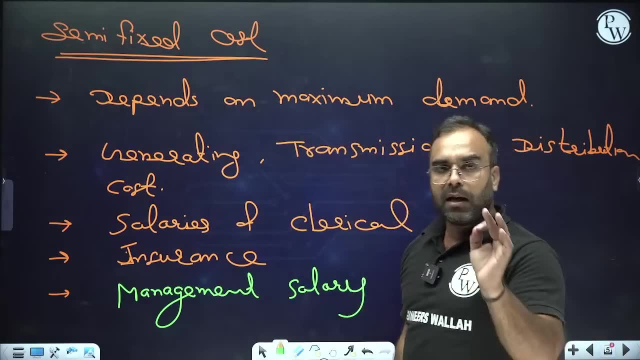 So write it here: Management, Management salary. So what will happen with us All this will come in the semi-fixed cost. But keep in mind the question in the exam will ask. The question in the exam will ask that the semi-fixed cost depends on whom. 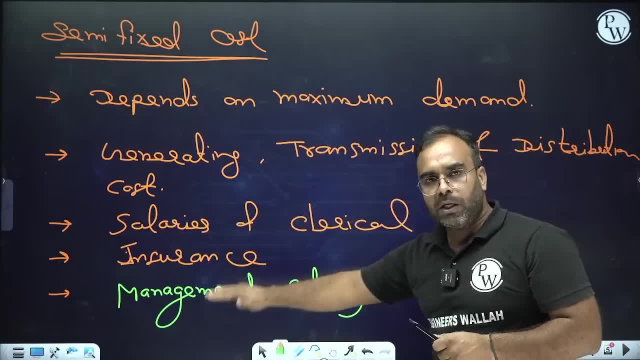 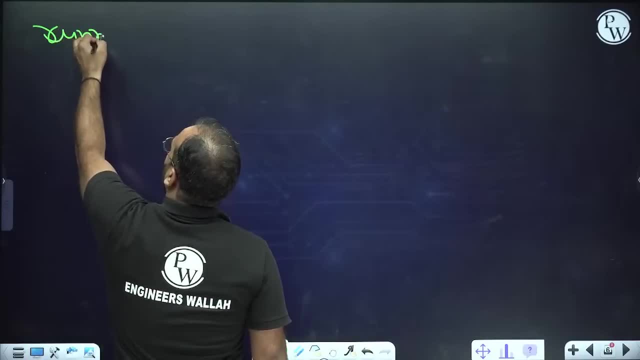 does not depend on whom and what will be included in it Next. after this, our next point will be the running cost. Now you tell me what is required to run the plant. What is required to run the plant? Now you have made the plant. 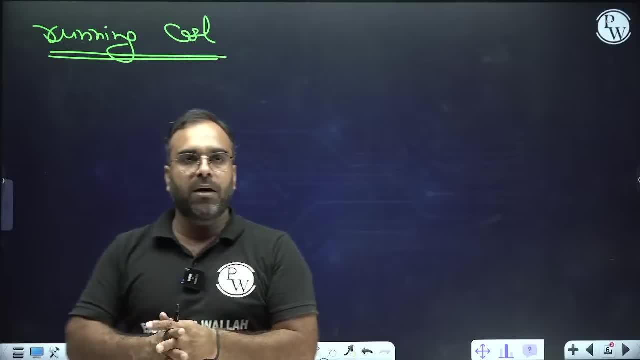 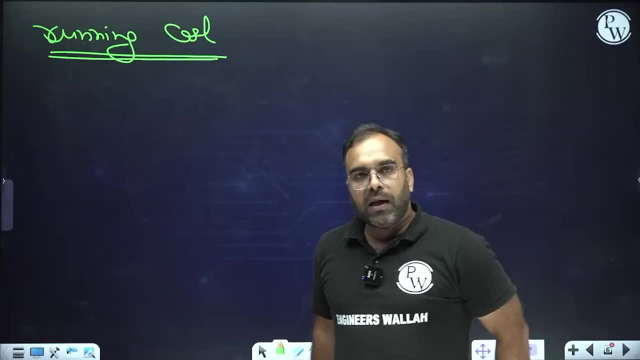 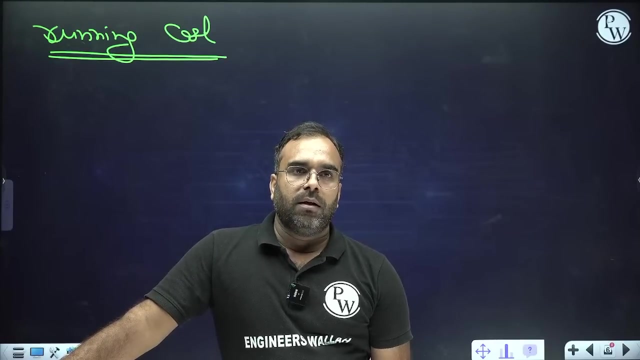 Assume that you have laid the transmission line. You have done all the work. Now the plant is to be made. What is required for running? Tell me quickly, If you want to run the plant, then what is required to run? Focus on your studies. 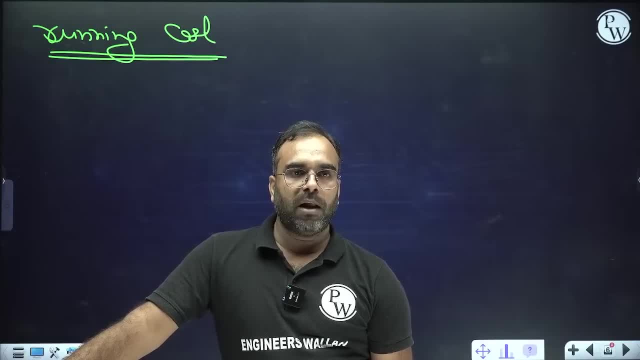 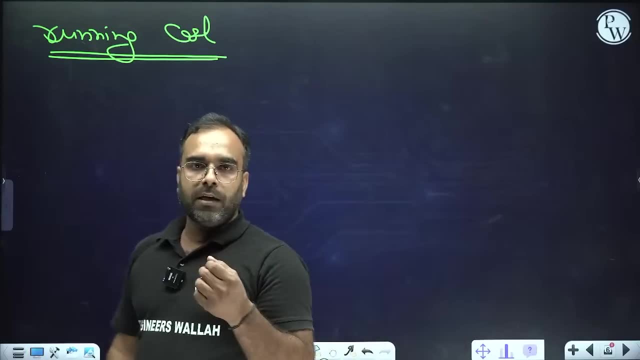 You have to focus on your studies, You don't have to comment anything else. You have to focus on your studies, You don't have to comment anything else. Fuel is absolutely right, Sir. we need coal and coal if we are talking about a steam power plant. 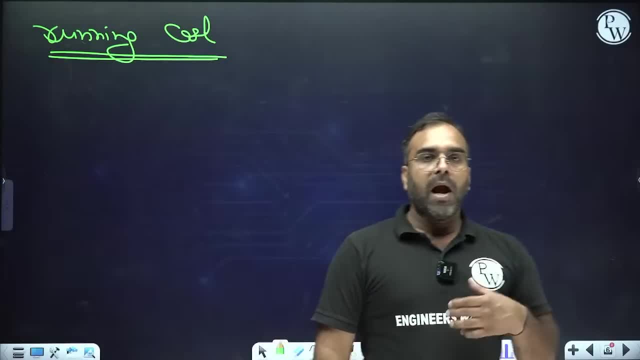 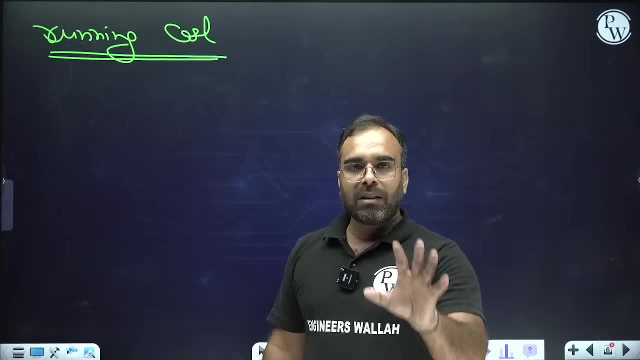 We are talking about a nuclear power plant. We need uranium. We are talking about a hydro power plant. We need money. So this means we need water, not money. Hydro power plant means we need water. This means we need fuel, So the cost of fuel will come under running cost. 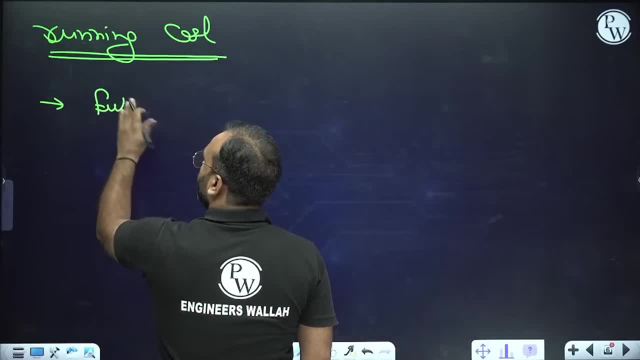 So here you have to pay attention. This will be the fuel cost. Fuel cost. Fuel cost Next, Next, After this. if we talk, then what will happen here? Water cost, Water money will also be applied. Water cost. 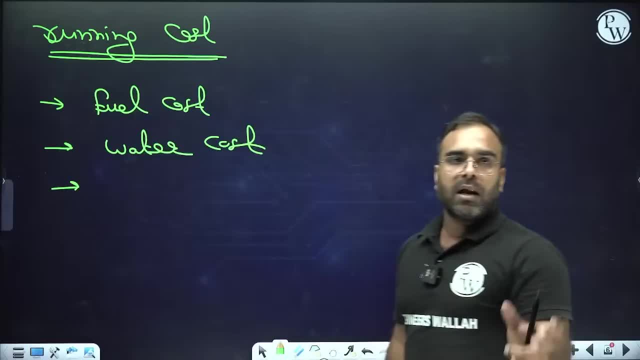 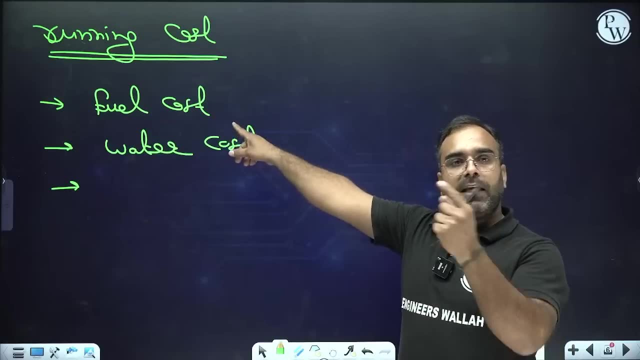 Next, All the lubricants. we will use Lubricants. Keep in mind: You know that we will have to use grease free there. We will have to use lubricants. So the cost of lubricants will also be included in this. 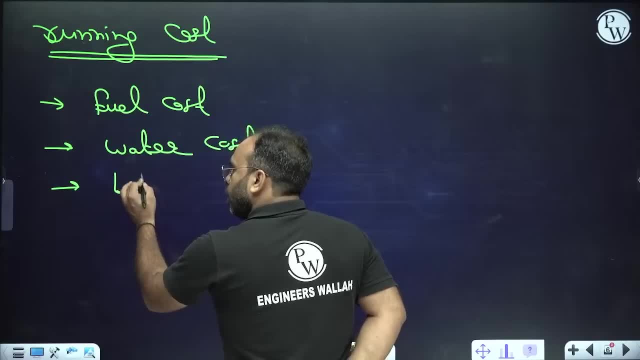 So here Next, What will happen? Lubricant cost: Lubricant: Lubricant cost will also be included in this. After this, if we talk about oil, The amount of oil we will have to use. Its money. 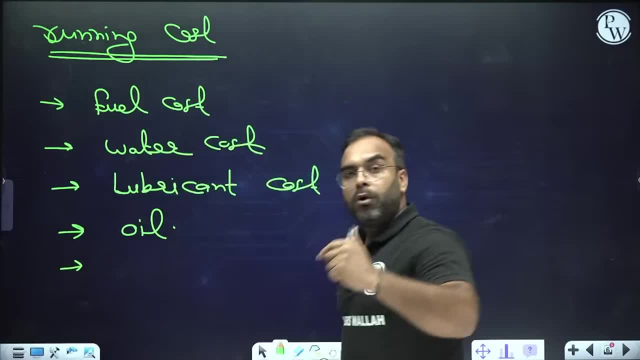 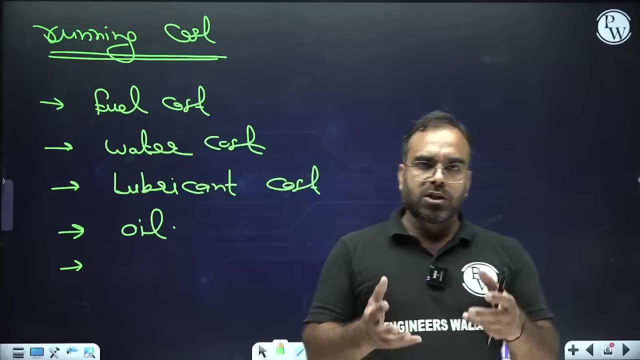 But you know what you will do If you want to do more generation, To do more generation When you have to do extra work there. So what will you have to do for extra work? You need a person who works there more, So their salary will increase. 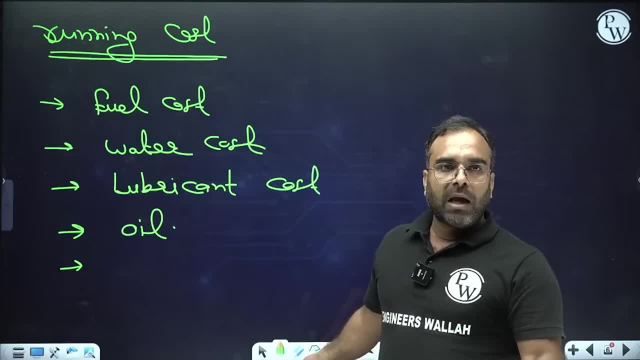 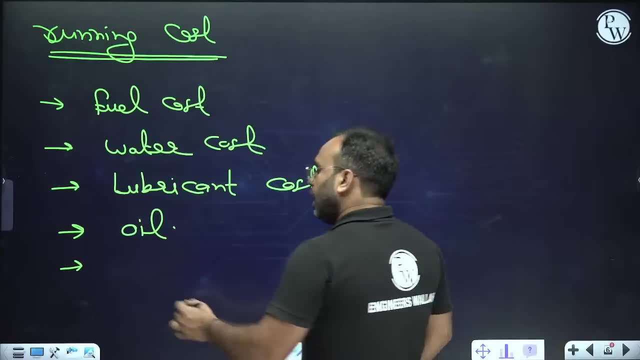 It will be included in this Under running cost. So keep in mind here, Under running cost, The salary of operating staff. You can say, You can definitely say: What do you write So here? What would you write here, Say, lary of. 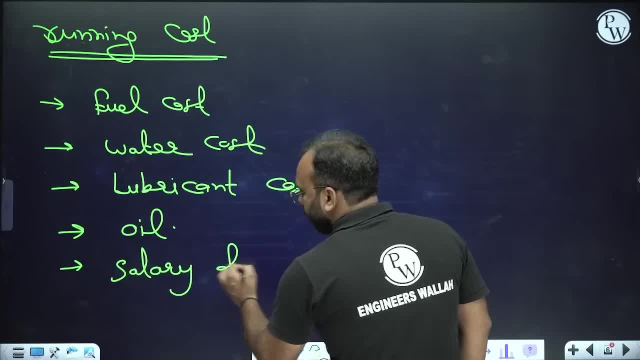 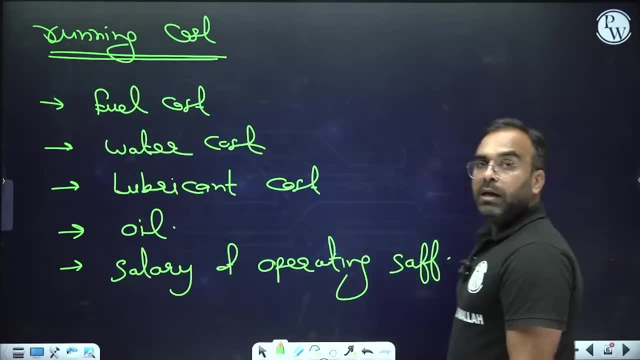 Say lary of, Say lary of. You can say operating staff, Say operating staff, Say operating staff Their salary. What did I say plus, If we have to do more work, We need more persons there, We need more people. 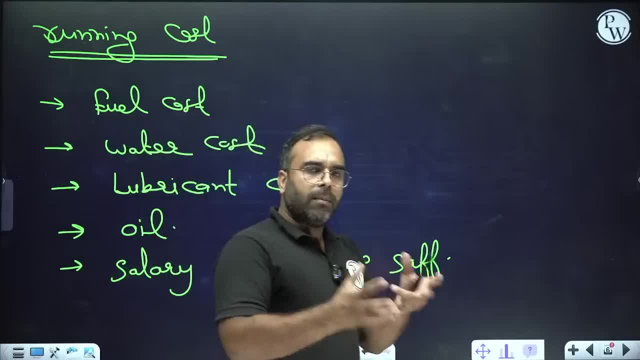 We need more people, Extra worker- So their salary will be included in it too. In which running cost? Now tell me, The running cost will depend on whom. From 10 people you have work now And you don't have to pay this much. 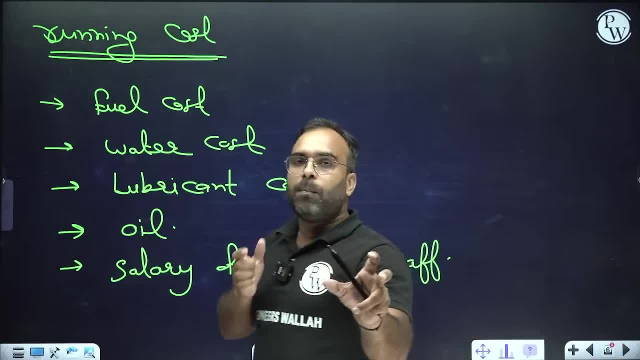 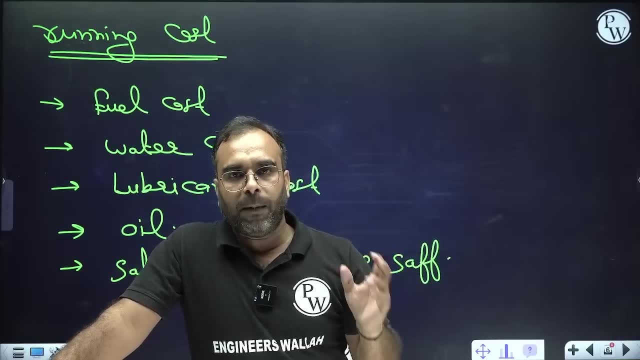 In discussing After from break. I will give you the cost, But in a new episode We will discuss work with 10 people, work with 20 people, work with 30 people. on whom will it depend? So you know that it will depend on how much you have to generate. 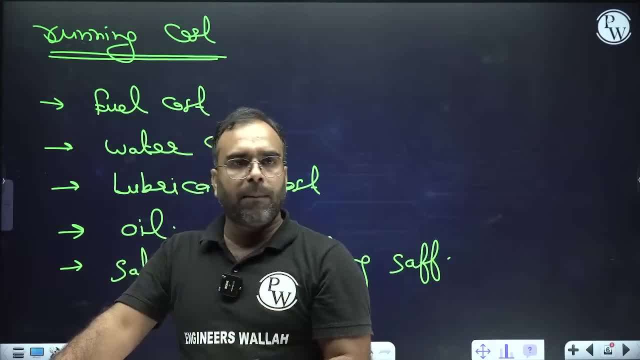 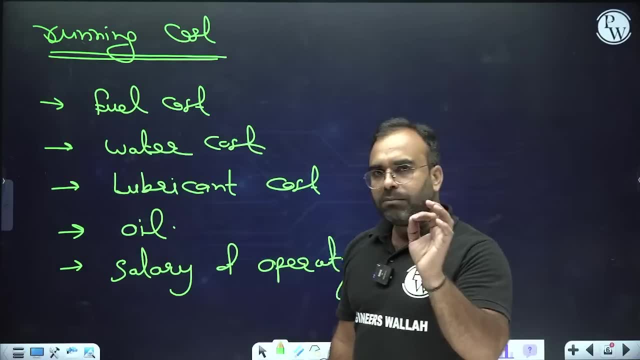 If you want to generate 100 units, then according to that we will need money. lubricants will be used there. If we want to generate 200 units, then according to that, lubricants or fuel will be used. This means that according to the number of units to be generated, 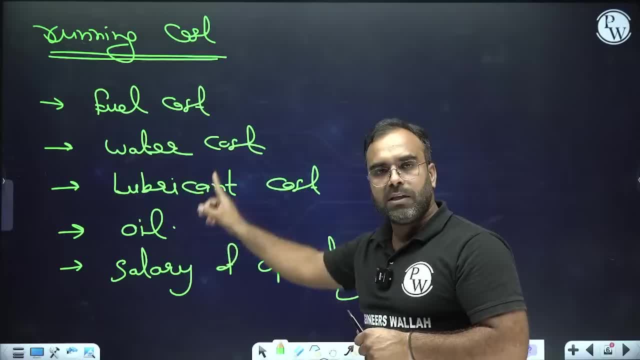 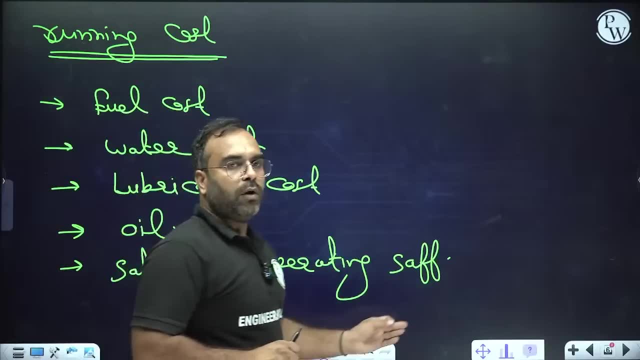 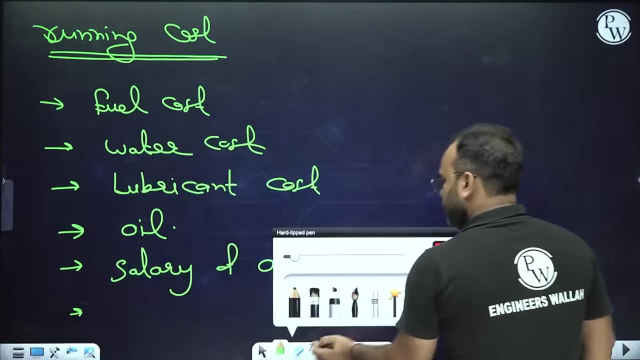 our fuel or the salary of all these will be affected. This means that it will depend on the unit generated, right? Yes, questions like this will be better. You will also get questions like this. There is no problem, So keep in mind here what will come in this. 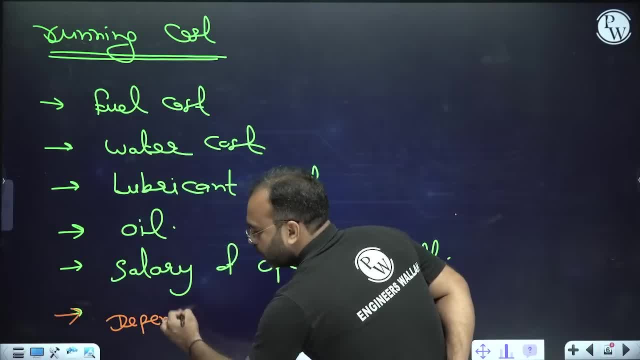 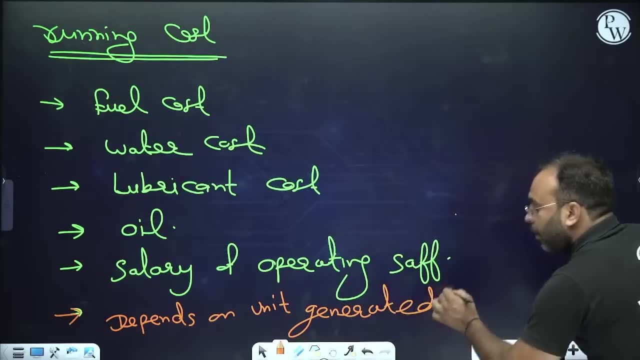 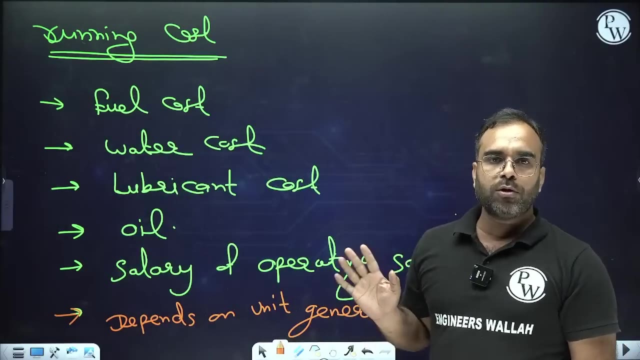 So it will depend on whom it will depend on. So keep in mind, it depends on the unit generated. It will depend on how much our running cost will go. But yes, you have examiner experience. He asks such a question that what is the highest running cost of which plant? 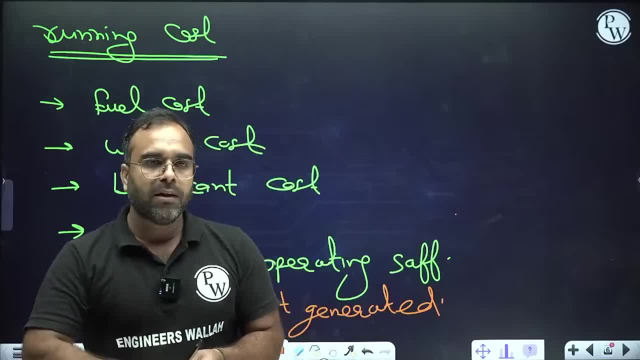 We will tell you quickly by commenting once: Man, that juice is not visible, right? You don't have to finish the juice, right? Okay, you don't have to finish the juice. Juice is still 1 to 1.5 months left. 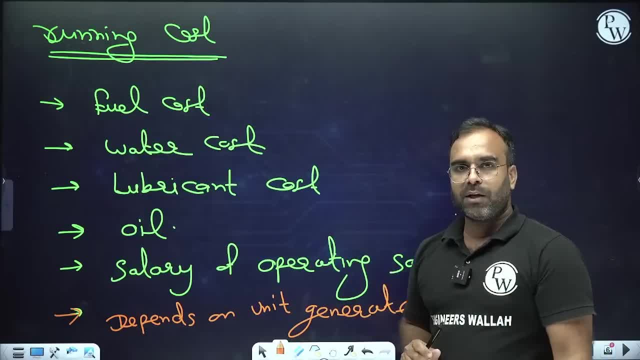 Till then you have to make juice and keep it, And till then you have to make juice for men's also, Because after 50 days you also have a CBT 2 exam, right, Okay, come on, tell me quickly here. 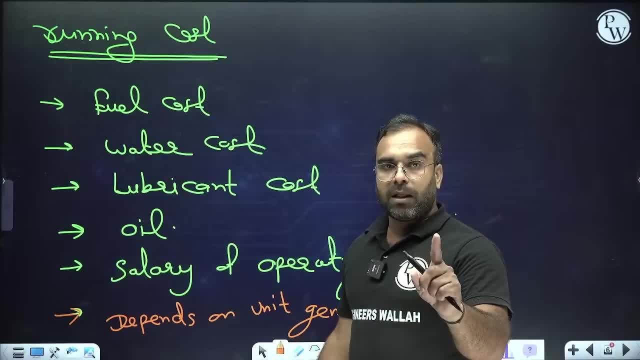 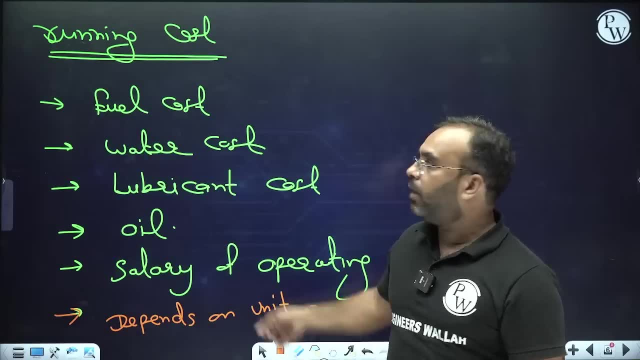 What is the highest running cost? If you are asked, I am talking about running cost Money for running. Where will the most fuel be used? Thermal power plant, steam power plant? The correct answer is that it will not be used for nuclear. 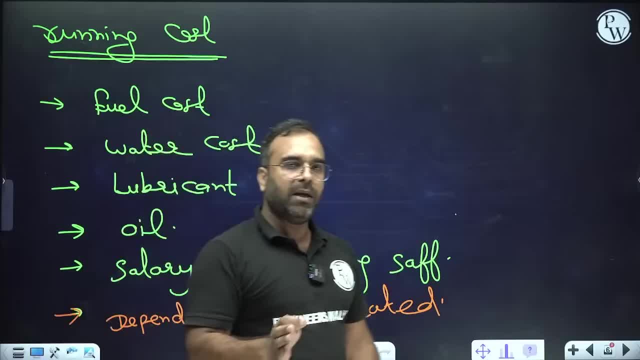 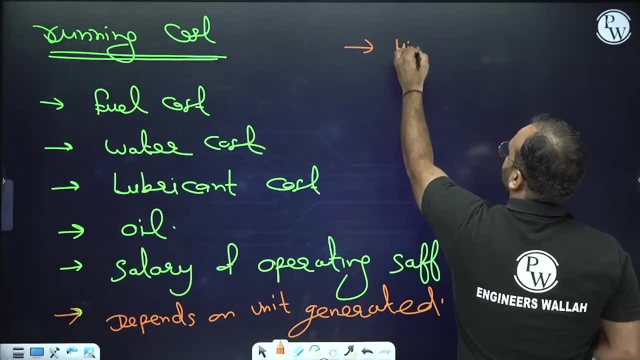 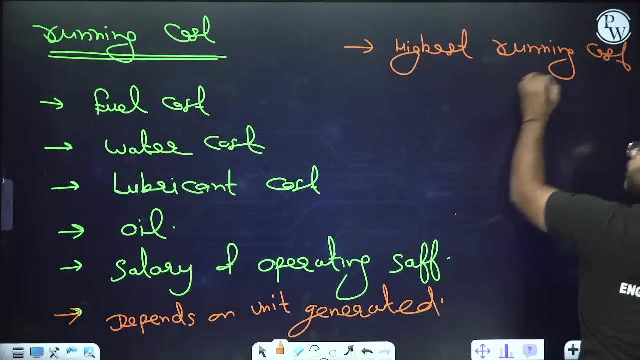 The highest running cost will be the running cost we will have. Nuclear, sorry steam power plant or thermal power plant, right, So write it here: What is the highest running cost? Highest running cost. The highest running cost will be the highest running cost we will have. 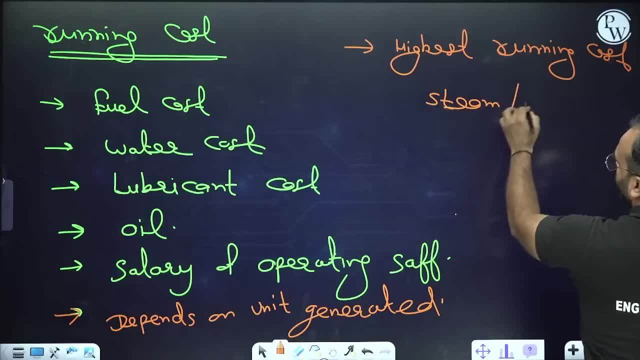 Steam power plant. steam or you can say thermal power plant. You can give it in any option, Right? Both have the same meaning. The cost of steam or thermal power plant is the highest. We will have the highest cost. Come on, tell me quickly. 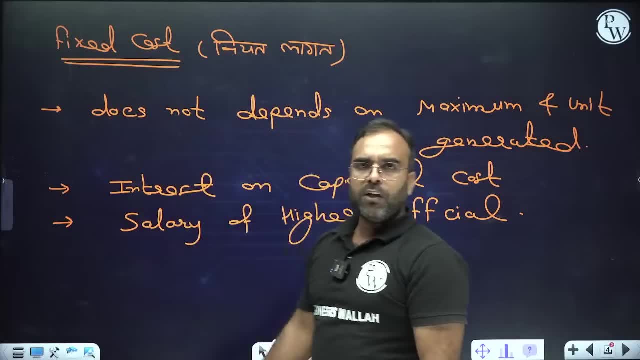 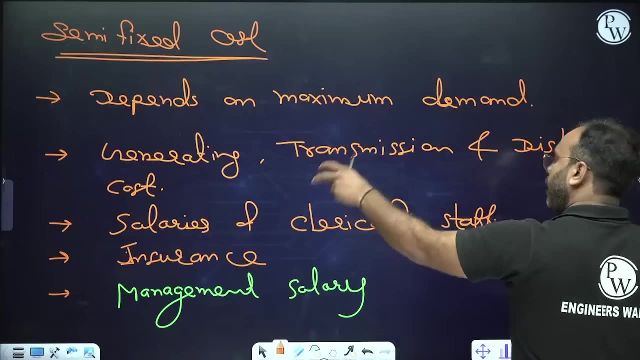 If we talk about fixed cost, fixed cost, If we talk about fixed cost, we will talk about the most. Come on, we will talk about fixed cost later. See, it has become fixed, It has become semi-fixed And we have running cost. 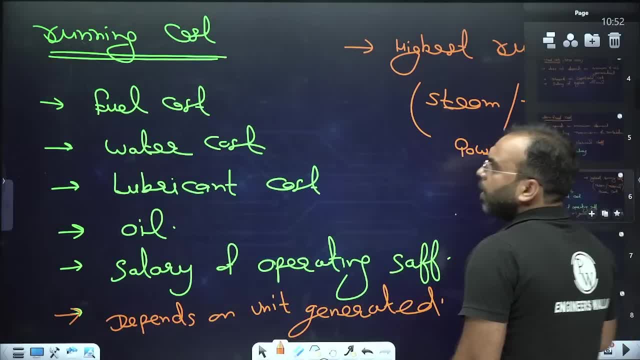 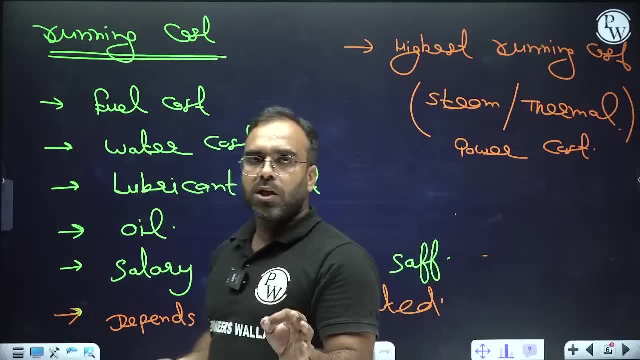 We have three types of cost. If, let's say, you are told that whose is the highest construction cost, right, Whose is the highest construction cost. So what will be the answer? Someone is saying, sir, the lowest cost. 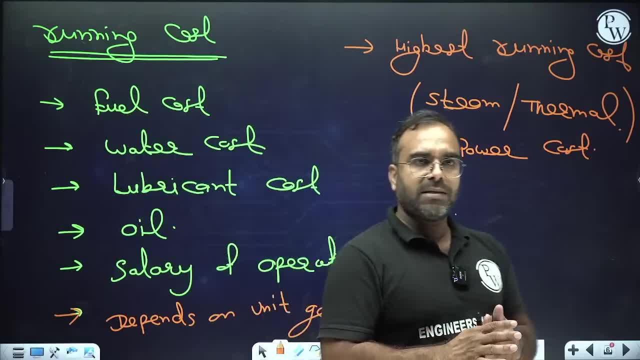 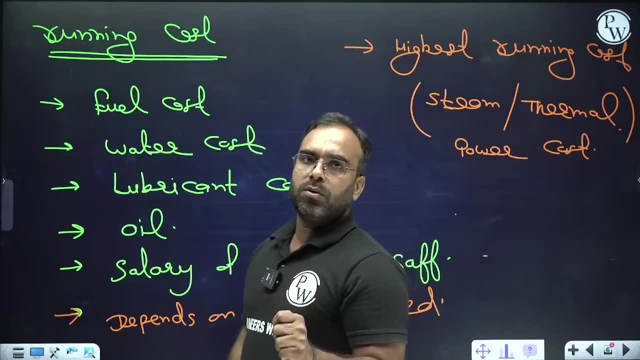 See, here the question is asked in different ways. We have to give the answer in different ways, right, Come on, tell me quickly Whose is the highest construction cost, When you have to make it right If he is talking about construction cost or designing cost. 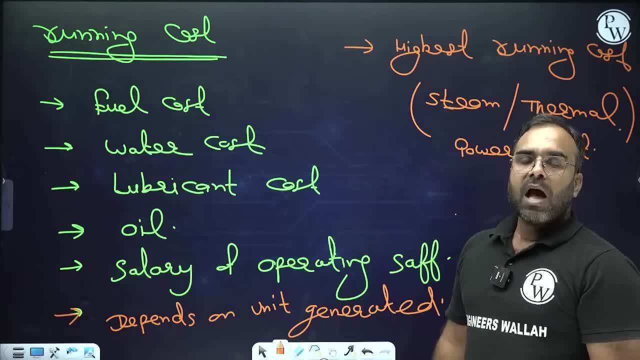 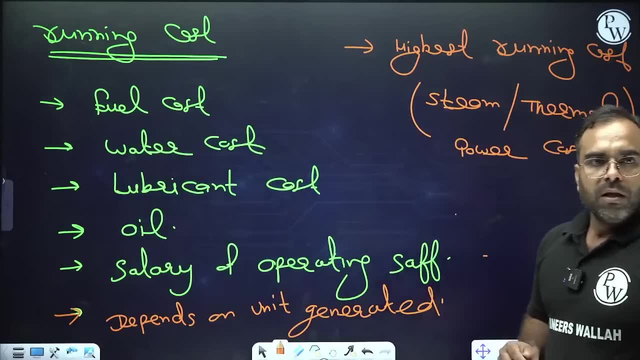 then hydro power plant will be the highest. Very good Hydro power plant. I will make you a table at the end. Whose is the highest cost? We will talk about all that, right, Come on, if we talk from here. 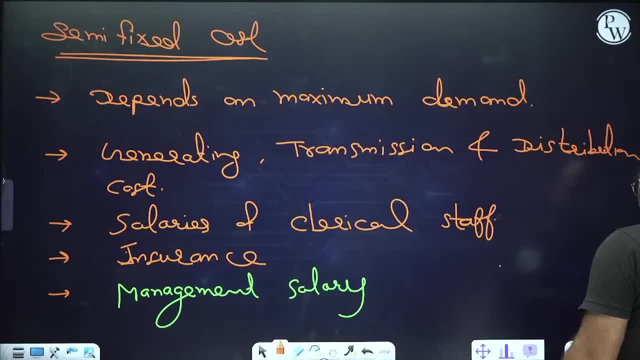 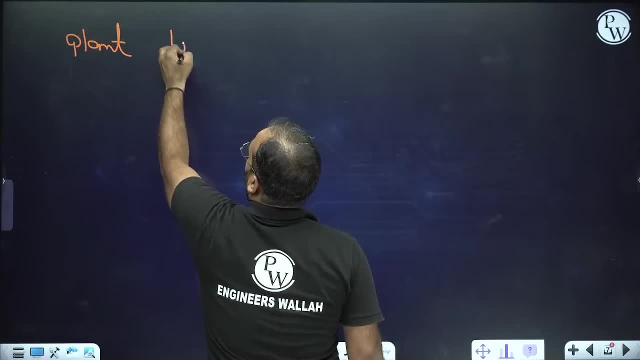 we have three types of cost. Now the examiner asks you about plant life. About plant life, whose is the life of the plant? If I talk about plant life, tell me quickly. what is the life of the hydro power plant If you are told that? 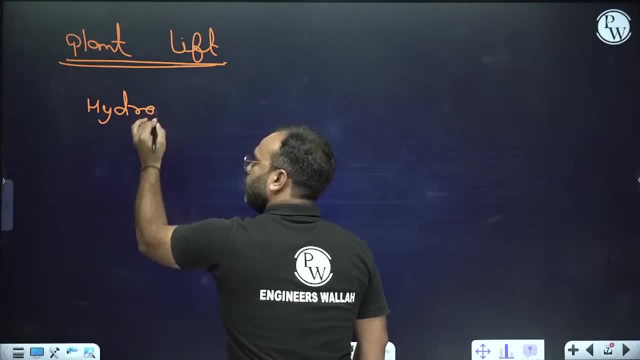 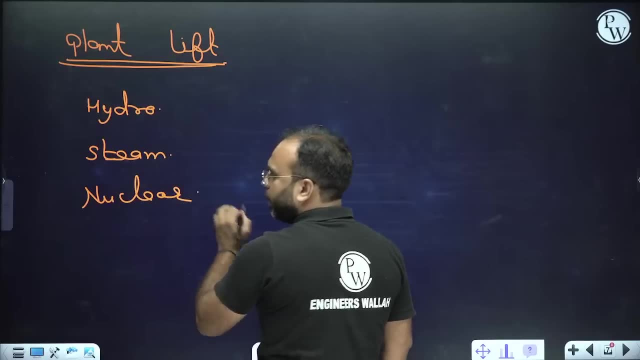 what is the life of the hydro power plant, Hydro? then after that I will say: what is the life of the steam power plant? Next, the next person will ask you: what is the life of the nuclear power plant? Next we will have 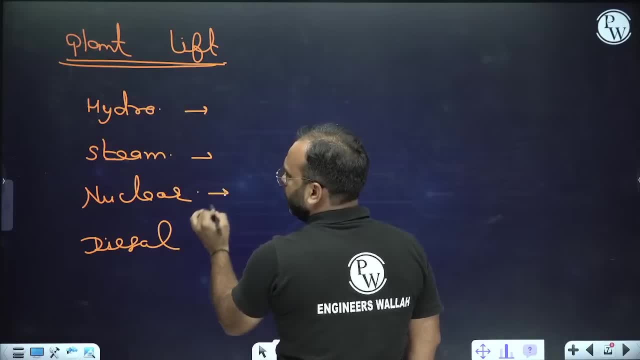 what is the life of the diesel power plant- Hydro, steam, nuclear and diesel? Tell me quickly. Hydro is called water power plant, steam power plant, nuclear is called steam power plant and diesel is called diesel. So if we talk to everyone, 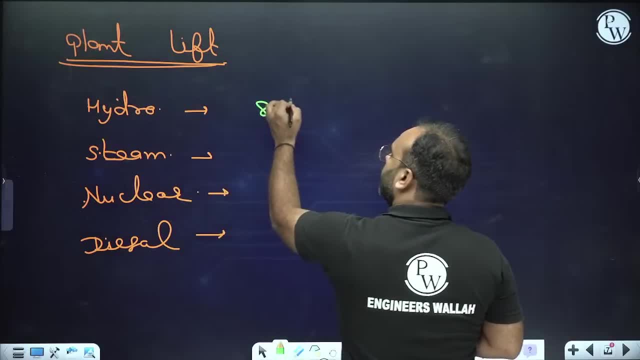 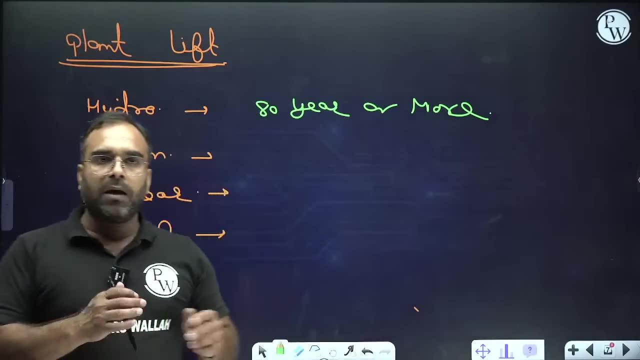 the life of the hydro power plant. keep that in mind: 80 years, 80 years, or what will happen to us? it will be more than that, right, More than 80 years, we will have hydro power plant. Come on, so see. 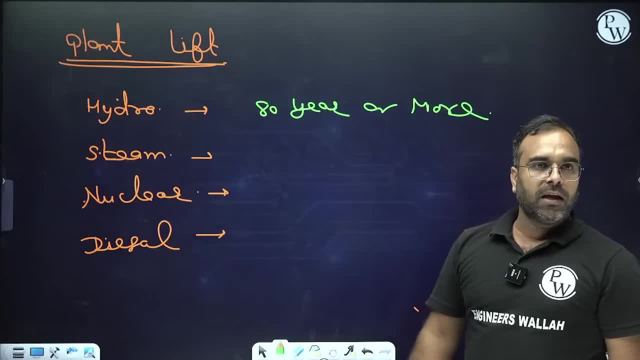 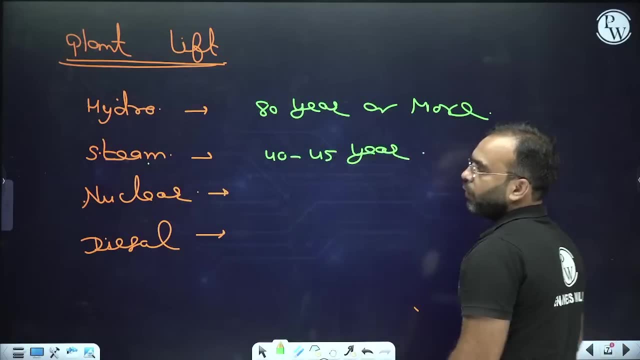 if we talk from here, then it will be more than 80 years or more. Next, if we talk about steam power plant, then keep in mind 40 to 45 years. its life will be. here means once you make a steam power plant. 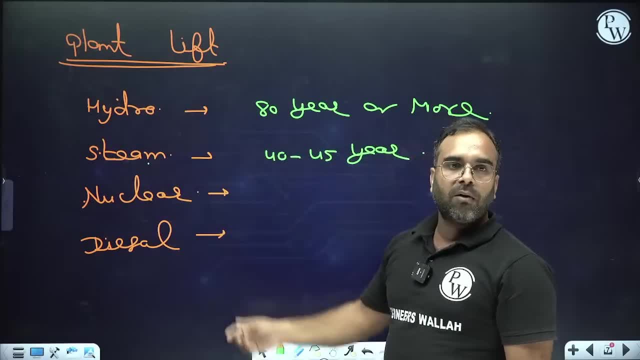 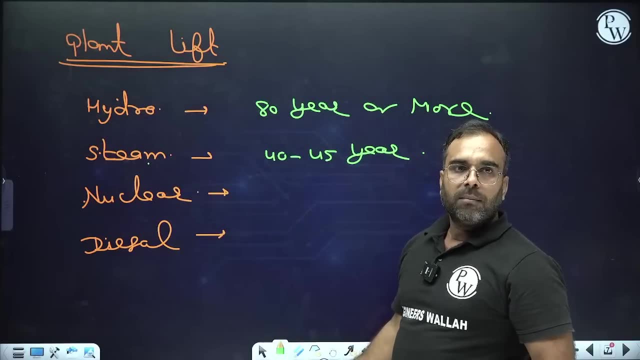 then in 40 to 50 years, what will happen to us? Son Priyanshi focus here. after the crash course of the machine, son, do revision, do revision properly. right Now there is no machine, there is power stream going on. 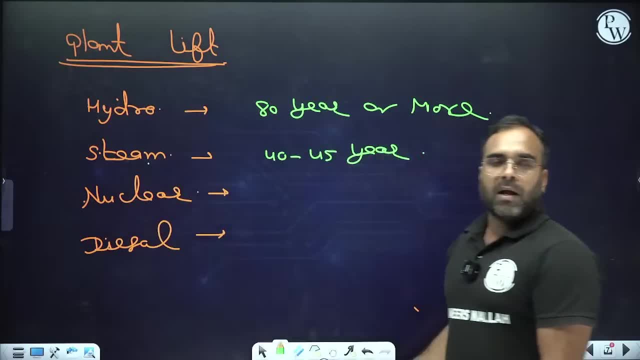 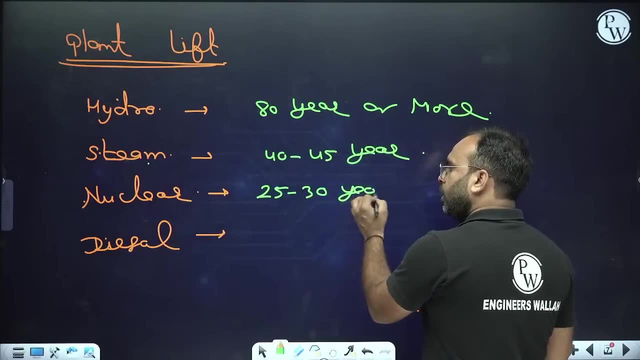 once. focus here, come on next. if I talk about the nuclear power plant, then the life of the nuclear power plant, how much we have 25 or 20,, 25 or 30 years, maximum, that is, we will have this much. 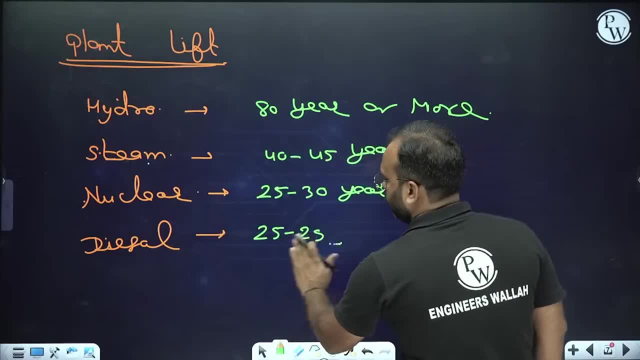 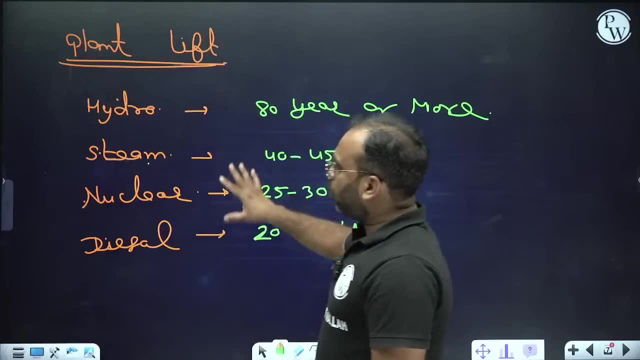 and about the diesel. we have this much about 20,, 25, that is the life of the diesel power plant. that will also be with us. so what will happen? in total, we have 4 power plants, mainly. 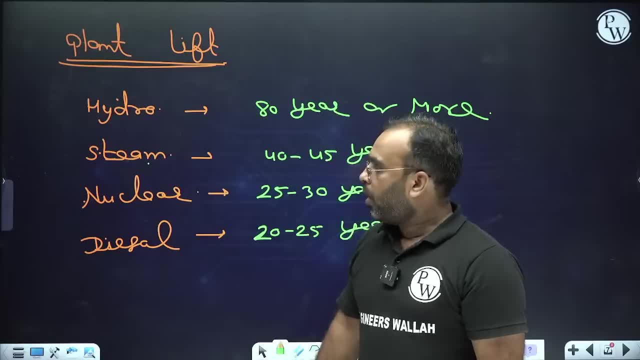 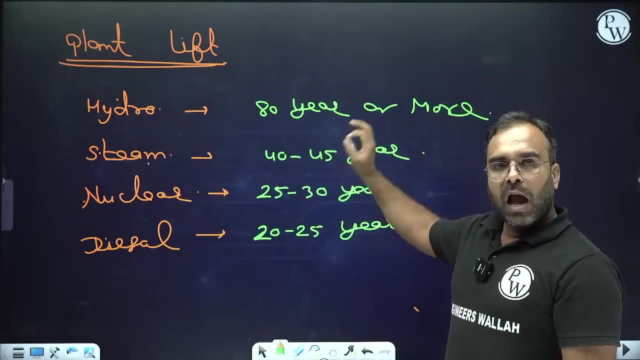 many questions are asked, but we will also talk about non-conventional here. we will also talk about non-conventional, so remember the life of hydro, steam, nuclear and diesel power plants. okay, you will be asked by the examiner. 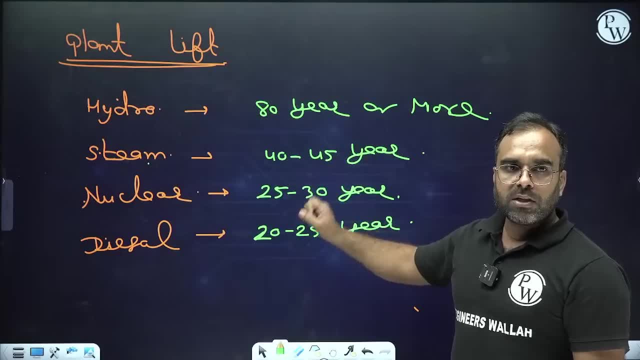 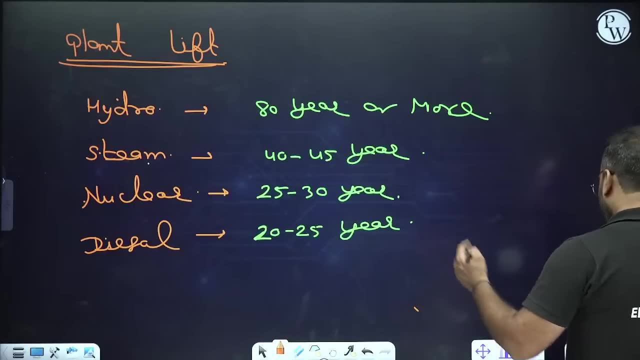 whose life is how much you can tell from here. next, after this: if we talk here, and what will the examiner ask, then we come here. the part of cost has been done. next, we will talk about depreciation. next, we will talk about depreciation. 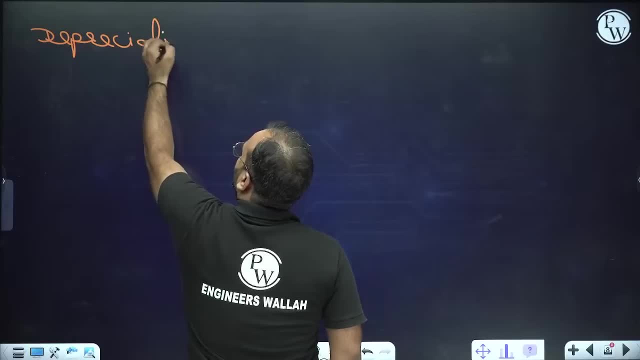 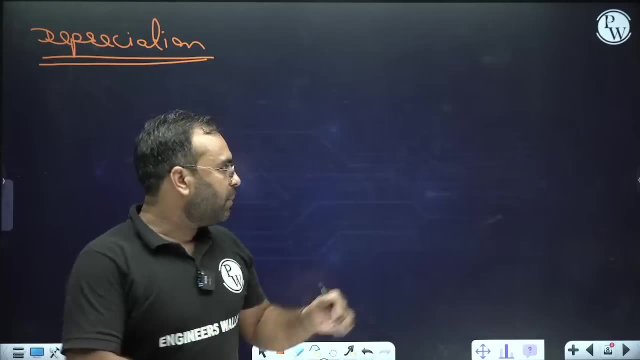 depreciation. so in depreciation, if I talk, that is, you will be asked by the examiner what is depreciation? so let's say, if you buy a phone, let's say today you have bought a phone for 25,000 rupees. 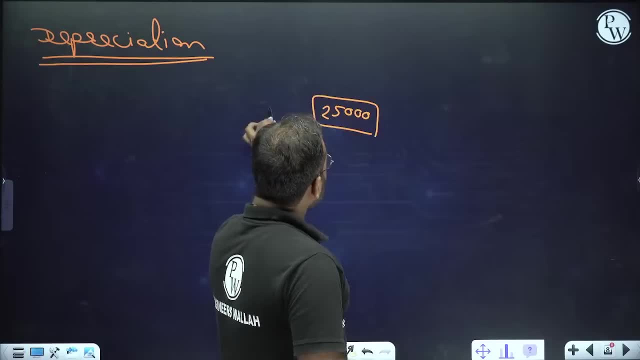 let's say I tell you tomorrow you have to sell it. if today, if you come with a phone for 25,000 rupees and after that I tell you you have to sell it after 2 days. 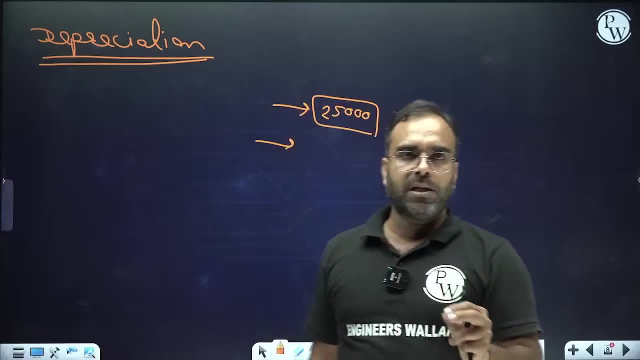 will you get 25,000 rupees? tell me quickly, if you are told, what is depreciation, what is the meaning of depreciation. I am explaining to you, that is, if you buy a phone for 25,000 rupees. 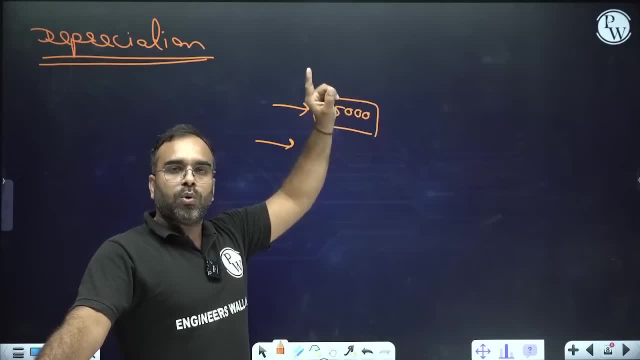 that is, if you buy any equipment, then what will happen here? that equipment, if I talk about the next day, it will not be of that much money. what will happen? there will be a slight decrease in its value. what will happen? 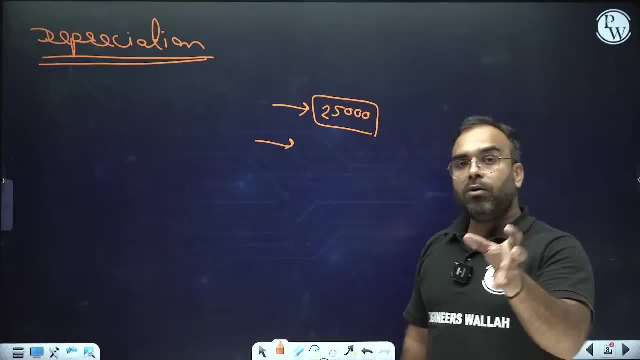 its value will gradually decrease, isn't it Okay, many are saying only 15,000 rupees. don't fall so much. if you come with a local company Chinese phone, then I can accept 15,000 rupees. but if you come with a good company, then if you come with a phone for 25,000 rupees, if you give it after 2 days, then, yes, you will get 22,000 rupees or 25,000 rupees. 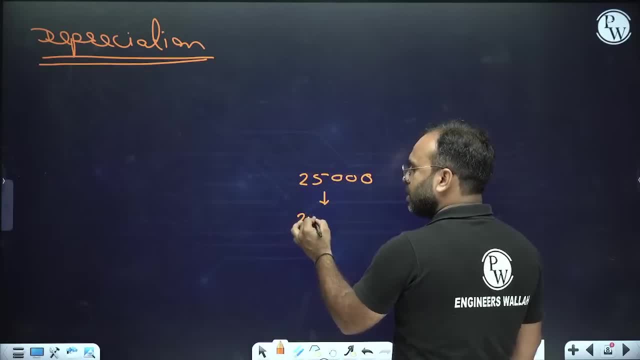 if you buy a phone for 25,000 rupees, then yes, you will get 22,000 rupees or 20,000,, 20,000,, 20,000 or 22,000, you will get it. 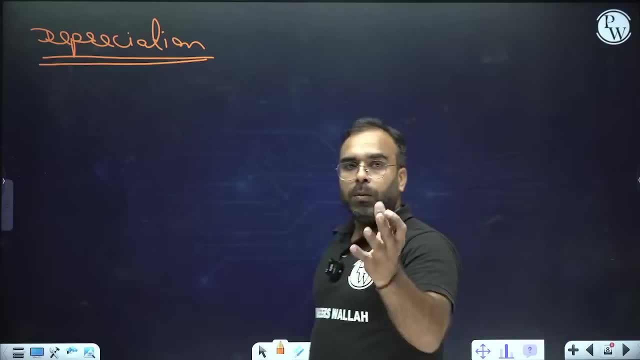 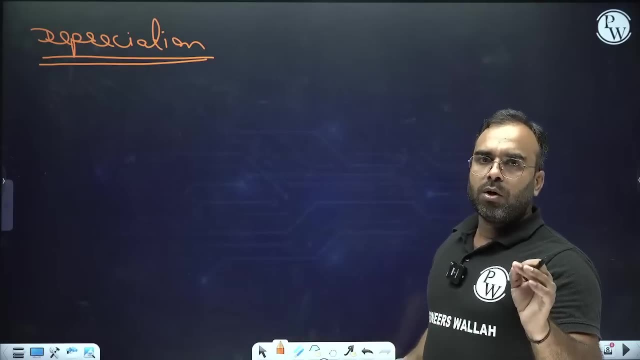 isn't it? So see, understand here what happens here, that when we buy any equipment, then its value gradually decreases. that is what we call depreciation, isn't it? What will be the depreciation? Reduction in cost of equipment or whatever you have. 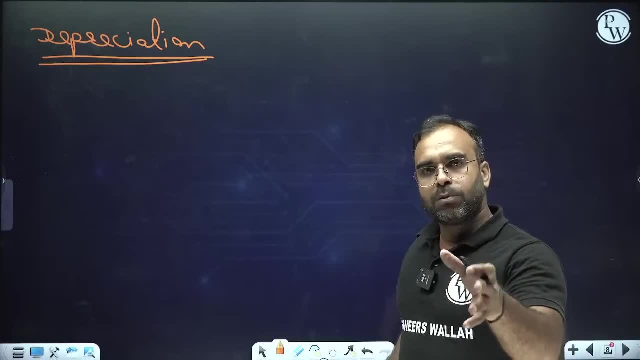 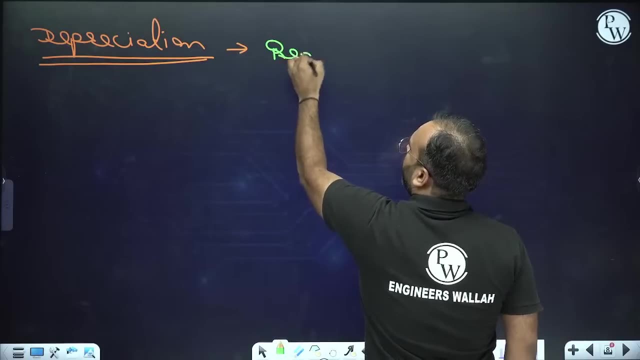 the main cost is: overall, there will be a reduction. so here you write: reduction in cost. what is it called Depreciation? what will be the depreciation? Reduction in cost, so the reduction, what will happen? So what will happen. 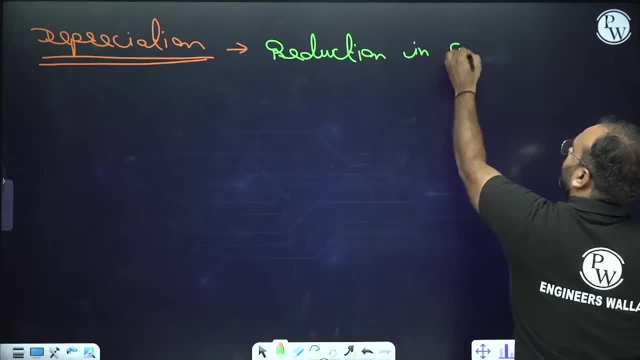 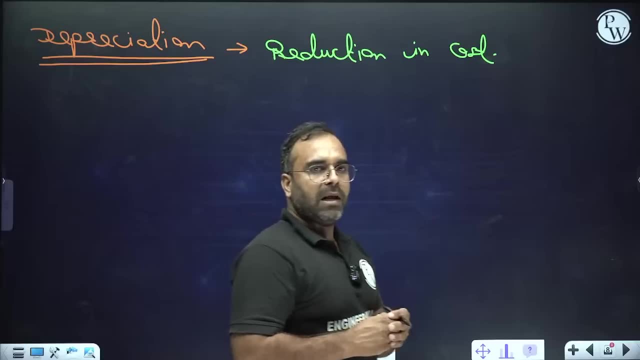 Reduction in cost. what will happen? The reduction in cost of any plant. we will call it depreciation. but the examiner will ask you: yes, we will read the solar power plant separately. son, I will write everything to you. I will make a table ahead. 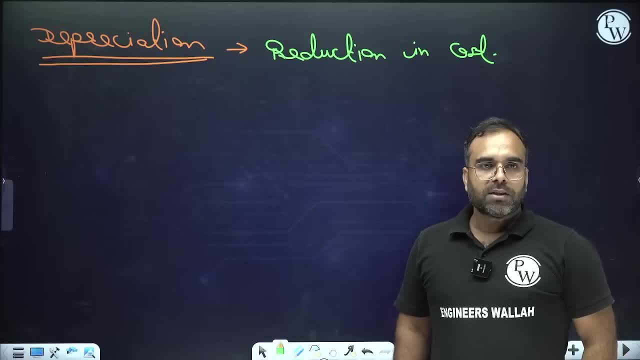 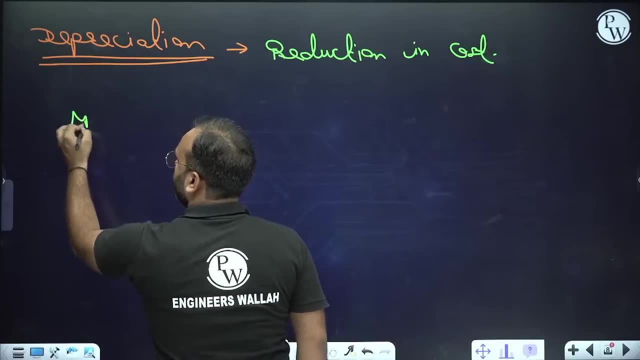 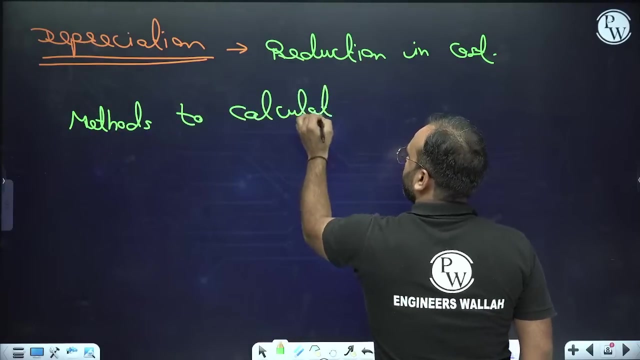 isn't it? Nothing else next understand? yes, next, if we talk about it later, then after depreciation: here he will ask you methods for calculation of depreciation, methods to calculate, methods to calculate, depreciation methods to calculate. 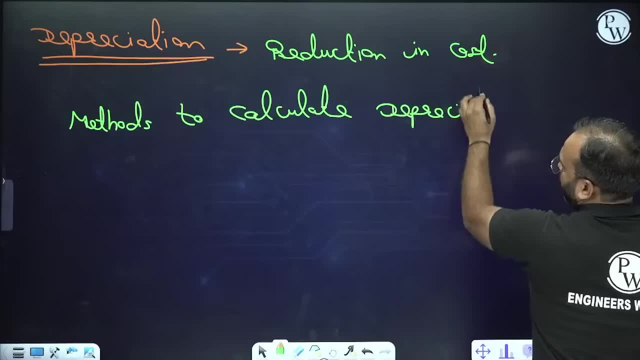 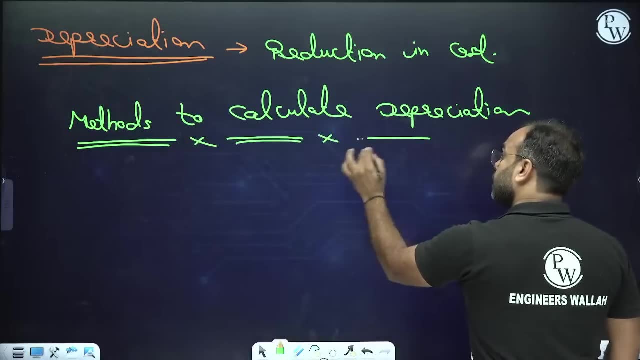 depreciation. tell me quickly what are the methods to calculate depreciation. Once everyone will comment quickly, because this question has been asked many times in the JEE level exams or in the AEE level exams that I have to calculate depreciation. 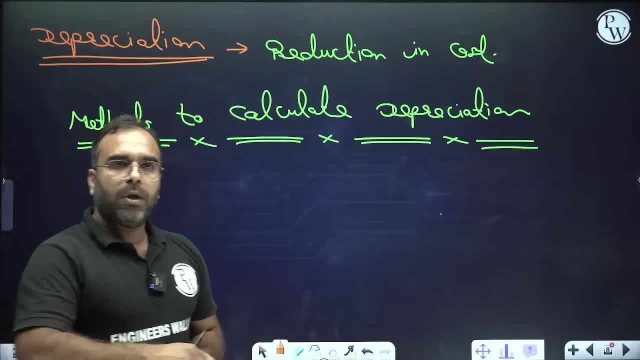 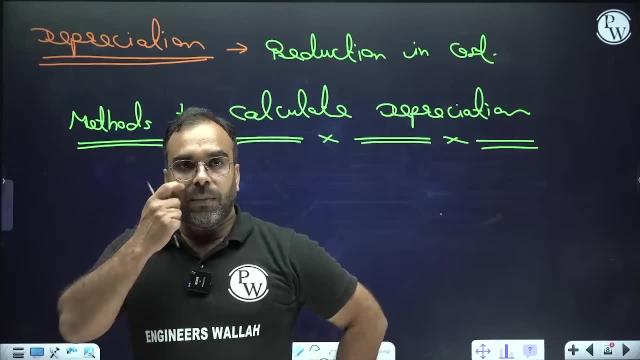 what will be the method to calculate it? Well, Anamaker has given the answer: straight line method, diminishing value method and sinking fund method. correct answer: what will we have here? Yes, Makbul will definitely be the question. 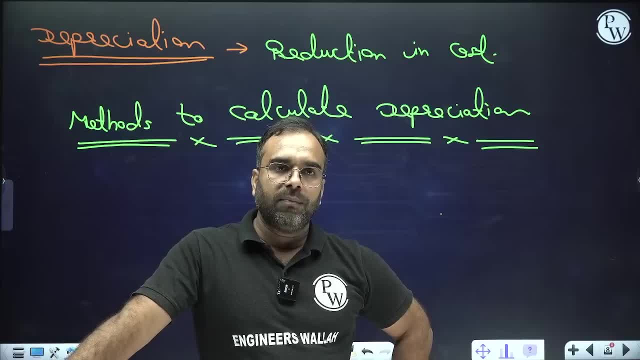 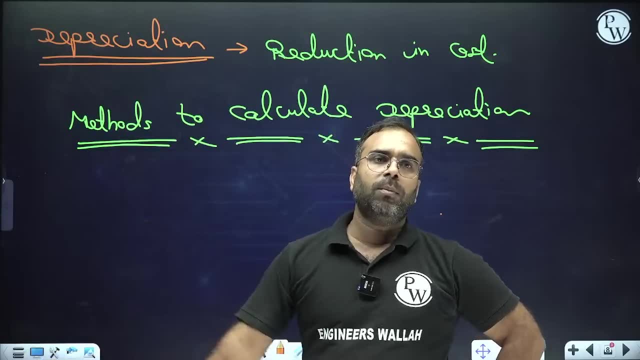 you make it and see, okay, what will happen here, straight line method, diminishing value method and here the sinking fund method, all three methods, which is the correct answer means all of you have done revision very well. daily you have to do revision like this: 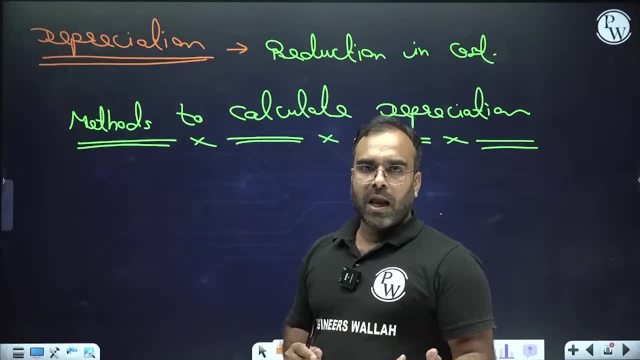 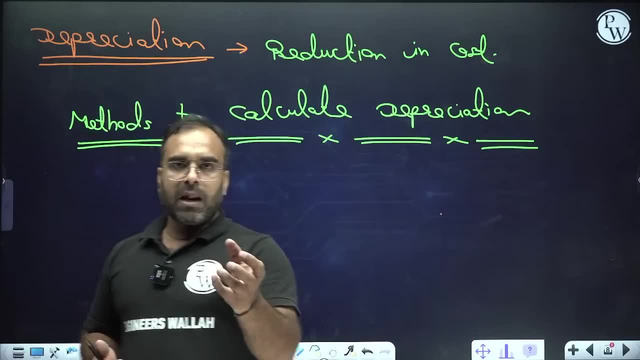 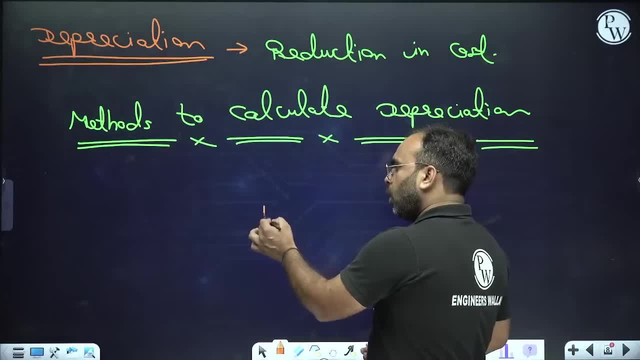 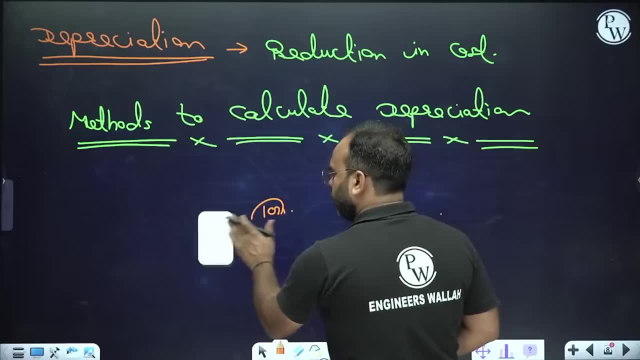 MP, MP, MP, MP. but in the state, let us assume approximately from 100, from the 50 questions only: question of power storm in Maharashtra. also the same, approximately 25 to 30 questions also come. 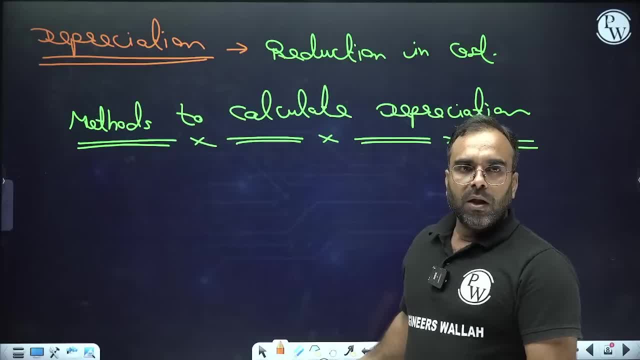 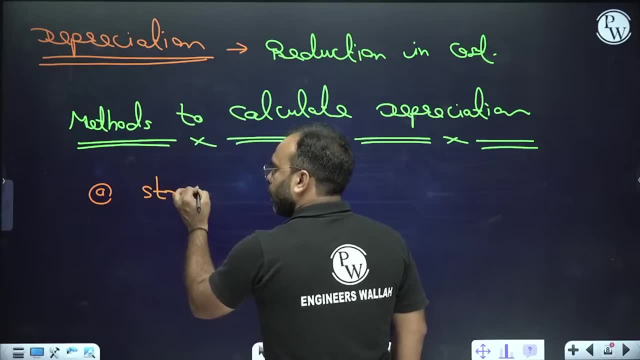 so the weightage remains very large. according to the state, it can be done vary. so what will happen here? we will have three. first of them will be straight line method. first will be straight line method. straight line method. 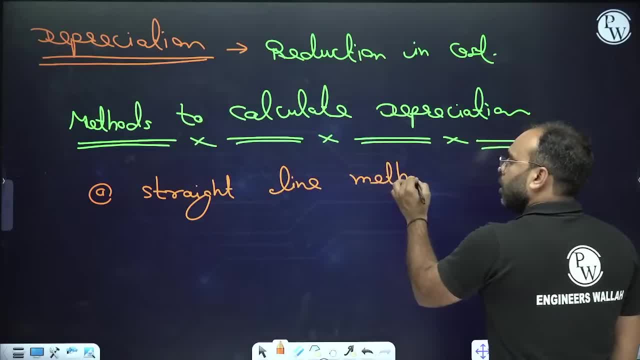 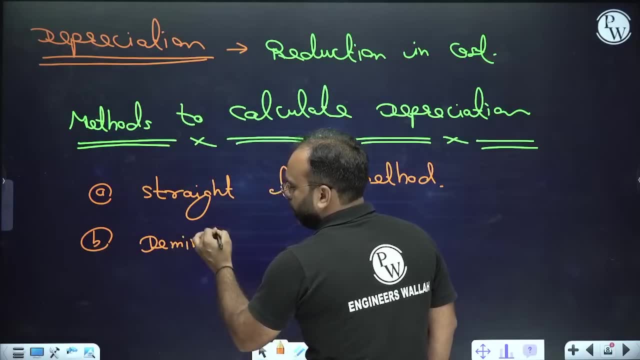 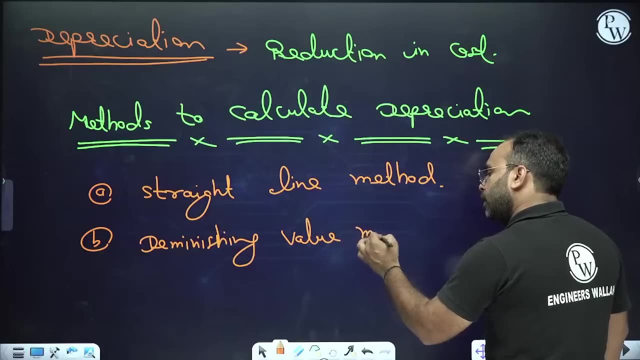 straight line method. that will be first, next second. what will come next? diminished value method. diminishing value method. diminishing value method. it has one more name. someone will comment quickly: there is one more name of diminishing value method. what is that tell? 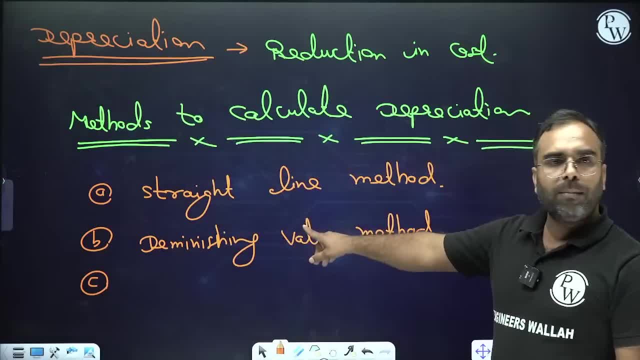 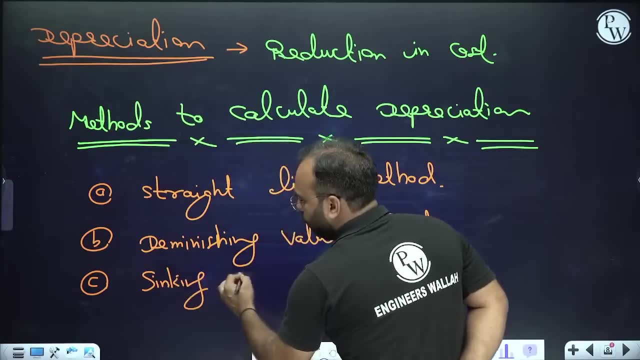 me quickly, because many times the examiner will not ask in the name of diminishing value method. if he does not ask here, then he can ask in a different name. next one is sinking fund method. sinking fund method, which is the sinking fund method. it will be with us. 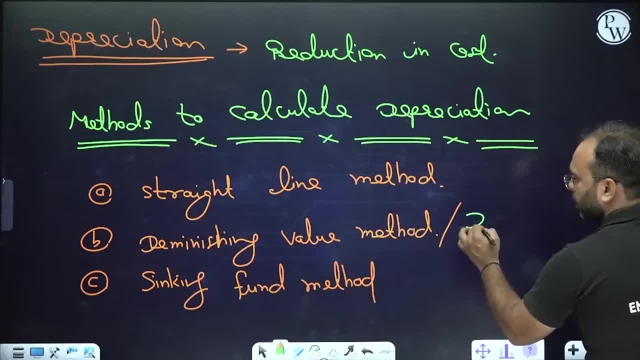 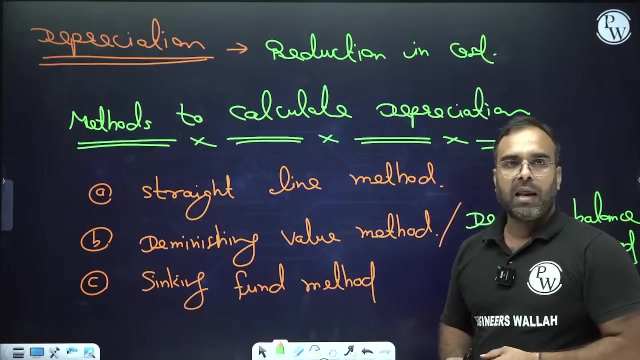 so this is called declining balance method. what is it called? declining balance method? declining balance method, declining balance method. so in the name of it, examiner can ask you know. so remember this name, declining balance method, which is absolutely correct: declining balance method, declining balance method. a lot has given the right answers. 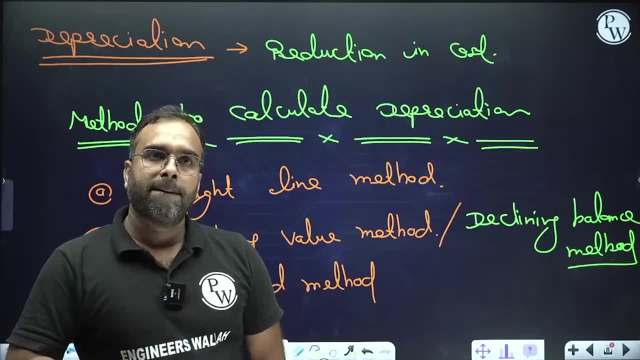 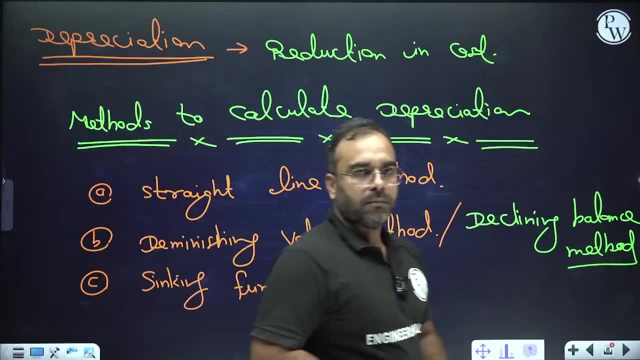 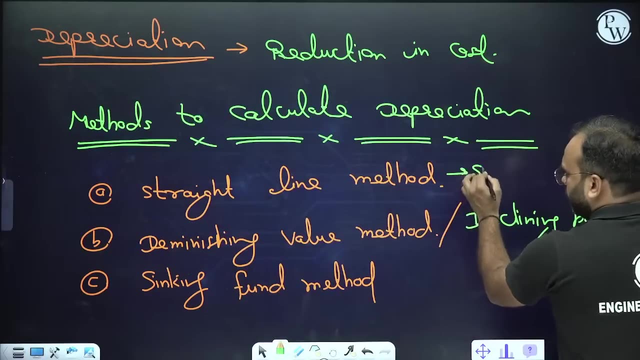 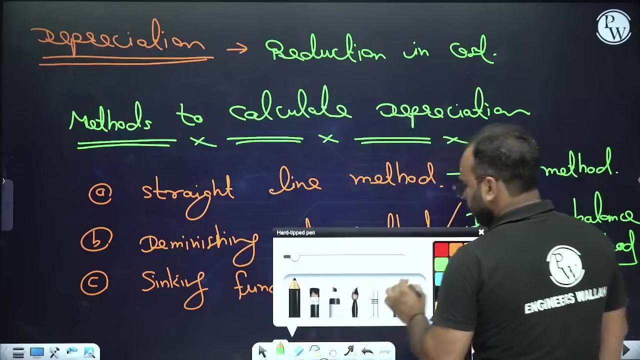 absolutely fine. So these three names you will remember. if I talk to everyone, then which is the simplest method? then this method will be the simplest method. this will be the simplest method. it will be easy to understand and remember one formula here that it should be told to. 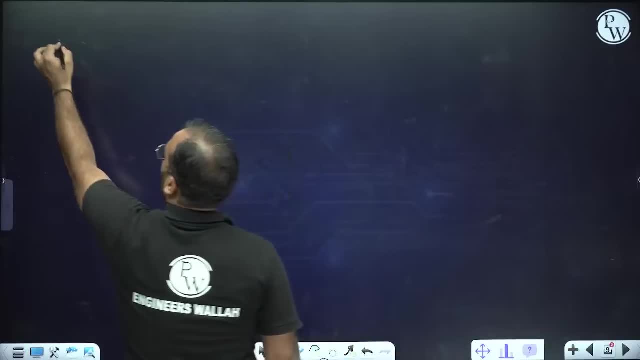 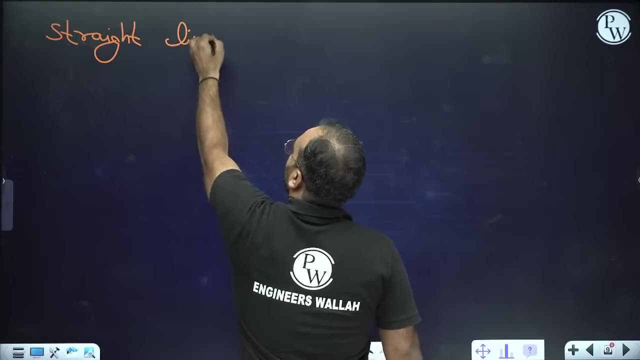 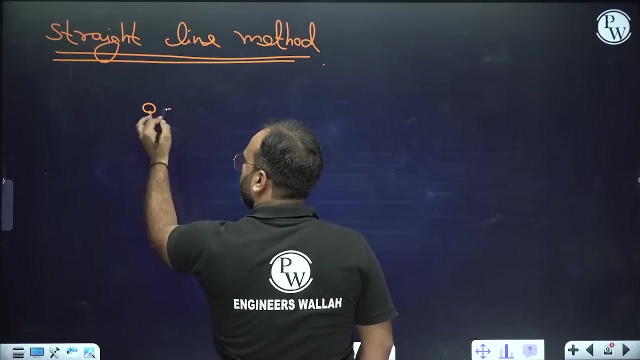 you here. I am telling a formula here from that sometimes numerical is asked to you: straight line method. if I talk to straight line method, straight line method, straight line method. so here, if we talk first of all, I will use a notation, P, that will be: 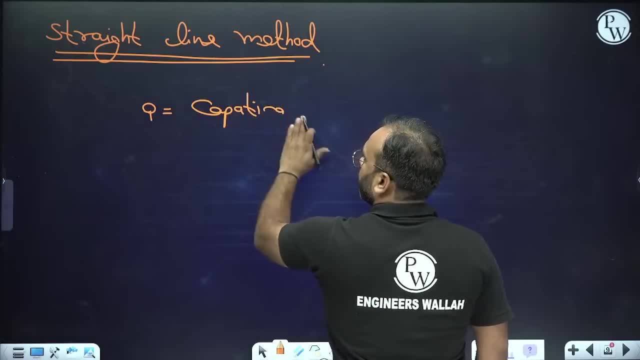 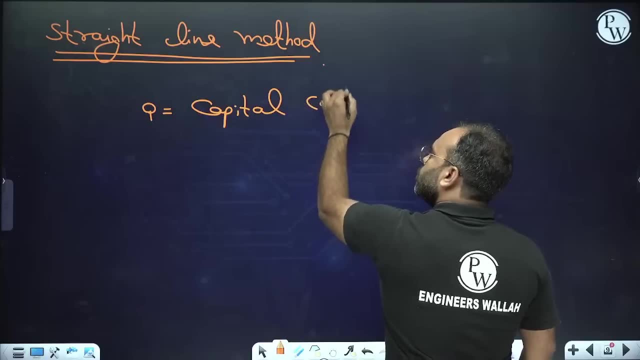 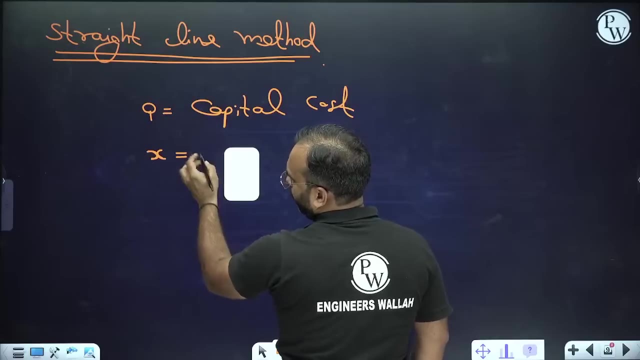 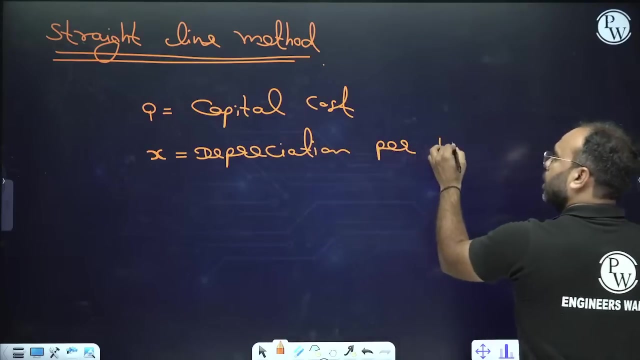 capital cost, capital cost, capital cost. let's tell it quickly: capital cost, and here X will be with us. what will happen? X will be with us. depreciation per year. depreciation per year. depreciation, depreciation per year. per year. I am asking you a numerical. 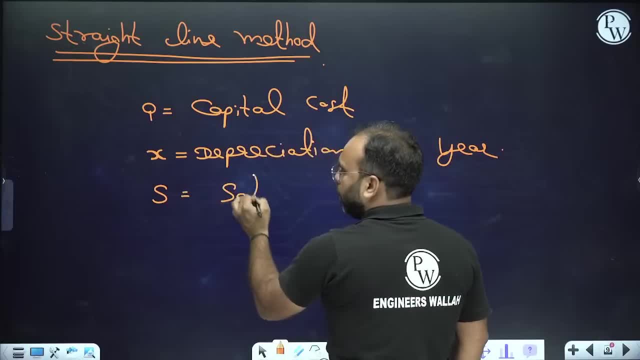 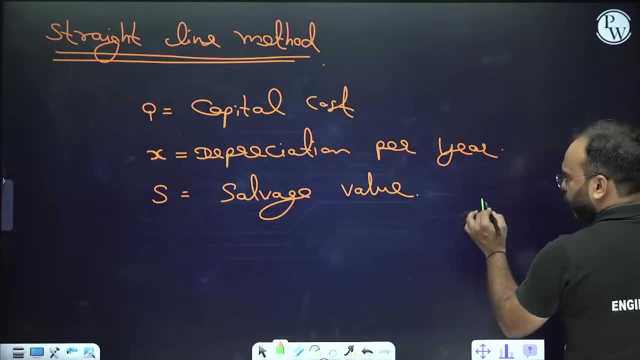 examiner will ask you the same question. what will happen here? salvage value, right, salvage value. many times examiner asks about this. you must have heard the name. if suppose you come with a phone for 25000 rupees, you come with a phone for 25000 rupees and that phone. 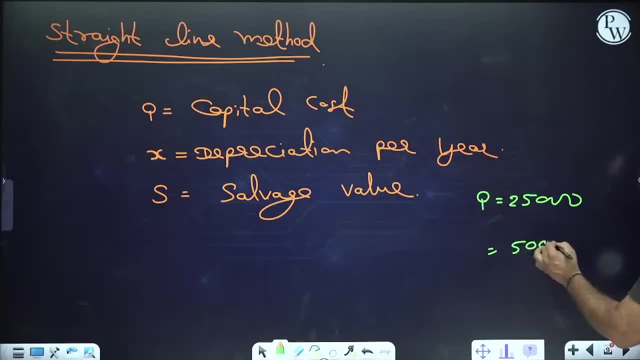 at last, you sell it for 5000 rupees. Yes, So you sell it for this much money and you have used it for 6 years or 10 years, right, you have used it for 10 years. you have bought a phone for 25000 rupees, used it for 10 years. 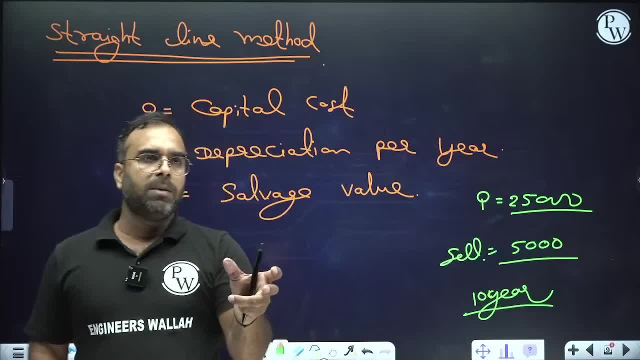 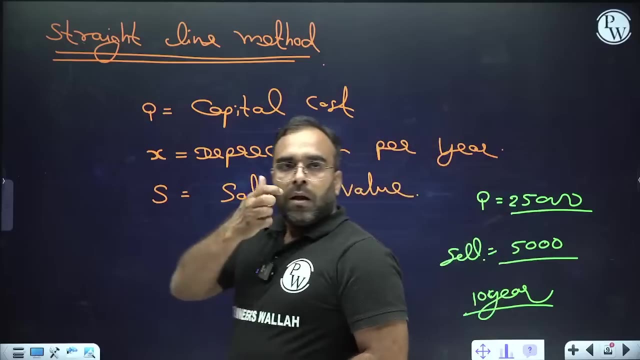 sold it for 5000 rupees. tell me, you will ask: how much will be the depreciation per year. how much will be the depreciation per year? what will be the answer? tell me quickly: how much will be the depreciation per year? yes, good morning, Kittu baby. good morning. 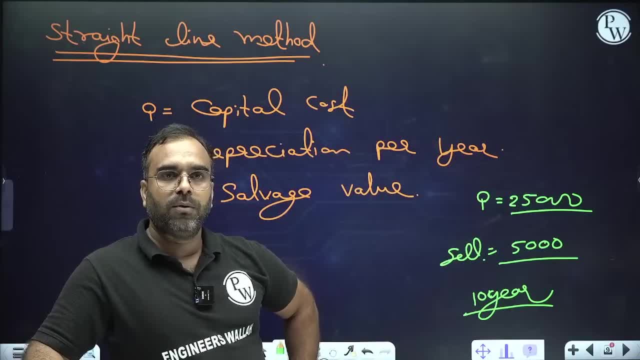 good morning. remember the name properly. remember the name properly. keep the name. you have a good name. it will be a good name. then write the name. come on, tell me quickly what is the answer here: 2000,, 2000,, 2000,. understood completely correctly. see here. 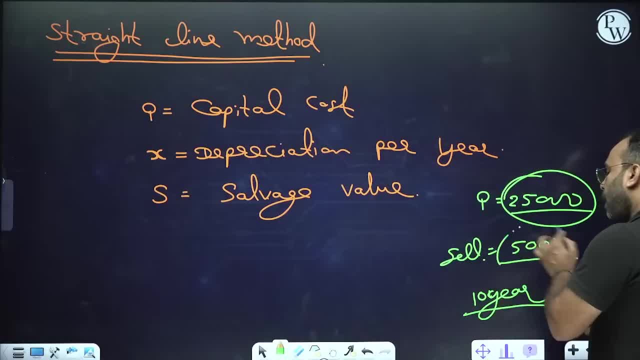 if you have bought a phone for 25000 rupees, you have sold it for 5000 rupees. then tell me how much is its depreciation? how much is the depreciation for the whole 10 years? then how much will be the decrease in its value in 10 years? what does depression mean? 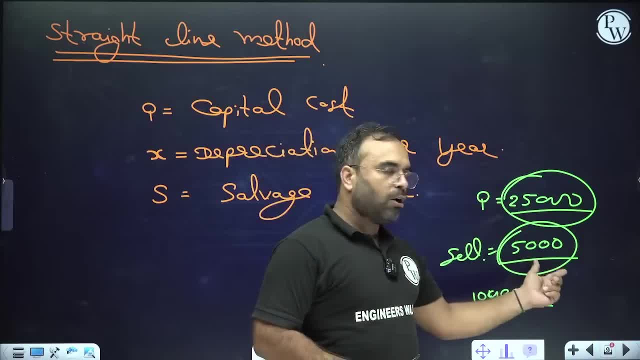 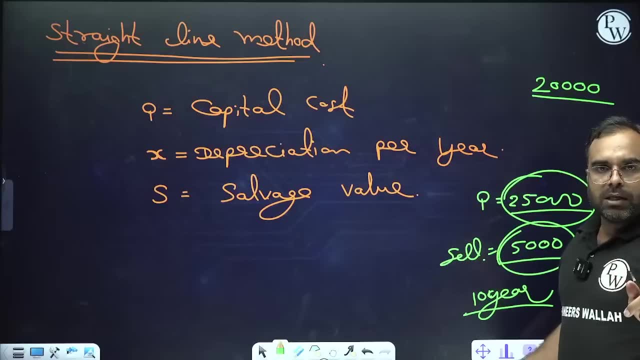 there will be a decrease in its value. so how much will be the decrease? there will be a decrease in the value of Rs 20,000, if Rs 20,000 have been reduced by 20000 and you have used it for 10 years. so if I talk about per year, then divide it by 10 years, then 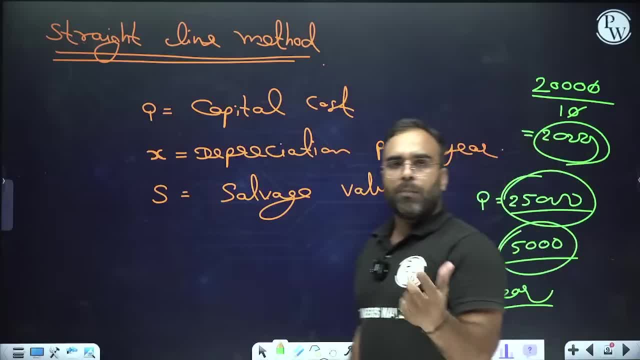 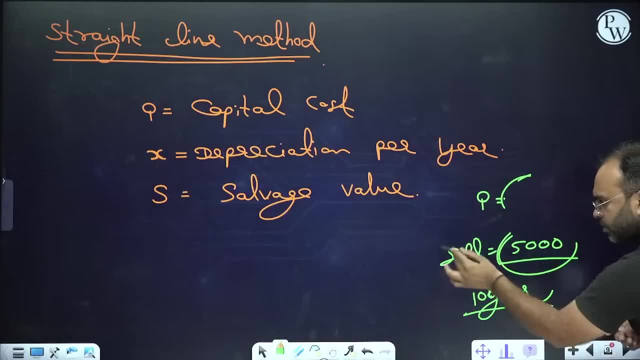 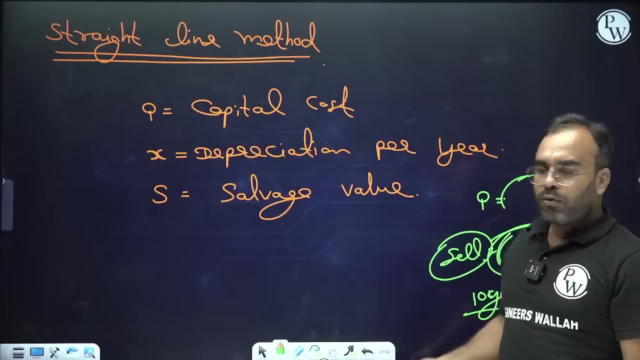 every year the value of your phone is falling from 2000,. it is falling from 2000,. so here, if I ask you here, then the cost at which you have sold. we call it the salvage value. what does salvage value mean? How much value is left with us? we call it this. so 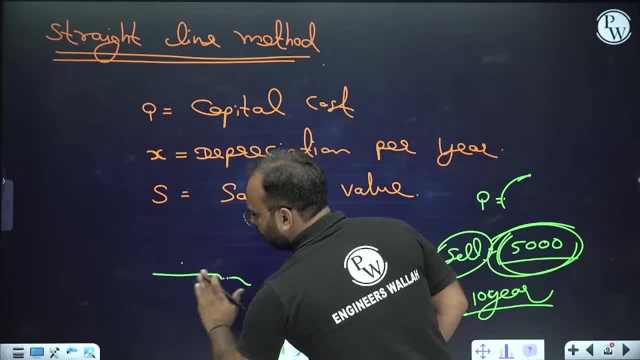 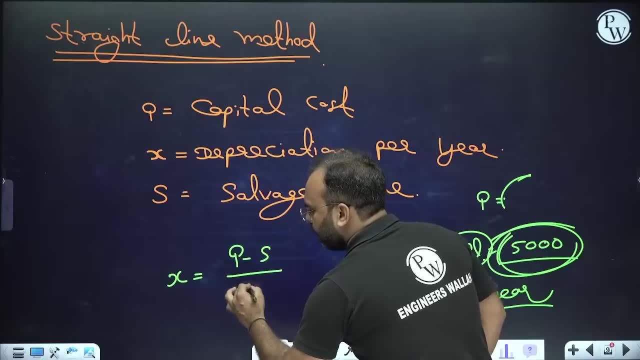 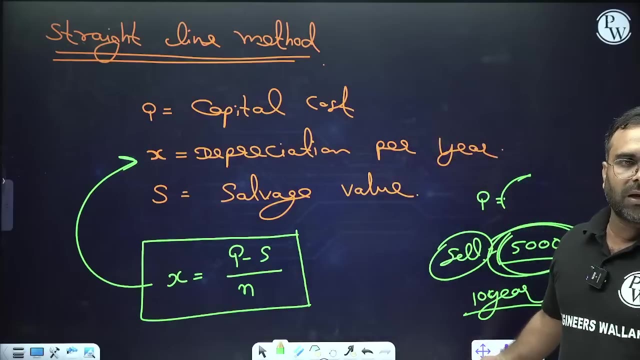 So if you want to find the value of depreciation per year, then you will divide S by N from P. So this will be our formula to find the value of depreciation per year. So remember this formula. Tell me quickly: how did you understand this? 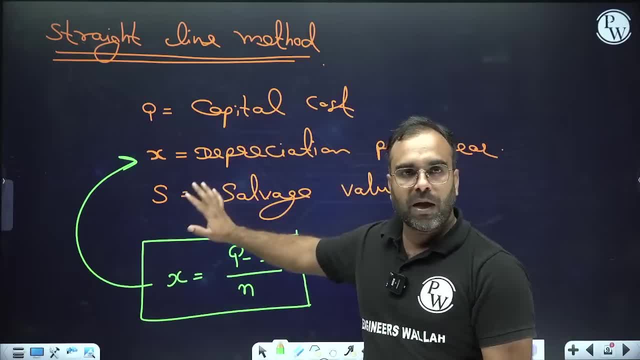 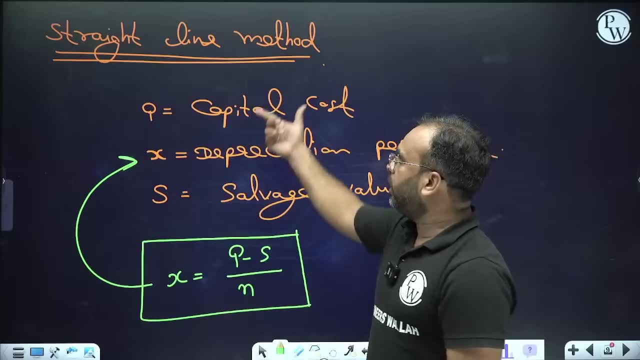 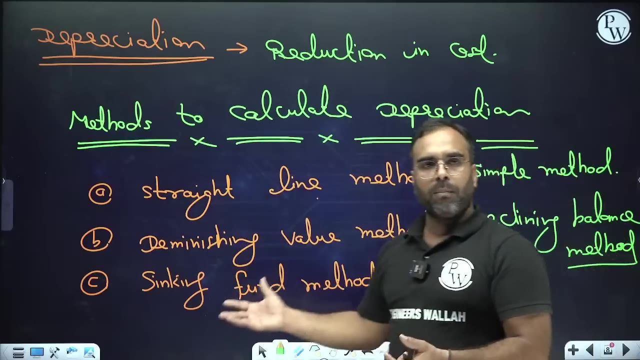 Tell me quickly, how did you understand this formula? Tell me quickly. how did you understand this formula? So remember this formula of straight line method, Rest. if we talk about diminishing value method or sinking fund method, there are also formulas, but they are so big that they will never ask you. 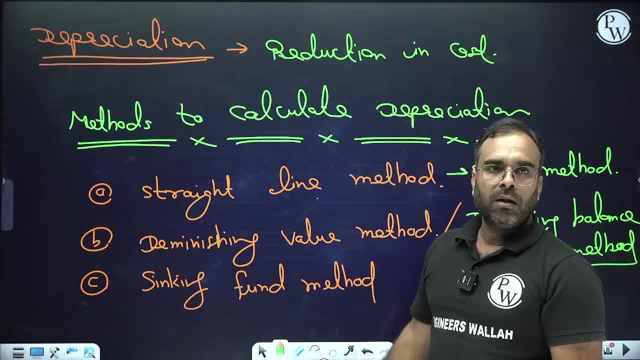 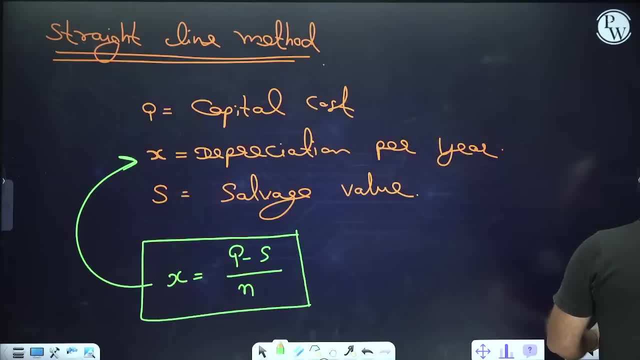 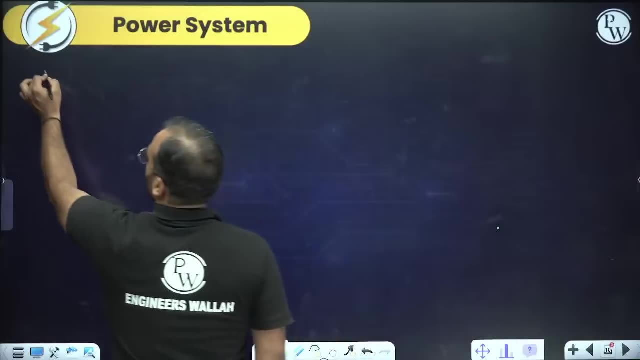 They will never ask you a question. Let's go Clear, clear. clear, So you have understood till here. Next, after this: if we talk about cost and depreciation, we have it Now. let's talk. Next important topic. 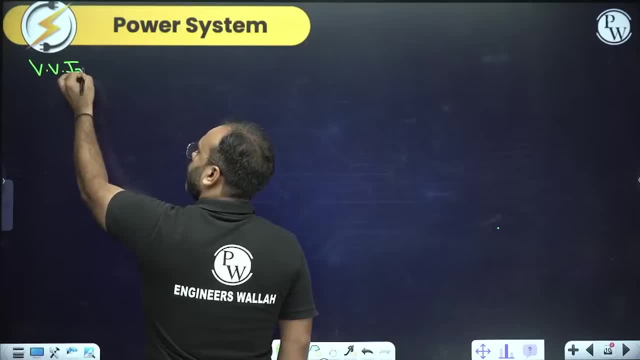 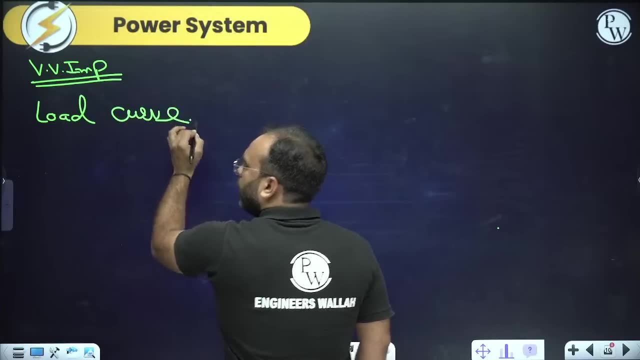 Remember this. This topic is very, very important for you And we have it. Load curve: We have load curve. Now what is the meaning of load curve? You have to understand Here we will talk first. We will make 3-4 curves. 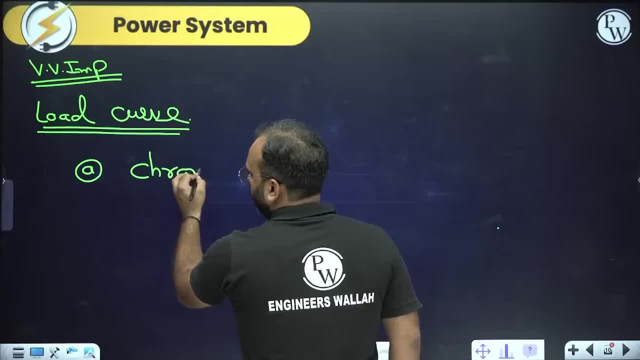 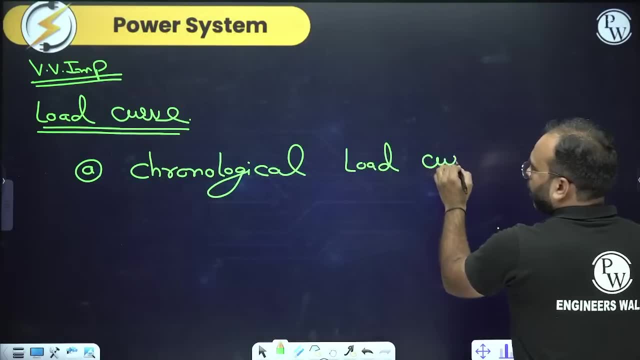 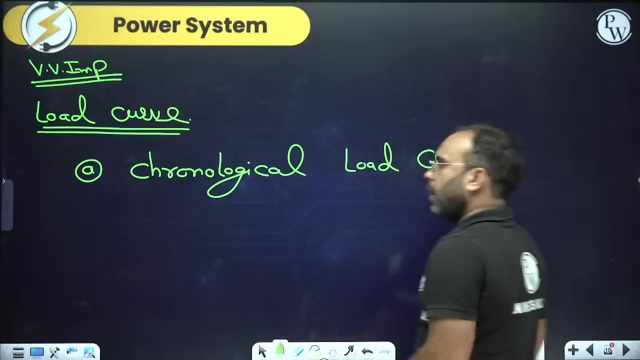 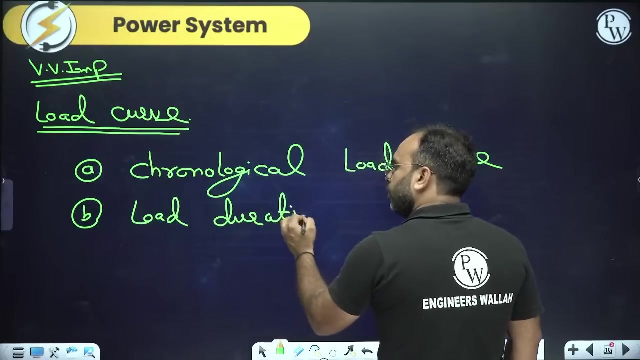 We will make one curve, Chronological load curve. What will we call this? Chronological load curve. Next, what will be Chronological load curve? Second, we will make here Load duration curve. Next, we will make third here. 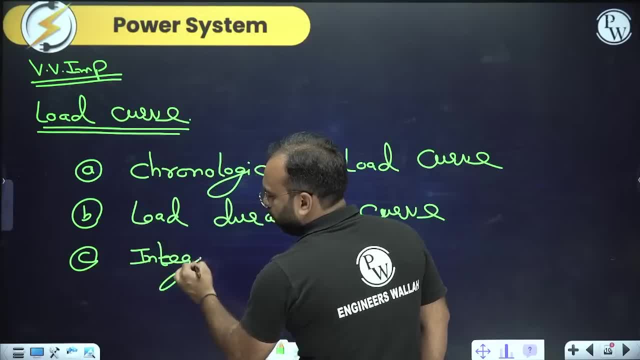 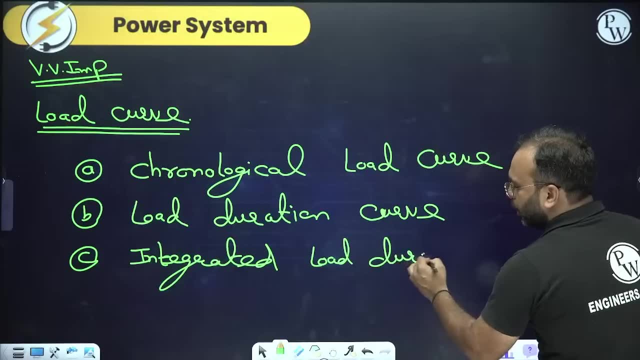 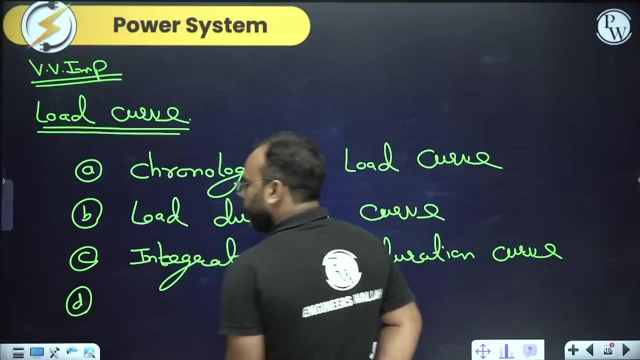 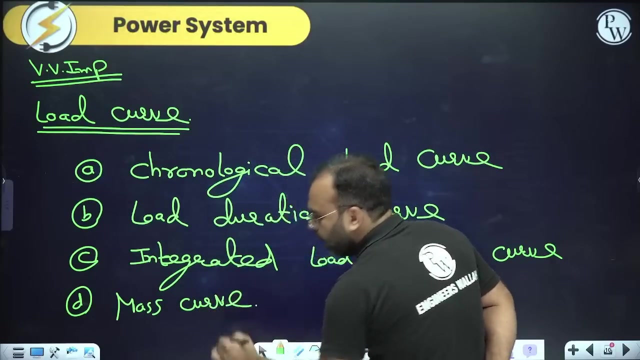 Integrated load duration curve. Load duration curve. Next after this, if we talk So, the next one will be D. The fourth curve will be with us. That will be mass curve. That will be mass curve. So the first question in the exam is that: in which respect is it plotted? 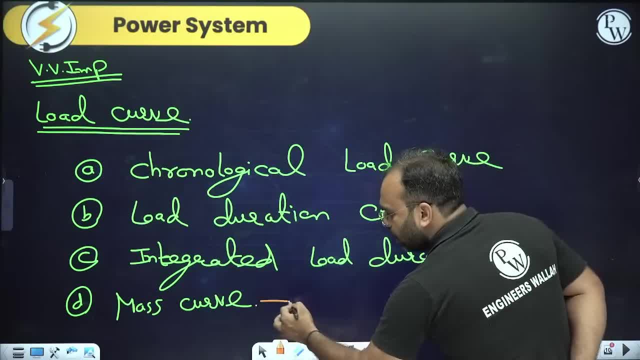 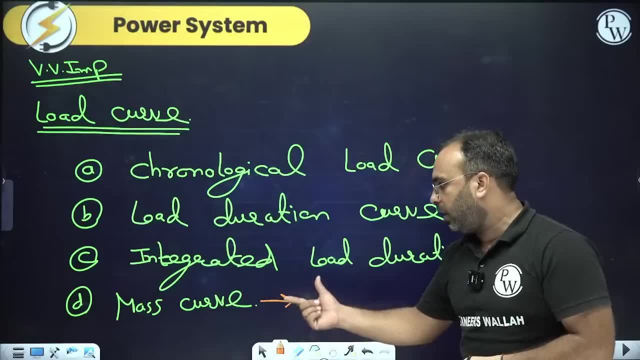 If the examiner asks you that, tell me in which respect is the mass curve plotted? You will also get to see such questions: In which way do we plot the mass curve? We will give the answer quickly: In which way do we plot the mass curve? 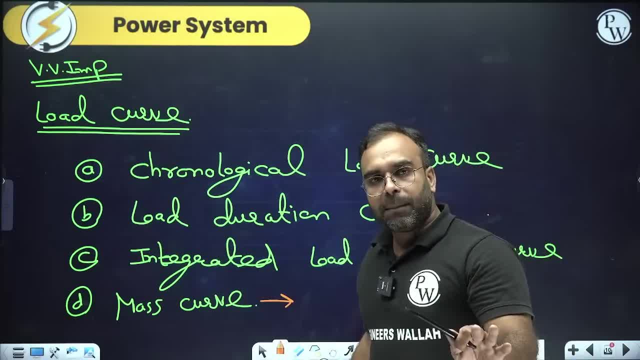 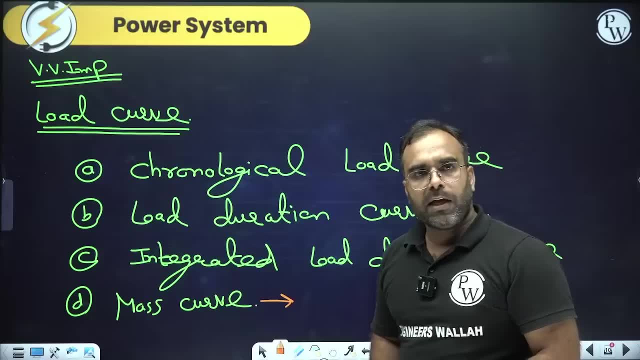 Yes, in which way do we plot the mass curve? See the same question in your JEE exam. What do we write on the y-axis in the mass curve And what do we write on the x-axis? So the mass curve is plotted. 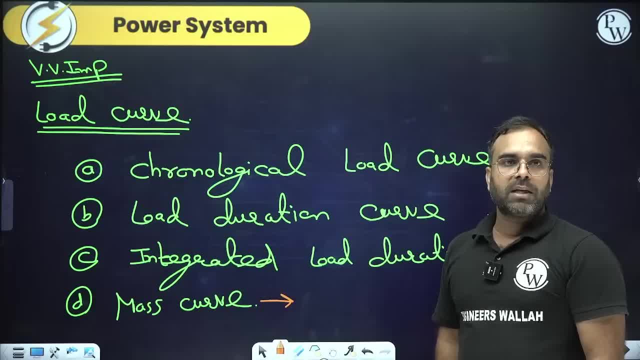 Energy versus time. Energy versus time. Yes, the answer is absolutely correct. Yes, Makbul, everything will be done. First, focus on studying. Focus on studying. Leave the other things. Focus on studying. Ok, there are many students among you. 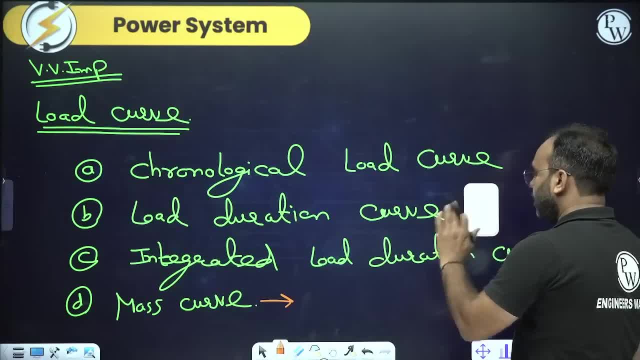 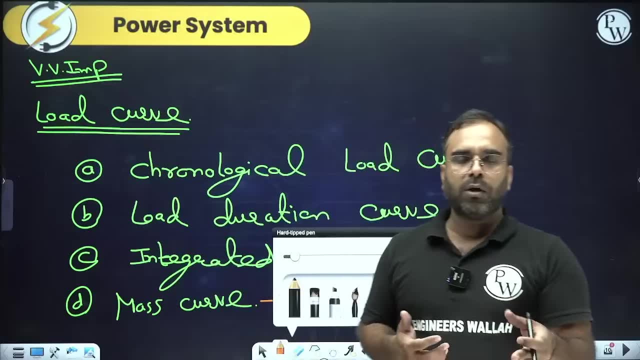 I must have told something to many students. I will tell you again. If you are preparing now, So if you guide many people or tell someone to study, So do you know what he will say? He will say: what do you have to do after studying? 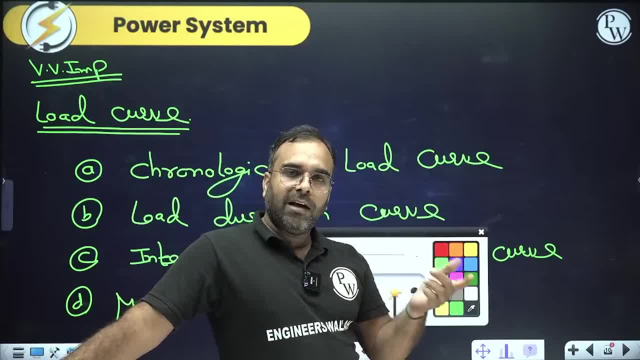 What do you have to do after studying? So their dialogue is fixed. What did you bring And what will you take? So what do you have to do after studying? After studying, You will get a lot of such dialogues. 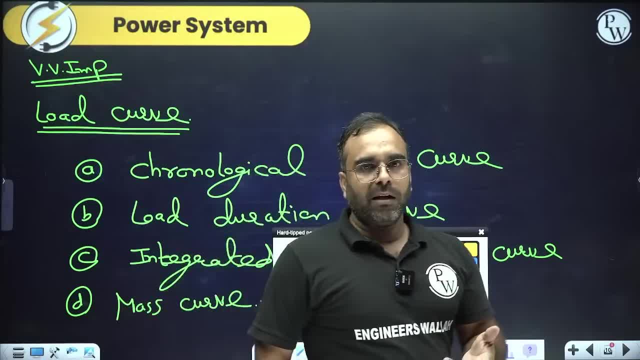 You will get a lot of such dialogues. Those who talk to you will meet The new boys who speak to read. they have this fixed dialogue That. what do you have to do after studying? There is no going to get anything later. 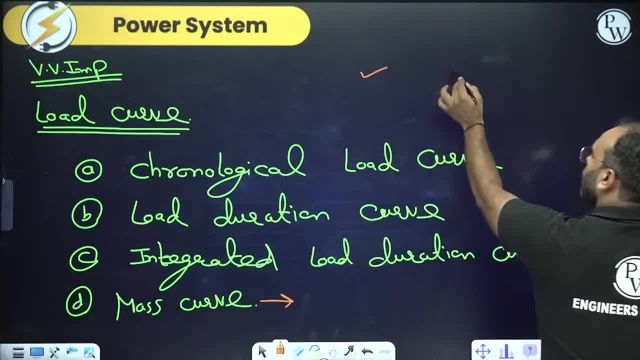 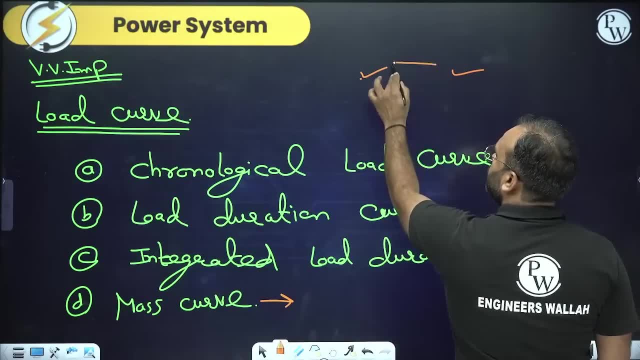 So here, this is fine, I agree with you. What did you bring And what will you take? I completely agree with that. But, man, the thing you brought and what will you take in between, This is a 50-60 years of life. 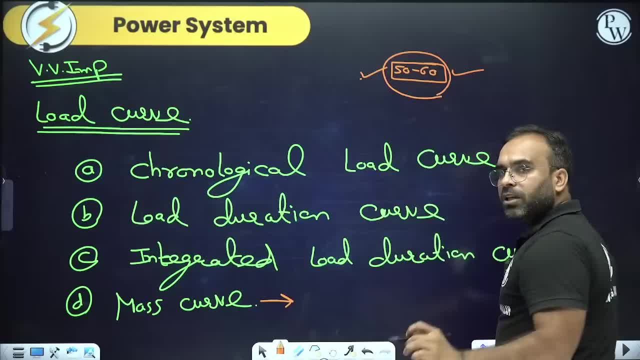 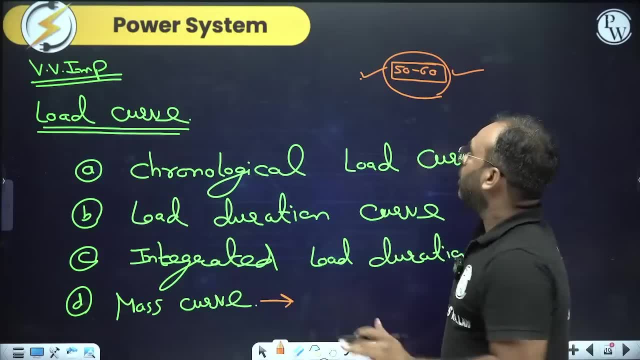 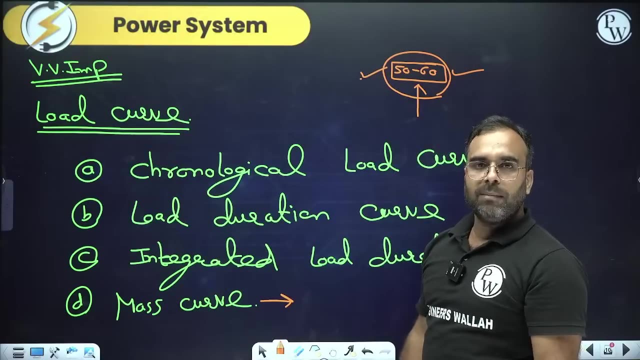 We have to find that out too Now. if you want to live a life of 50-60 years, If you want to live a better life, then you will have to do a job for the money you need. So here you will not get anything, but if you want to live a better life, then you will have to do a job. 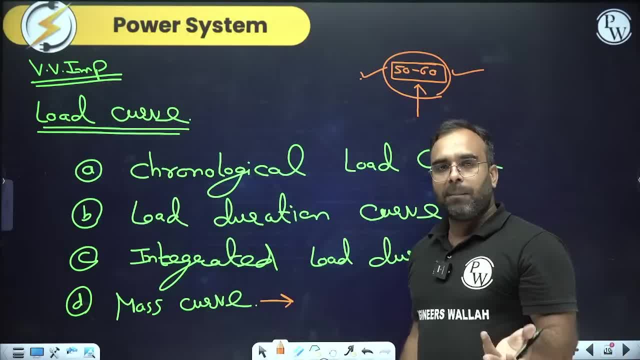 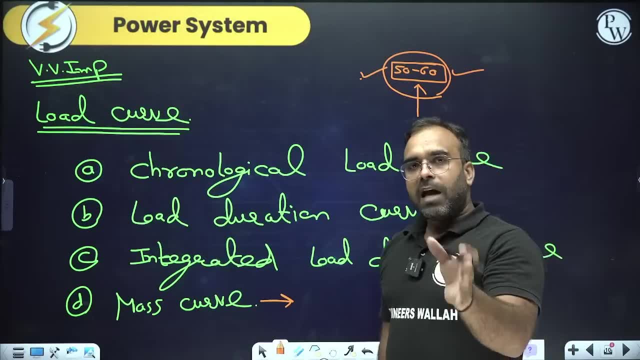 Now many of you will say that why am I doing a job then? what to do with the money that is? all this money cannot be bought. Like there are many dialogues, you will find many people saying that all this money cannot be bought. 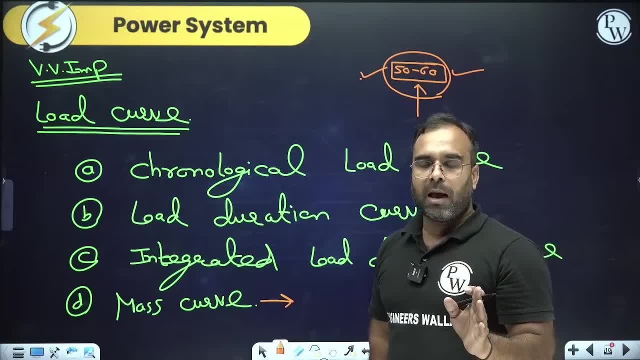 Okay, I agree that all this money cannot be bought, but you all know that the things that make us happy, we need money to buy it. So, finally, if we consider all things, every happiness that we cannot buy with money- but nowadays we get happiness by buying a mobile phone- 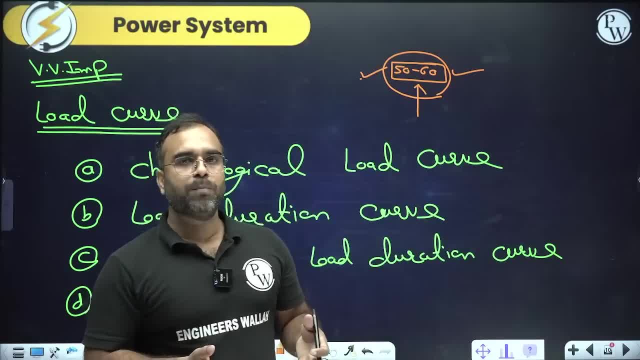 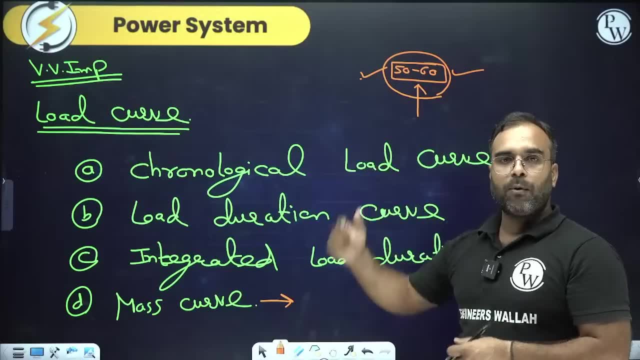 Or hand in hand. We have to wear watches, wear good clothes, wear shoes. we get happiness from them. Okay, roaming around. then you also need money for that right. So for that you will have to do a job, for that you will have to study right. 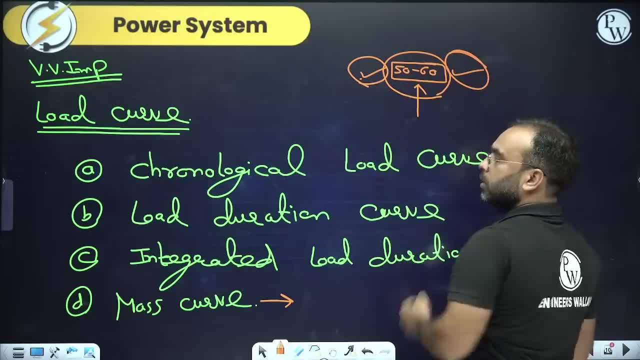 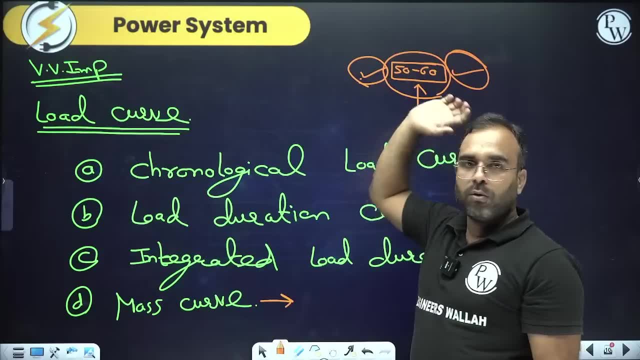 So you don't have to listen to those people who tell you that what you brought, what you will take, you don't have to believe them. Tell them. if someone says like this, what you brought, what you will take, tell them that you have to live a life of 50-60 years in between. 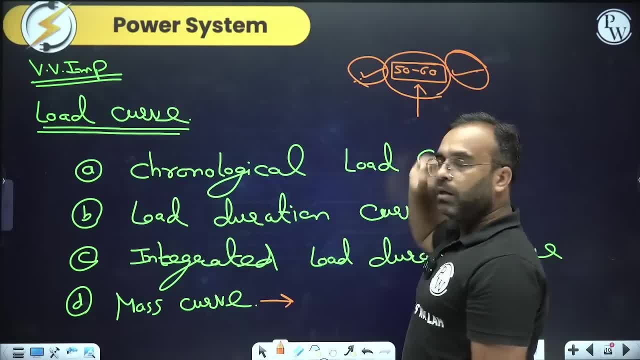 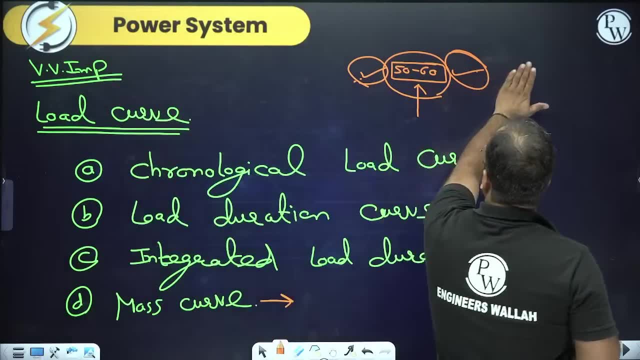 Brother, why are you forgetting that? You are just talking about being born and dying one day. Think about the middle thing. So definitely you have to live a life of 50-60 years. You will also feel like studying, right, So you have to take care of this thing, right? 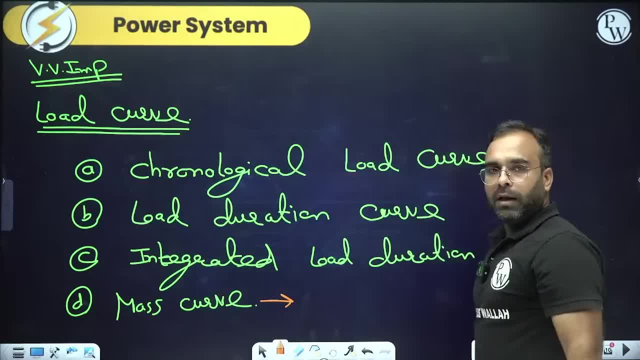 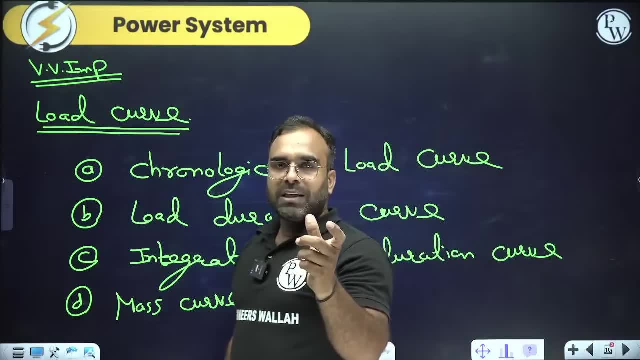 You don't have to listen to other people. You don't have to listen to other people. Okay, And there is one more thing, right? I will tell you one more doubt. There are a lot of students, right. They say, sir, in the first attempt, SSC JEE or UPSC JEE, or I am talking about my state JEE. 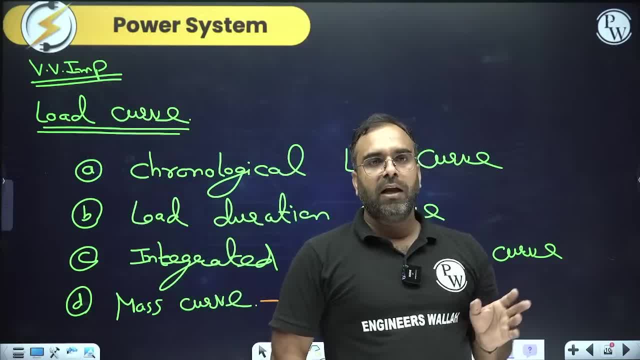 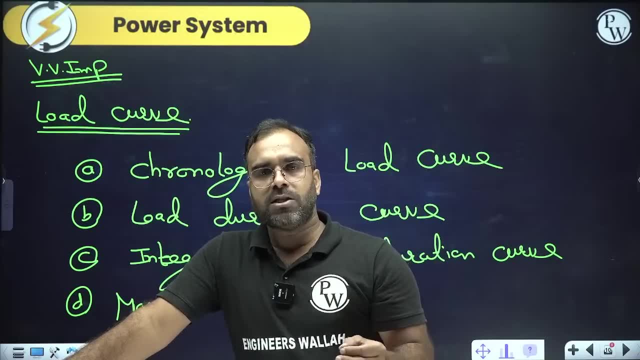 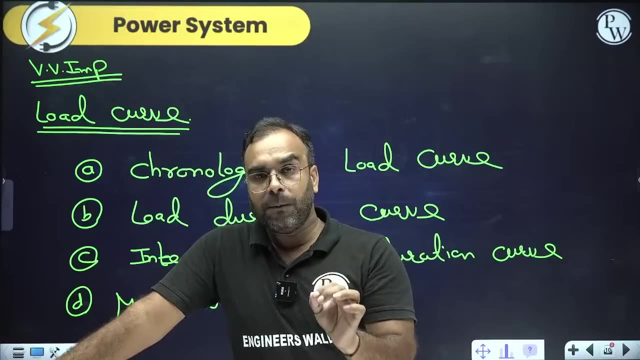 Can the exam be cleared in the first attempt. So I say definitely right, Definitely. whatever exam- it is UPSC exam, Whether it is SSJEE or any other exam- You can clear it in the first attempt. But the condition is that have you given your 100% to clear that exam? 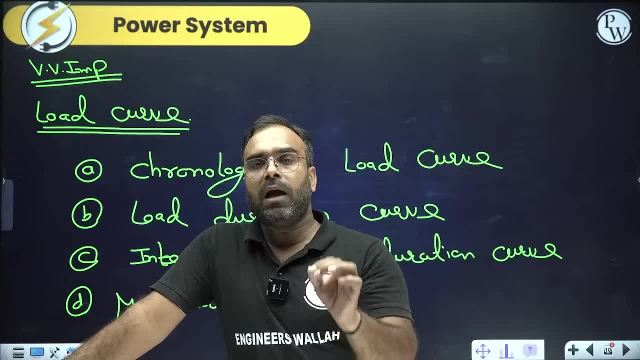 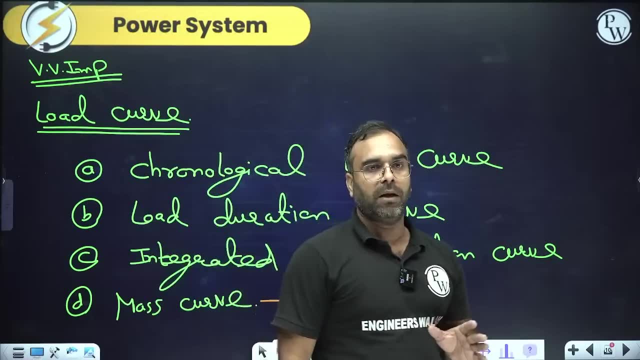 If you are giving your 100%, then I am saying that your exam is 101%. it will be cleared. But for that you will have to work hard, day and night, Understood. So it will not happen that you will work hard for 2-3 months. 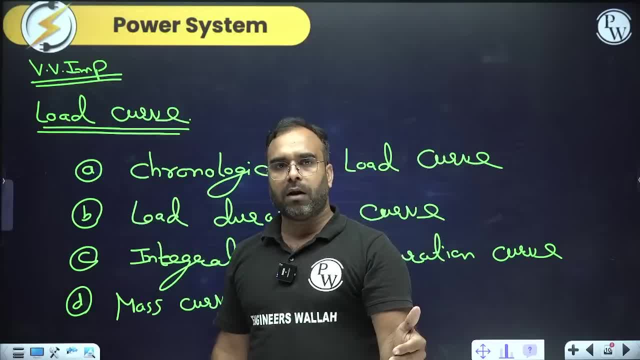 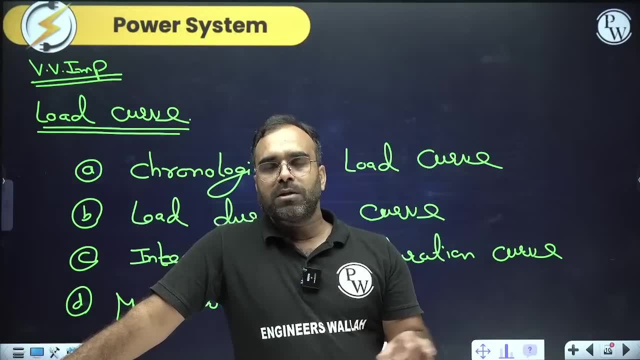 No, Those who have been trying for 6 months to a year. from the beginning. they will definitely clear it easily, But for that you will have to put in continuous effort. Now many of you must also be thinking that my friend has got an exam. 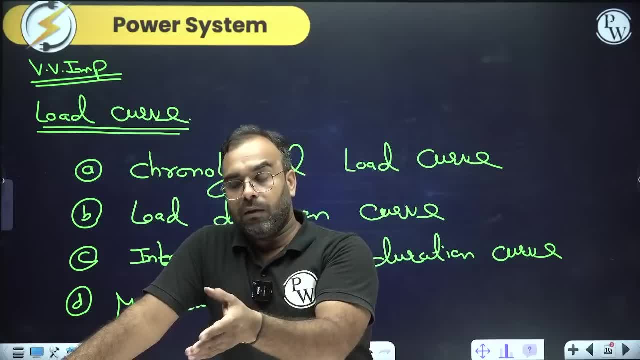 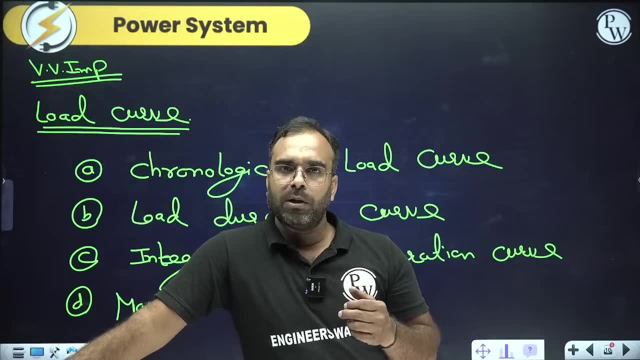 But now many will also comment that what is the exam that has come out? He has taken an attempt in the second attempt when his exam came out, But he has taken it in two attempts. Why should I tell? Because he knows that he did not work hard in the first attempt. 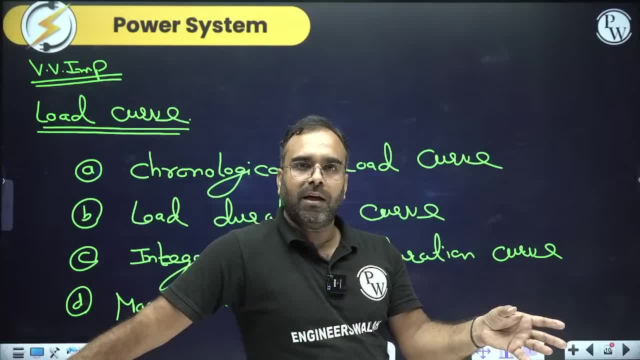 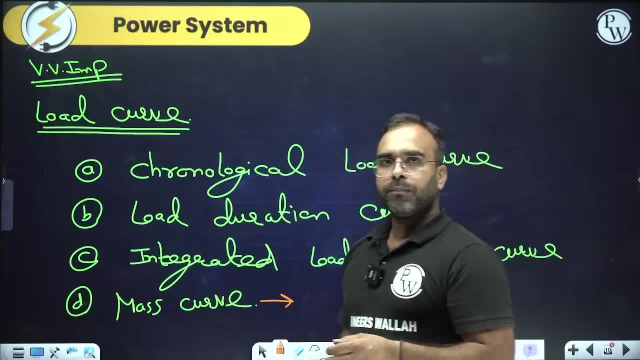 If a person takes the second attempt only when he does not work hard in the first attempt, then he did not work hard in the first attempt. that is why he took another year. You should work hard in the first attempt itself, so that you do not need to take another year. 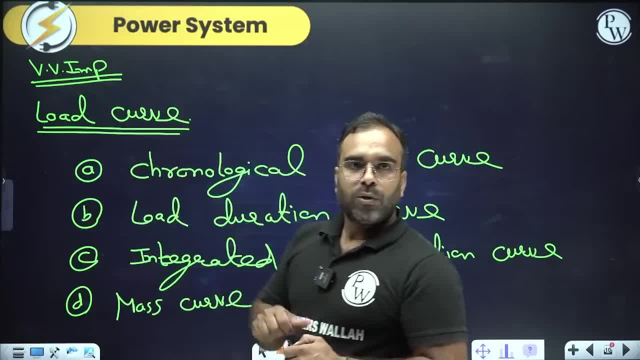 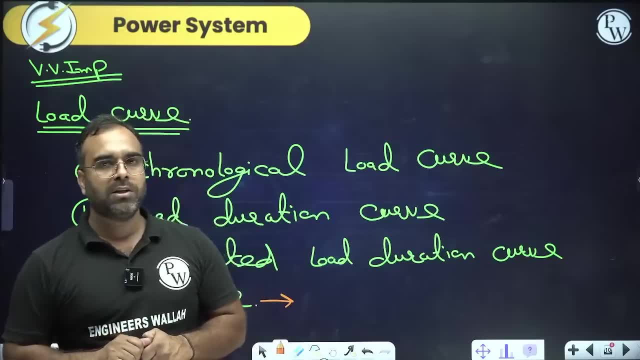 Understood. So here you will have to work hard. You will have to work hard in the second attempt. That is why I am telling you to focus on your studies and not on other things, And you do not have to talk about those things. 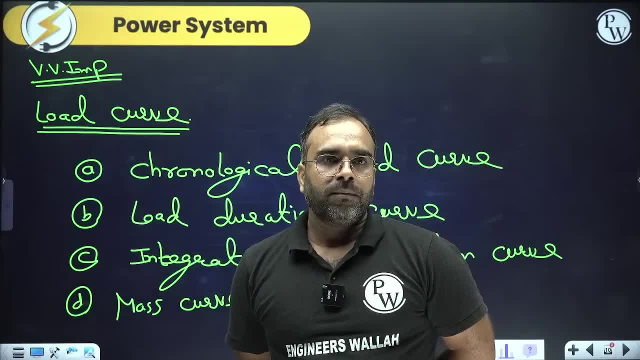 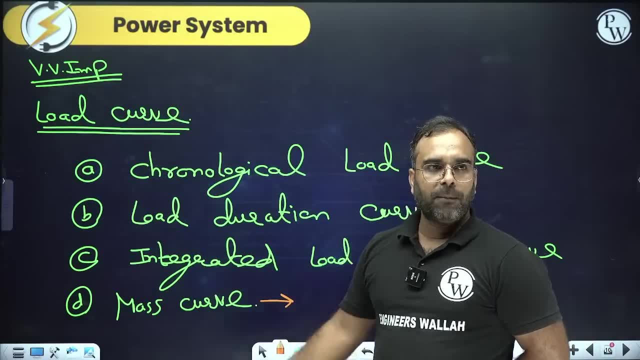 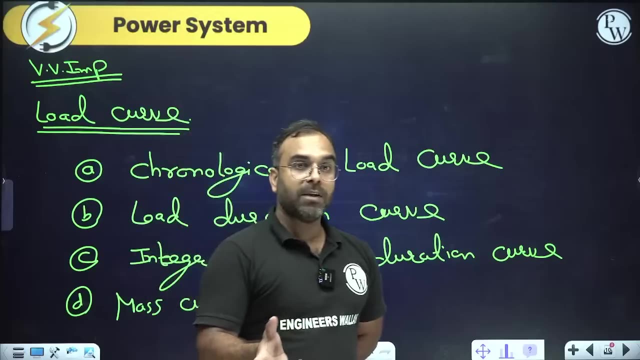 What did Jehak Khan say? Yes, definitely. Thank you so much. So here you have to focus on your studies and not on other things, Because I was seeing that many people were changing their names and laughing in the chat. They were not studying that much. 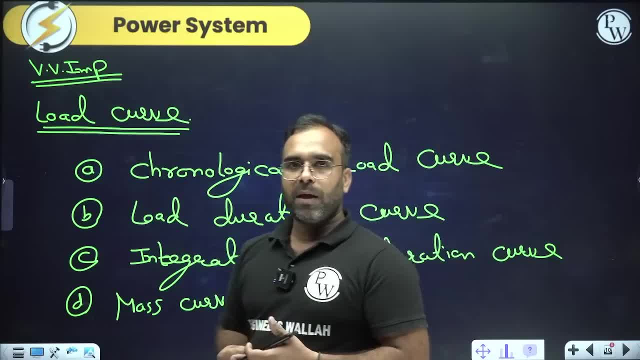 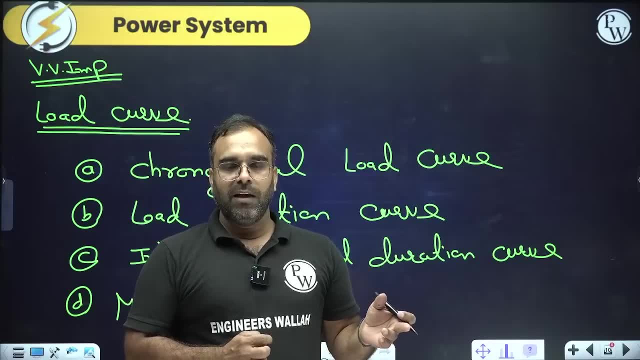 Because I know that studying is our secondary work. What is our first work? First of all, we come here to enjoy Sir Suresh. sir will dance and show you, He will laugh and joke with you, So you do not have to do that work. 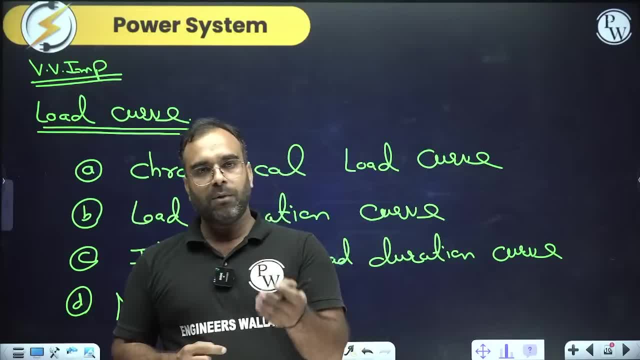 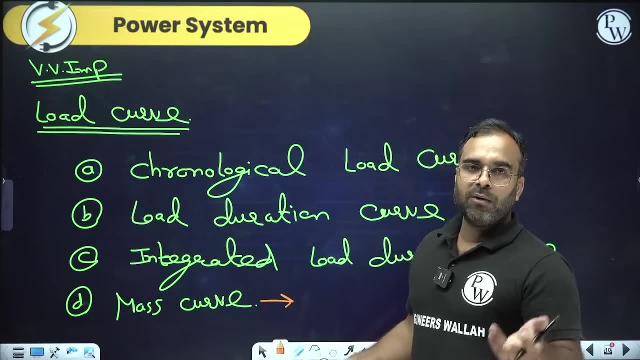 Keep the name that you have kept. Keep that name So that everyone else is not disturbed. So that everyone else is not disturbed. They also study. Otherwise, many people run away in that They do not know what they are thinking while changing their name. 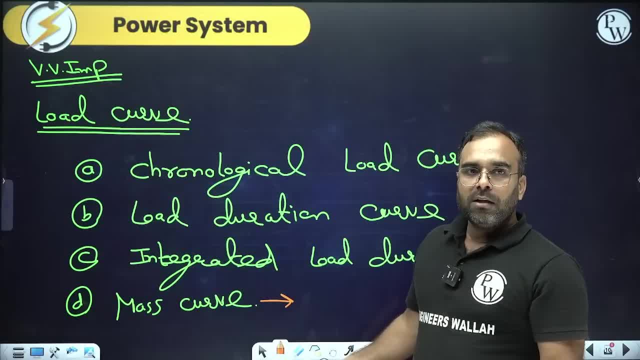 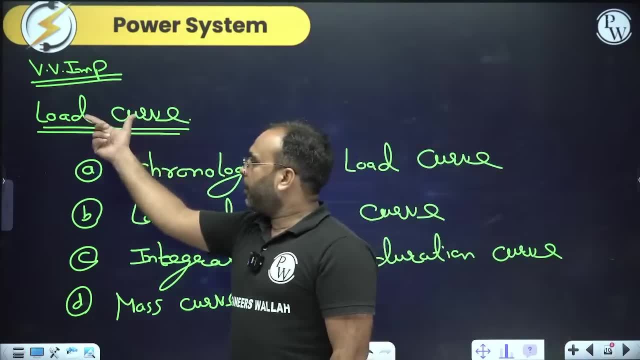 They do not pay much attention to their studies and focus on their comments. Okay, So focus on your studies here. Focus on your studies, Leave everything else, So come here again. So see, here we are talking about the load curve. We will make four curves in total. 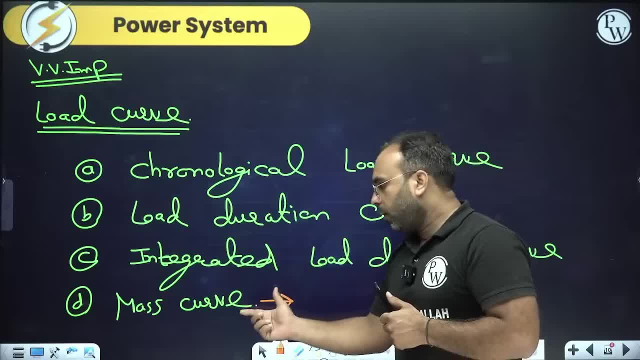 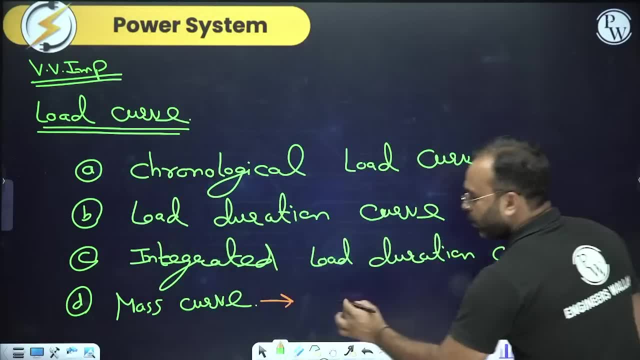 Chronological load curve, Load duration curve, Integrated load curve And mass curve. So the answer to the mass curve is definitely- You all have given the correct answer, Sir- the mass curve that we plot, That energy versus Energy versus. 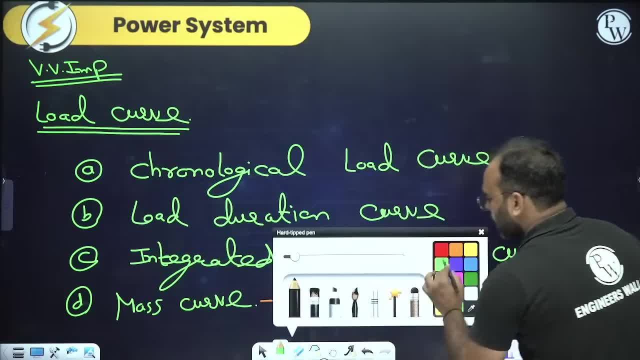 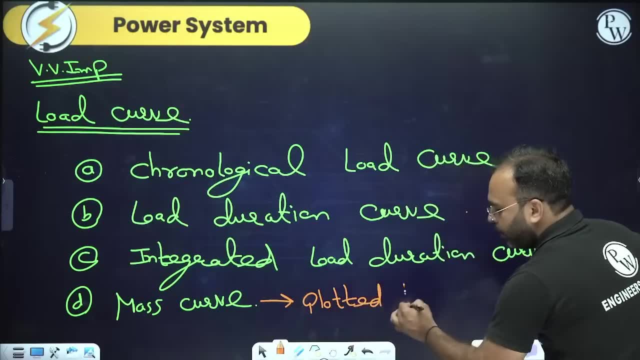 Keep in mind We plot in between time. So write here The mass curve Plotted between. Write the point here: Plotted between. Plotted between: What will we have Energy? Plotted between Energy versus time. Correct answer. 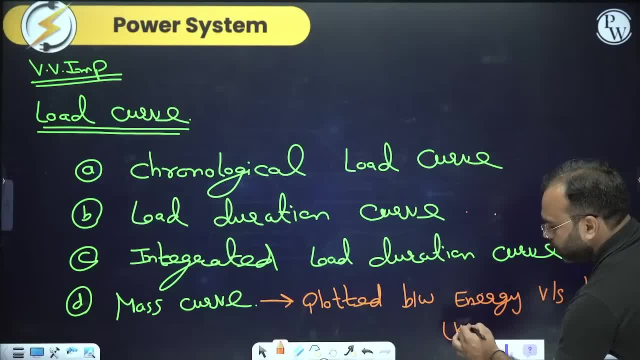 Keep in mind the energy, This kilowatt hour. Where will it be written? Y axis, We will write on the Y axis. We will write on the Y axis. And where will we write the time? The time will be written on the X axis. 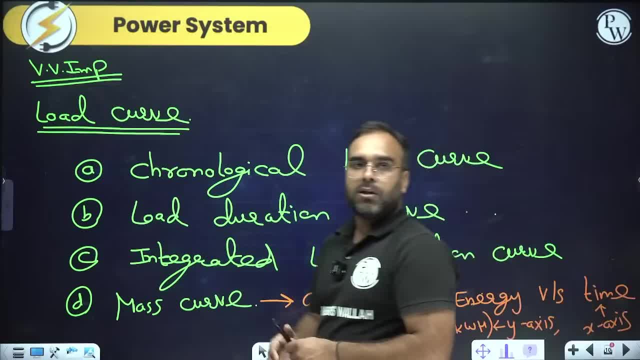 If the examiner asks you, Then you can also tell this. Next, Tell me quickly Integrated load duration curve: In which are we plotting? Integrated load duration curve: In which are we plotting? Tell me all the answers quickly. In which are we plotting? 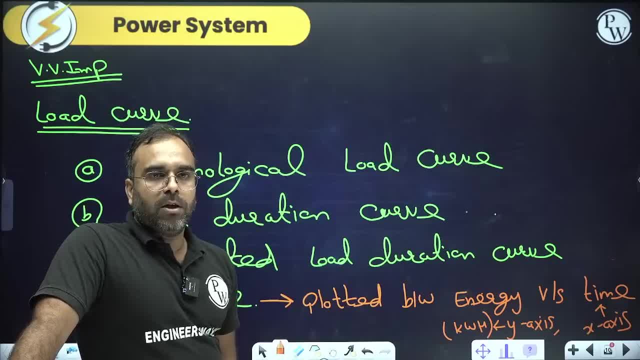 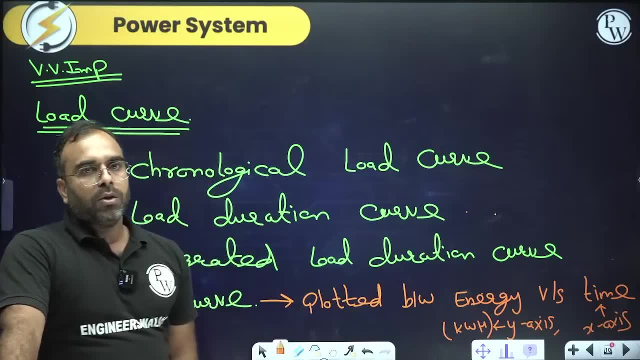 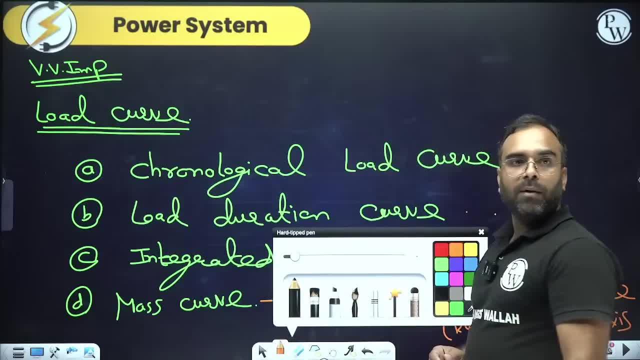 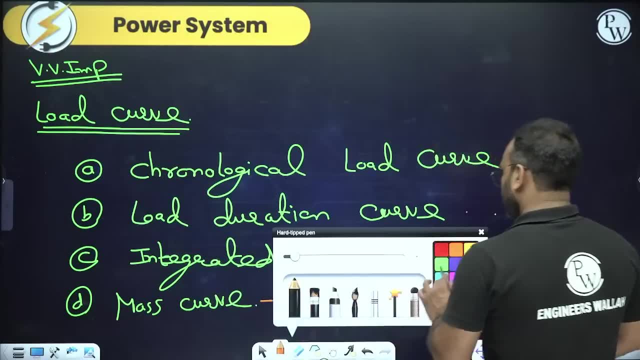 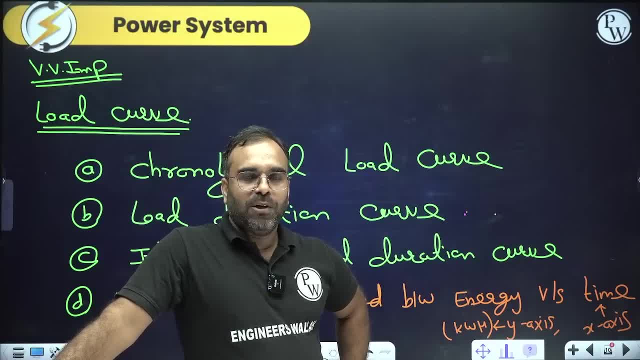 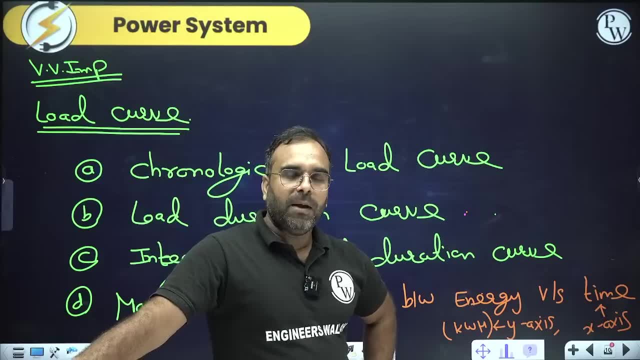 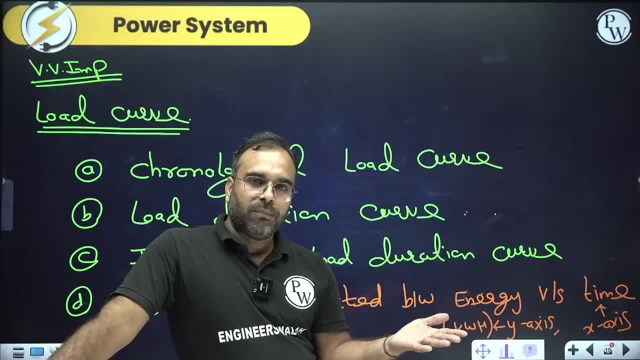 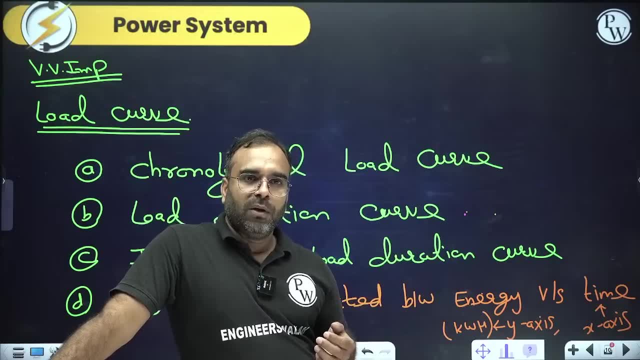 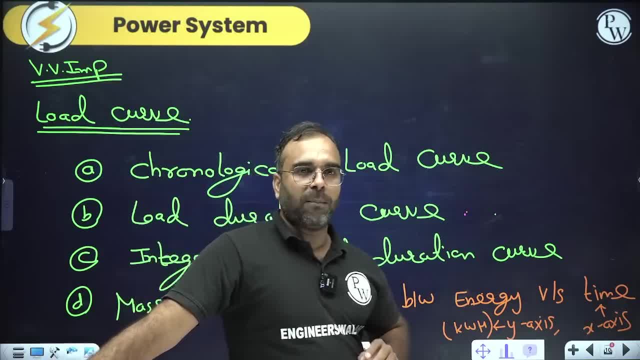 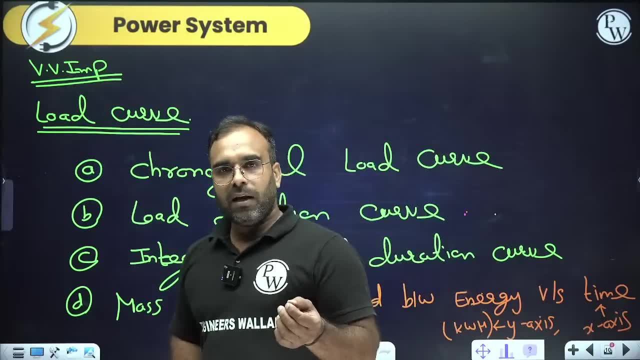 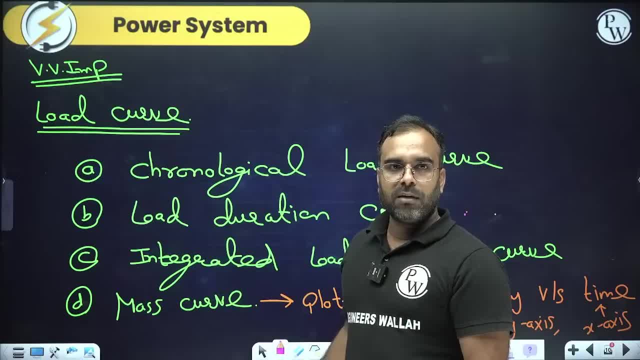 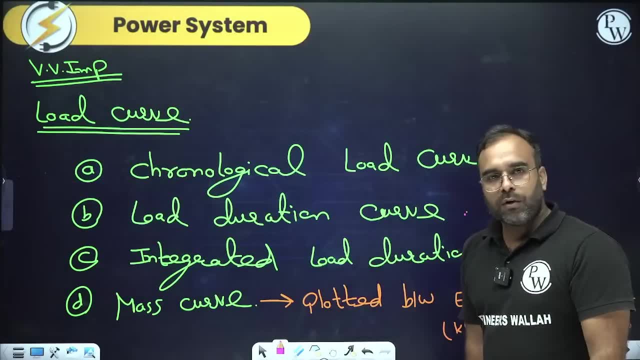 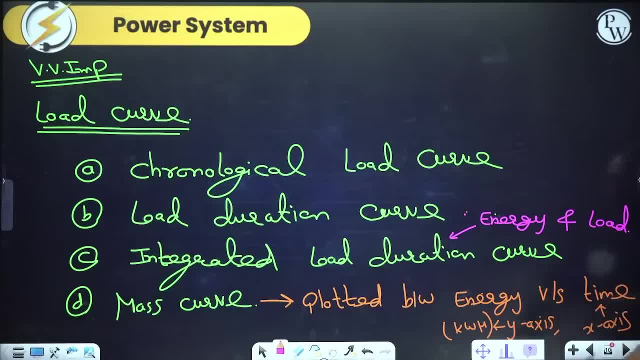 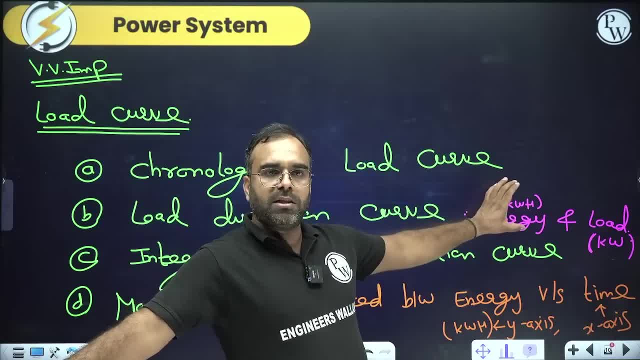 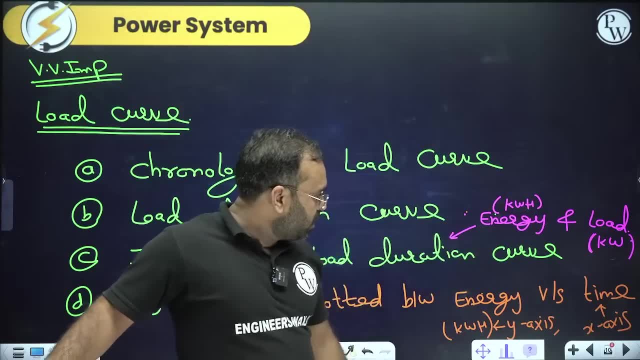 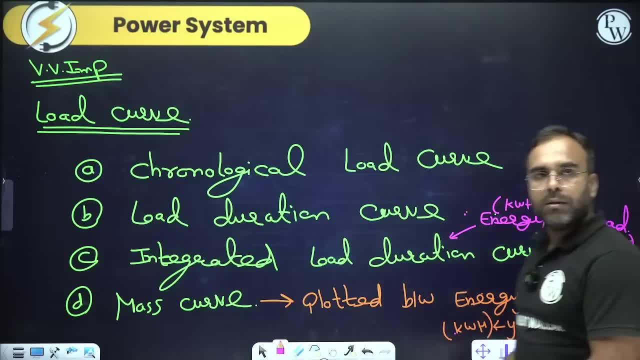 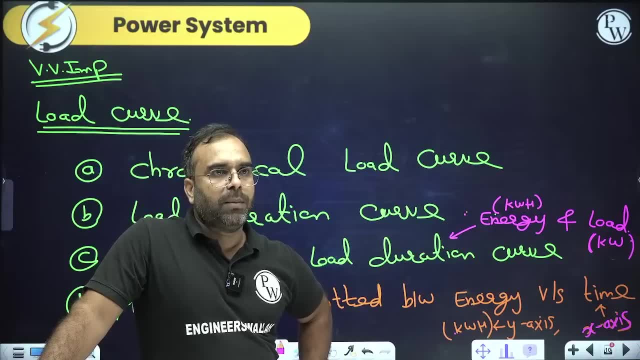 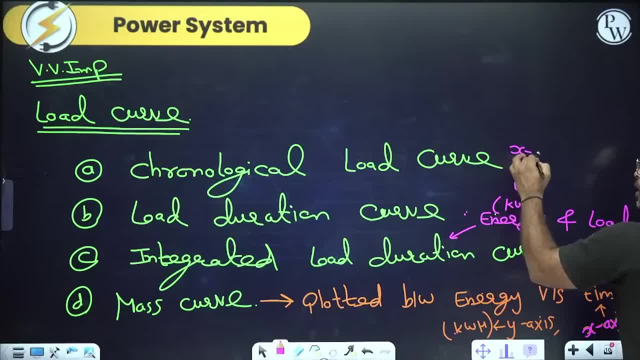 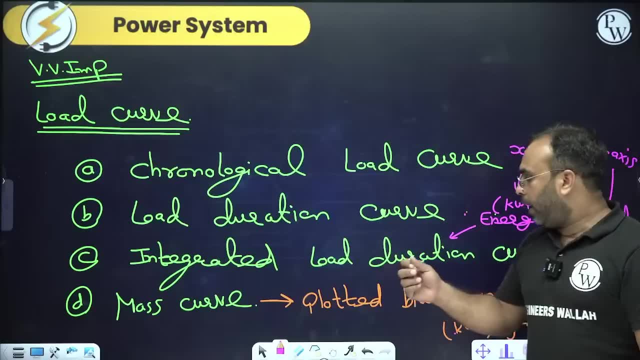 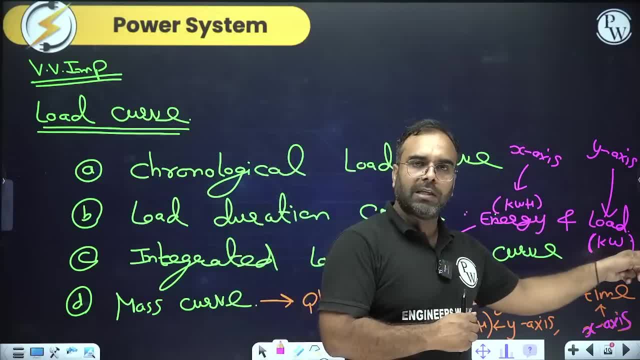 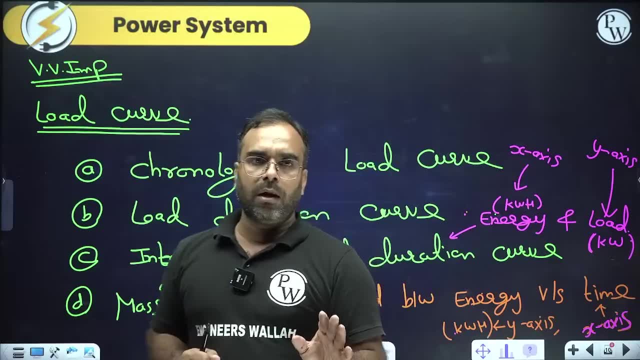 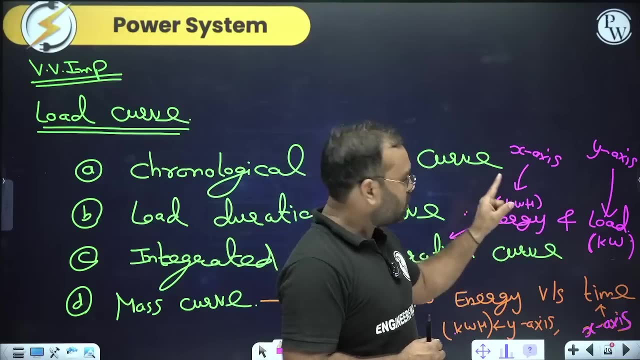 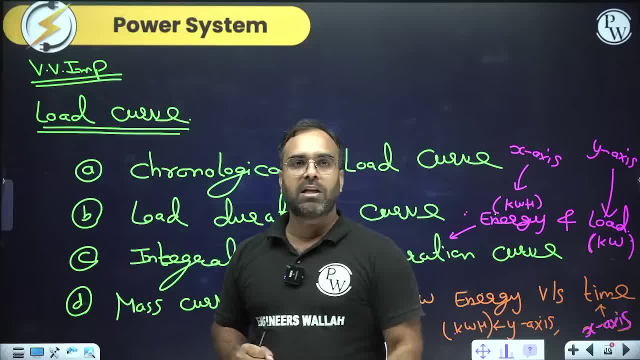 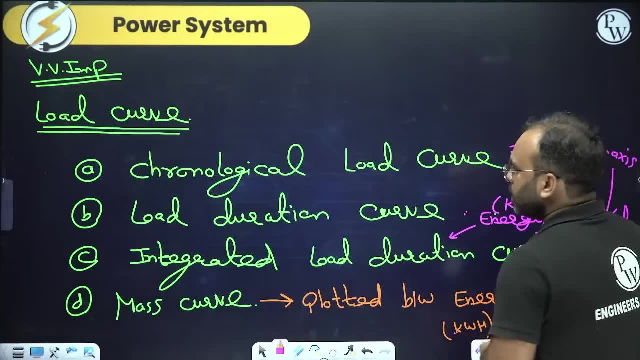 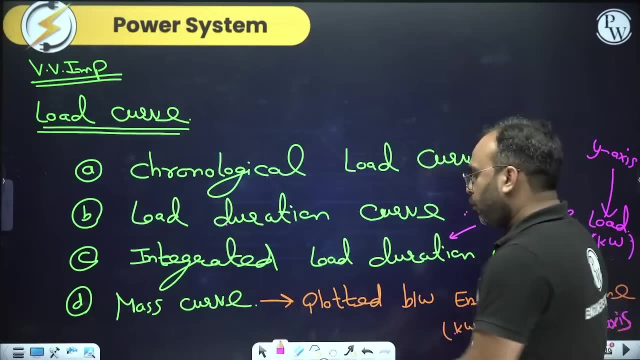 y axis and what is written later will come to x axis. there is nothing like this, ok. Next, after this, if we talk about next, understand this is with us. after this, do load duration. the examiner will ask you to do load duration in which they plot. so 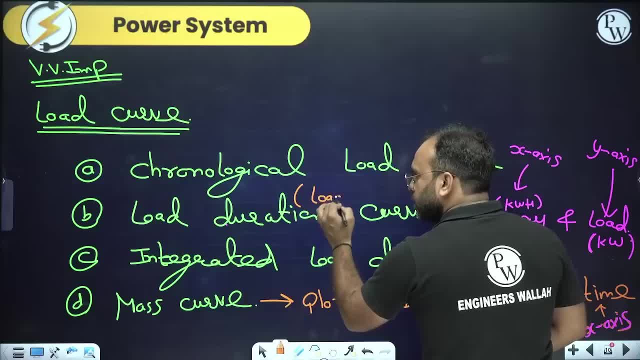 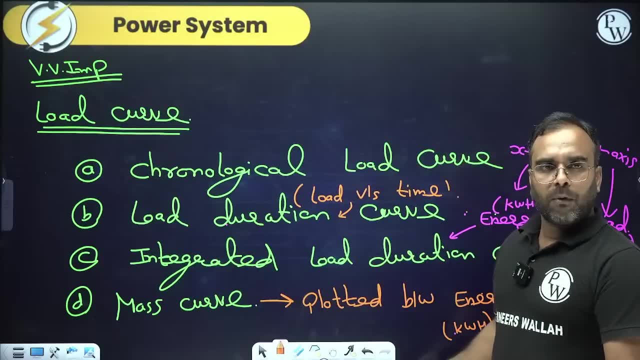 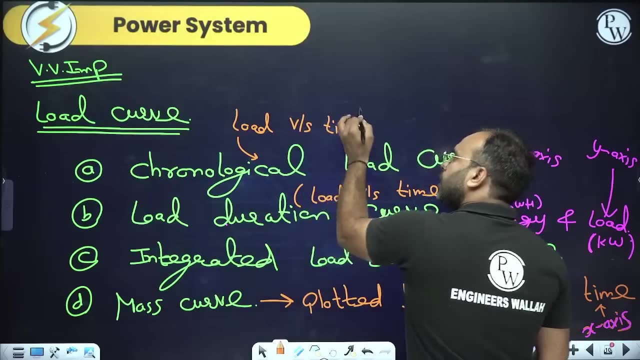 see, in the input of load duration we plot load versus time. this is the Shannon load versus time. and this too we plot in load versus time. so we will tell you so soon that what is the difference. the load curve of the chronologist is also plotted in load versus. 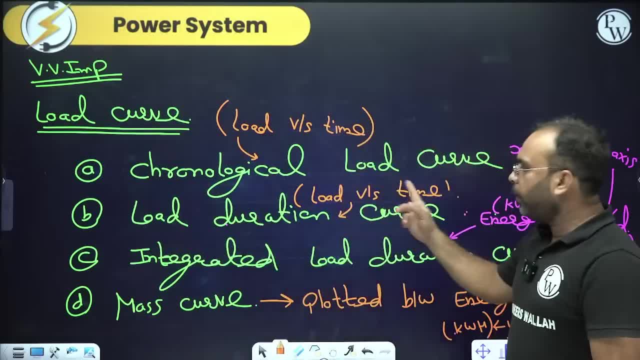 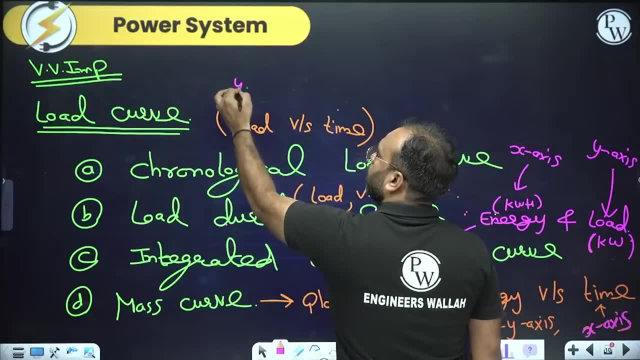 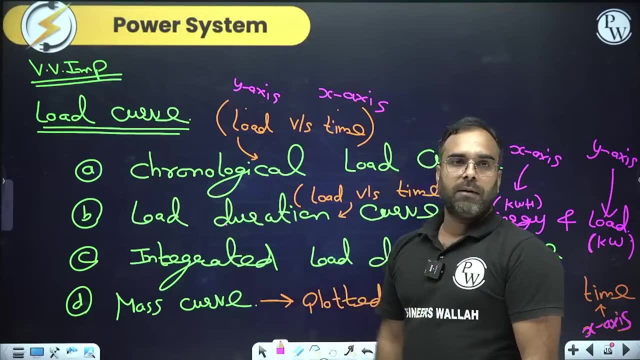 time during the load duration. it is also plotted in the load versus time in which load is on y axis, time is on x axis. This will be on y-axis and this will be on x-axis, But the examiner will tell you that. what is the difference between these two? 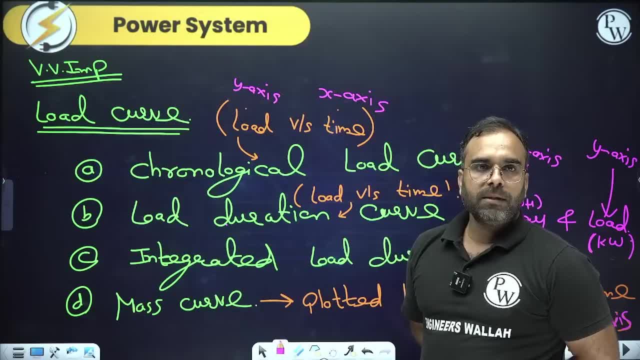 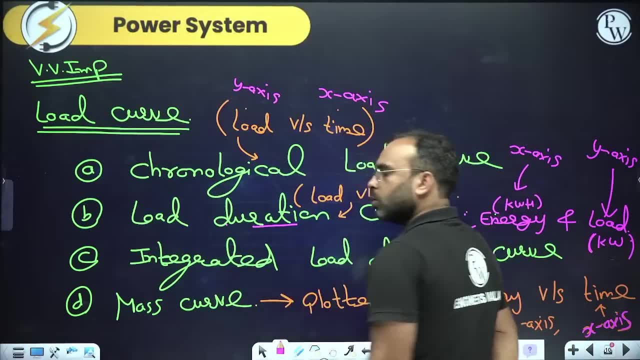 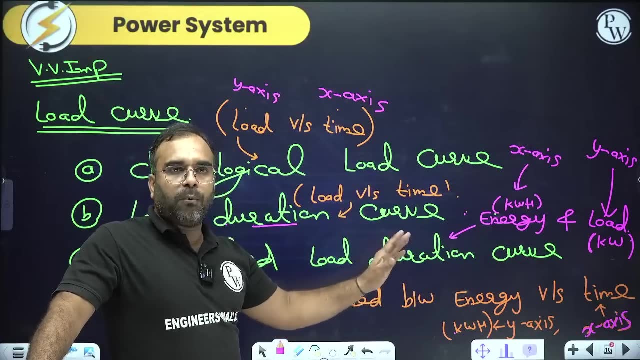 What is the difference? Tell me quickly. What is the difference. Yes, it is in decreasing order, So the load in the low duration curve is in descending order. I will explain you the meaning of this, because you will get many questions from here in the exam. 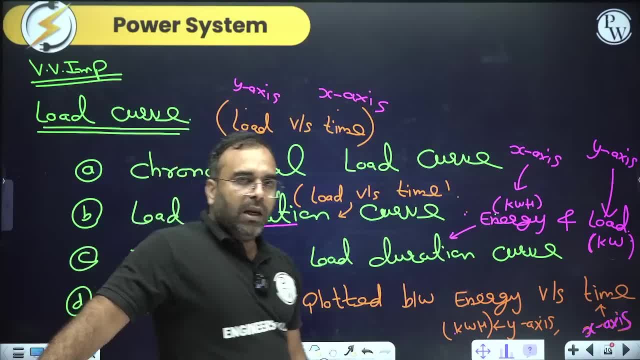 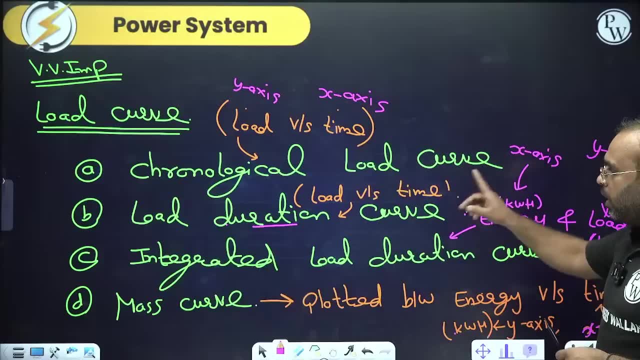 You will definitely get it in the exam. So did you understand What I said? Chronological load curve, load duration curve, integrated load curve and mass curve. You will remember all these questions. Now I will tell you the difference between these two. 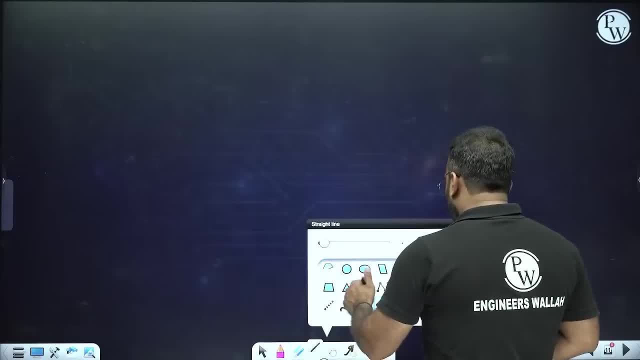 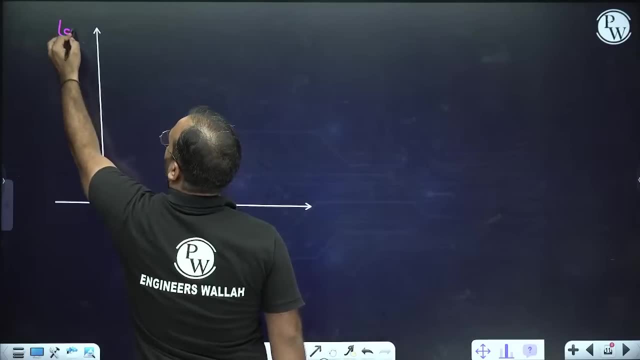 What is the difference between them? Suppose if I talk about your daily load curve. So what will happen in the daily load curve? Here you are consuming power, Here I am writing load on y-axis And on the x-axis. we will have time. 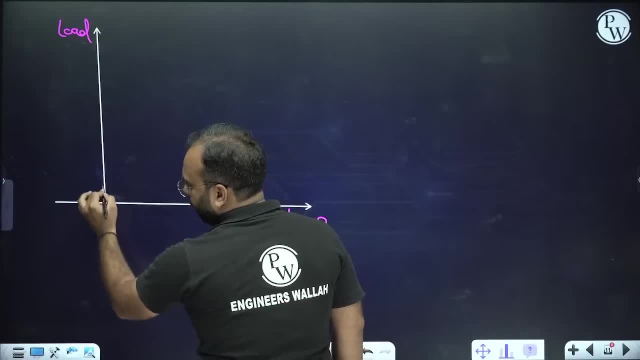 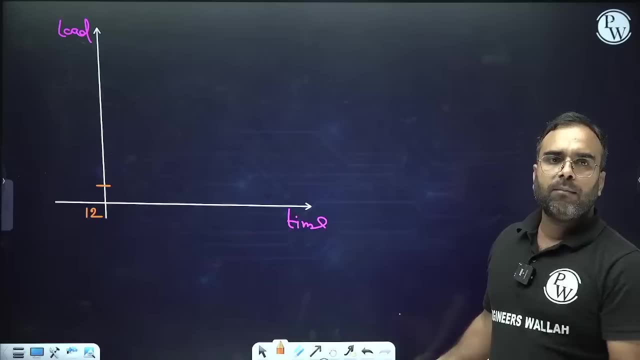 If I talk about the demand of power at 12 o'clock at night, You all know that you must be sleeping, You must be reading a lot, Otherwise the demand of power is the lowest at night. But as soon as it is 10 in the morning, then when the demand of power is 10 am, 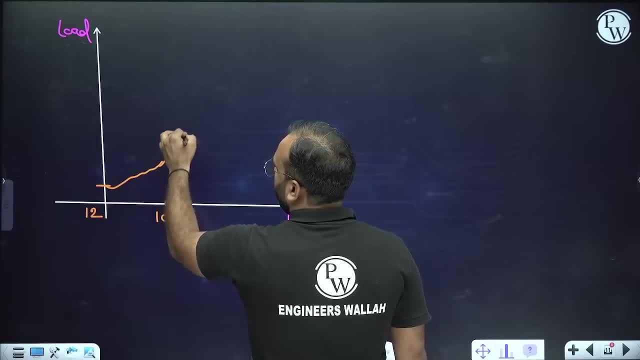 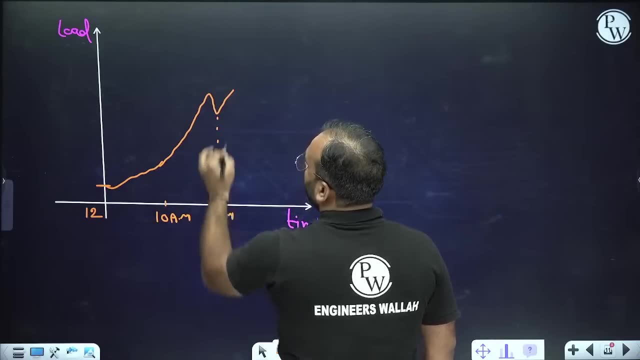 Then the demand of power will gradually increase And the demand of power will increase. But around 1 o'clock in the day the demand of power comes a little deep, Approximately around 1 pm. Then the demand of power increases And the maximum peak goes between 5 to 7.. 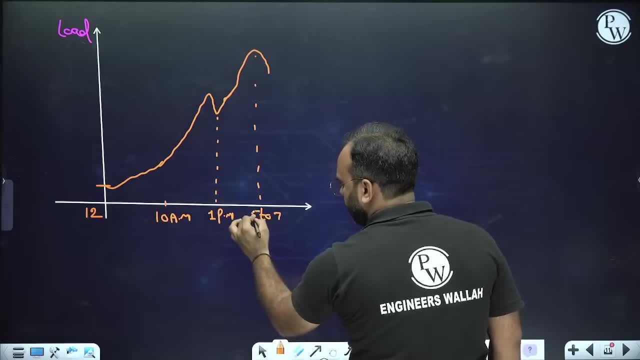 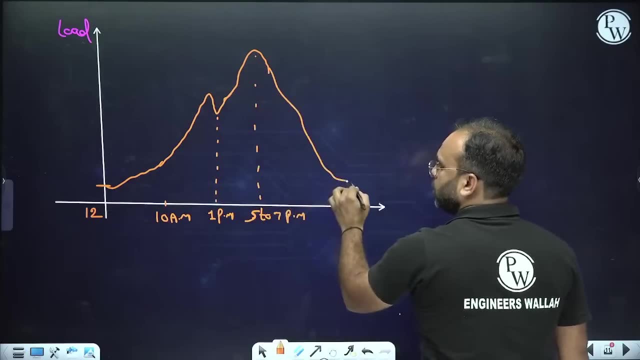 Right Between 5 to 7 pm, The demand of power increases a lot, And after that, if we talk about it, Then again at 12 o'clock at night, the demand of power comes the same. Such a curve is plotted on the substation. 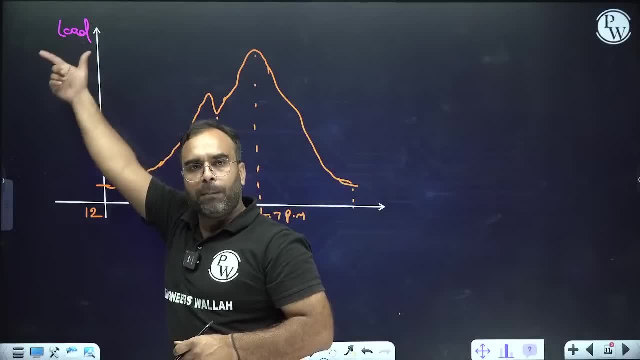 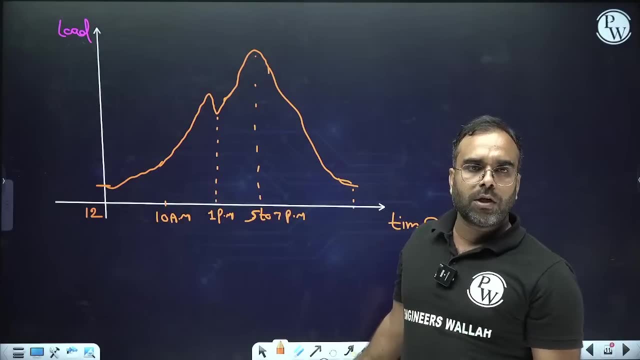 The load power that you consume on the substation, And here, in respect to time, that curve is plotted, This is called the load duration curve. So I have made this load duration curve in front of you, Sir. we call this chronological load curve. 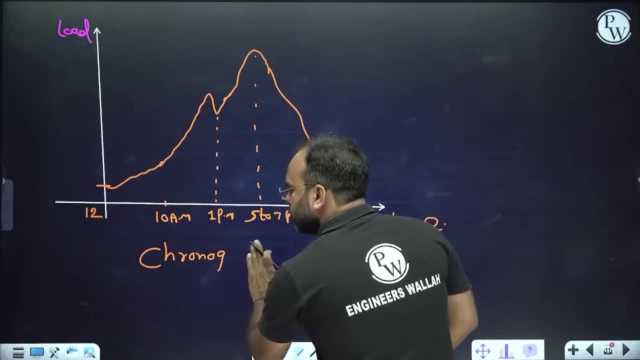 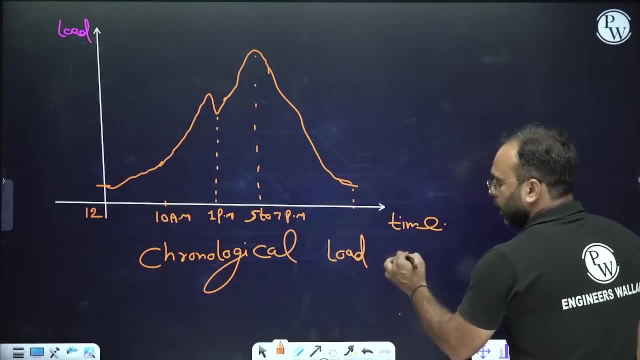 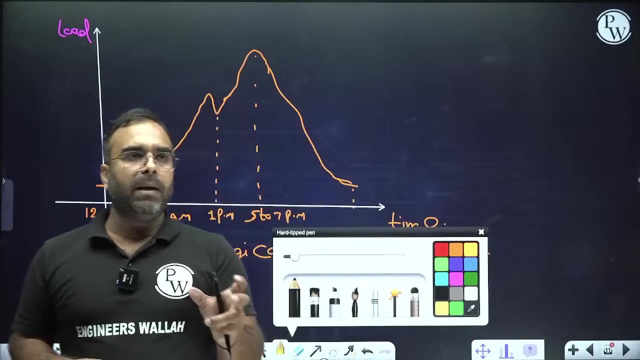 We call this chronological load curve. This will be in front of us: Chronological load curve. This will be the chronological load curve. Now the examiner will ask you a question In the exam. the maximum demand of power in the whole day. 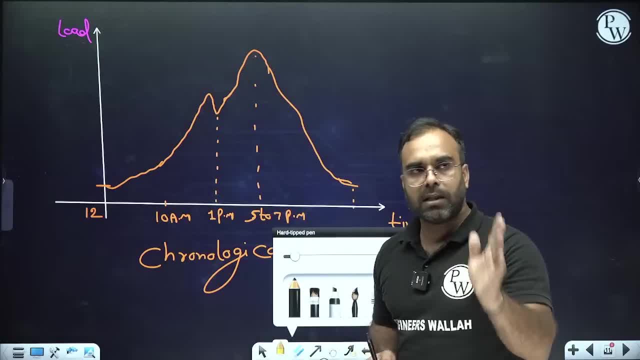 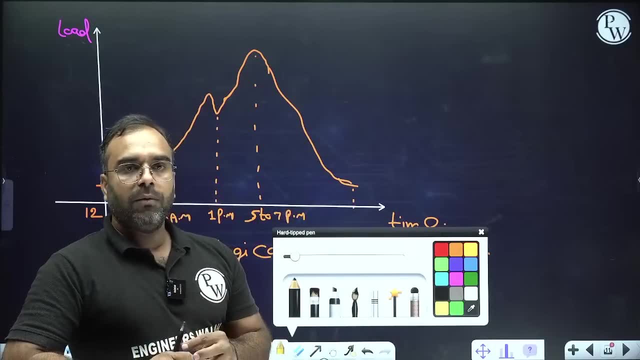 What is the maximum time duration? What will be the answer? We will tell you quickly. The examiner will ask you That, in the whole day, What is the maximum demand in the whole day, What is the maximum duration? So your answer will be: 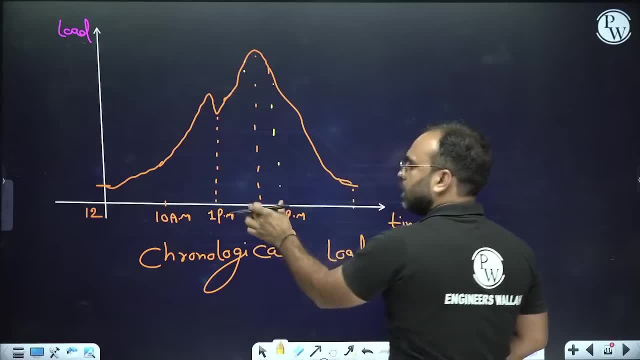 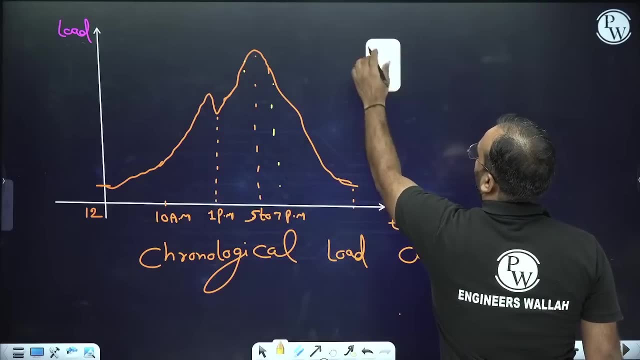 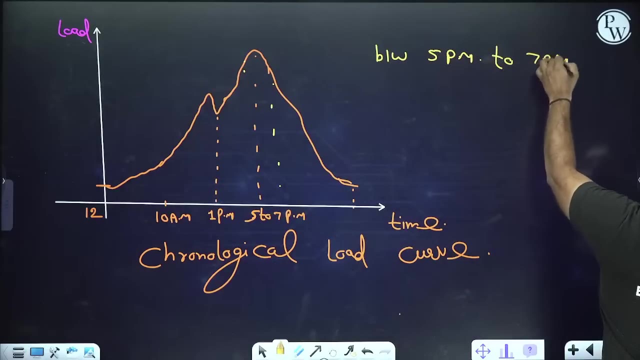 The time duration of 5 to 7.. The time duration of 5 to 7.. In that the maximum demand will be more. So here write between: Write a point here. Between 5 pm to 7 pm, What will be? 7 pm. 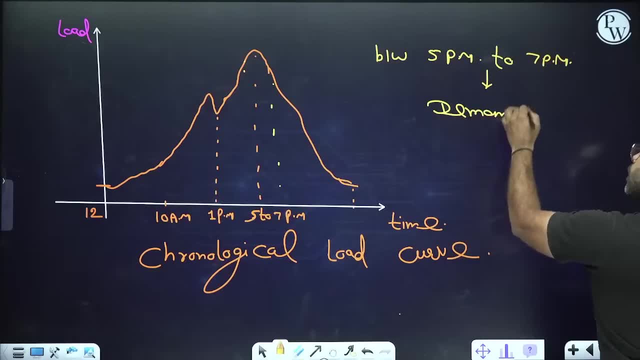 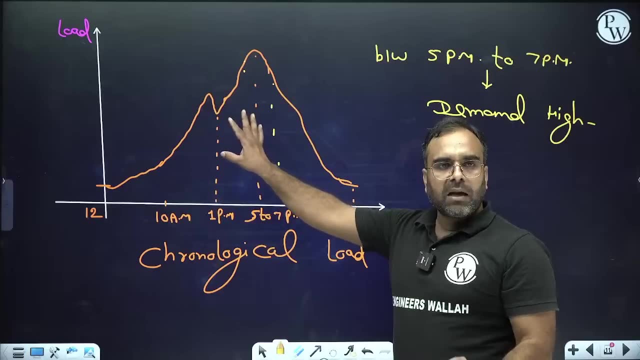 The demand will be high. What is the demand? The demand will be high or the demand will be increased. The demand will be the highest among us. So I have made this curve. But if we do this kind of representation of this curve, 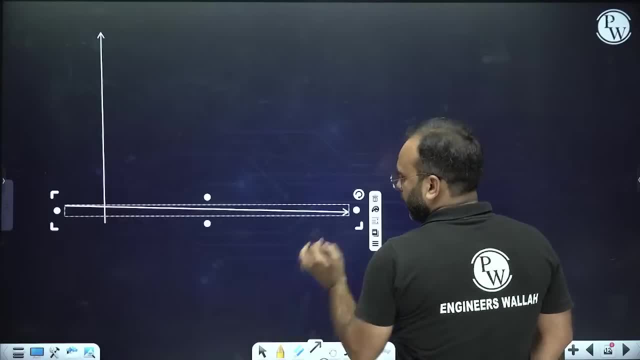 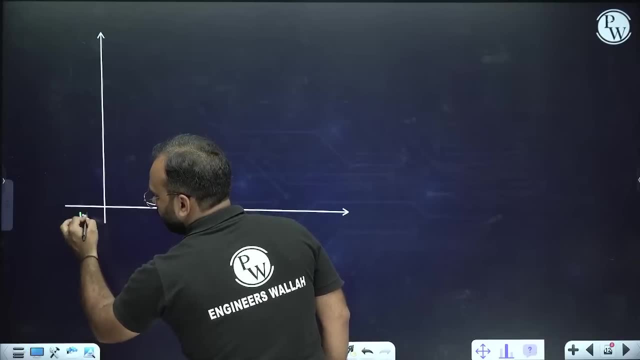 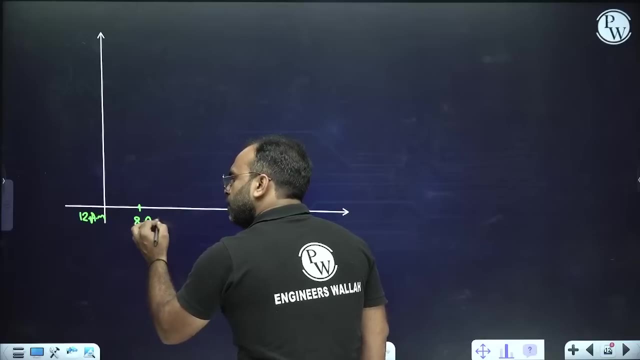 If I do this kind of representation of this curve, That what will happen here? Here, let's assume that from 12 am to 8 pm, From 12 am to 8 pm, From 12 am to 8 pm, The demand of your power is this much. 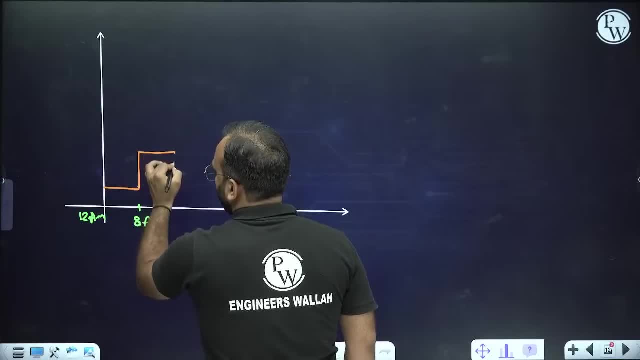 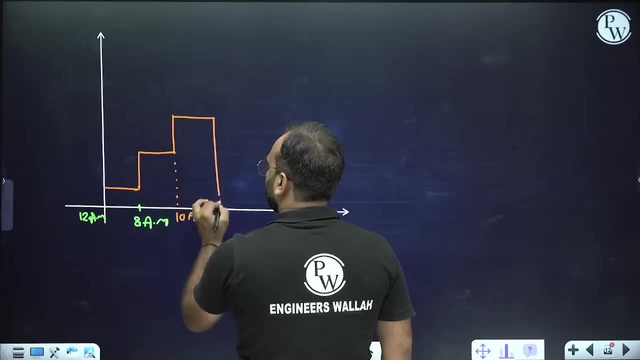 Then, from 8 am to 10 pm, The demand of your power is this much: This is till 10 am. Then after that, The demand of your power is increasing till 1 o'clock. This is till 1 pm. This is till 10 am. 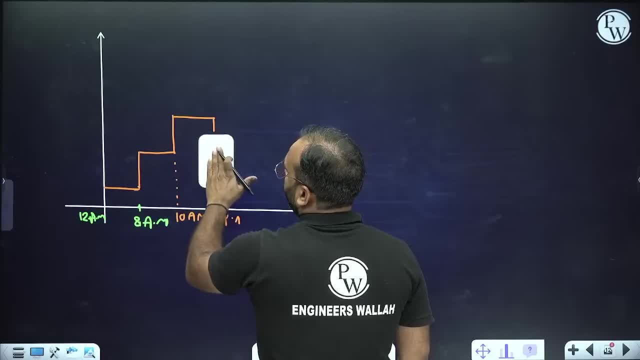 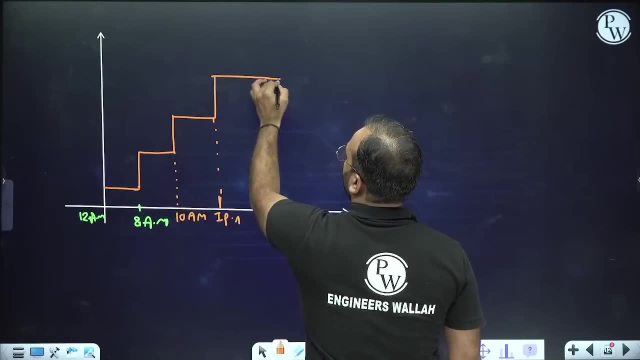 This is till 1 pm. This is the demand till 1 pm. Next, What will happen after that? What will be our demand? From 1 pm to 7 pm? The demand of your power is this much: This is till 7 pm. 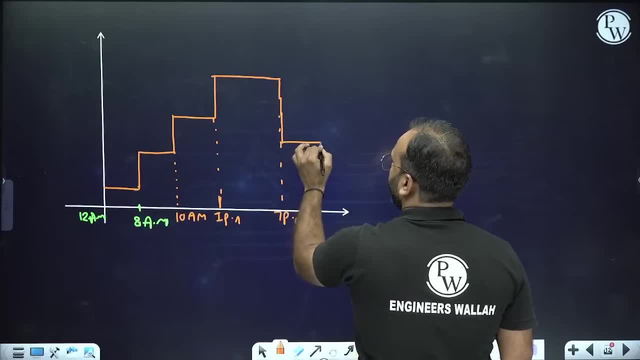 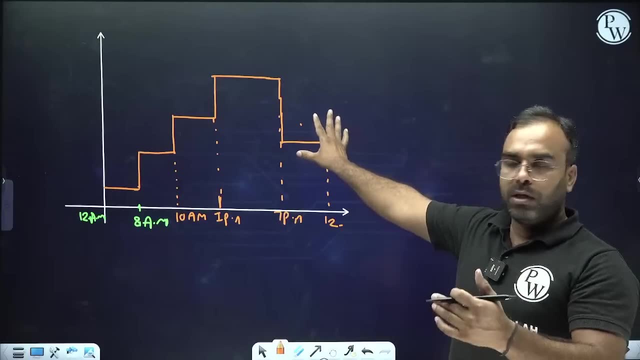 Then from 7 pm to 12 pm. This is the demand till 12 pm. This is the curve that I have made. Actually, this is the chronological load curve, But this is not the load duration curve. Note that this is not the load duration curve. 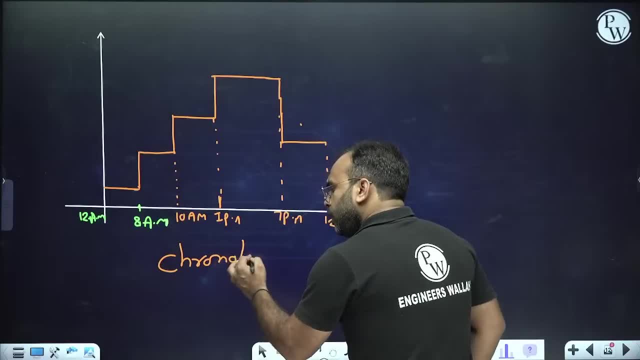 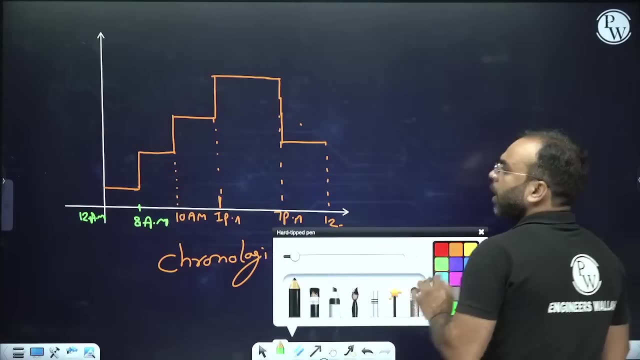 This is also what I have made. This is the chronological curve. Now, what will be the load duration curve of the chronological curve? So understand, Suppose here you have a demand of 30 kilowatts. Here we are writing the load in kilowatts. 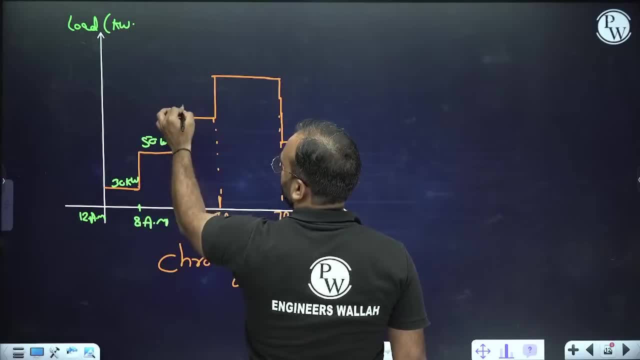 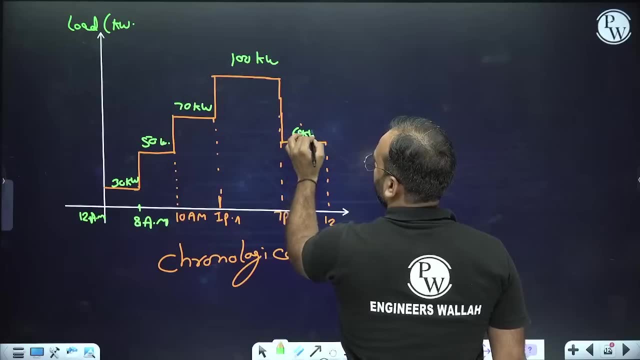 Here is the demand of 50 kilowatts, Here is the demand of 70 kilowatts, Here we have the demand of 100 kilowatts And here is the demand of 60 kilowatts. This is the demand of our load. 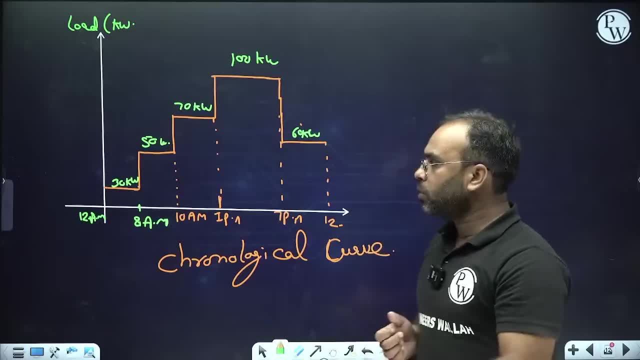 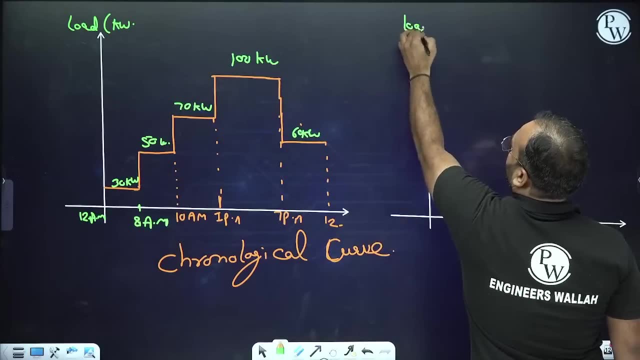 If I want to make a load duration curve here, If I want to make a load duration curve, So understand, I will write the load on the y-axis, We will write the load on the y-axis And here we will write the time. 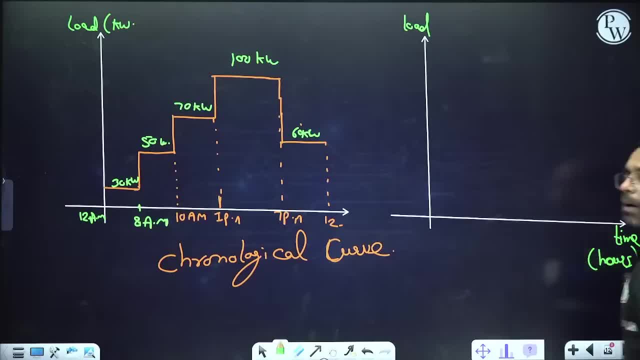 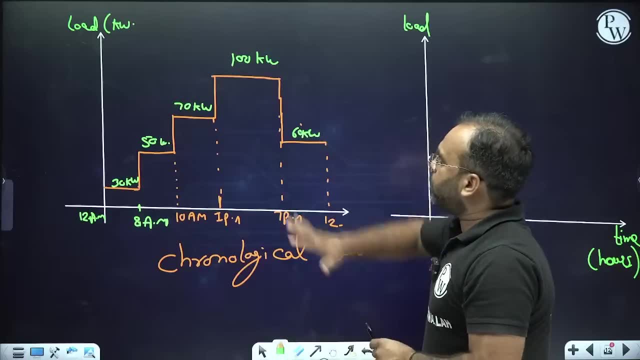 But keep in mind that the time will be in the hours here. The time will be in the hours here, Nothing else. So there will be one change: The time of the x-axis will always be written in the hour. Now you tell me for how many hours your power is the most. 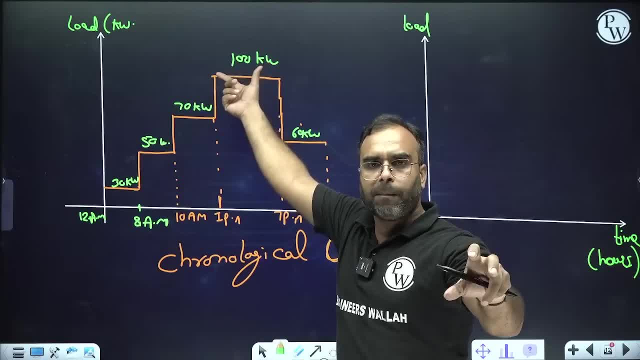 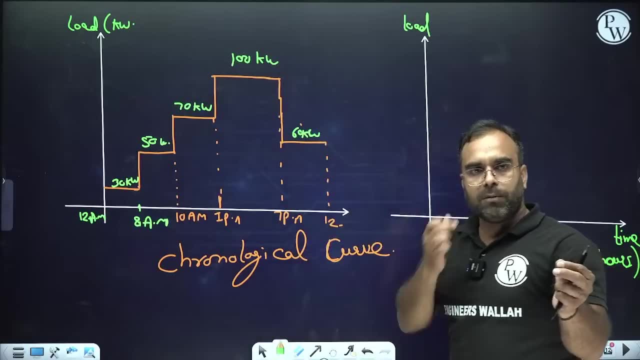 First of all what to do. Write in descending order, That is, write the highest power first. So the highest power is 100 kilowatts. For how many hours, Tell me quickly. Here you are told that the highest power is 100 kilowatts. 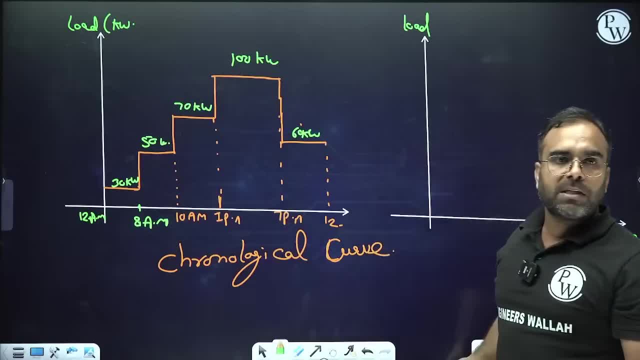 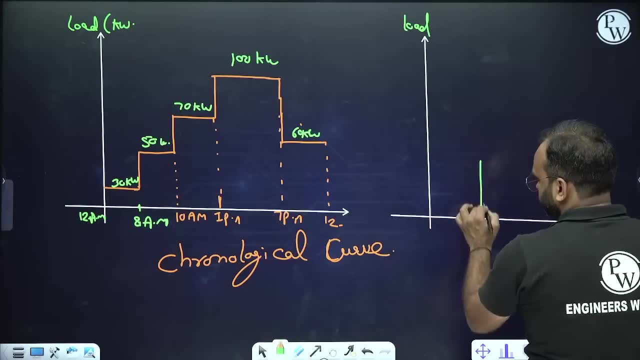 And for how many hours? So from 1 to 7, how much will we have For 6 hours, From 1 to 7, what will we have If I talk for 6 hours? So for 6 hours there is a demand of 100 megawatt power. 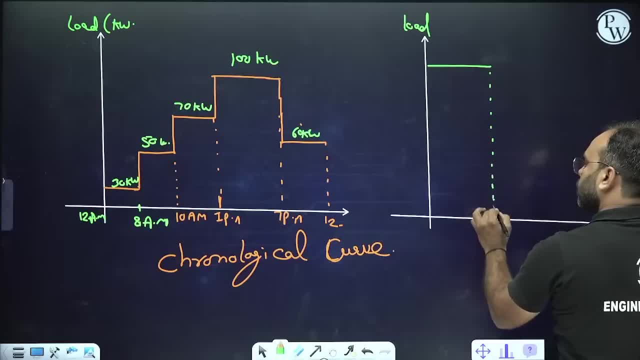 So this is our 100 megawatt, But for how many hours? So keep in mind, For how many hours? For 6 hours After that, who is there? So you are getting 70.. For how many hours is 70?? 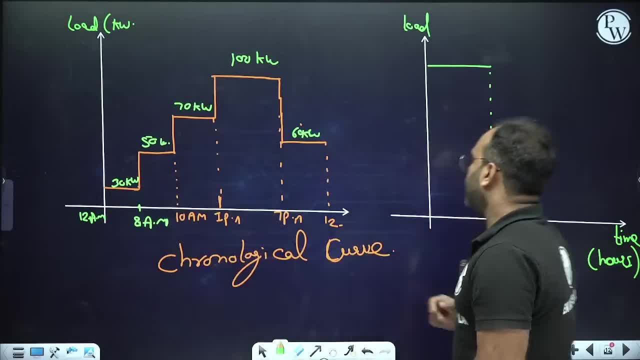 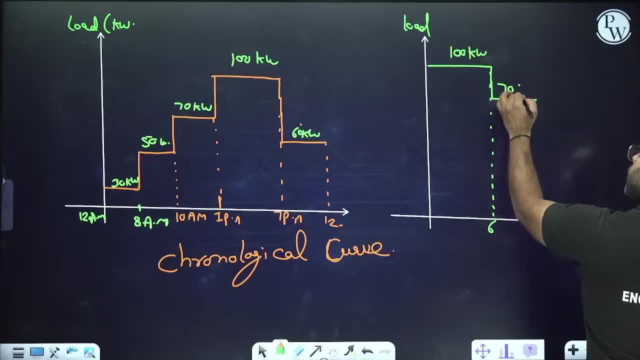 From 10 to 1.. From 10 to 1 means for 3 hours. For 3 hours is 70. So these are kilowatts. How much is it for 3 hours? 70. And where will we get that? 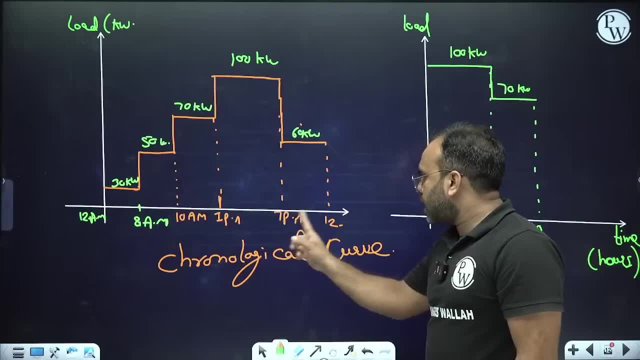 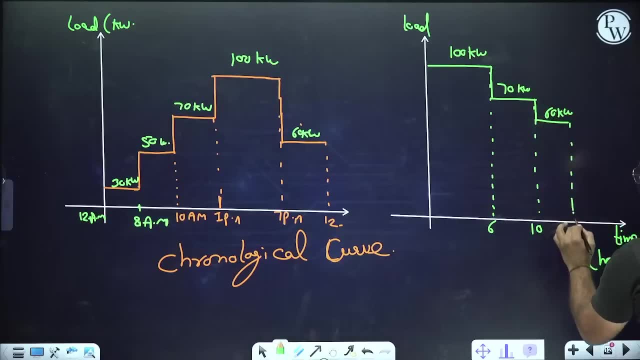 It will be 10 hours After that. for how many hours is 60?? From 7 to 12 means for 5 hours. For 5 hours is 60. So here 60 will be for how many hours? For 5 hours means it will be 15 hours. 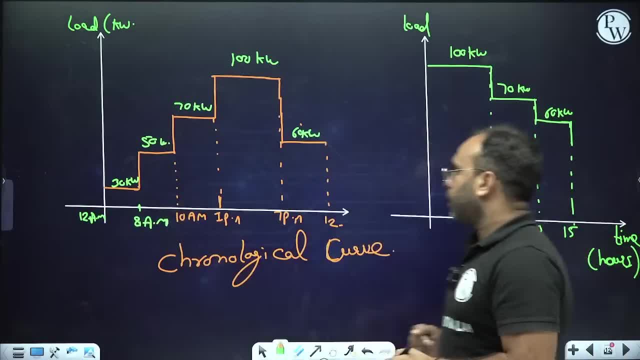 Next, what is after this? So here, for how many hours is 50?? For 2 hours? So for 2 hours. from 8 to 10 means for 2 hours, So it will be 17 hours. It will be 17 hours. 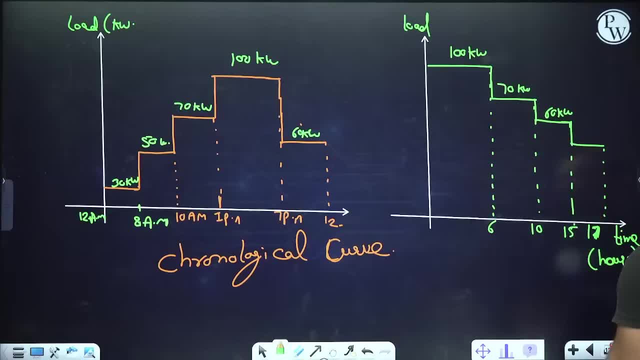 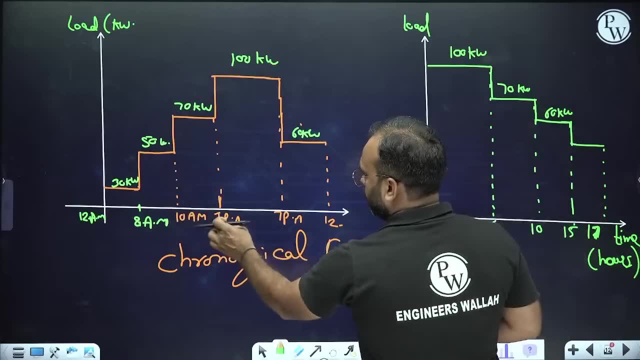 And if we have 17 hours from here, Has anyone made any mistake? From 7 to 12 means 5 hours. First, what do we have? From 1 to 7 means 6 hours. From 10 to 1 means 3 hours. 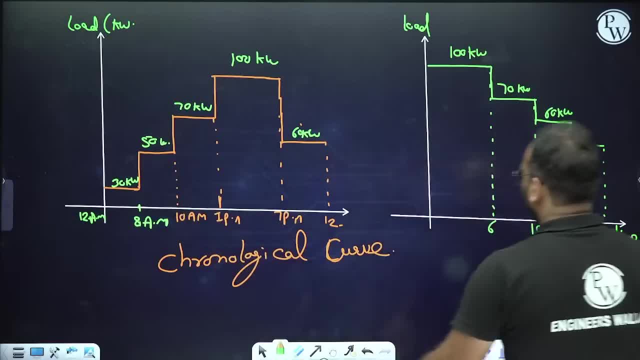 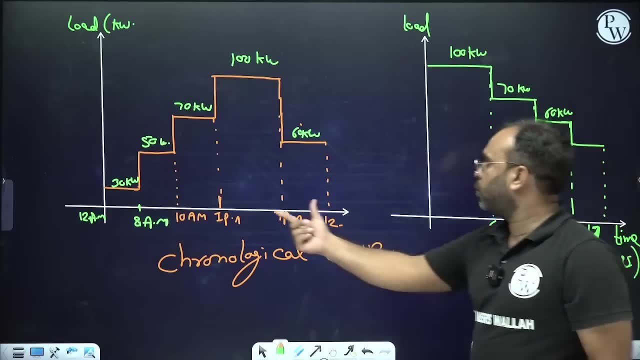 This is 5.. 5 and 6 and 2 means 5.. And how much will be here? Will there be any changes Here? what we will have First 6 hours. Second, what do we have For 3 hours? 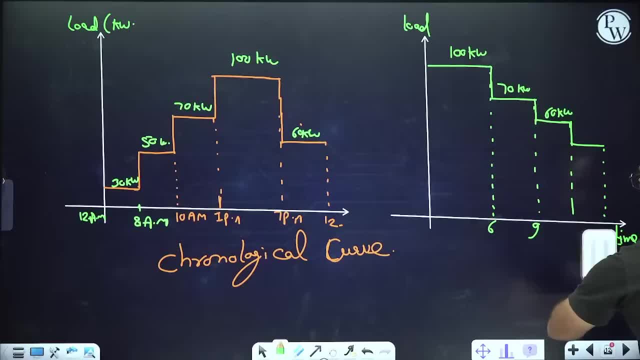 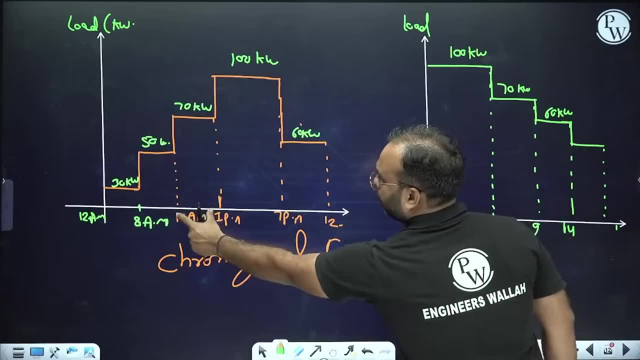 So it will be 9 hours After 9,. if we talk, then here is 5.. So it will be for 14 hours After 14,. here it will be 2 hours, So here it will be 16 hours. 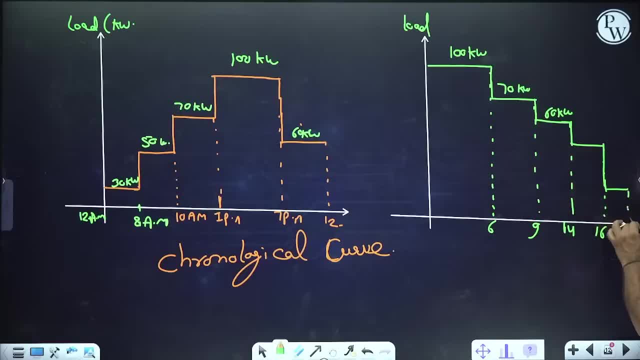 And for next 8 hours it will be 30 hours. So this is 24 hours Like this we have. Yes, 9 will come Definitely 6, 9,, 14,, 16,, 24.. This curve which I have made, 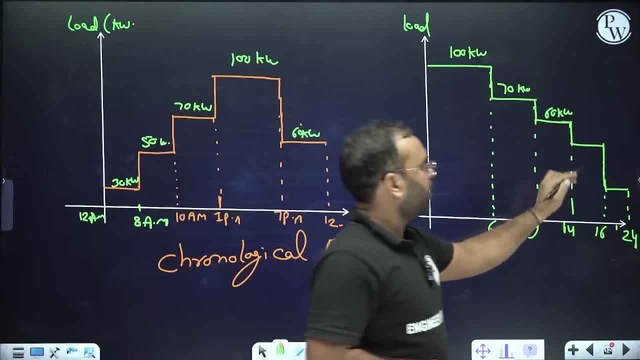 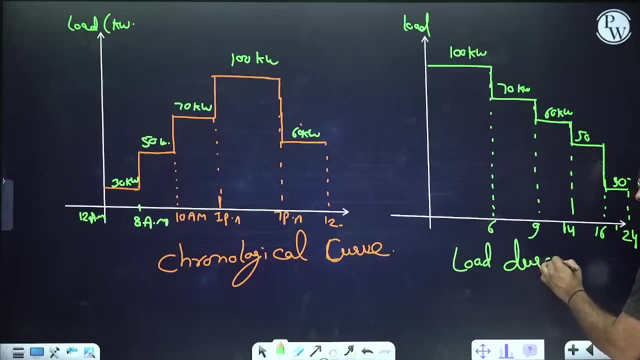 This is called low duration curve. I have made 30 here. This is 50 and this is 30. Finally, you have understood that. what is low duration curve? Tell me quickly. Tell me quickly what is low duration curve. What is low duration curve? 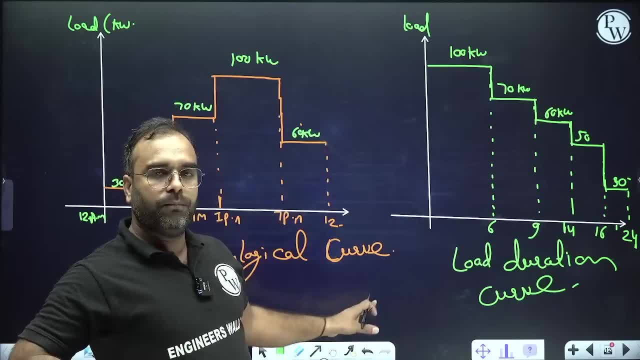 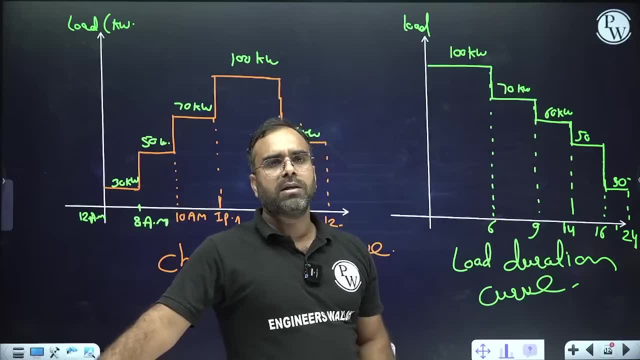 That is not understood. I mean, the most important is that this is how the low duration curve is made. So I am assuming that in CBT1, there are few chances, But in CBT2, there are a lot of chances of numerical coming on it. 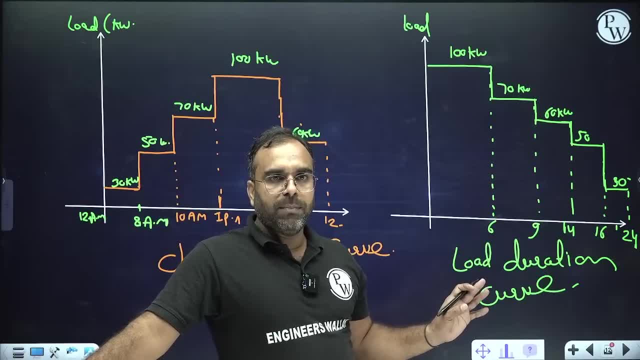 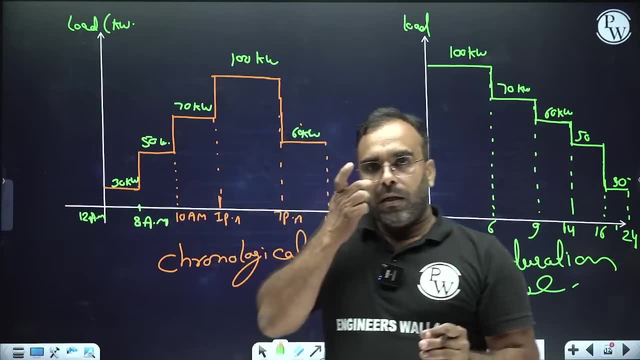 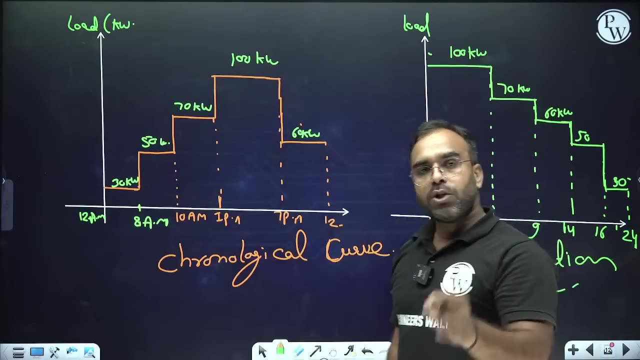 Many questions will be asked in the exam. Did you understand this? Yes, here our load will go in descending order. So the examiner asks you the question that the peak of the low duration curve here or the peak of the chronological load curve. what will it show you? 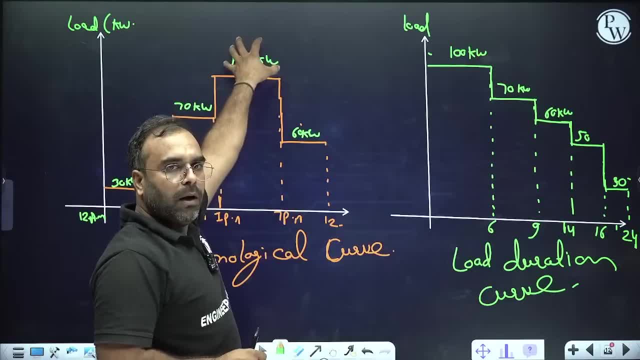 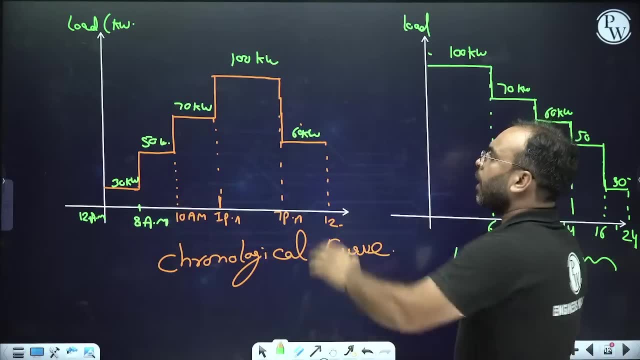 Then it will show us the maximum demand. That is, if you are ever told. if you are ever told that the maximum demand of any system is how much, then the maximum demand will be the peak. Whose peak will it be? Whether you talk about the peak of the chronological load curve? 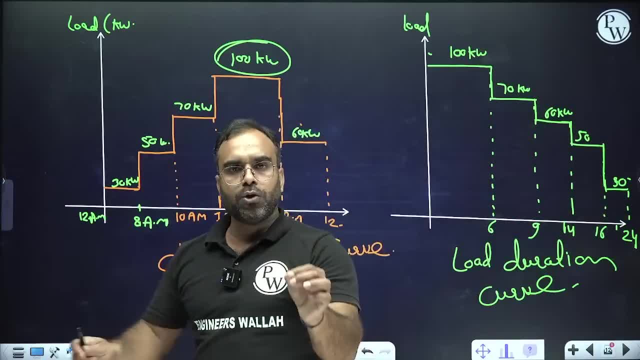 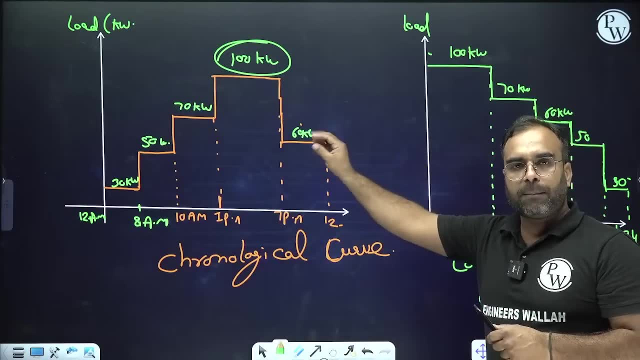 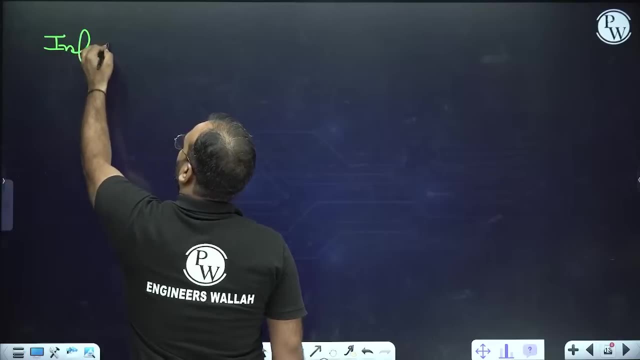 or the peak of the low duration curve, then its peak will always show you the maximum demand. So the examiner question is that: what information do you get from the load curve? Tell me quickly, You will be told, the information obtained from information. information from: 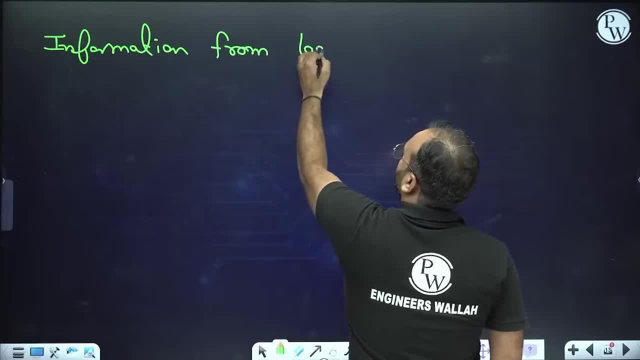 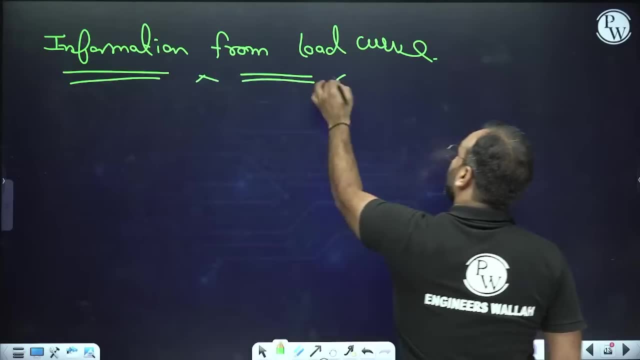 where? Tell me quickly, Load curve. So what information do you get from the load curve? You will be asked this examiner question. So what will be the answer? Tell me quickly, What information did you get? The first information you have got is that 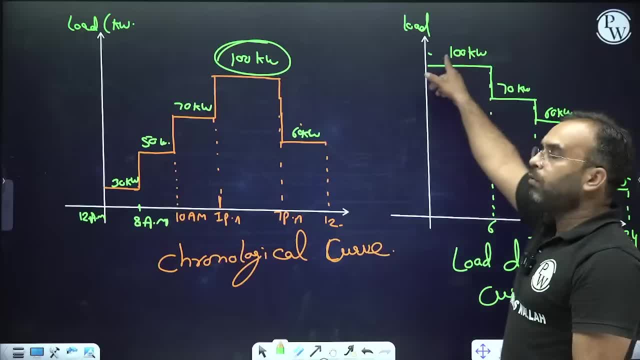 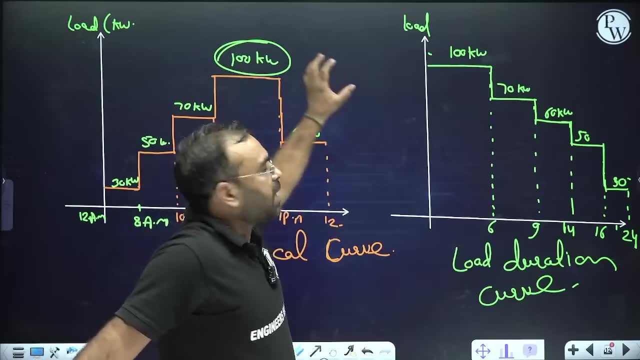 what is the maximum demand of your system? If I give you the load curve, I will make it for you. I will make it for you. I will ask you, tell me, what do you know? What will you say, Sir, we know the maximum demand. 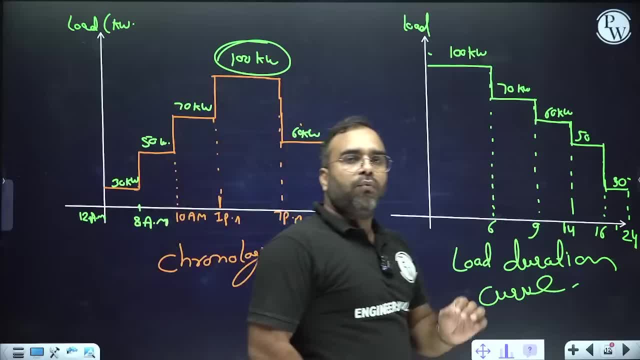 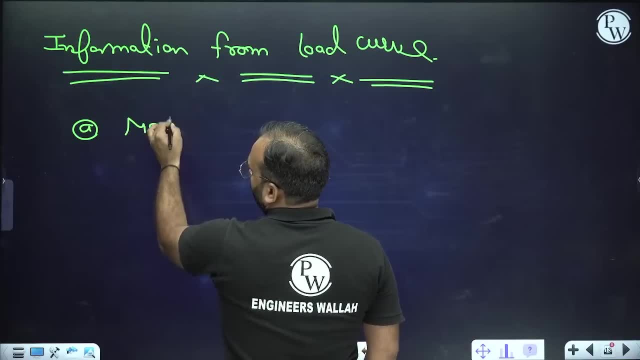 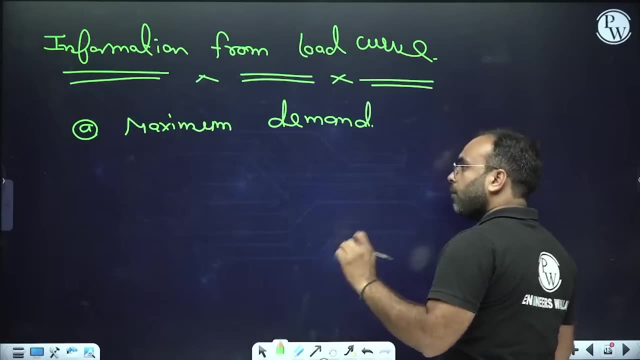 What do you know, Sir? we know the maximum demand. So what does this mean? We will know the maximum demand. The first will be about the maximum demand, Maximum demand. Someone is saying that it is only for domestic load. No, we are making the load curve of the entire power system. 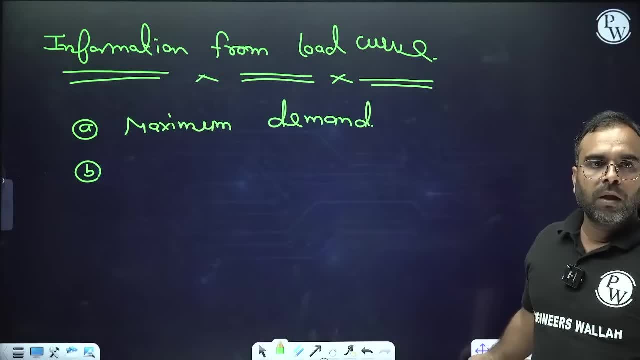 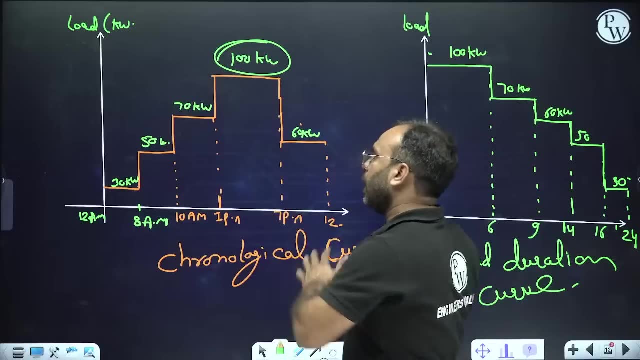 The load curve of the power system is not for domestic load. Next, After this, we will get the maximum demand. Suppose I have to calculate the average load for the whole day. If I have to calculate the average load, what will I do? 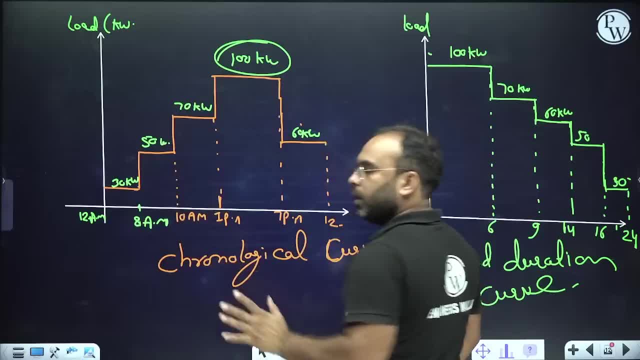 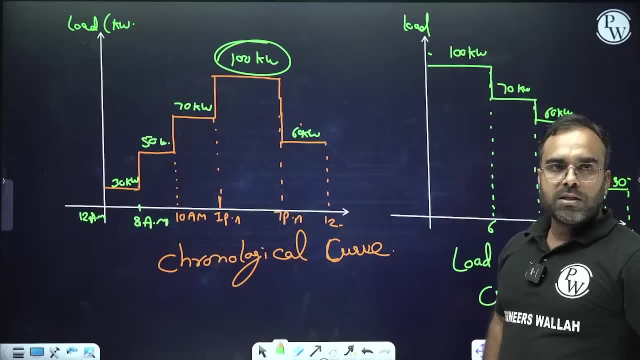 I will calculate the area and divide it by the time period. How do we calculate the average Area divided by time period? Yes, we will do that too. We will do the total status too. So keep in mind, If you are ever asked that, what is the average load? 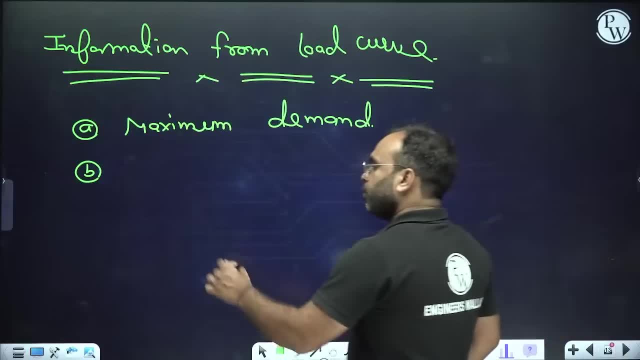 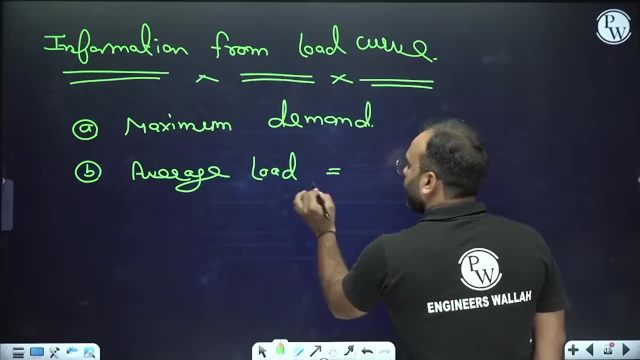 You can get it from 20.. So if you are asked that, what will you get? We will get one more. We have the average load, Average load. If you have to calculate the average load, what will you do? Area: Underload the area. 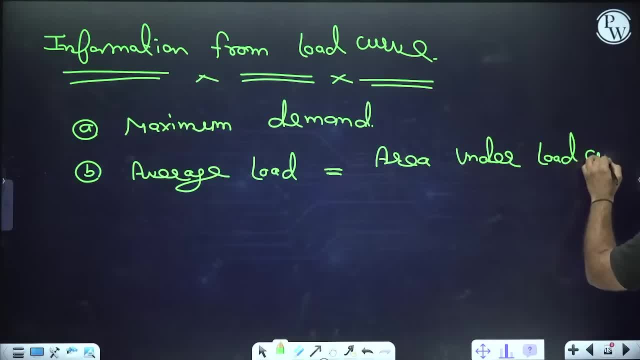 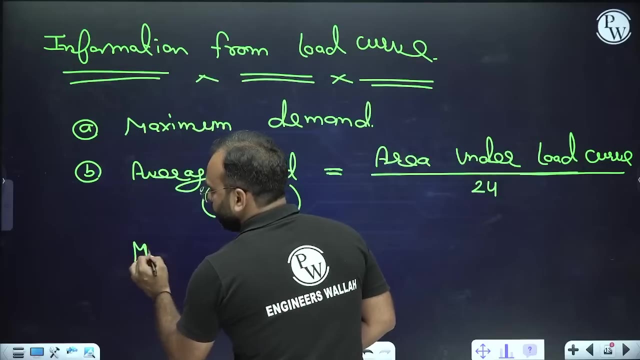 Underload the area. Underload the area. What will it be divided by? We divide it by 24 here. So this average load is daily. What will that be? That is daily average load If you are asked monthly. if you are asked how much is the monthly average load. 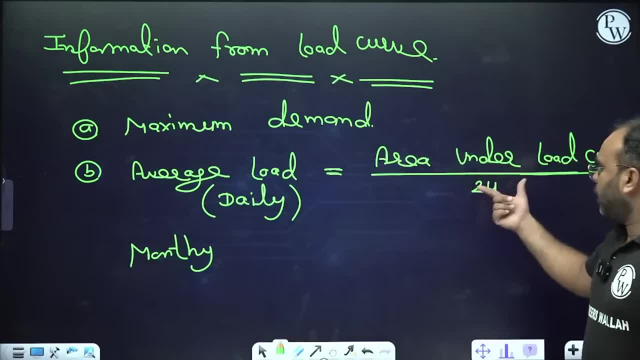 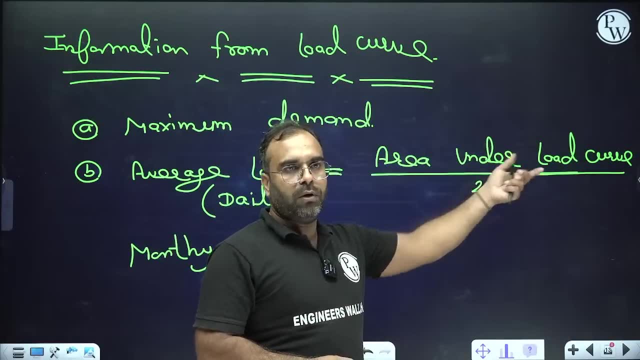 If you are asked monthly, then you have to divide the hours of the month. If you are asked yearly, then you have to divide the hours of the year. I will write that in the formula. But if you ever have to calculate the average load, 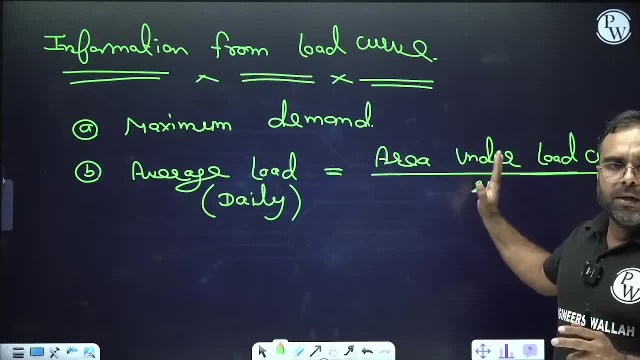 then you will do area divided by time period, Nothing else. You will do area divided by time period here. Yes, the divide of 720 will come And the divide of 8760 will come. Absolutely right For yearly, But let's go to that. 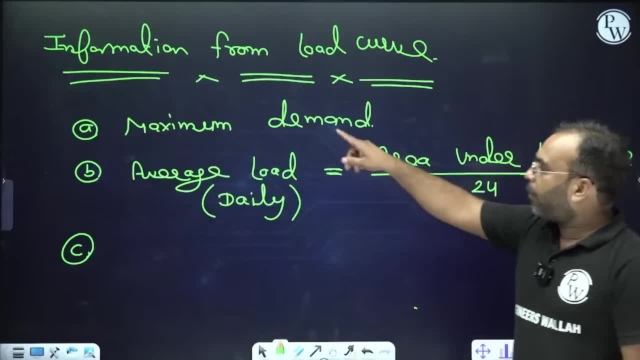 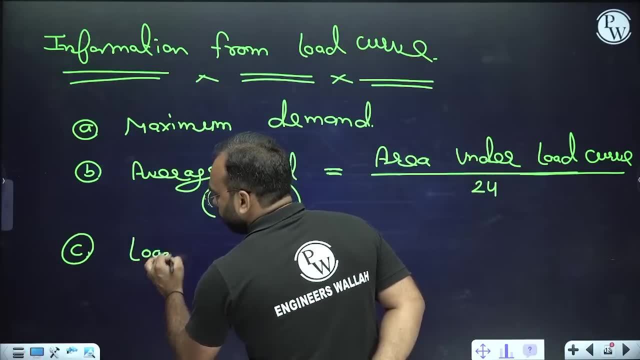 Before that, let's write one more thing here. If you know the maximum demand, if you know the average load, then what can you get from here? Load factor: Tell me quickly, what is the formula of load factor? The question from here is: 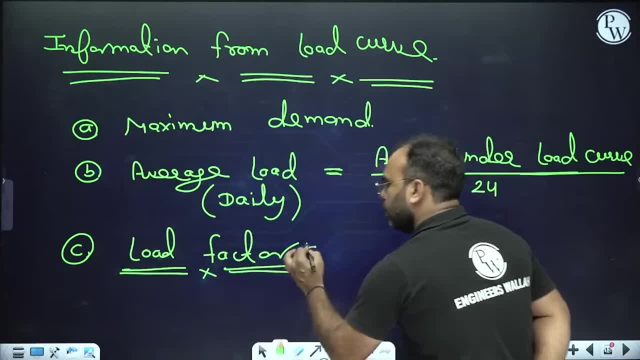 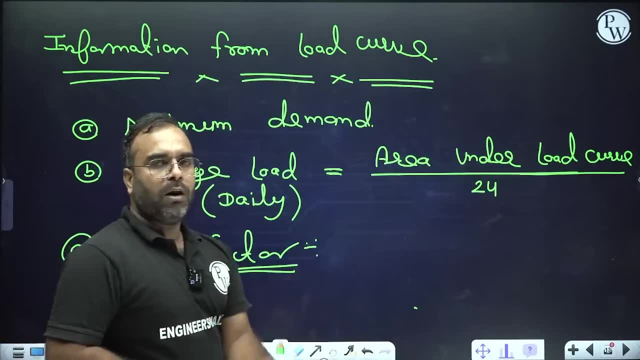 every year in SSE, JEE, almost every paper has two questions. with all these formulas, I am going there. I am going to the important topic. Keep in mind, it is a very, very important topic. From here, I will write you a lot of definitions. 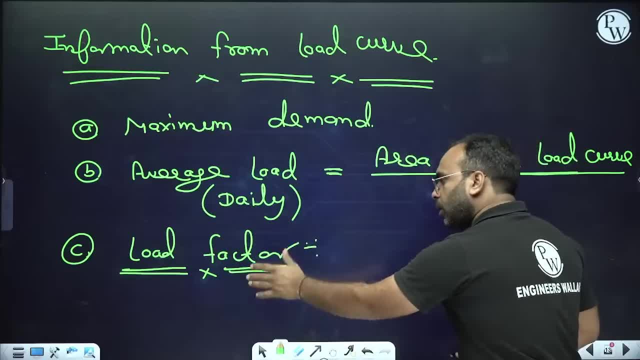 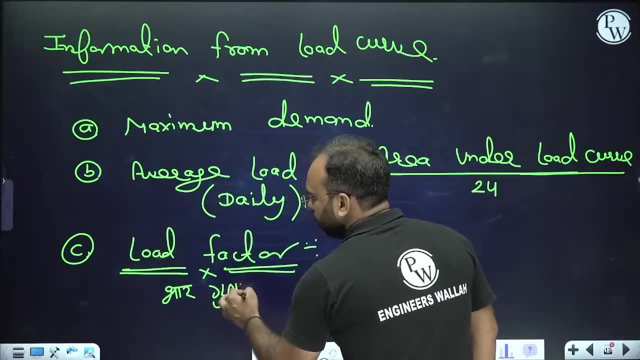 Then I will also do numerical. So the examiner will ask you tell me what is the load factor. We call load factor as Bar Gunank. What do we call it Bar Gunank? We call it Bar Gunank. Maximum demand is called in Hindi as: 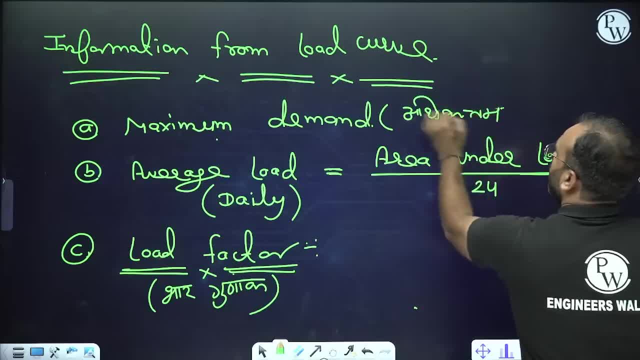 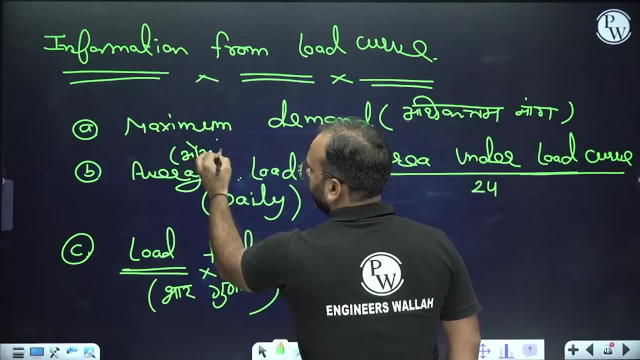 Adiktam Mang. If there is any student of Hindi medium, then here we call it Adiktam Mang And here we call it Ausad Bar. We call the average as Ausad Bar. What will be Ausad Bar? It will be the average load. 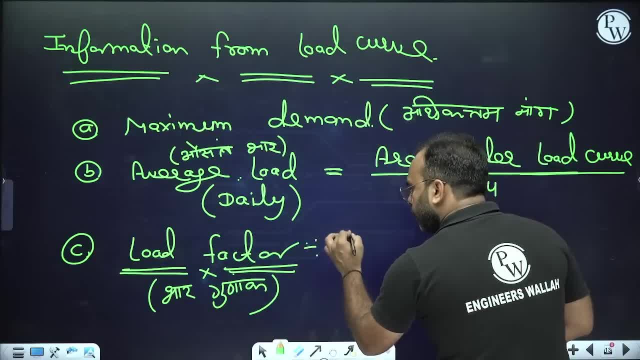 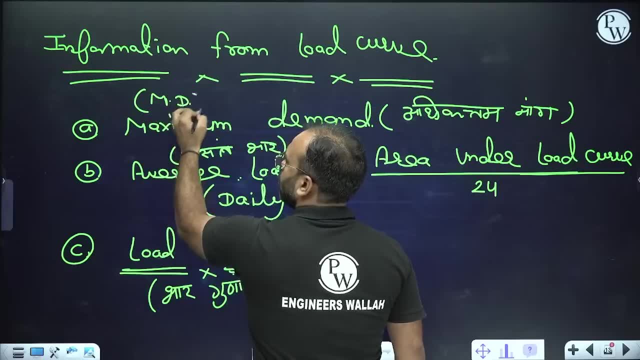 So if I ask you about the load factor, then what will be the load factor? Average Load Divided by Maximum Demand. We will write MD in short. We will write MD in short And we will write AL, which means Average Load. 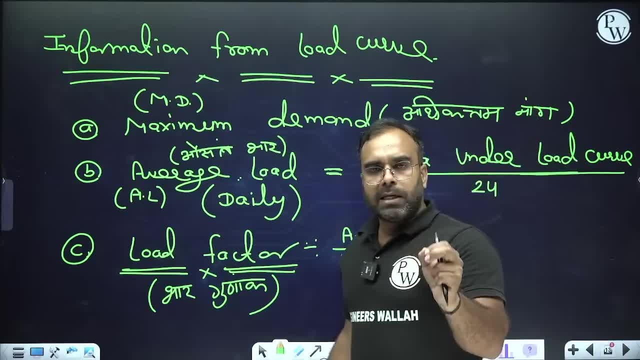 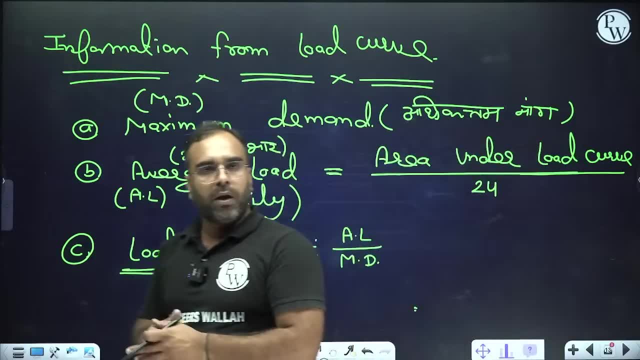 So this is the formula of our load factor. If we tell you that the load factor is always less than 1 or greater than 1. Tell me quickly: the value of load factor is less than 1 or greater than 1.. 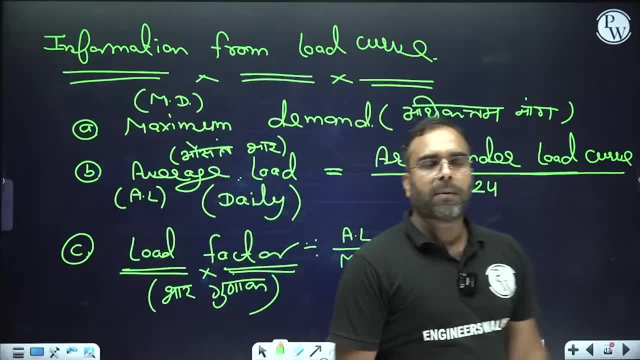 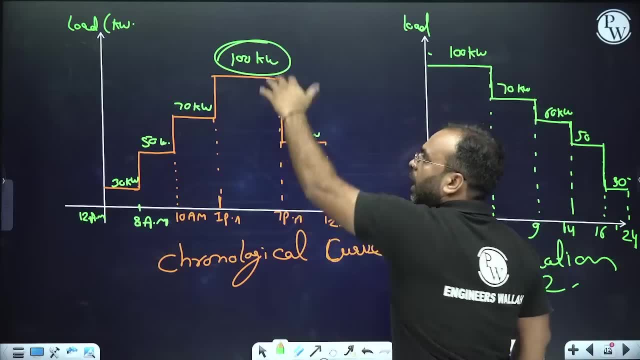 If the examiner ever asks you, then what will be your answer? By the way, you know that the maximum demand- suppose this is the curve- its maximum is 100.. What will be the average? If everyone gets it, then it will be less than that, right. 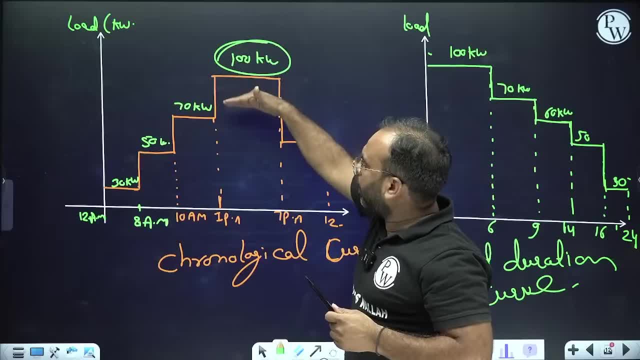 As I say, the maximum is more, the average will be less than that. If the average will be less than that, it means, what can I say from here? That if the average value is less, then the maximum will be more. 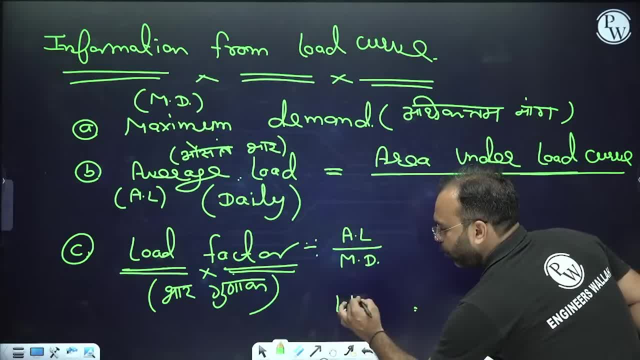 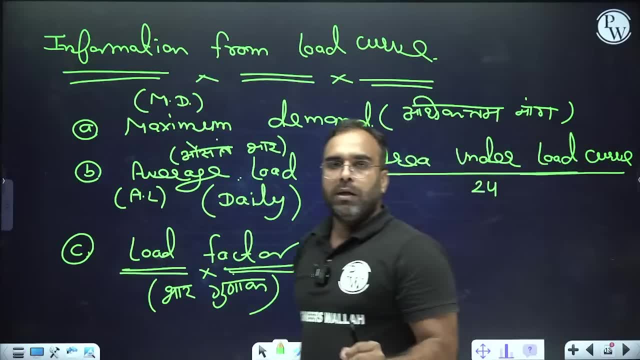 means less than 1.. So this is also an important point. Remember that the load factor is less than 1.. The value of the load factor will be less than 1. And you know that if the examiner asks you such a question. 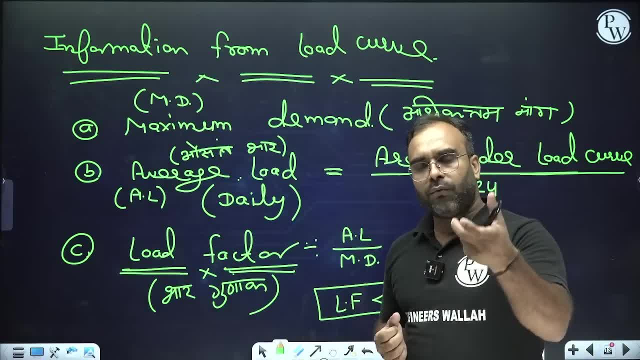 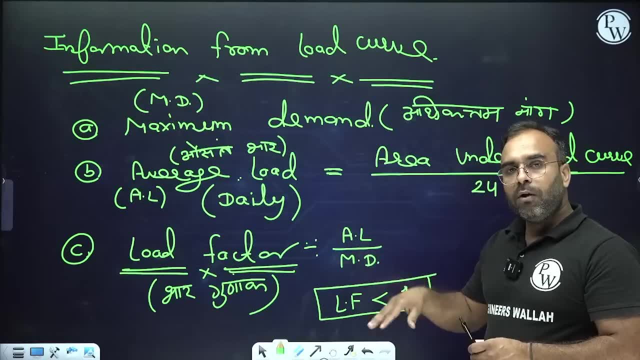 that if the load factor is more, if the load factor is near 1, then what will be the benefit? Tell me When the value of the load factor will be improved. then whose value will be decreased? Tell me quickly if the load factor will be increased. 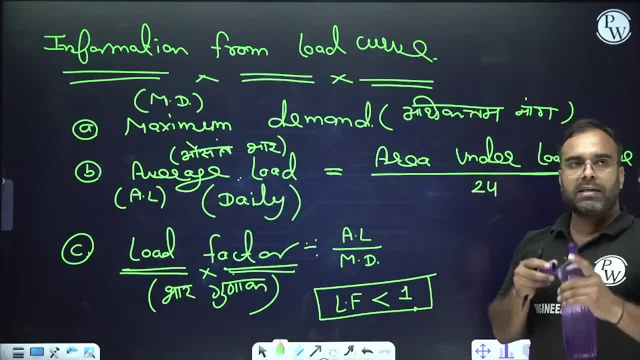 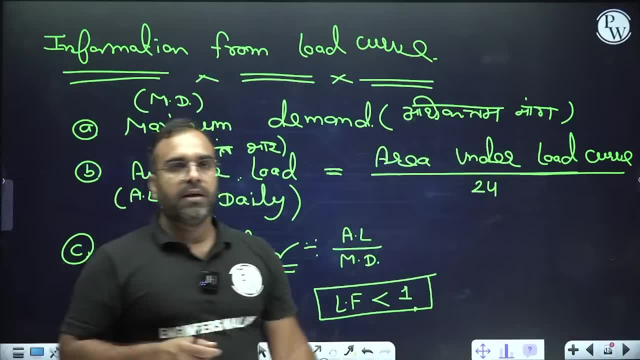 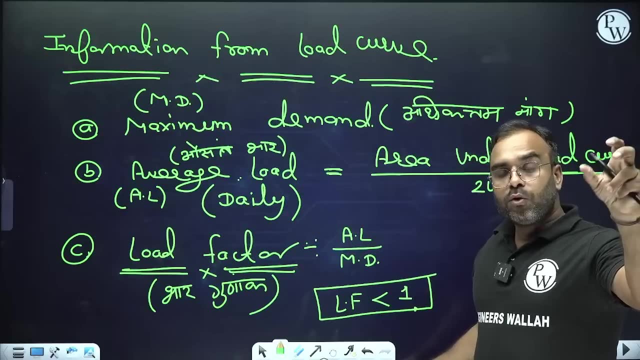 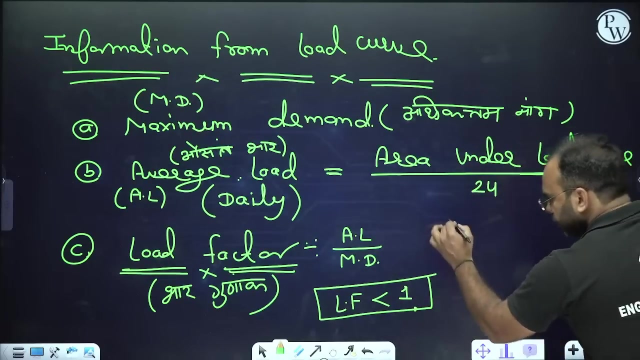 then whose value will be decreased? This question has also been asked to you in the exam. What will be the answer? Per unit generated cost? Absolutely right. If your load factor will increase, then the generation cost will be decreased. So the answer is absolutely right. 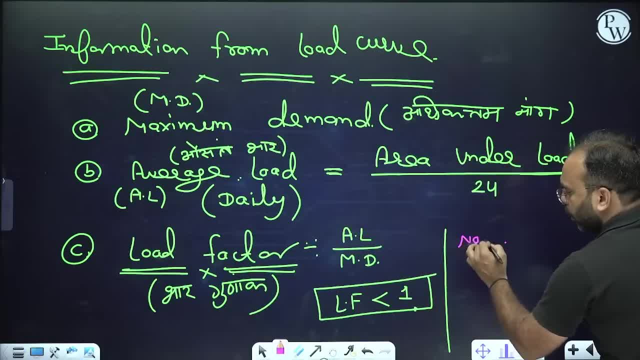 So we will write a point by writing a note here. Write a point by writing a note. Write a point by writing a note. If your load factor will be increased, then per unit generated cost, per unit generated cost, what will be with us? 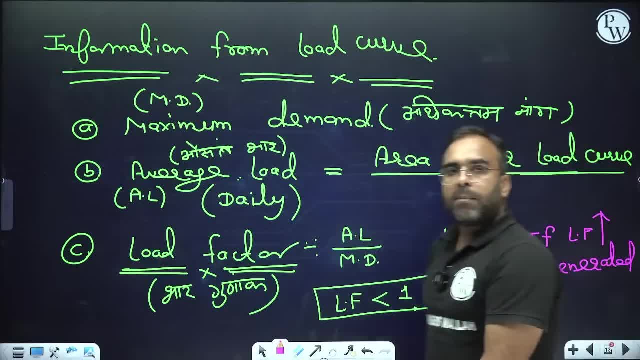 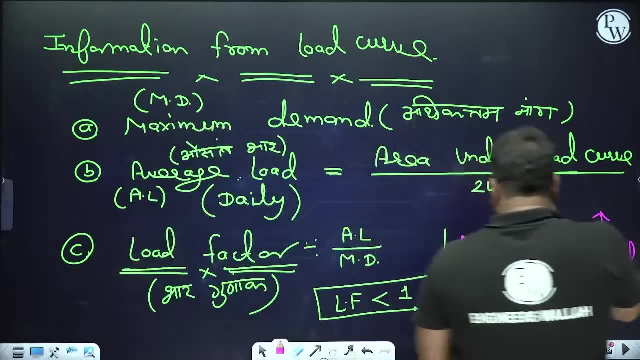 The generated cost will be decreased, Right, So you will ask this question in the exam. This will be given in the option You can answer from there. Next: Now we have this load factor. Next, the examiner will ask us a question. 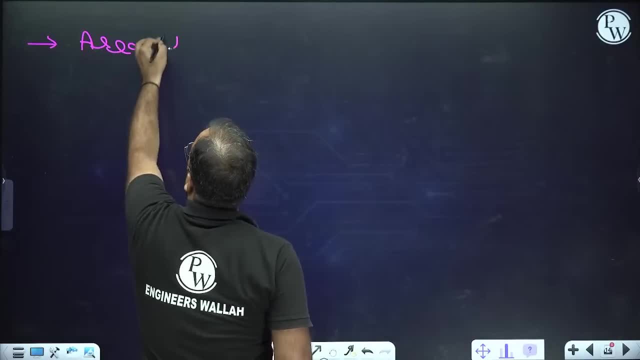 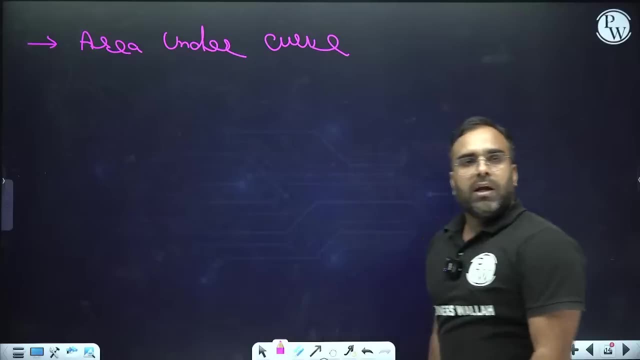 Tell me what do we get in the area under load curve, Area under load curve, Load curve. So load curve means the area of the load factor. what do we get? Tell me quickly What will we get in the area under load curve. 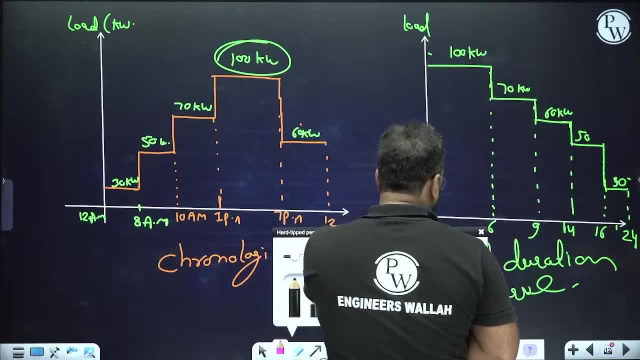 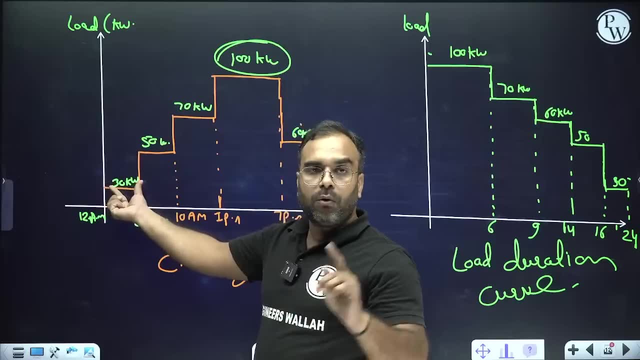 See, we have to find its area. Everyone knows that. if you want to find its area, then what to do here? What will you do for its area here? Height divided by base: See what is there. on the height, There is power. 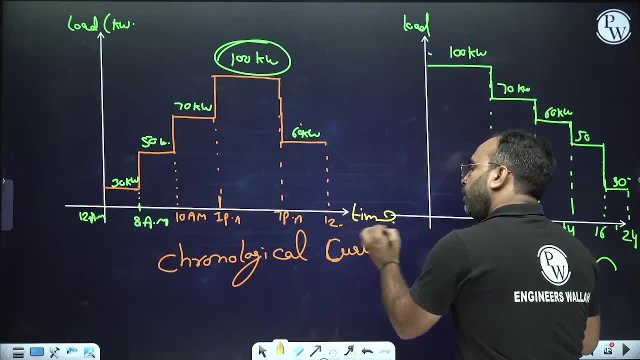 What is there on the base? There is time. What is there on the base here? There is time. So there is time in the hours. So, from here to here, how many hours are there? From 12 to 8 o'clock. 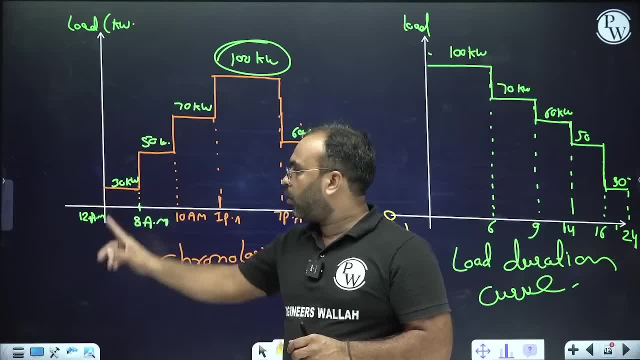 it is 8 hours. So here, if you multiply 30 with 8, then when you multiply kilowatt with hour, then how much will it be? Kilowatt hour will come, And that kilowatt hour is the energy. 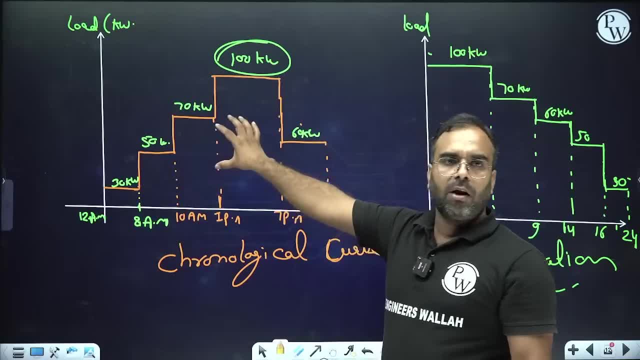 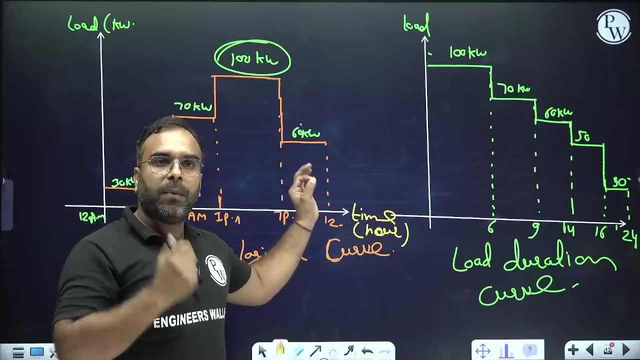 This means that the area under load curve that you will get here, or area under load curve or chronological curve- you can say anything- that you will get energy consumed here. How much energy is your load consuming? So keep in mind. 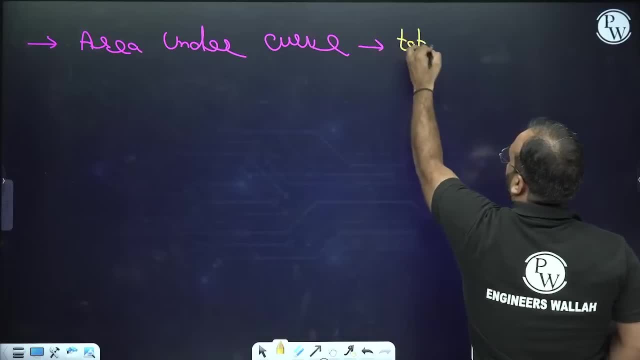 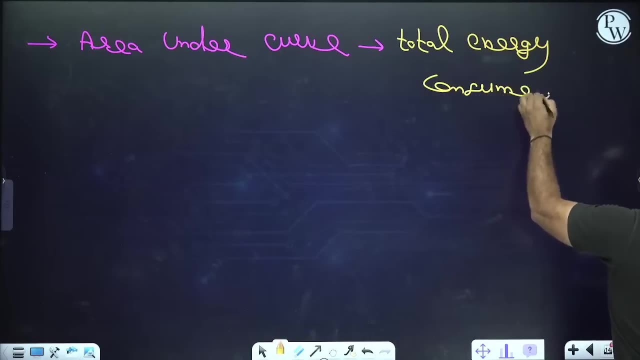 what will you get in the area under load curve? That will be total energy consumed. Total energy consumed that we will get area under load curve. So this is an important point we have Next after this, if the examiner asks you such a question, 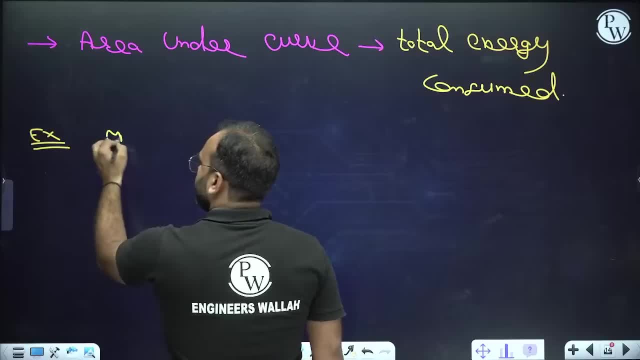 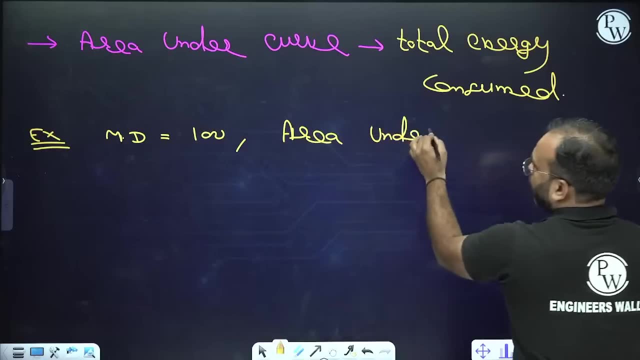 keep in mind- the examiner will ask you such a question- that the maximum demand is 100. And the area under load curve, the area under load curve, the area under load curve, how much is that? we have, That is, 80 megawatt. 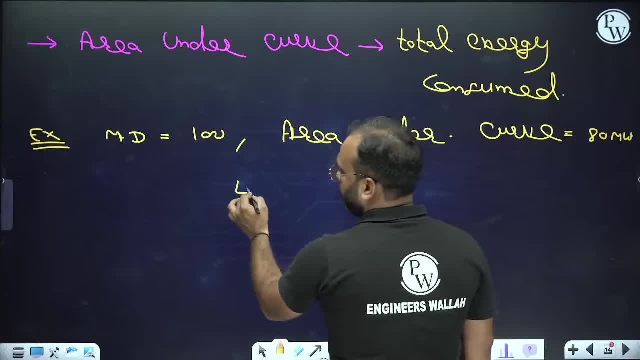 80 megawatt. So he will ask you: tell me what will be the load factor. Tell me quickly what will be the load factor if the examiner asks you such a question, And he will say area under: 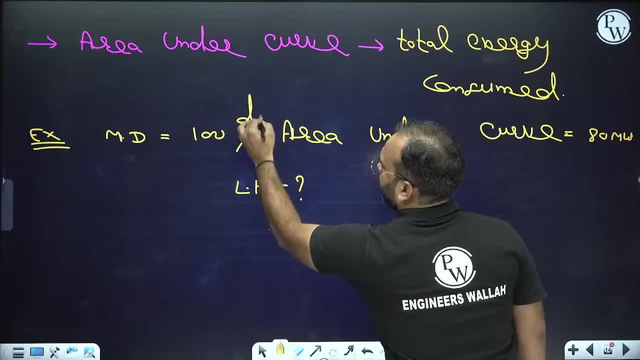 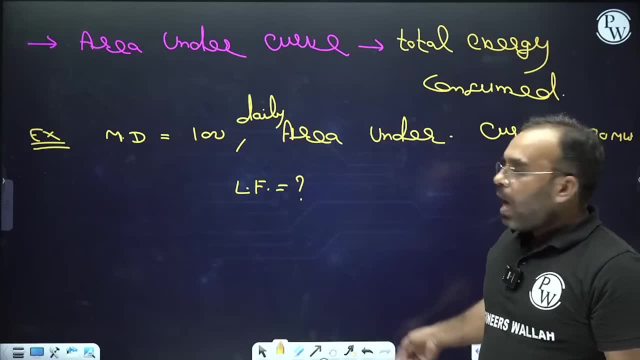 what will it be? Daily, I am talking about the daily area. Daily, I am not talking about yearly. He will ask you: tell me what will be the load factor. What will be the answer? The examiner will ask you: 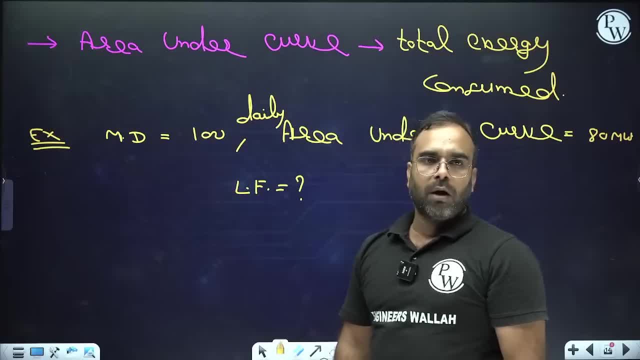 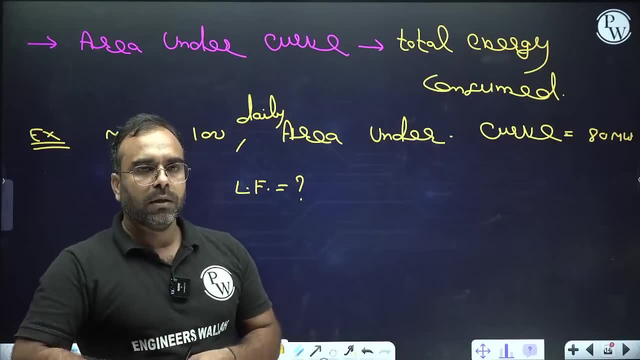 he will say: the maximum demand you have is 100.. Daily, the area under load curve is 80.. Tell me what will be the load factor. What will be the answer? What will be the load factor? Point it Ok. 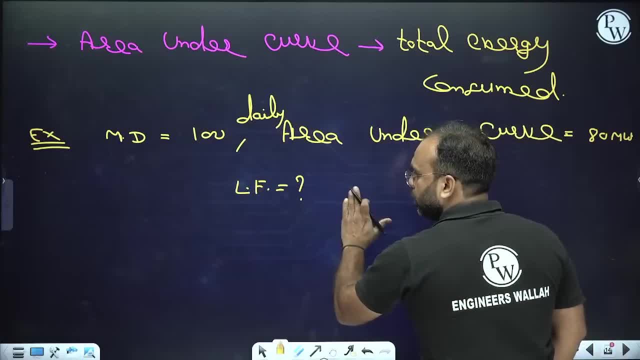 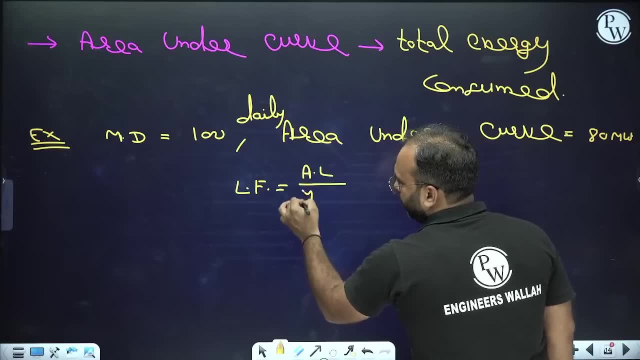 So understand here what I said. the average load, the load factor that you have, we have average divide by maximum demand. Keep in mind average load divide by maximum demand. So we have answered this point, it Ok? 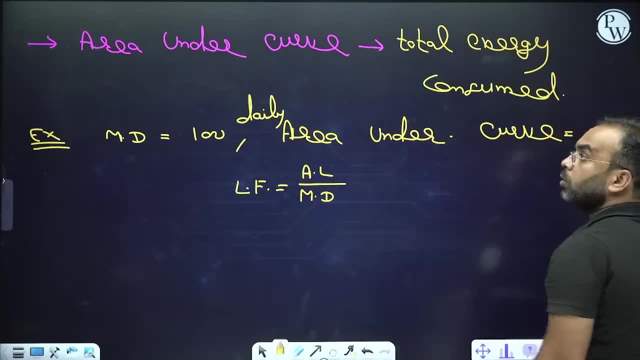 Now understand what is the daily area under load curve. Is it the average load? Keep in mind: the area under load curve is the energy. What did I say? Understand the language of the question. Don't make mistakes in haste. I have given you the area under the curve. 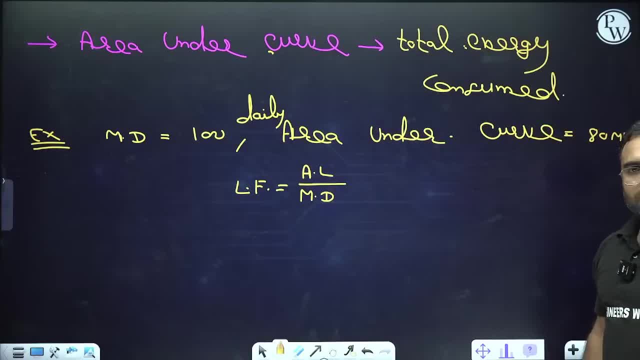 So I have given you the daily area under the curve, which is 80.. Have I given you the average? No, I haven't given you the average. You will have to subtract the average. So how can you say it will be 0.8?? 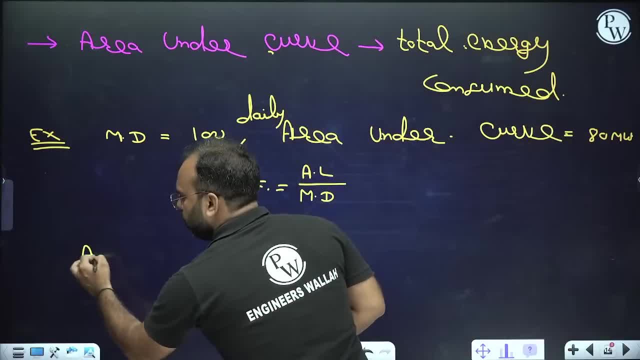 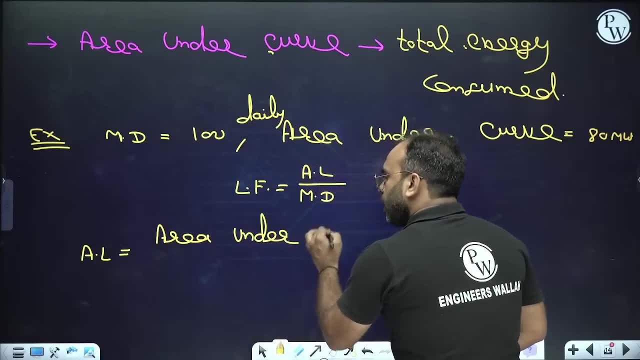 Here you will have to subtract the average load first, And this is what I want to say, that the average load that we have, area under area under daily load curve, daily load curve, area under daily load curve, divide by 24,. 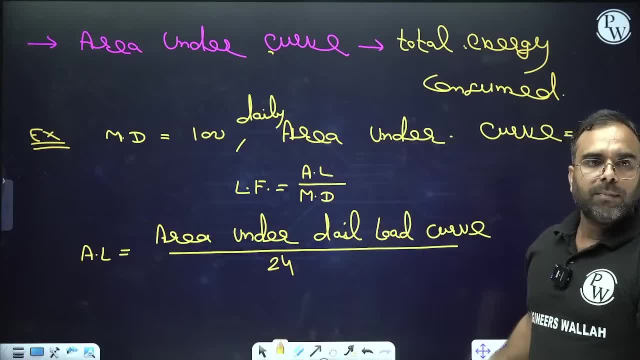 you will have to do it first, Are you understanding? First you will have to do 24.. Yes, this kilowatt hour will come. This kilowatt will not come. This megawatt hour will come. Make it 100 megawatt hour. 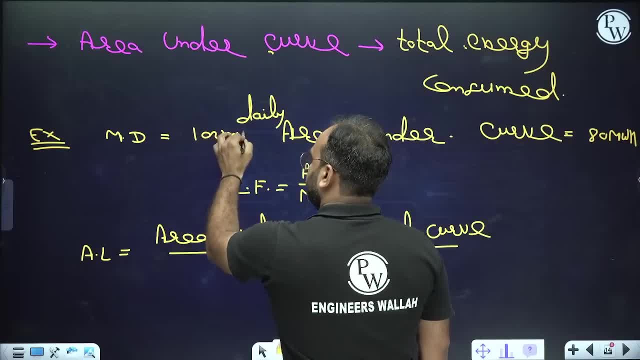 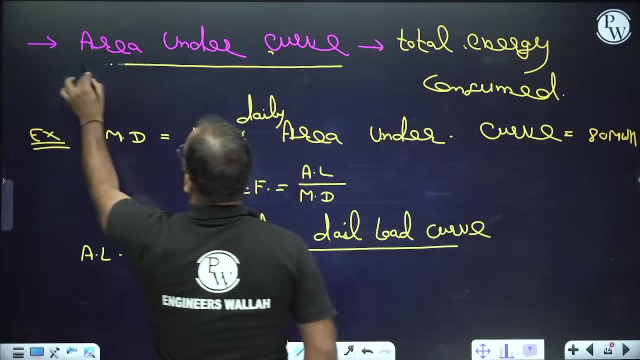 Megawatt will not come, And this is the answer in megawatt. Make it in megawatt, Make it in megawatt hour, Because I will get that energy. So remember the area under load curve. you don't get the average. 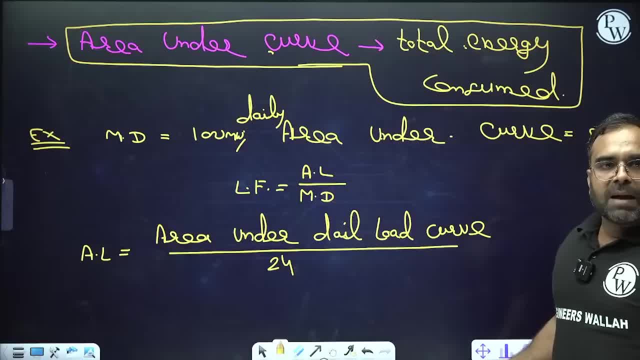 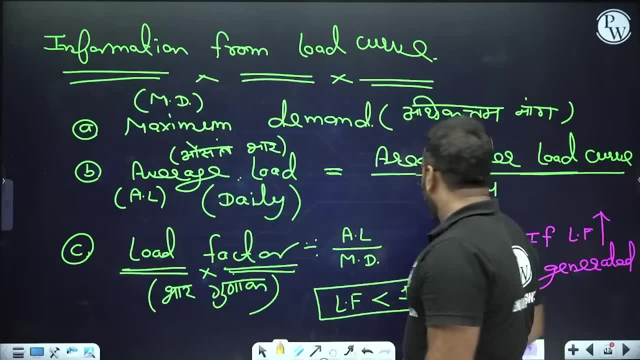 you get the energy. So first you have to subtract from there. Let me explain again. understand: I said: when we subtract the area, then the area we will get, the area we will get here according to this see. 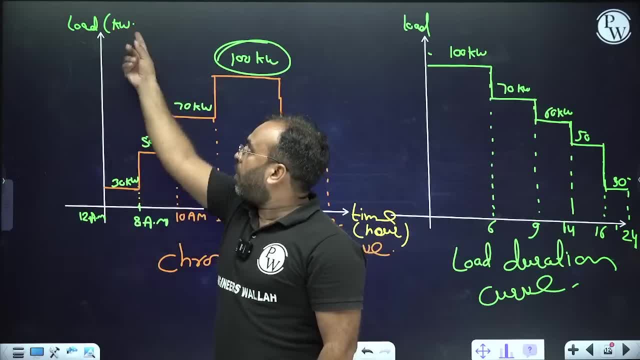 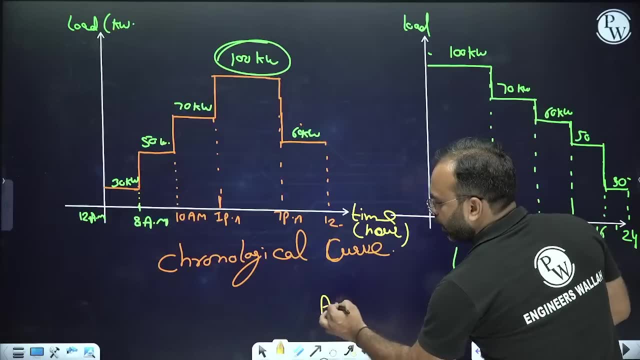 power is on the y-axis and time is on the x-axis, So power into time, that energy will come, that area has come, But we have to subtract the average. So what is the average? The average is we have area divided by time period. 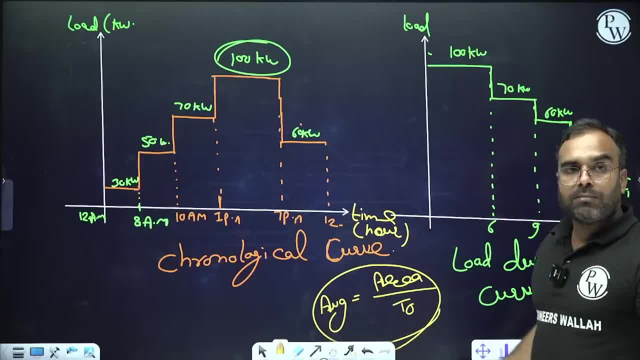 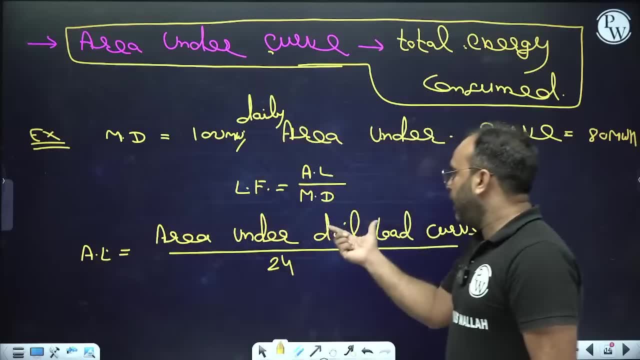 So in the area you have to divide the time period, then the average will come. So that means that means what you have to do is first of all you have to subtract the average load, that area divided by 24.. 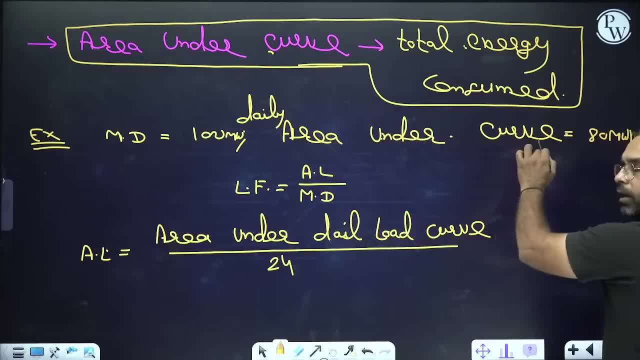 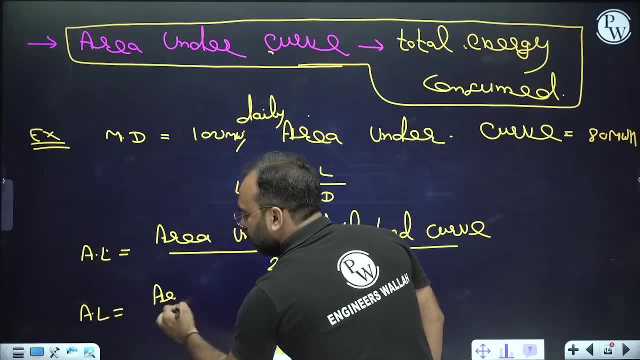 But remember I have given you daily. area under curve. If it will give you monthly, if here, remember, if it would have given monthly, then how would you subtract the average Area? remember all these formulas here: area under monthly load curve. 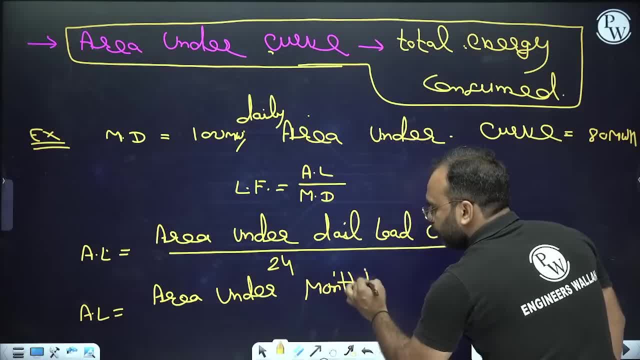 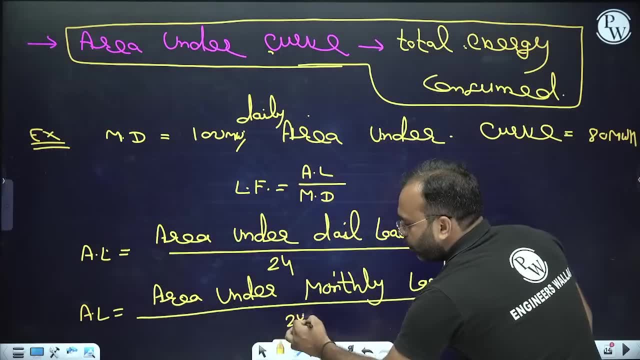 area under monthly load curve. monthly load curve. So you will subtract the area of monthly load curve, What will you divide by So 24, into you. tell me how many days are there in the month. So there are 30 days. 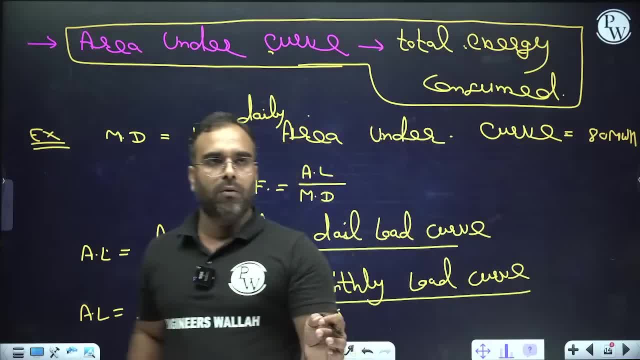 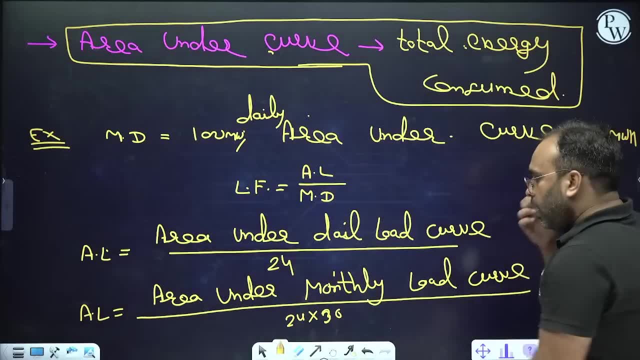 So you will multiply by 30. That means you divide by 720.. If you divide by 720, then the average will come from there. Okay, you have to do 720. But suppose here I can give you anything in the question. 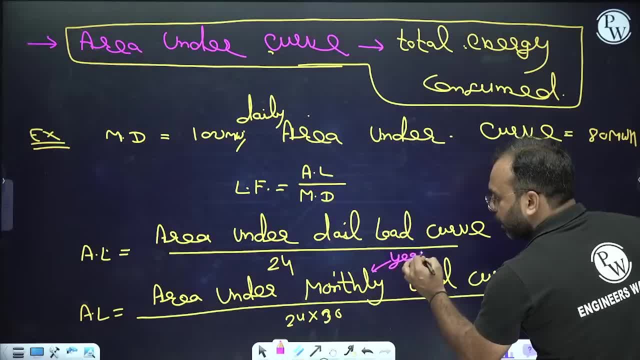 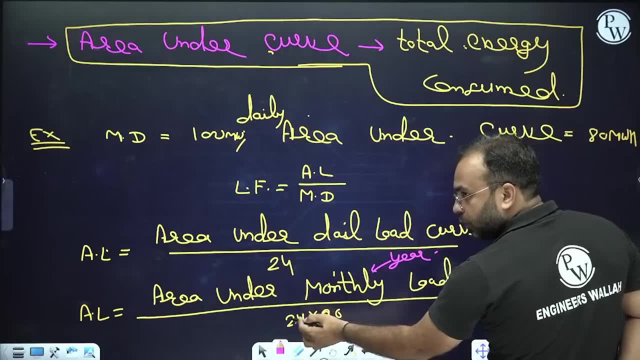 See here, instead of monthly, if it will give yearly. if it will give yearly, then you have to multiply it by 365.. So better than that, you have 365 days here, multiply it by 24.. So 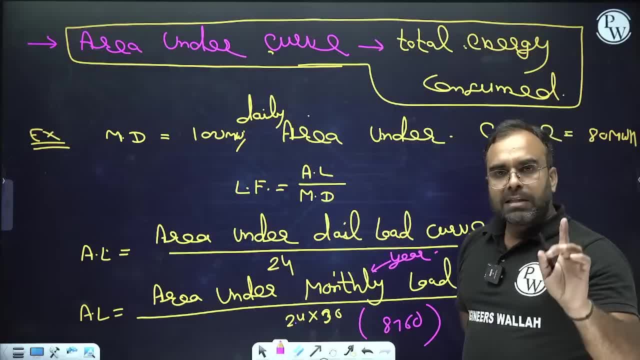 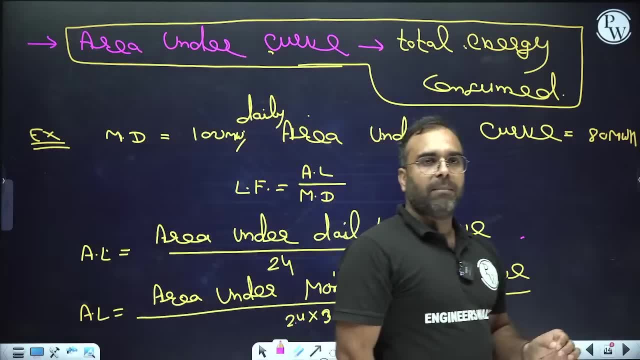 then you have to divide by 8760 here. So take care in the exam, Don't make a mistake in the hurry. You will get such numericals. They come every time. You get them in the exam every time. But 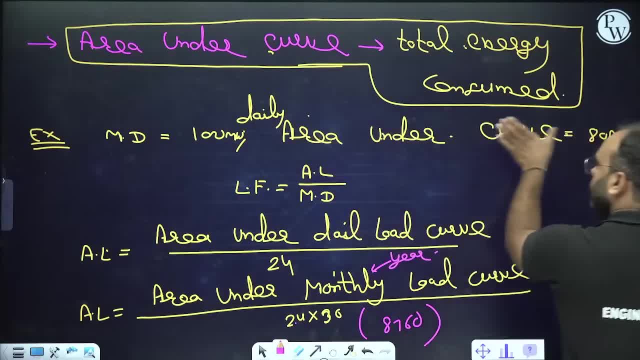 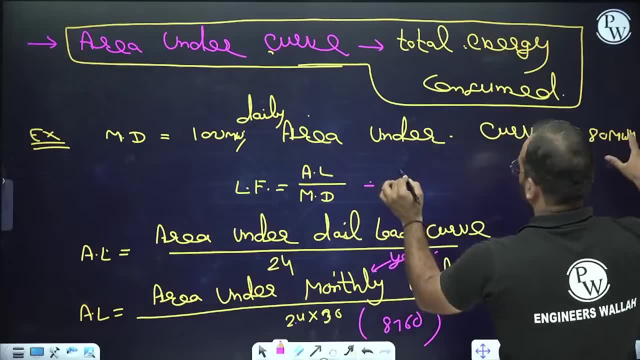 you make a mistake in the hurry. So whenever you are given an area, then what will you do? first You will take out the average. So, to take out the average, what will you do here? I have given you 80.. 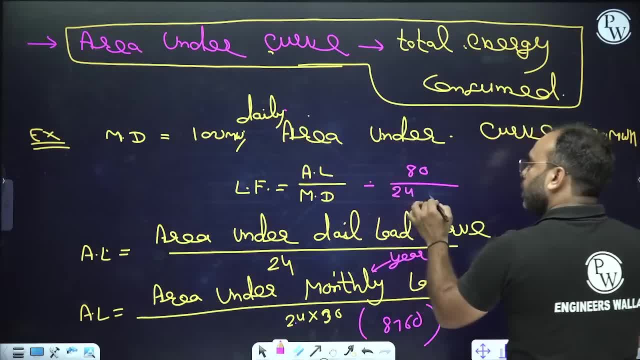 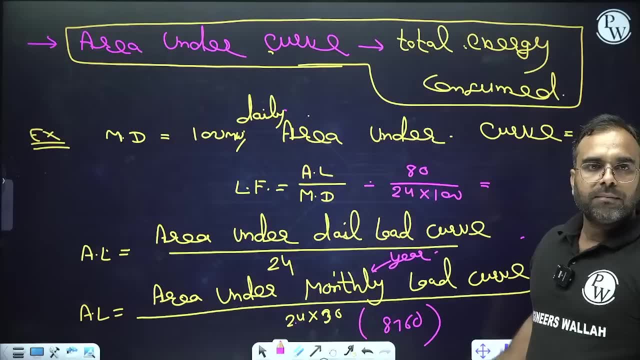 So you will divide by 24. Because I gave you daily And what will be the maximum demand. So that is 100.. So that is 100.. Now you can take it out from here, Understood. 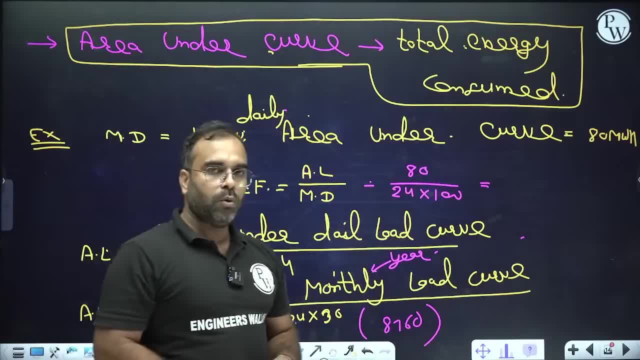 Son, there is a question in the pre. There is a question in the pre. I am not talking about the mens. There will be a better level of question in the mens In the pre. you will get to see such numericals in CBT-1,. 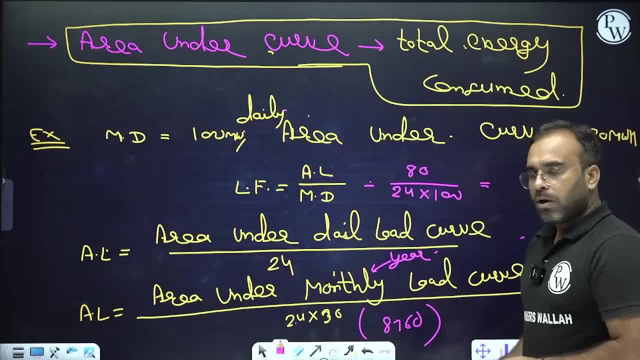 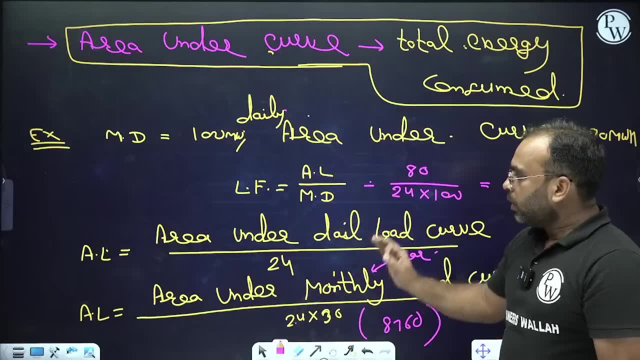 which you must have given the exam before this, which someone must know, Or you must have applied PYQ. So you must have seen such questions. Now I will make you practice, But finally just tell me that. did you understand this thing? 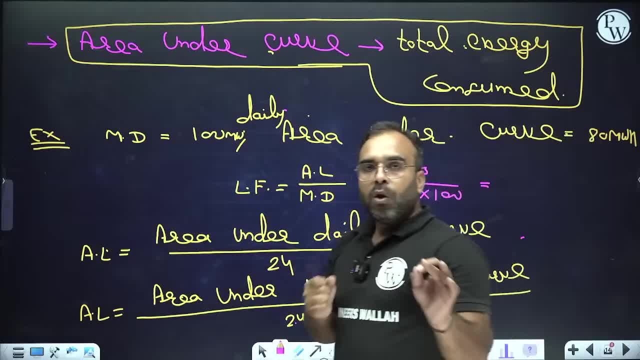 If you have to take out the average or if you have to take out the load factor, how will you take it out? If you have to take out the load factor, then you will do average divide by maximum demand. But 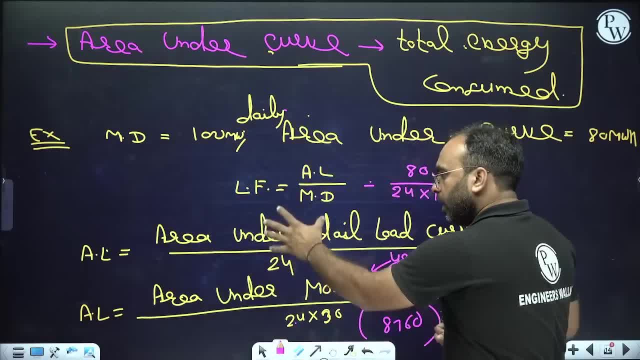 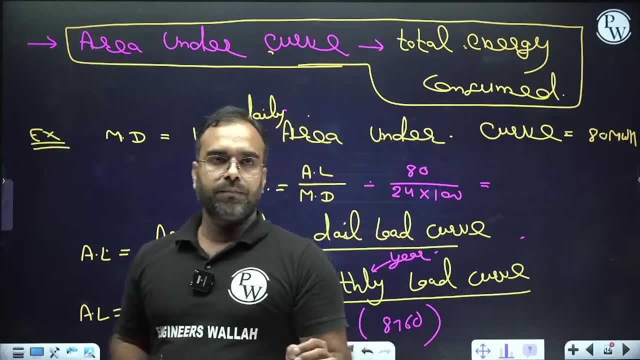 just don't make a mistake here. To take out the average, first you have to go through these formulas, But when, When, I will be given the area under load curve, Then Clear. So you must have understood this thing. 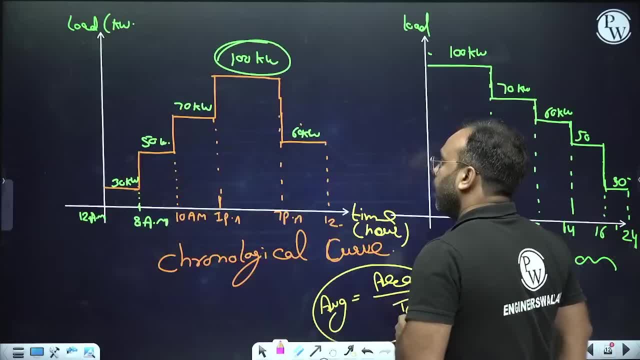 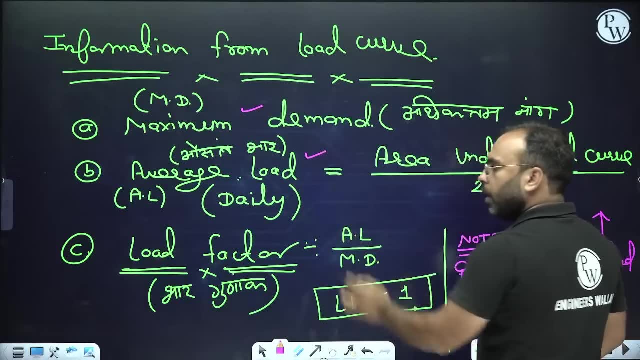 So that means the load curve I have made here. So what information did I get from the load curve? Tell me, I have got the information from the load curve. I have got the maximum demand. I have got the average load. 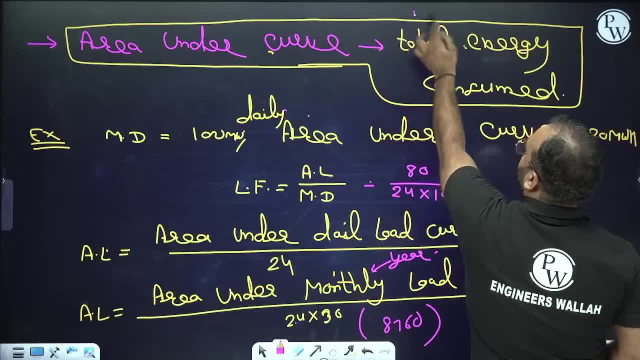 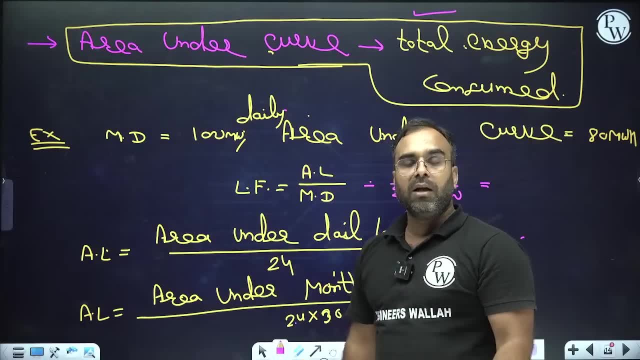 I have got the load factor Here. how much energy am I consuming? How much energy am I consuming? We have got that. That means who gets so much information From the load curve? That is why you must know that the load curve is made on our substation. 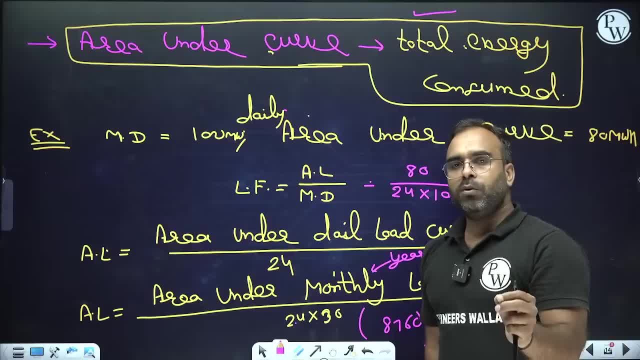 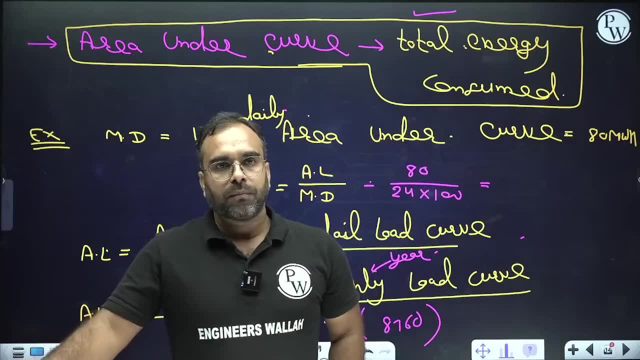 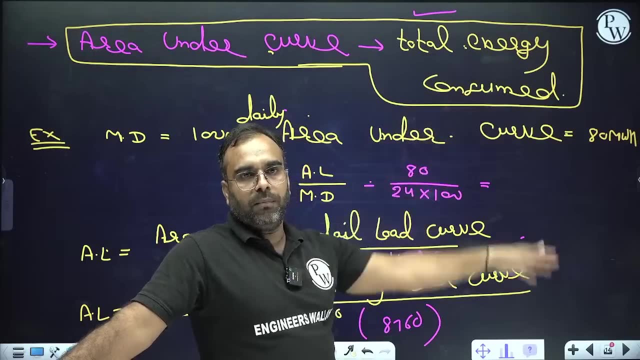 And to make that load curve we use an equipment. You will tell me by commenting the name of it Which is the equipment that we use. Tell me quickly Which equipment is used to draw this curve on the substation. I have given the name of that equipment. 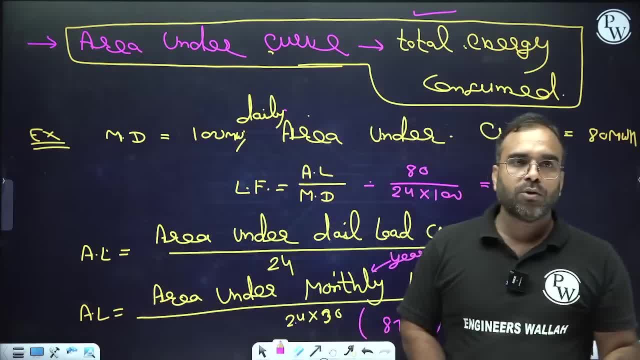 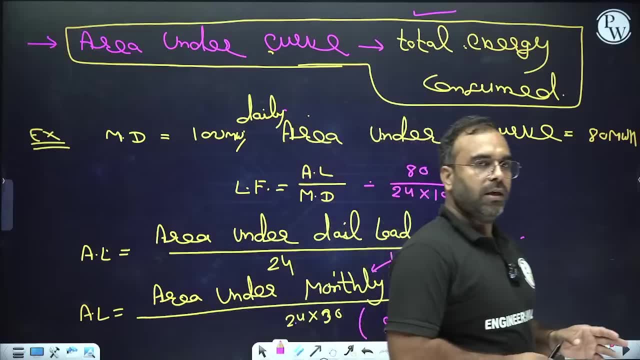 in the measurement. If you have studied in the measurement then you must have seen the name of that equipment. Which equipment they use: CRO. CRO is not used. CRO is not used. SCADA PLC. SCADA XY plotter. 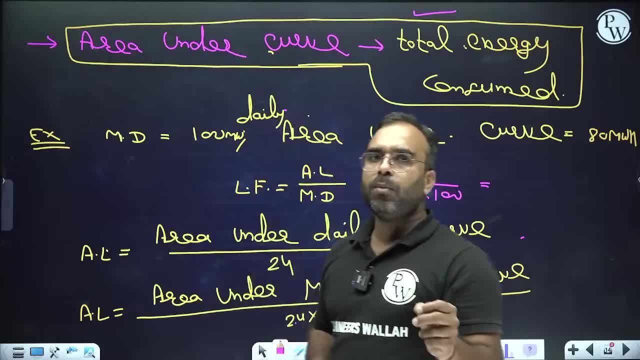 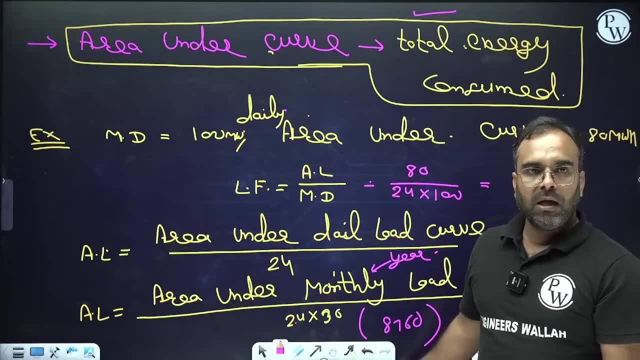 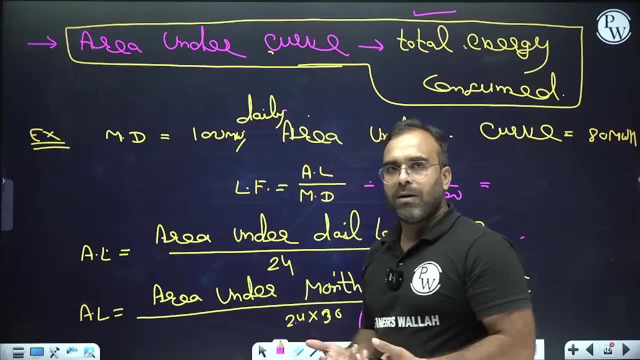 Someone has given the correct answer, sir: XY plotter or potentiometric recorder. Remember, XY plotter or potentiometric recorder we use. Correct answer is XY plotter or potentiometric recorder is the correct answer. is the correct answer. In CRO we can see how it is made, but to plot it we use XY plotter. 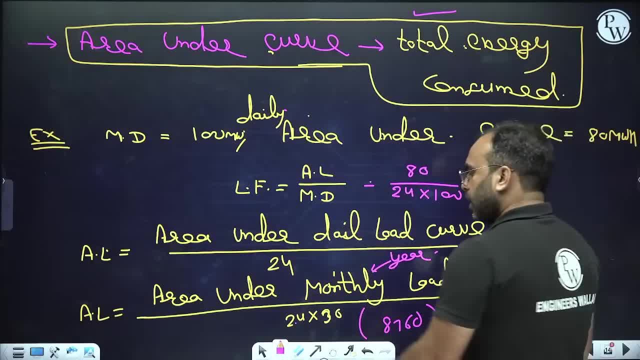 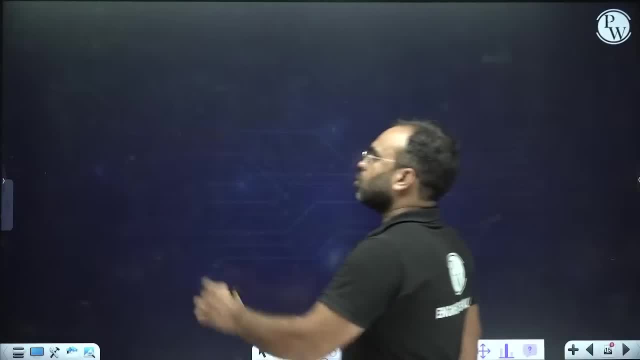 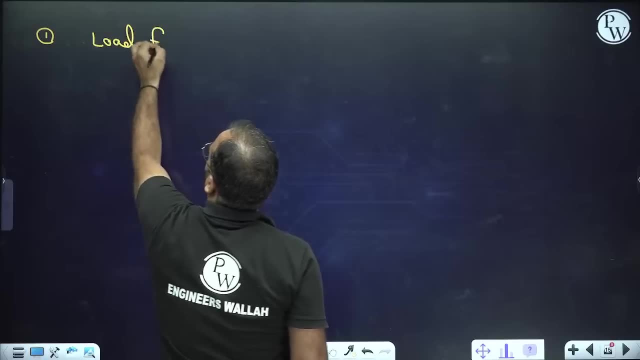 or potentiometric recorder. So keep this in mind. So even this examiner can ask you: Let's go next. So we have got one formula from here, So let's summarize it. Summarize is that you should know that the load factor, the load factor, means the formula of the load. 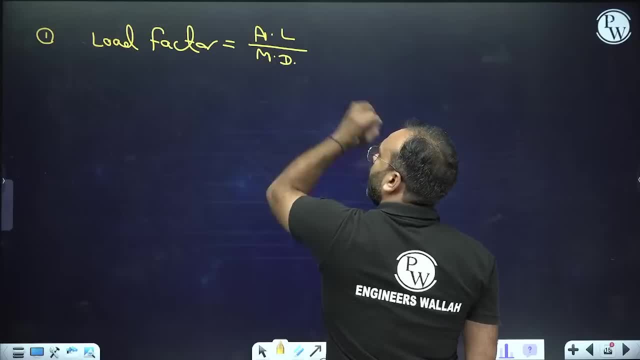 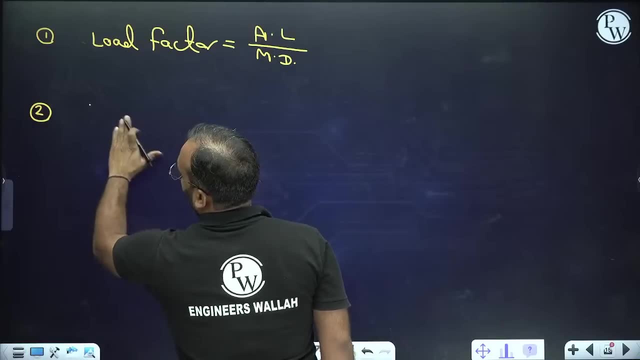 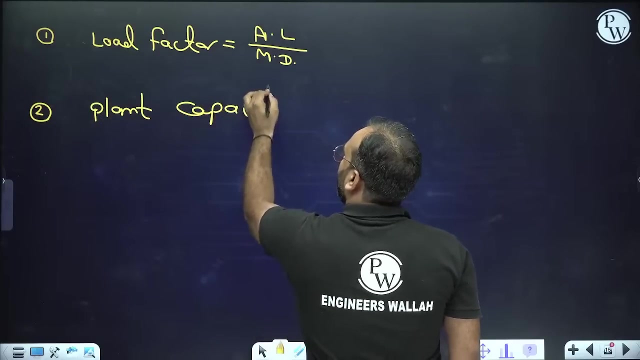 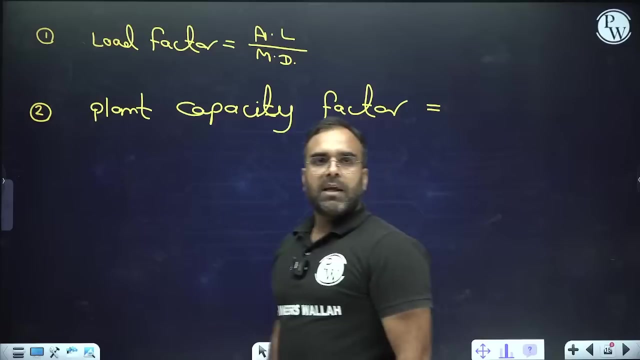 is average load divided by maximum demand. Next, if we talk about the second formula, then you will be asked about the plant capacity factor. Come on, tell me quickly What is the plant capacity factor. We will tell you quickly What is the plant capacity factor. 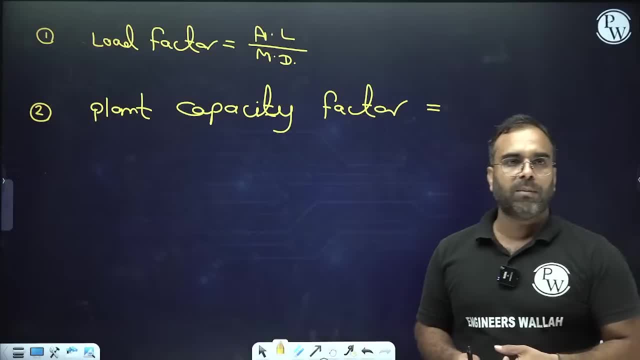 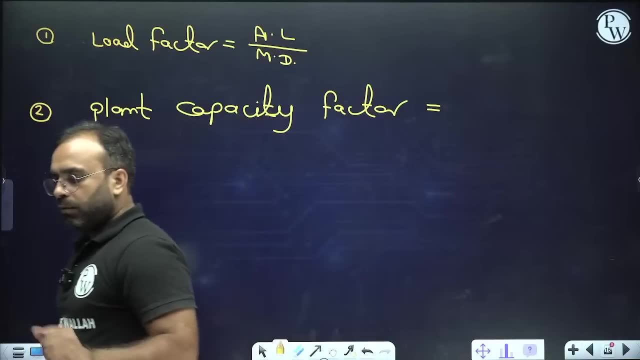 What is the plant capacity factor? If you have one formula, then you should know that the examiner will tell you. Come on, those who don't know, they don't say No problem, Those who know, tell me quickly What is the plant capacity factor. If the examiner 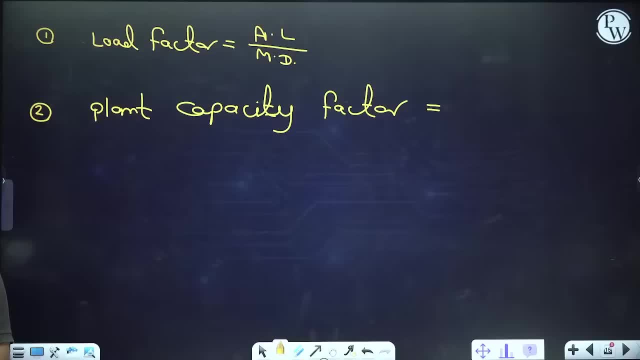 asks you about the plant capacity factor, then what will be the answer? What will be the answer? Average load divided by rated plant capacity is the correct answer. When will be the measurement? After that, your basic electronics will be done and Krishna sir will take the basic electronics in a very good way. After that, the last subject of 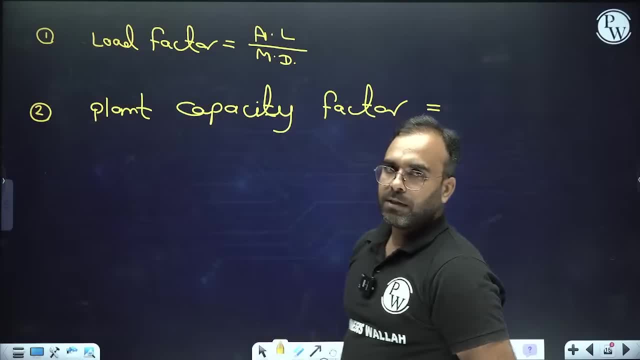 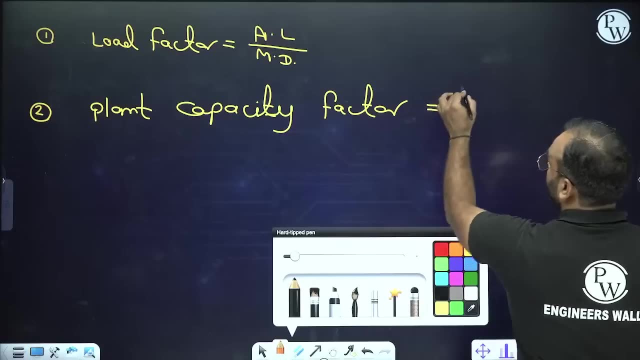 this crash course, the ending, which we will do, will be done by the measurement only. So measurement will be the last subject. After that we will do basic electronics. That is, After this, basic electronics will be done. so what will be the plant capacity factor here? 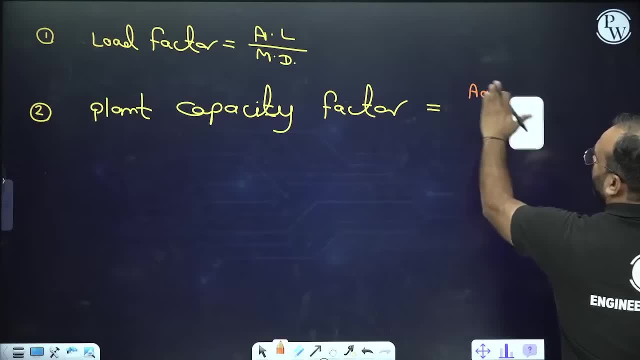 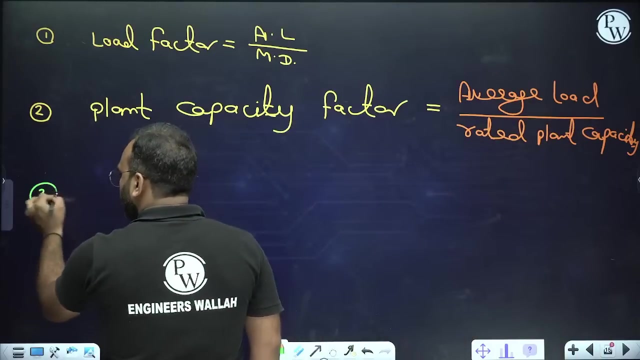 So we have the average load divided by rated plant capacity, which will be our formula: Rated plant capacity. so divide plant capacity by that plant capacity factor. But third, here comes the utilization factor. Utilization factor. quickly tell me what is utilization factor? 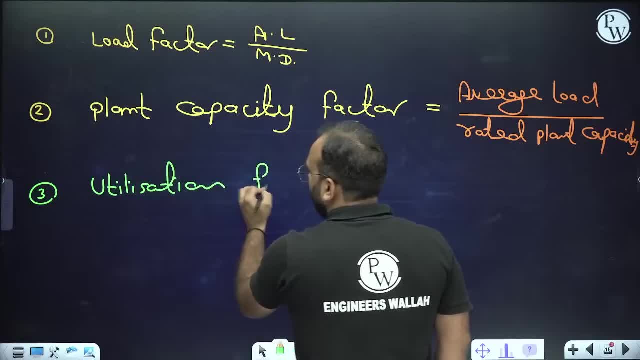 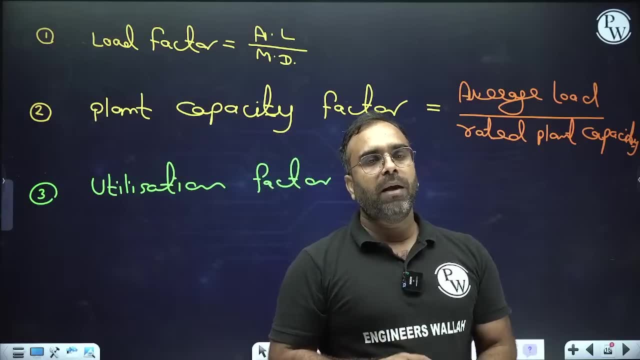 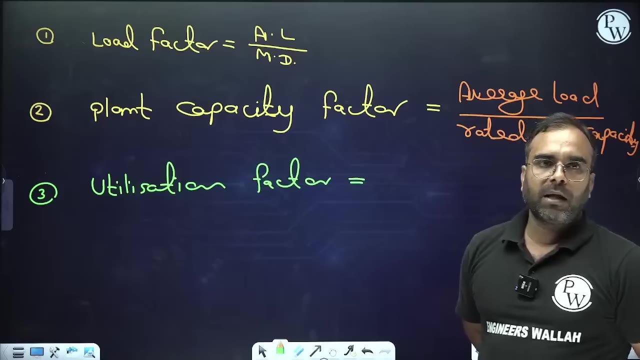 What is utilization factor? If we ask you examiner, then what will be the answer? Then we will make a relation between these three from here, because examiner also ask relation from here. Average by rated plant capacity is correct answer. Instead of this average you can also do unit generated by time. 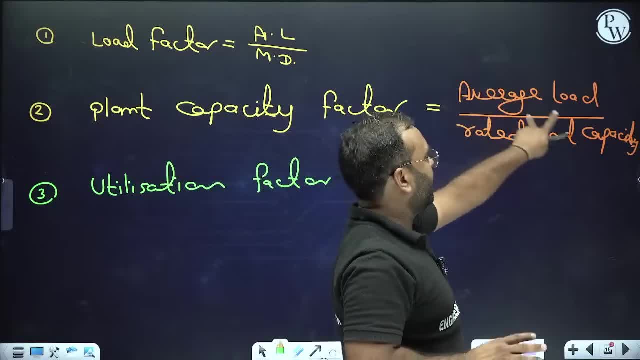 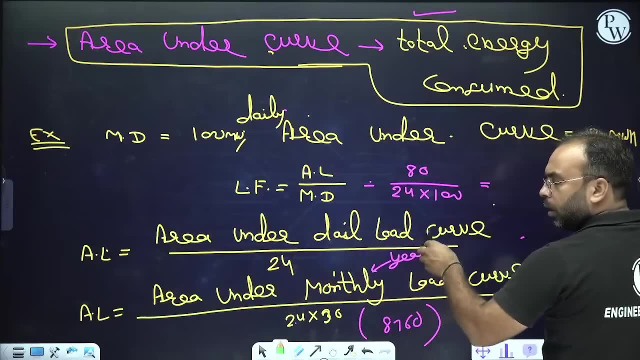 Remember many times, examiner will not give average by rated plant capacity. Now I told you that if you want to find the average, then you will find the average by under loading the area which we call unit generated. This is called unit generated or unit consumed. 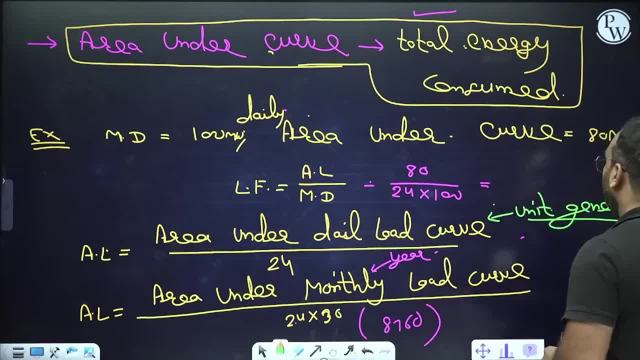 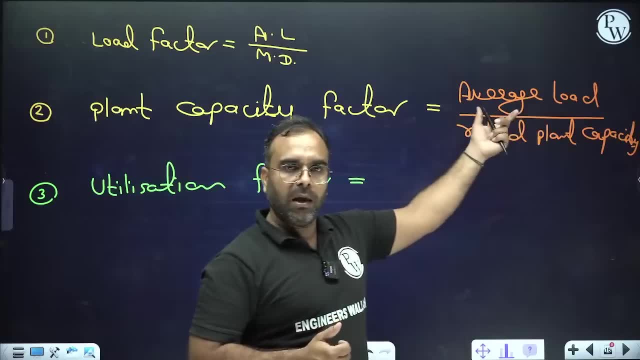 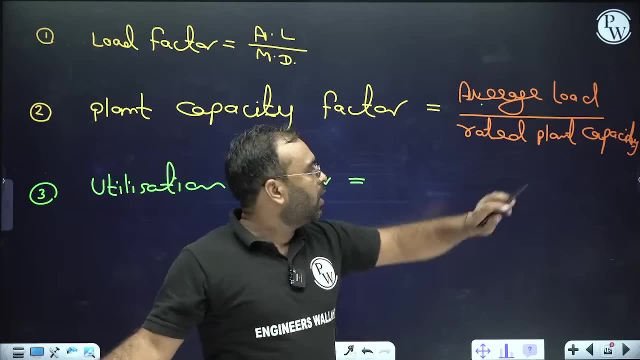 So it can also divide unit generated by time period. so what will it do in this formula? Instead of average, it will write unit generated divided by rated plant capacity into time. whose formula is this? Such questions are also made in exams. So here, instead of average, I told you to under load the area divide by plant capacity into time and ask: whose formula is this? 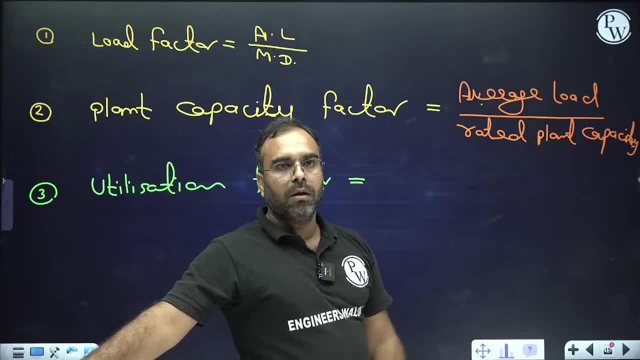 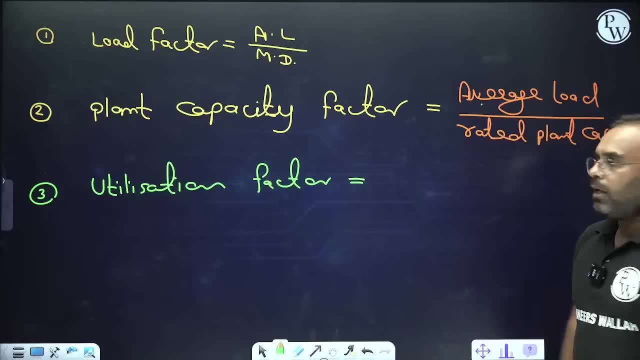 You should know. So what is utilization factor, Maximum demand divided by plant capacity? The correct answer is that we have the utilization factor Maximum demand. Maximum demand divided by What will be divided by Plant capacity. Plant capacity: The same rated plant capacity. 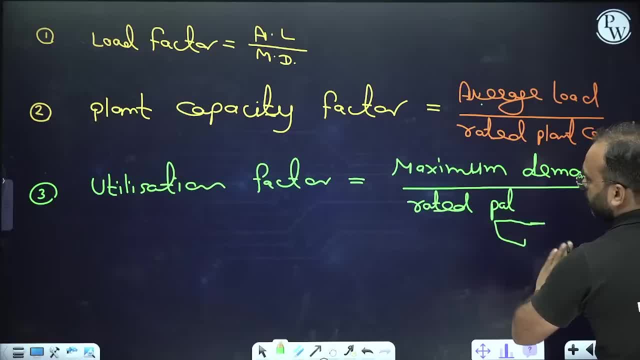 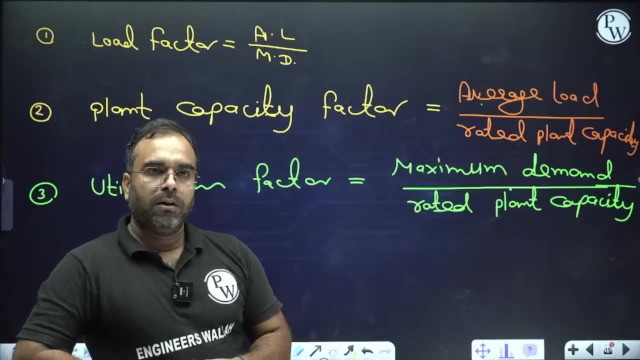 Write that here: Rated plant capacity. So what will be here? This will be plant capacity. Now see from here. can you see any relation between these three? Tell me quickly. Can you see any relation between all of them? Thank you so much, dear. 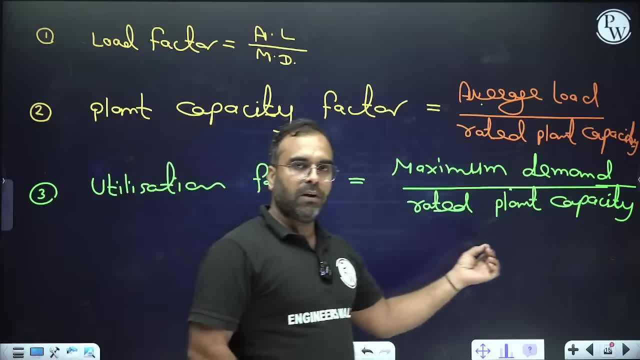 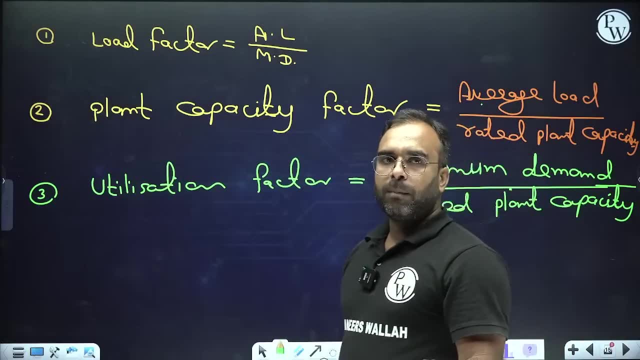 Any trick for formula, I will write you a page in the format of a table, All formulas in the last, All formulas in the last. So you put it behind the keyboard or wherever you put your mobile wallpaper anywhere, Because it has no trick. 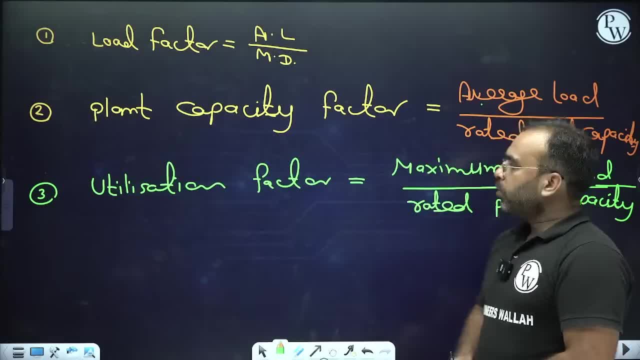 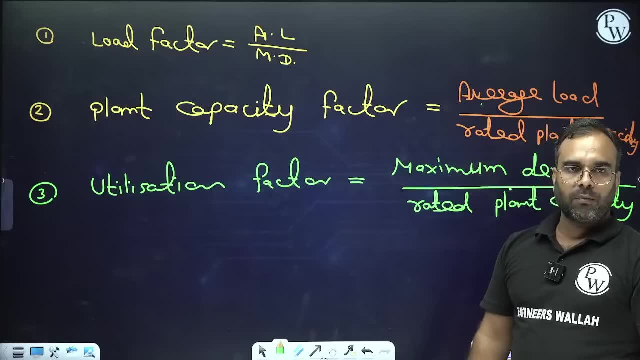 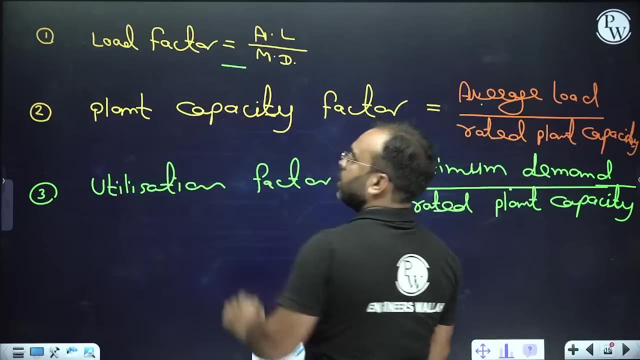 Actually you will have to remember. So see, do one thing from here. See here: If you divide the utilization factor in the plant capacity factor, If you divide the utilization factor in the capacity factor, then tell me what will come. Load factor will come. 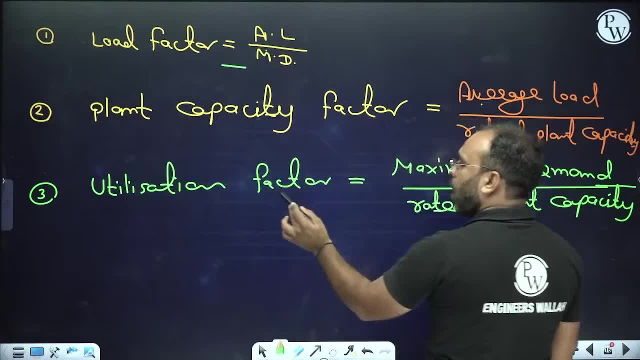 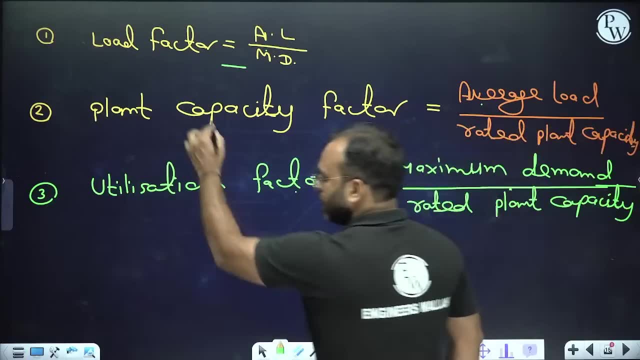 Or you can also do this: If you multiply the load factor with the utilization factor, then you will get the plant capacity factor, Whatever you remember. So this means that I am getting a relation from here: Utilization factor, and what will you do here? 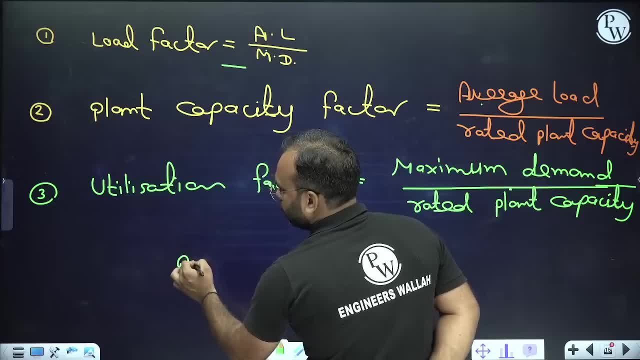 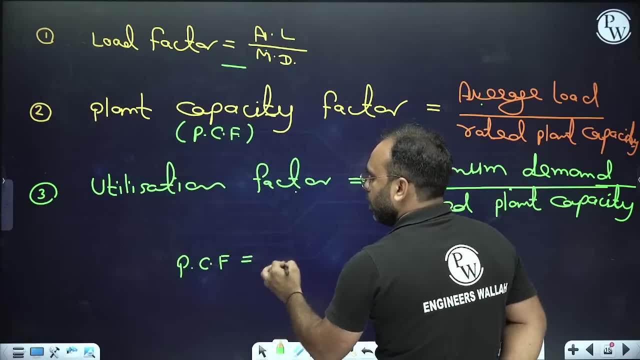 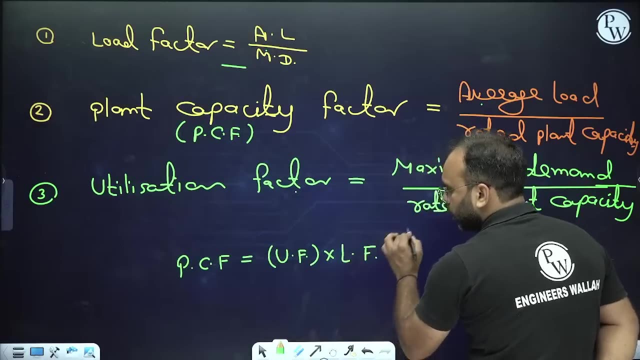 Load factor, So that will come plant capacity factor. So here you write plant capacity factor, in short as PCF. Plant capacity factor will be utilization factor into load factor And utilization factor will be the load factor. So see, the examiner will ask you such a question. 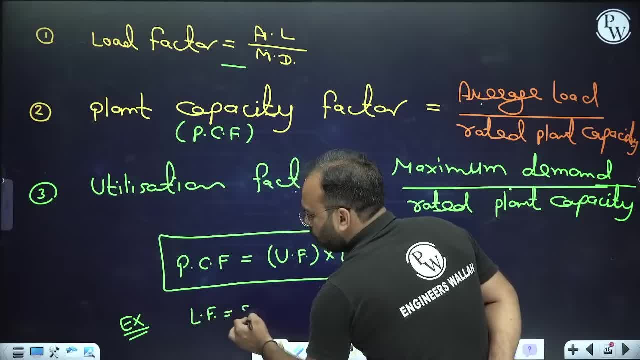 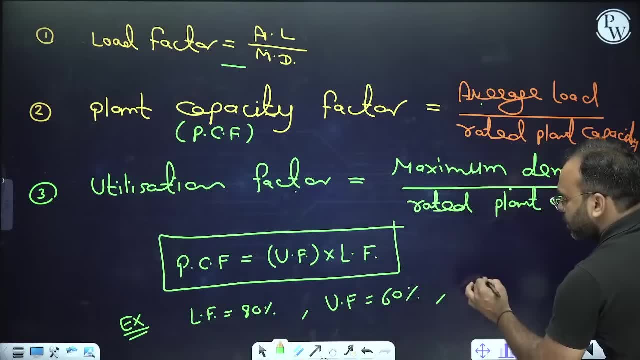 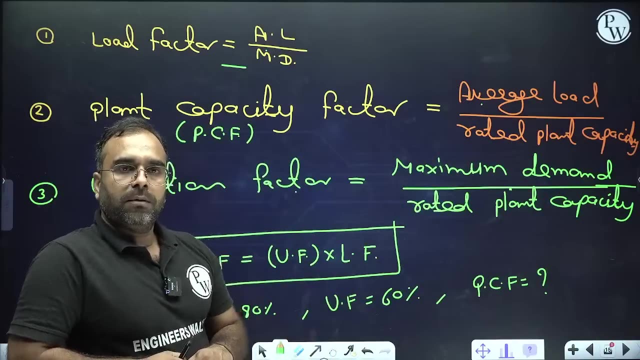 The examiner will ask you this question: The load factor is 80% And the utilization factor is 60%. Tell me what will be the plant capacity factor. Such a numerical examiner will ask you What will be the answer. Come on, tell me quickly. 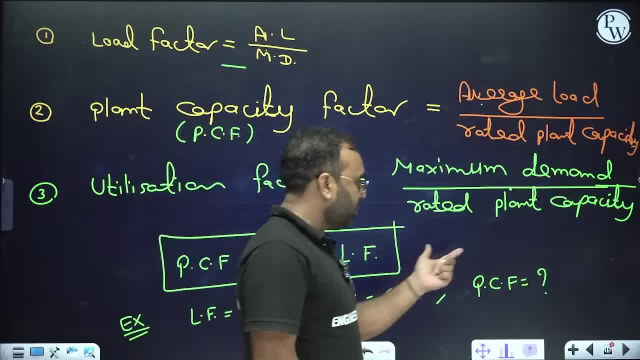 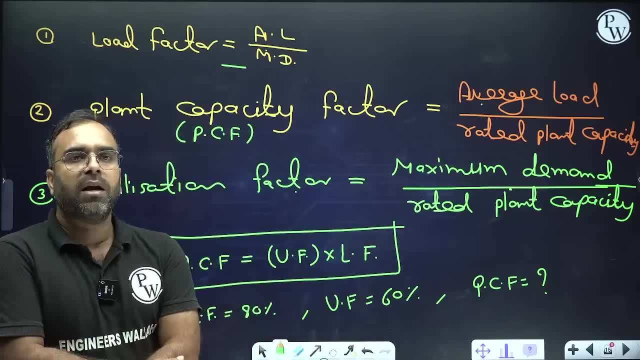 So here the examiner will ask you: The load factor is 80%, The utilization factor is 60%, And what will be the plant capacity factor? So what will be the answer? The answer is different. Some have 56.. Some have 48.. 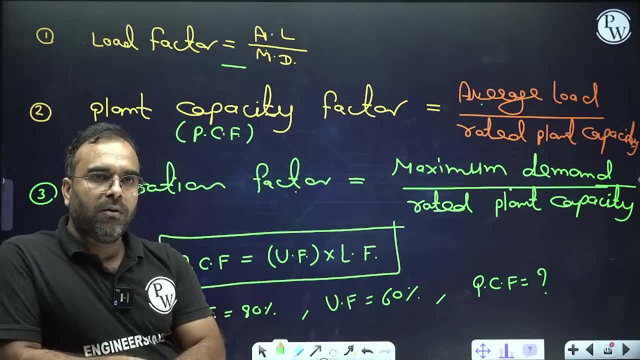 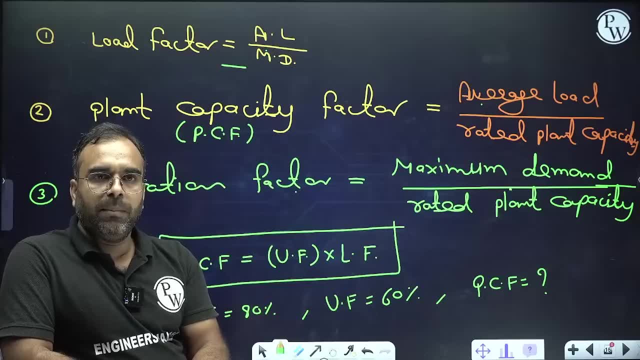 Some have 42. Brother, you are making mistakes in multiply and divide. You are making mistakes in multiply and divide. How will it work? Still, 54 is also going on and 48 is also going on. Come on, understand. 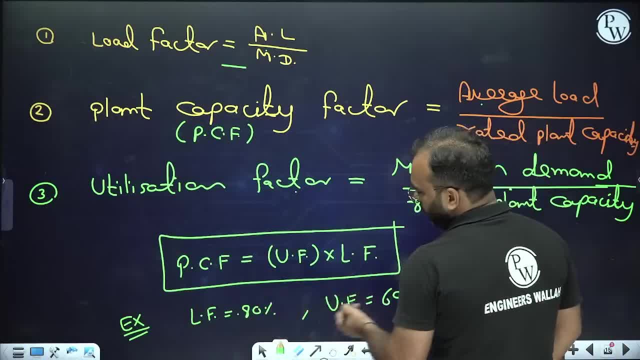 Here, If you ask such a question, Don't you know how to multiply 8 by 6?? Son, do one thing. I will write down the table From 2 to 20.. What do you know? It is possible. 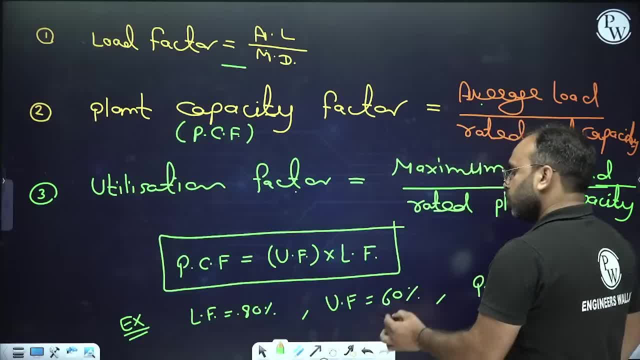 See, I am an engineer. Anything can happen. It is possible. There is no problem if there is no table: 8 to 6.. How much is 8 to 6? It is 48.. If it is 48,, what will be our answer? 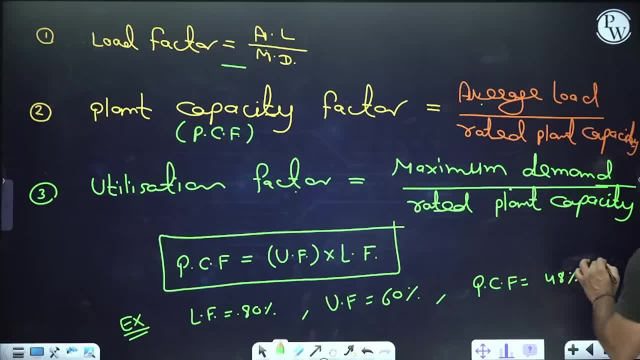 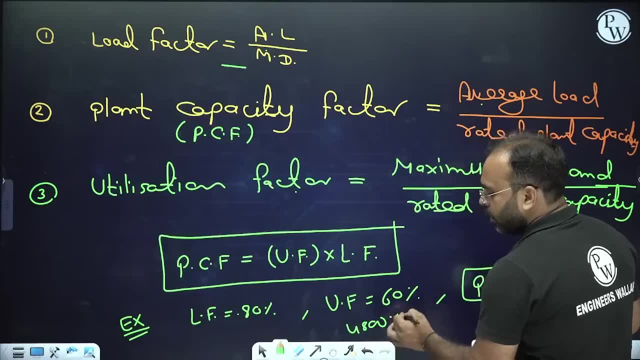 48% will be the answer. But don't do this by mistake. Many times we do the same thing. Sir, if we multiply 80 by 60, then we will have 4800%. Don't do this, Don't do this. 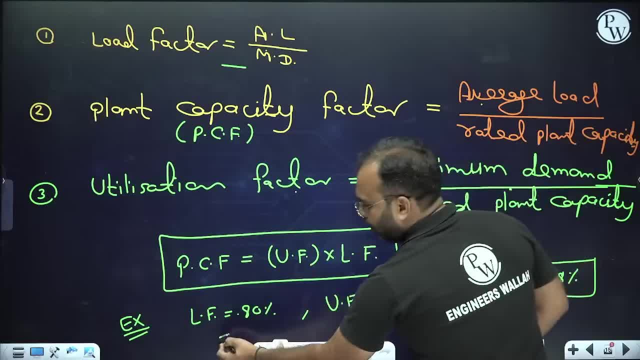 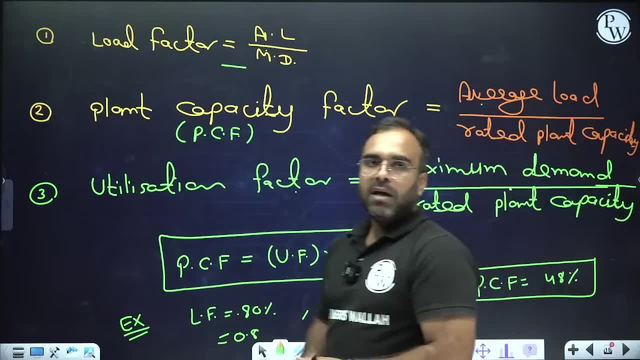 So what will be our answer? Write this first: 0.8, Write this 0.6 And multiply 0.8 and 0.6 by 100.. Our answer will be: Kelsey is not allowed. Yes, Kelsey is allowed. 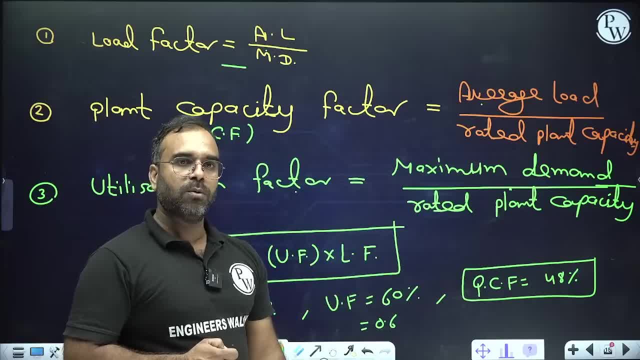 That's a good thing. I don't want to work so hard. Look who said it. Somya said it. Kelsey should be allowed. It is good, Son, do this much hard work. Do it by multiplying 8 by 6.. 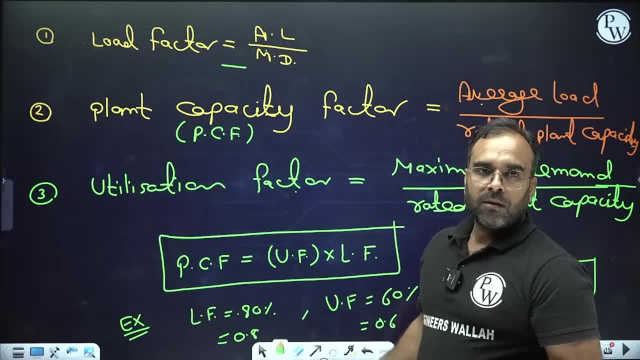 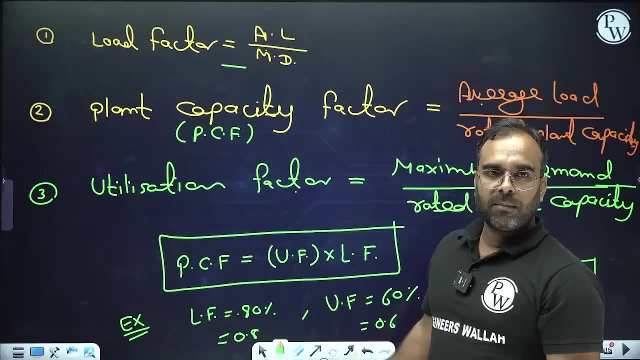 There will be a lot of chickens in this. You know me in school Because I also know a lot, Because I also make a lot in this. If you remember the table, then you have to make a chicken because of this. Who made it? 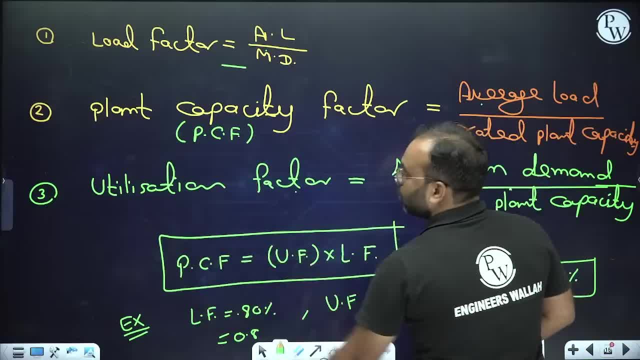 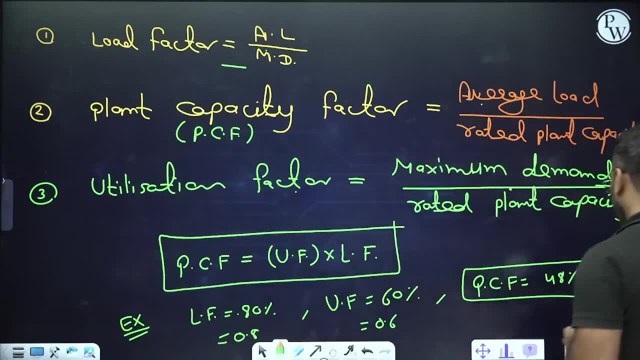 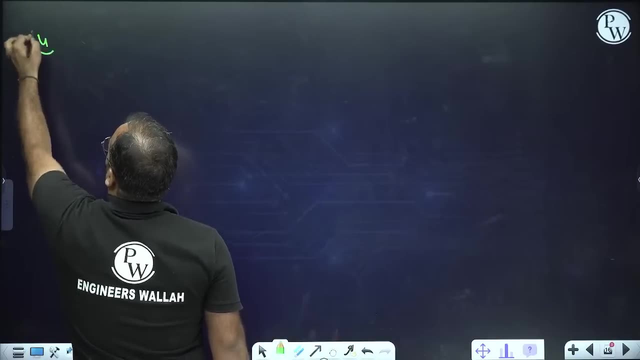 From you. Okay, you must have understood these three formulas, That we have a load factor, plant capacity factor, utilization factor, So we have these three things. Next, we will have the fourth formula, The fourth formula that we will have. 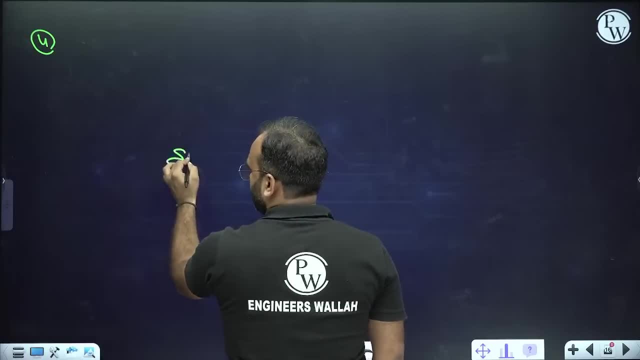 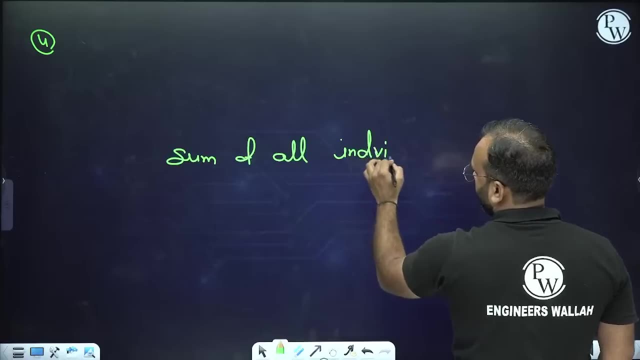 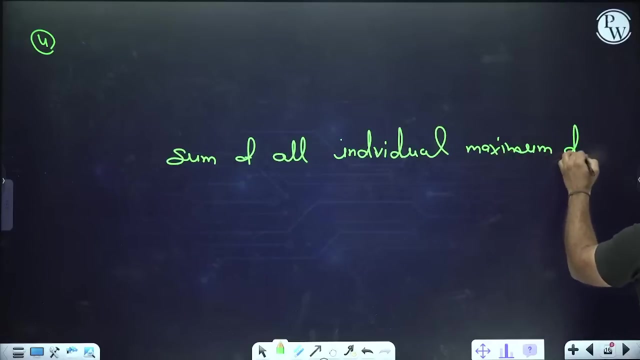 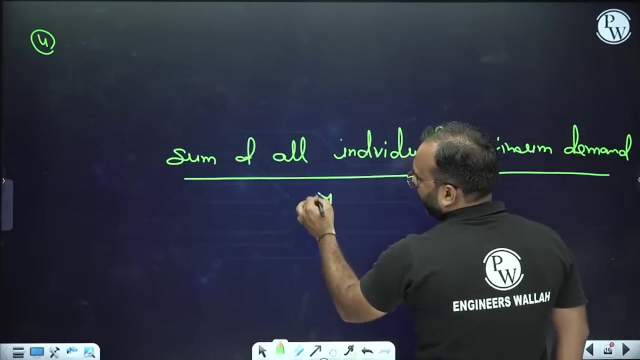 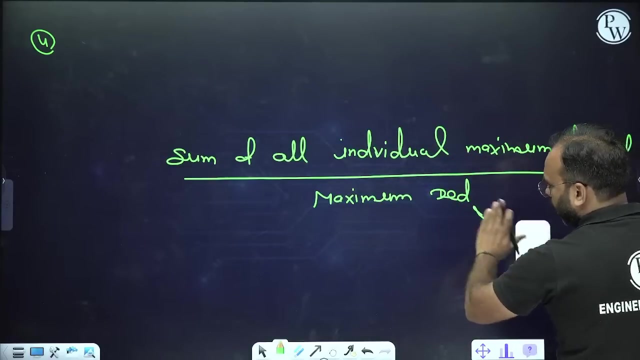 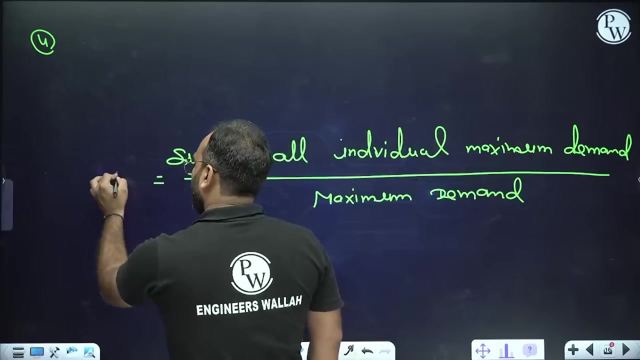 Come on, the examiner will ask you such a question. Some of all, some of all individuals: individual maximum demand, maximum demand, maximum demand. divide by what? by what? the peak demand of the system, or divide by the maximum demand system? what is the ratio of the demand divided by the maximum demand? what will be the answer? 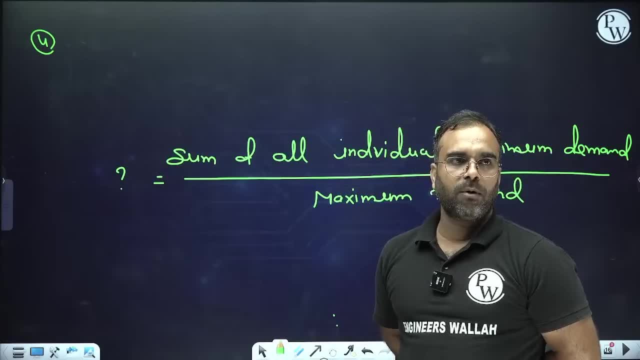 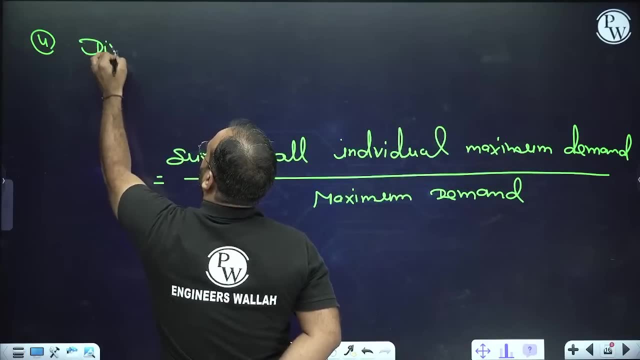 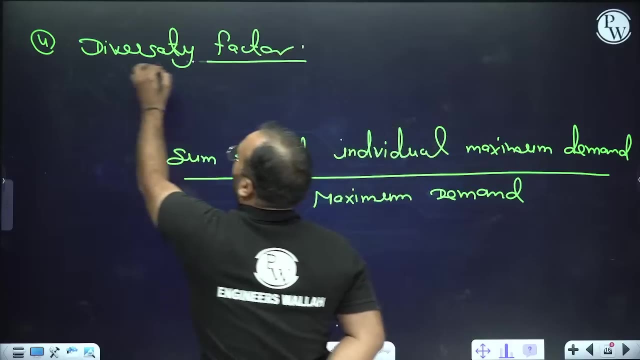 Before the question: you have started to write the answer. diversity factor is the correct answer: diversity factor. so the definition of diversity factor is written here: diversity factor, diversity factor. you all remember. then, where you don't remember, diversity factor. 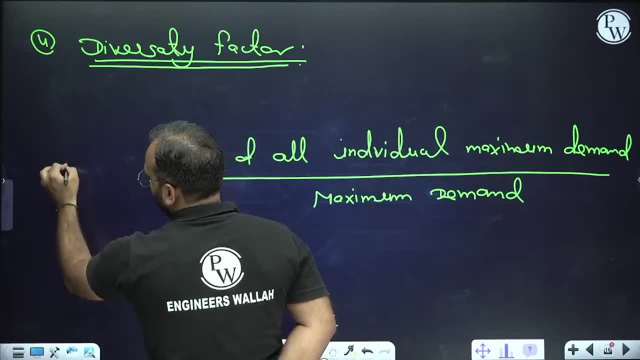 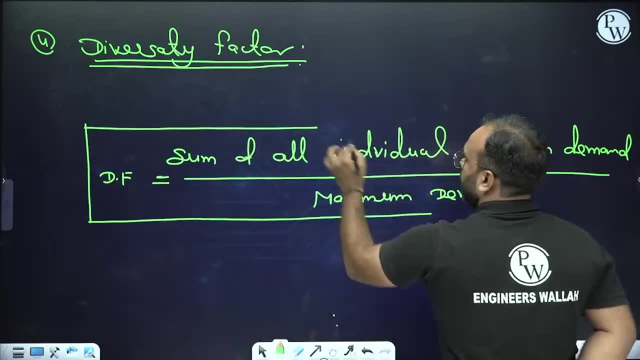 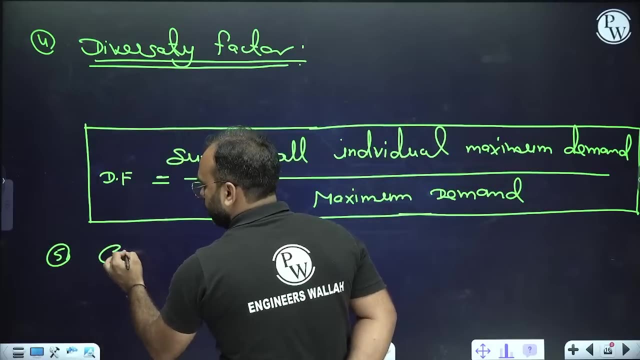 will remain with us, so write here. what is the diversity factor? sum of all individual maximum demand divided by the maximum demand of the system. next here examiner will ask you the same question: what is the coincidence factor? what is the coincidence factor? who? 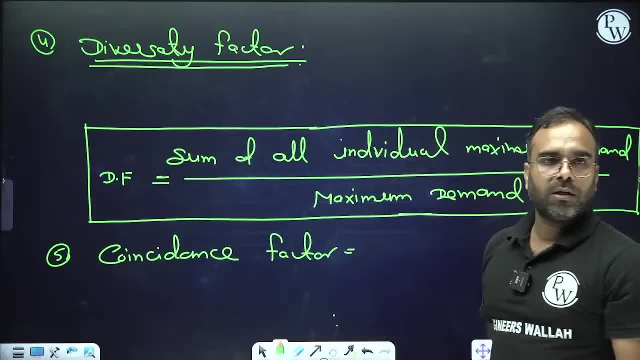 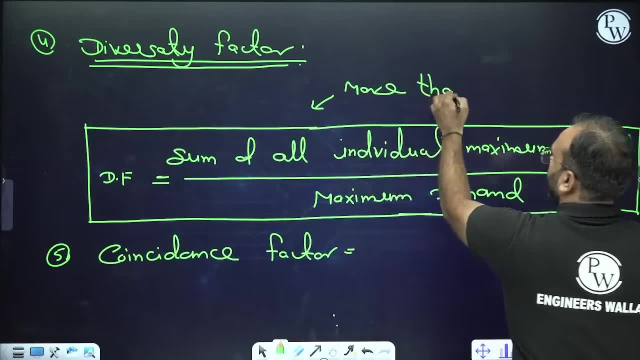 will give the answer to this, because I know this. everyone knows what will be the value of this. It will be more than one correct. its value will be more than one correct answer. more than one correct answer. it will be more than one. come on, tell me quickly here. 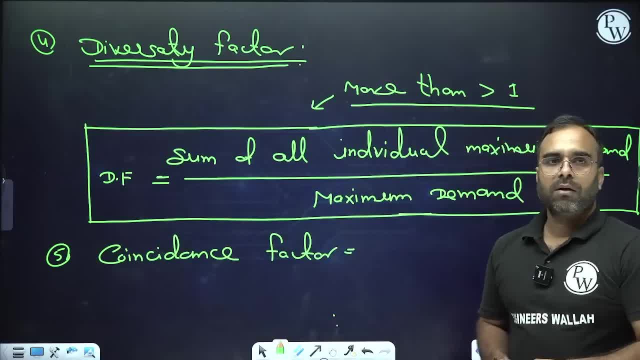 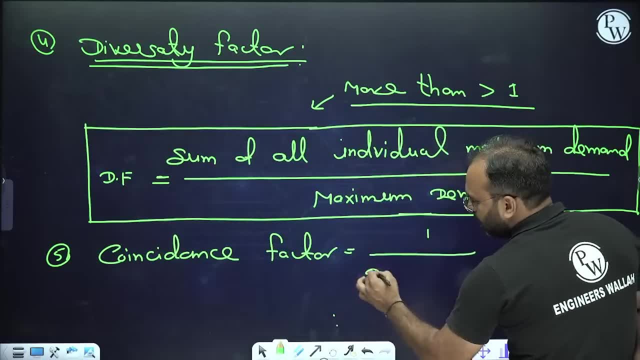 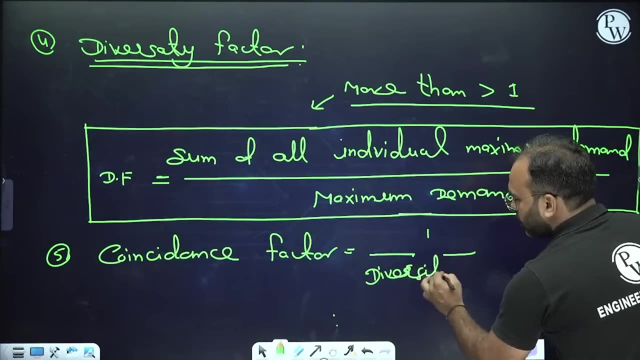 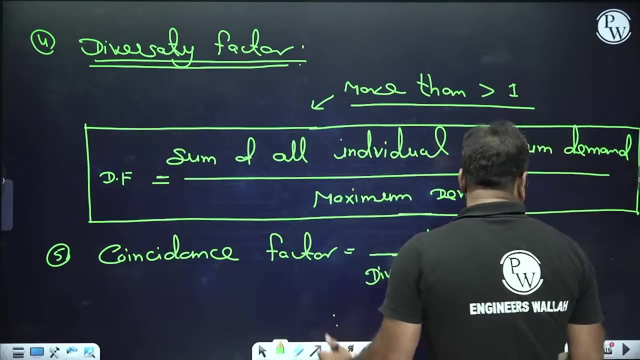 is the reciprocal of diversity factor. correct answer. what will be the coincidence factor? one upon we will have diversity factor. so diversity factor will remain. diversity factor will remain. this will be the correct answer. so here is one more formula. come on, let's. 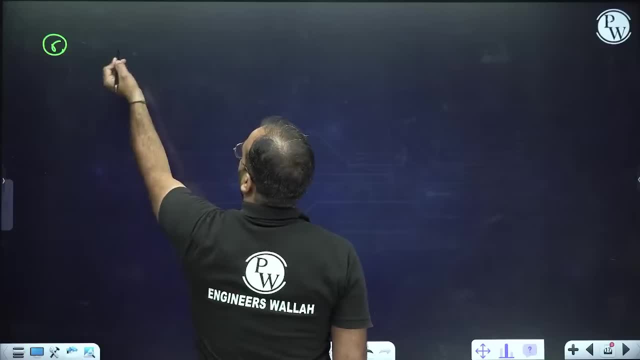 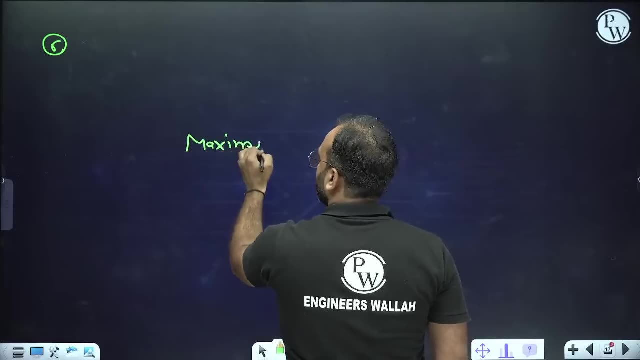 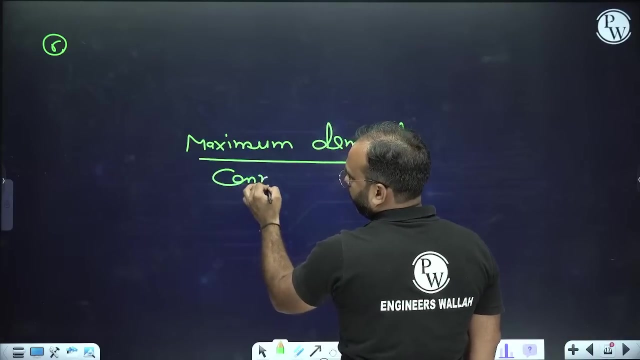 see who will give the answer to it. 6, it is said to you. if it is said to you, tell me maximum demand, maximum demand, maximum demand divided by connected load. what is this formula? Come on, maximum demand divided by connected load, what is this ratio? 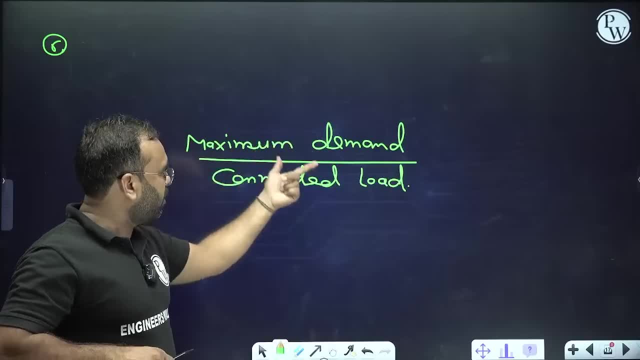 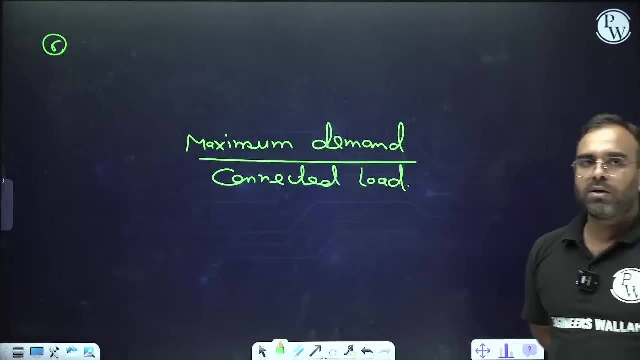 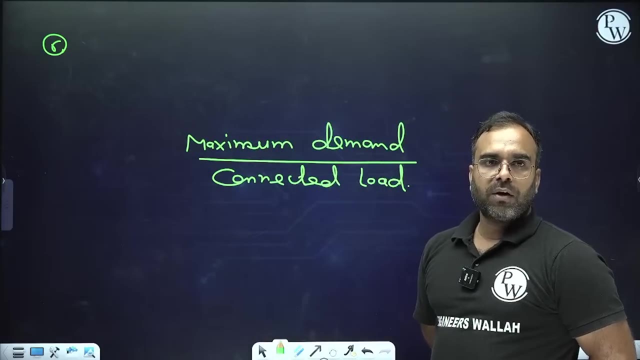 The examiner will ask you: what is the ratio of maximum demand to connected load? What will be the answer? Maximum demand divided by connected load. what will be the answer? Demand factor, demand factor. correct answer right Now. don't get confused in that DF, diversity factor and demand factor, right. 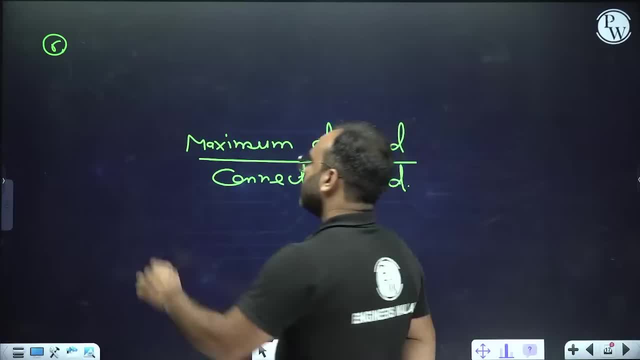 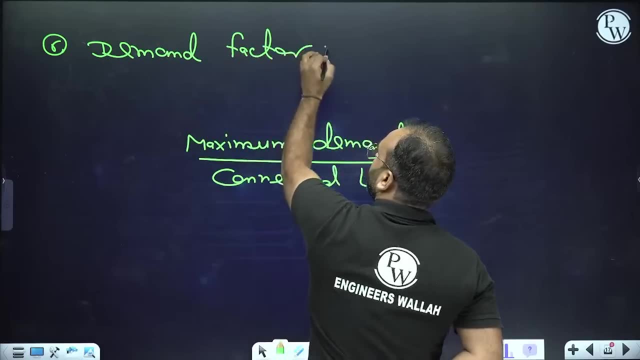 Come on. so demand factor is the correct answer. so here you will write one more definition. you write the definition of demand factor. what will be the demand factor? It will remain so. it will remain maximum demand divided by connected load. 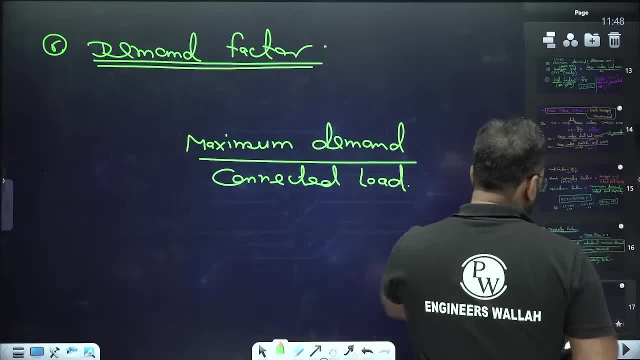 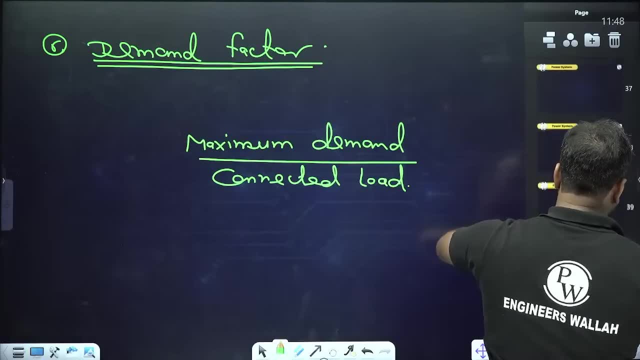 Come on, see, let's do one thing here. you will be asked some questions here, examiner. I will do some numerical related to them so you will get a little confidence that how numerical is asked. come on, you answer this question. come on one more formula reserve. 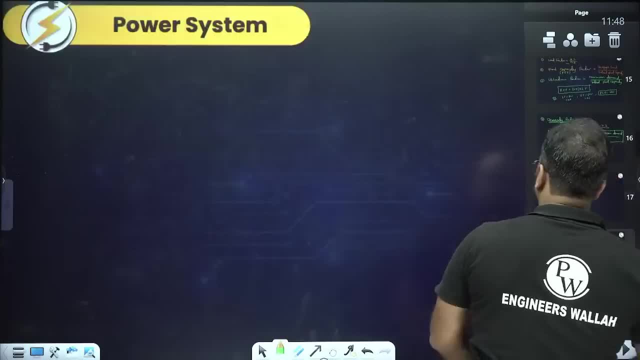 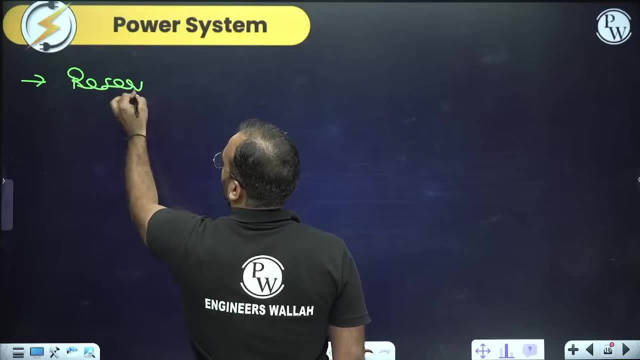 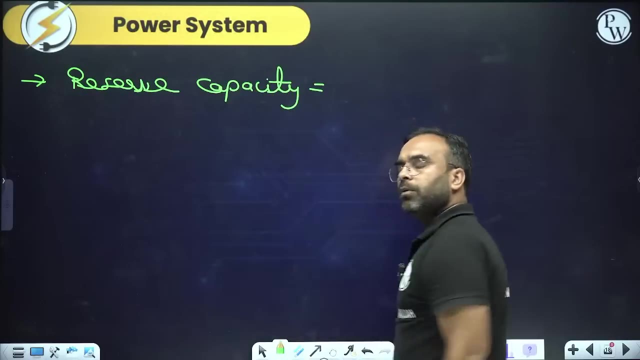 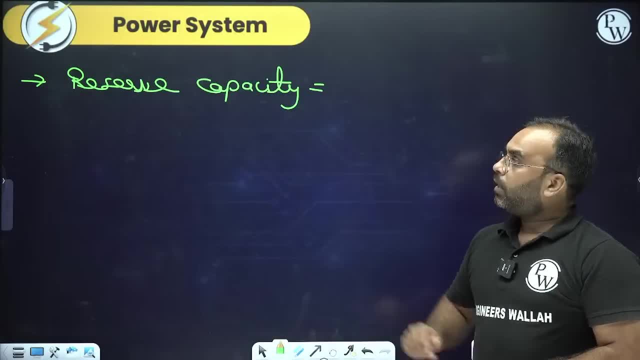 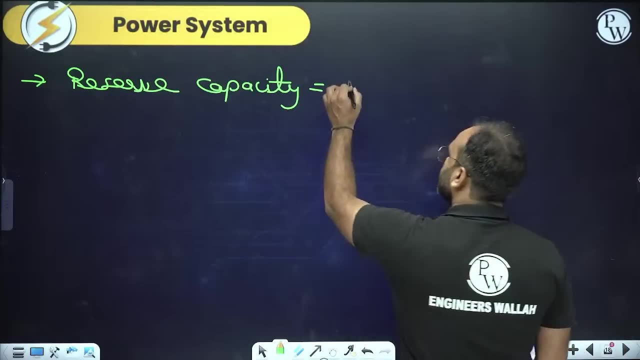 Come on, tell me quickly from here: if you are asked what is reserve capacity, then what will be reserve capacity? What will you do from plant capacity? If you minus the maximum demand, then the correct answer is that, sir, our plant capacity. 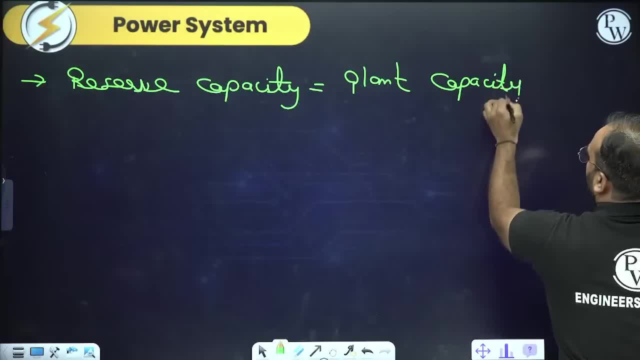 will be from plant capacity. We will minus the maximum demand, Maximum demand. So this will remain with us, the formula of reserve capacity. So come on, the first numerical is on this and you will tell me the answer. what will be the answer of the first numerical? 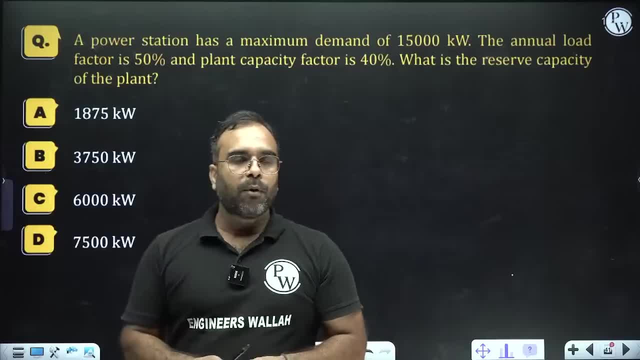 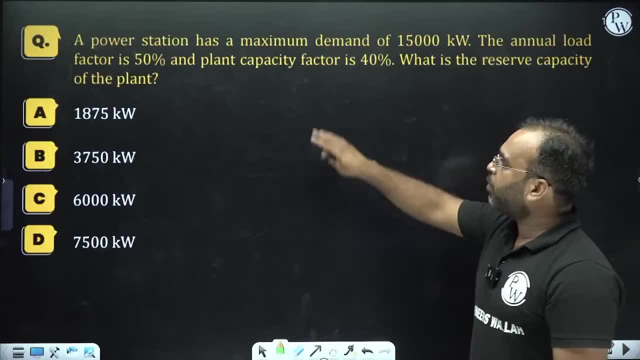 Come on, tell me the answer of this question quickly, And you know your exam will give you only 40 seconds to do. in 40 seconds the answer of this question should come. It is said to you that this is a plant station. the maximum demand is this much, the maximum. 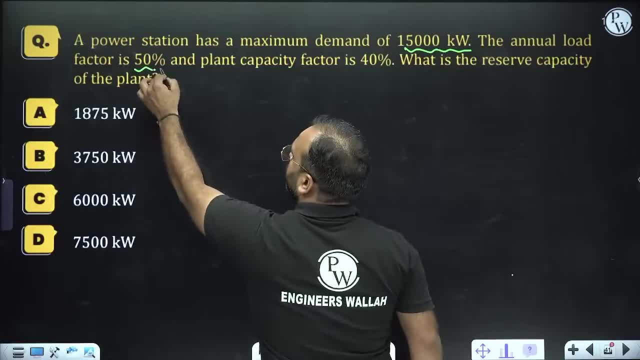 demand is this much. the annual load factor is this much. The plant capacity factor is this much. the reserve capacity has been asked from you. what will be the answer? What will be the answer of the reserve capacity? Your answer should come in 40 seconds. within what time duration? 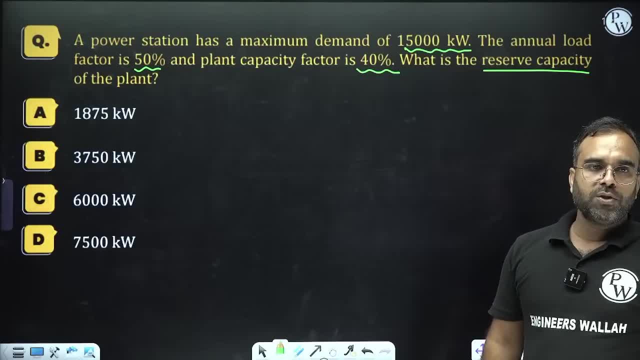 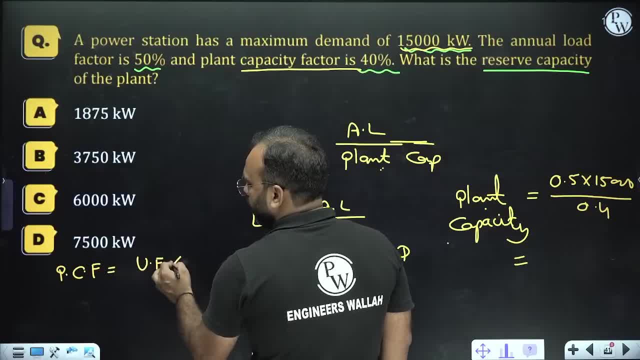 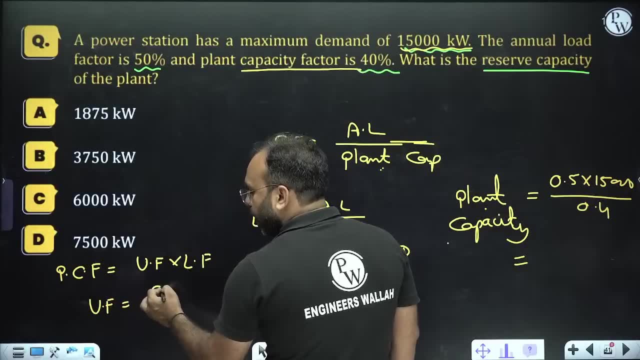 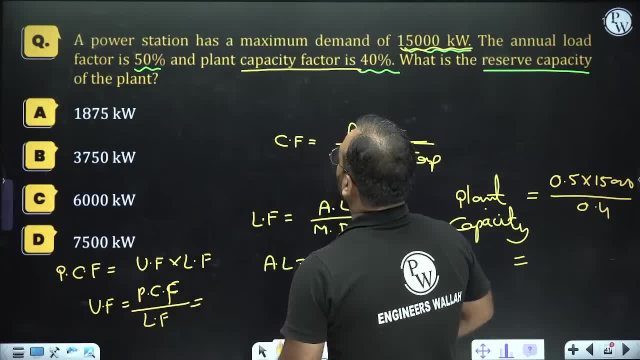 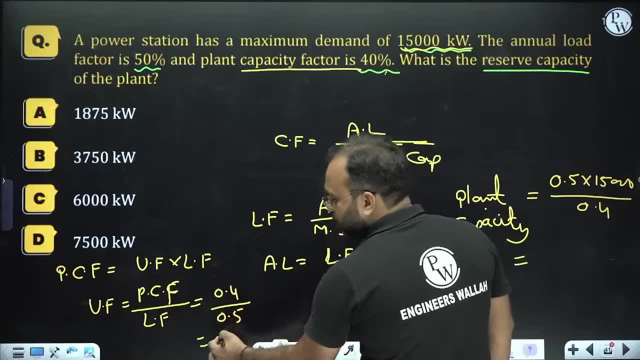 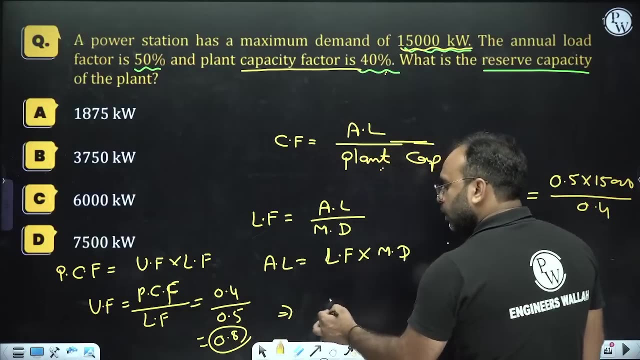 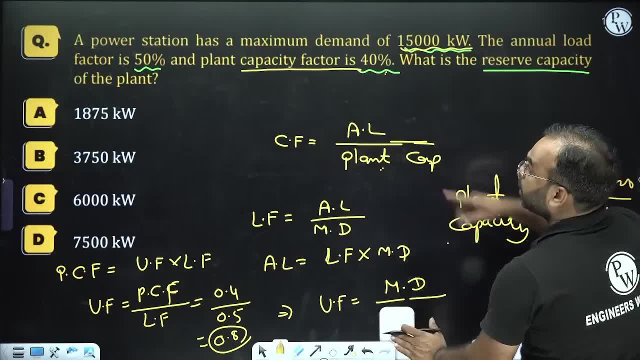 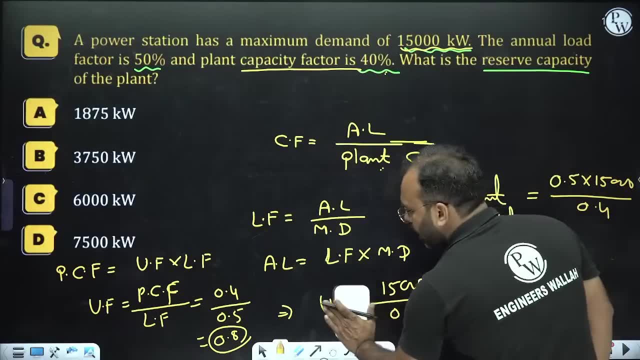 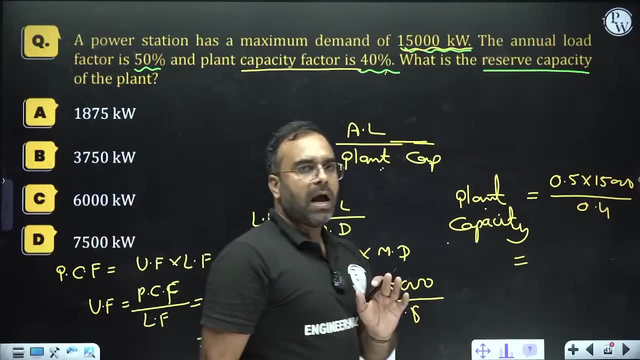 So if you divide the utilization factor by the maximum demand of 15000, divided by 0.8,, then you can extract plant capacity from here too. You can extract from whatever you like, but the answer should be correct. Now tell me what is the answer. some are saying B and some are saying A. 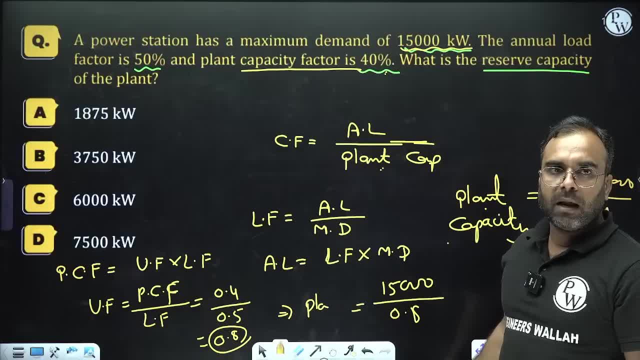 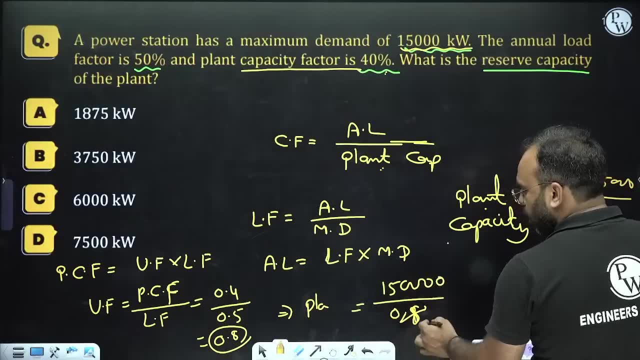 Some are saying A and some are saying B. Now tell me what will be the answer. If you divide it, then you will get 1.0 from here. If you cancel it from here, then you will get 1.. After that, 7 will be left here. 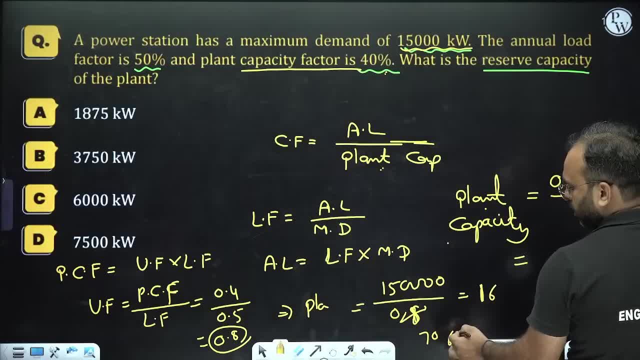 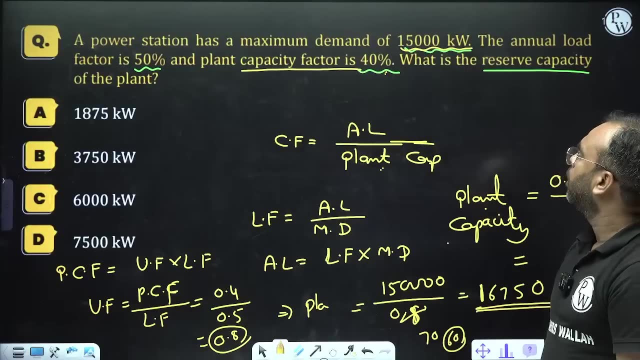 So this is 1.0.. So from here you will get 6.. You will get 16750.. Tell me quickly what is the answer. Try to divide it correctly. If you solve it here, then you will get 7500 from here. 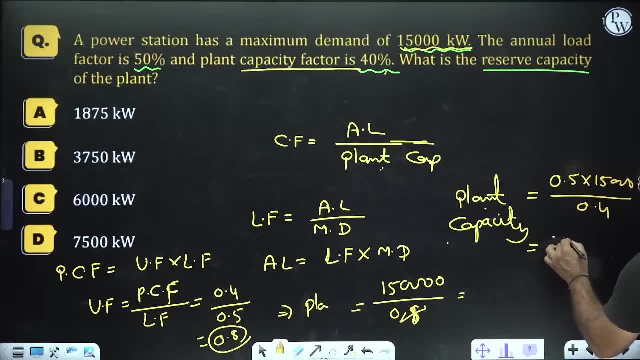 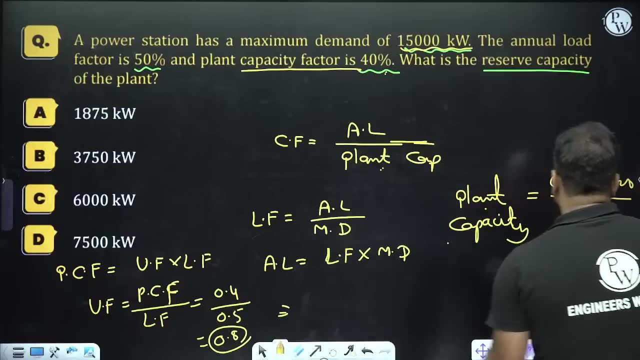 75000 and divide it by 4.. So from here you will get 1. And from here you will get 18.. And from here you will get 18750.. So from here you will get 18750.. This is the answer. 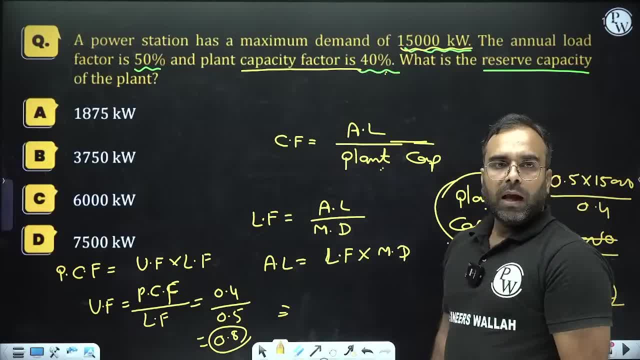 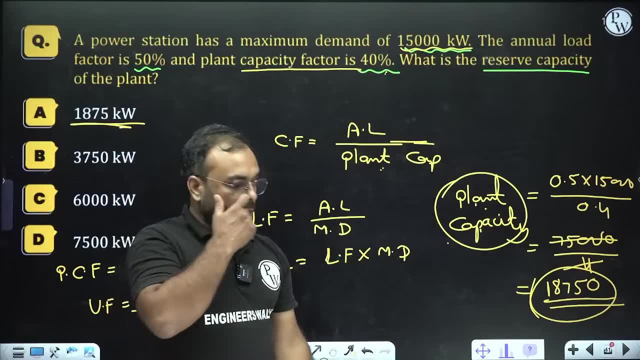 This is not a plant capacity. Actually, you are wrong about the answer. I did not ask you this, I did not ask you the plant capacity. Now you must be thinking, sir. our answer is 18750.. Let me tell you, if you are an engineer, there is no problem. 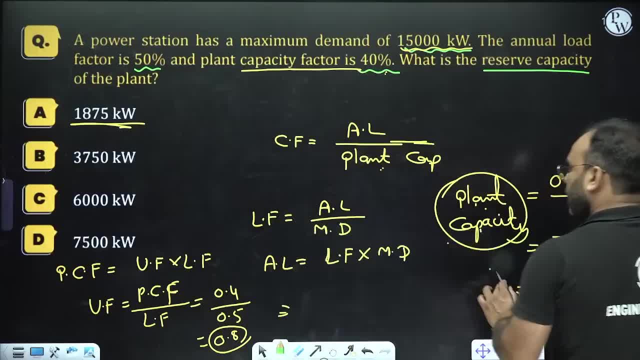 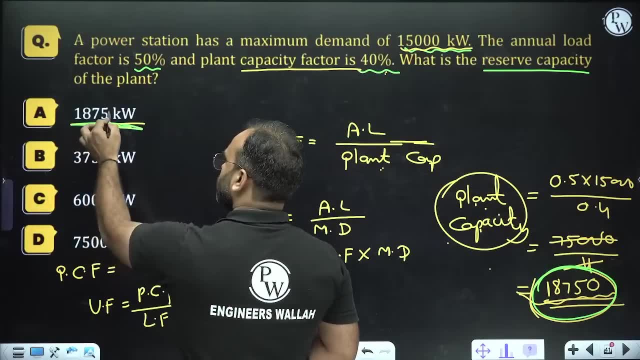 If you are an engineer, you can do anything. What will engineers do, Sir? 18750 is our answer. But, sir, if the option is not 18750, then we thought there would be a point mistake somewhere. So we put a zero from our side and put A in the answer. 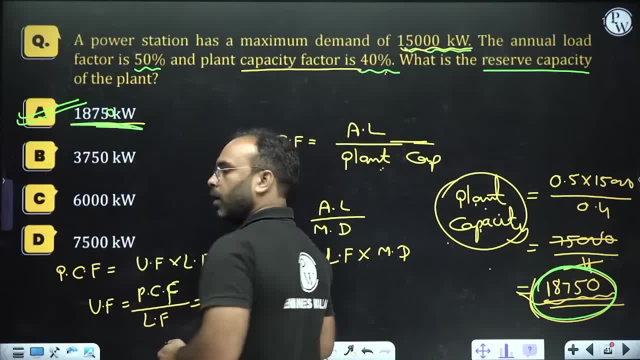 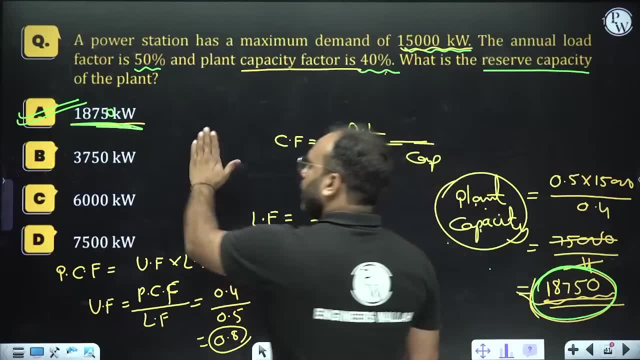 and if our answer is A, then it is correct. We can do this, we can do anything. Brother, I have not asked you this, I have asked you the answer. I have asked the reserve capacity. So to get the reserve capacity. 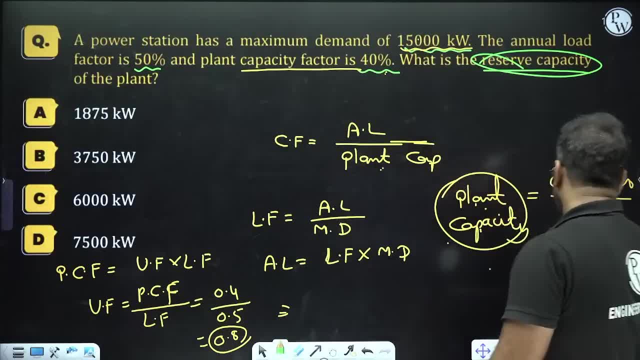 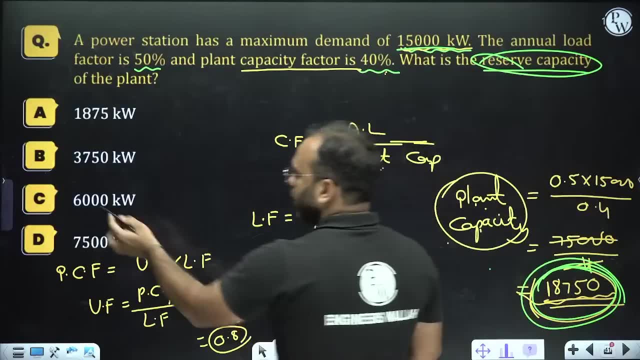 first, you minus this plant capacity and maximum demand. So out of 18,750, if 15,000 will be minus, then 3,000 will have to be minus, 3,750 will come. So look, you have two processes. 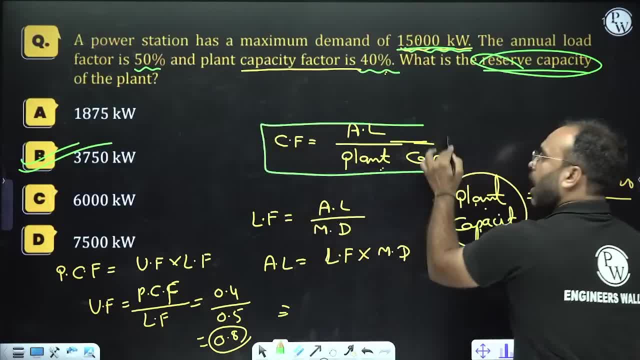 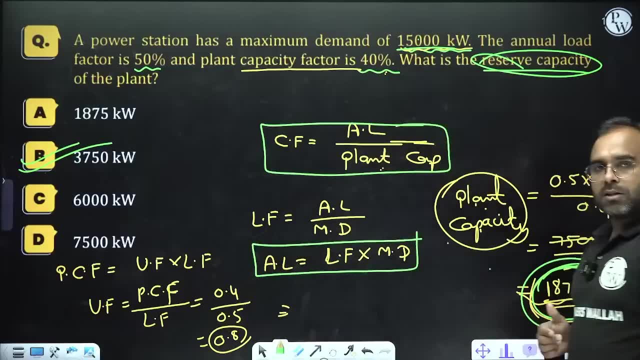 Two processes- if you want, you can do it from here. If you want, you can do it from here- In which you have to remove this average load. you can remove that load factor by doing maximum demand, Put this value here and remove it. 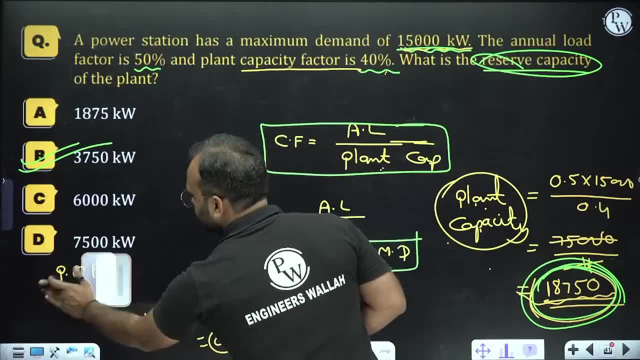 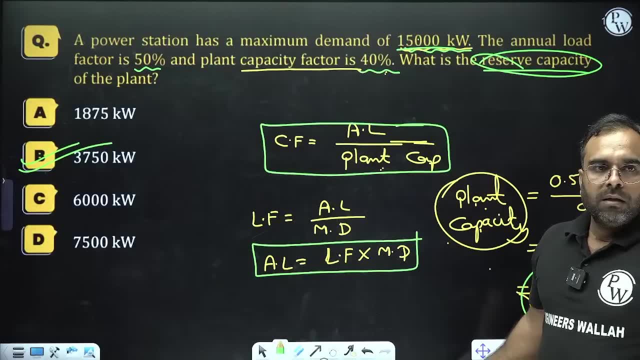 Otherwise, if you go directly to the utilization factor from there, then you can get the answer from there also. You can get the answer from there also. Your answer will be the same. Okay, Come on next. Tell me the answer of the next question quickly. 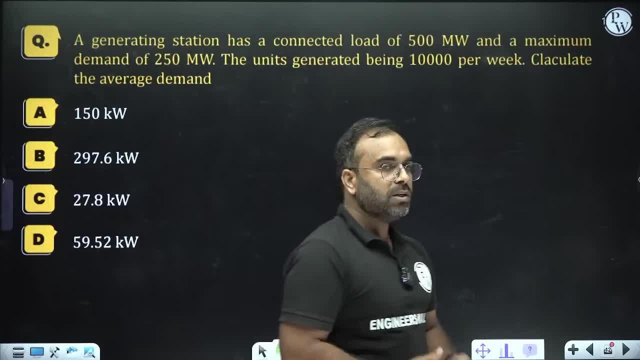 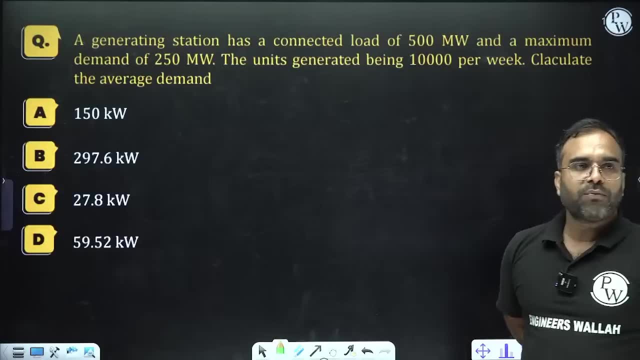 What will be the answer of this question? What will be the answer of this question? What will be the answer of this question? Come on, we will reply quickly once. Reply a little fast. I don't see that energy today. I should see energy in the class. 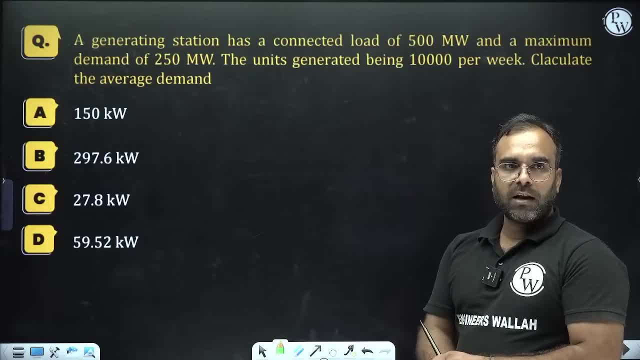 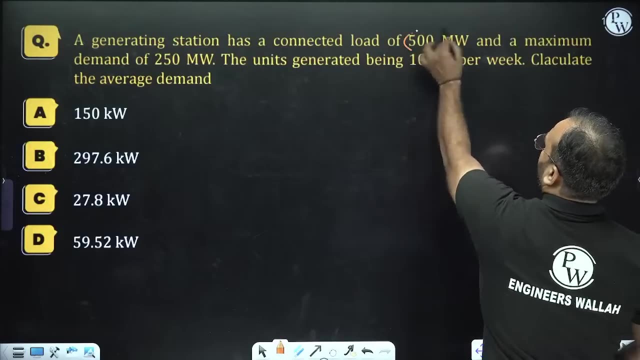 And it should be about studies only Today. I feel good that you are talking about studies only. You are not talking about anything else. You just have to focus. Come on. So from here the question is asked to you. Station has given so much connected load. 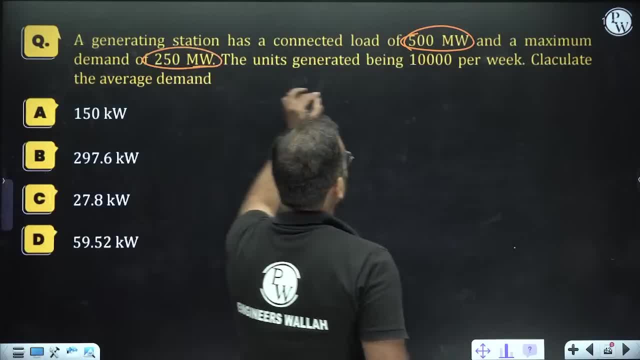 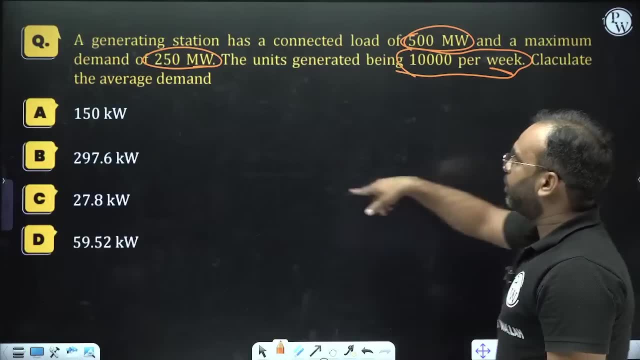 So much connected load, So much maximum demand given to you. Unit generated per week is given. Remember it has given a week. Unit generated per week is given to you. You are asked to calculate average load. Okay, If you want to calculate the average load. 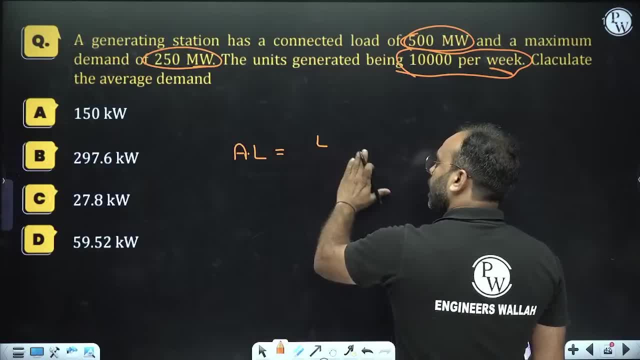 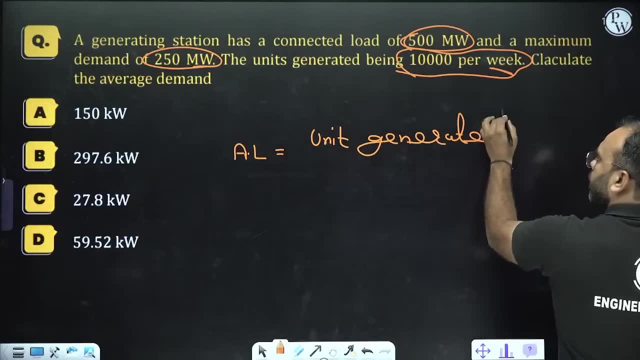 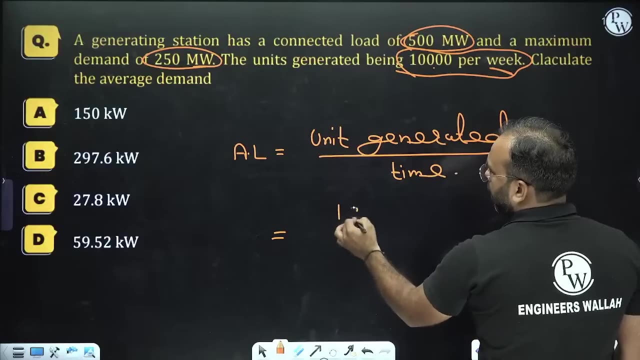 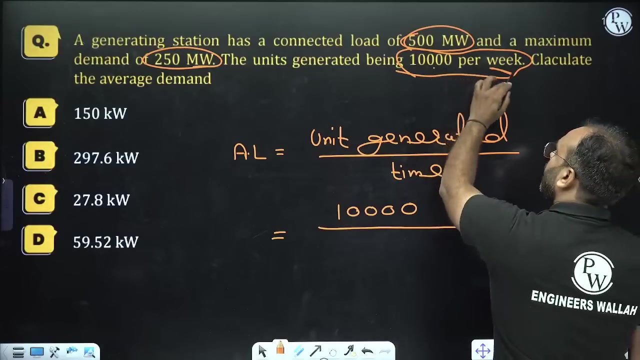 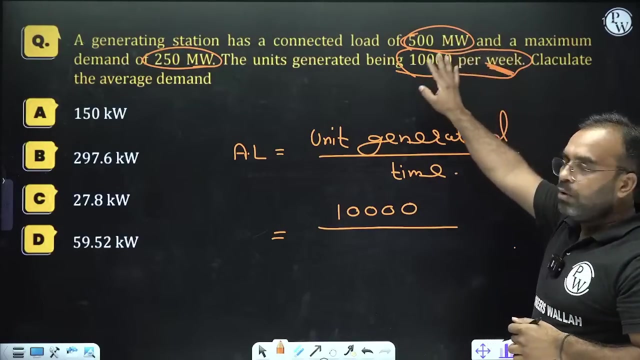 If you want to calculate the average load. So what did I say Here? unit generated. What did I say? Unit generated? unit generated divided by. you have to do time and nothing else. now how much is the unit generated? then he has given the unit 10,000, now if he has given me the unit generated, divide by the time, and if I talk about the time, then how many hours are there in a week? tell me quickly. here you have 10,000 per week. unit generated. unit means in kilowatt hour. 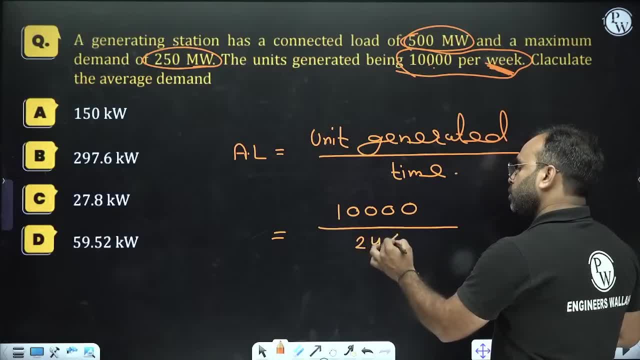 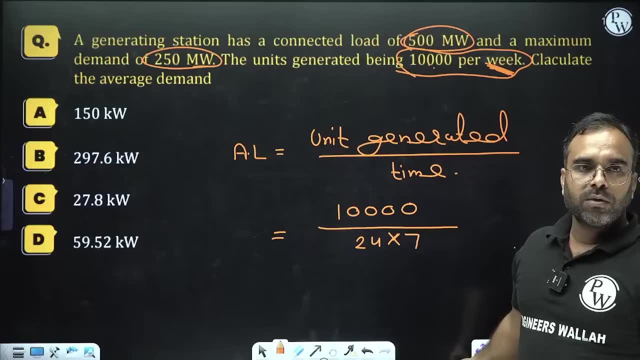 so here there are 24 hours in a day and I know that you must have remembered a lot in your childhood that there are 7 days in a week. there are 7 days in a week, so just take out the answer from here. tell me quickly what is the answer coming. 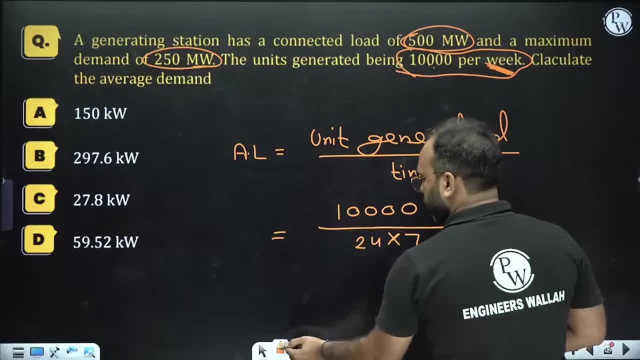 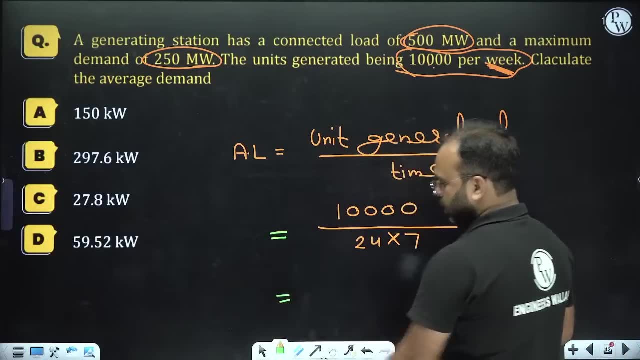 let's go. no problem, Kiran. now focus on studying. you don't have to watch more than 3-8 movies. what happens with that is that the mind diverts a little. then we start working on its rule. don't do that. 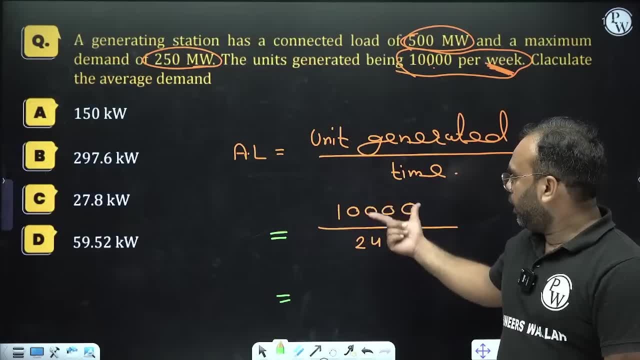 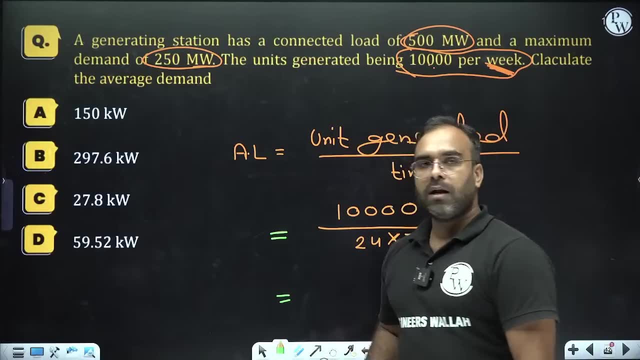 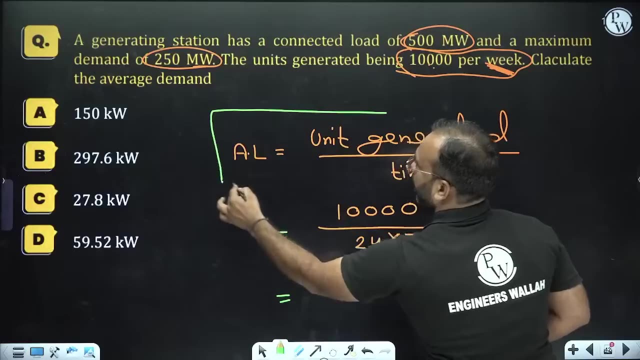 come here quickly. what is the answer? to divide 10,000 by this, then what is coming now? you have to divide it. there is no answer if you have to remove the Provost, if you have ever. I have asked you for the rpmge load. I have asked your load factor. some may be giving you an import of I200, this. is 250,. nothing has been done. I have not been asked anything related to it. I have given you such additional data. he will ask you: what is the work of 500,? it is about 250,. it will ask you: such additional data has given you. he has not given you additional data. they gave you any additional data or any data and he contribute these things stick only to you. for example, they are paid to get any additional investment ratio. employees feeling everyday. 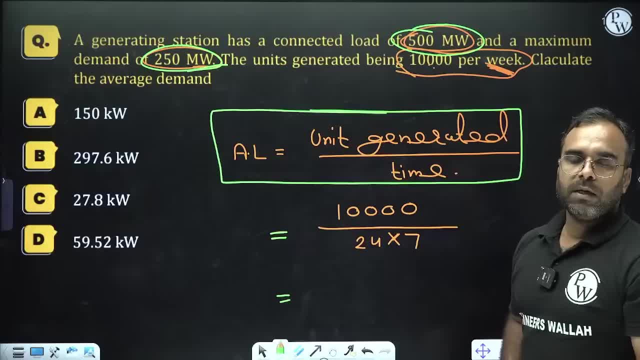 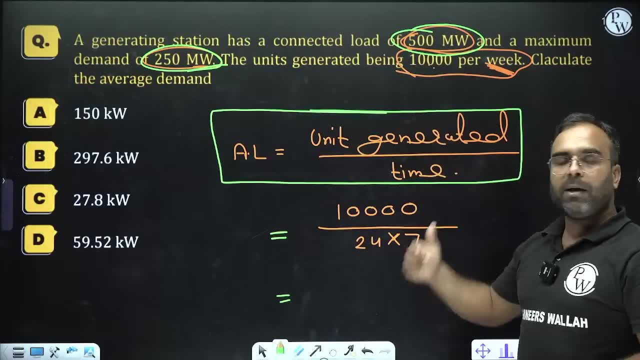 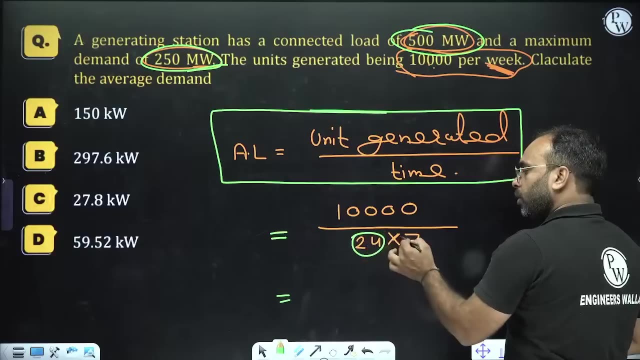 that's why the intensiverogữ Hack one send it, you get a complete option and forever gain too much risk. I have not been asked anything related to that. he has given additional data to you. he has not asked. there is no work related to that. I just asked how much is the average load that unit generated, divided by time, and how many hours are there in a week. so in one week there are 24 hours in a day and there are 7 days in a week, so you can get the answer according to that. 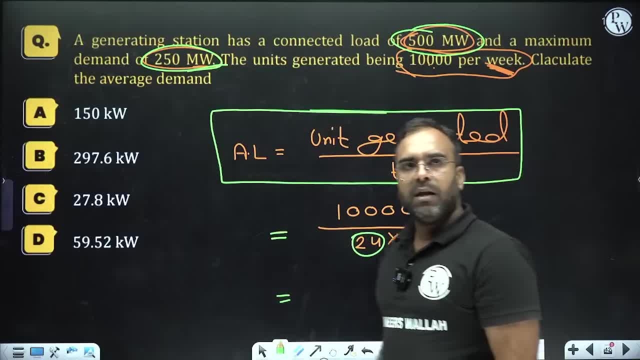 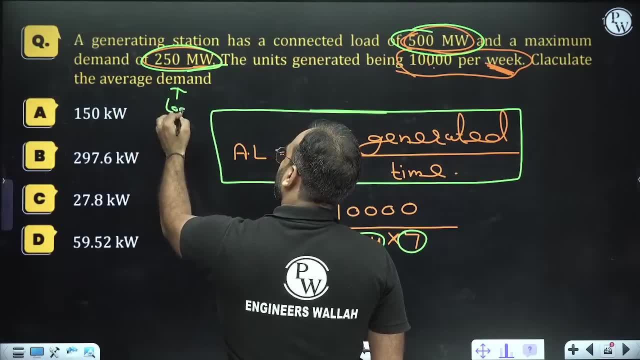 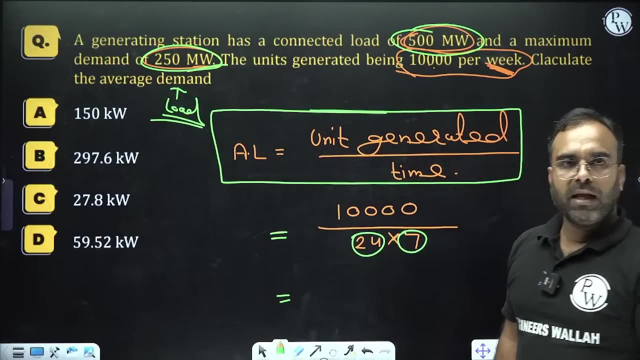 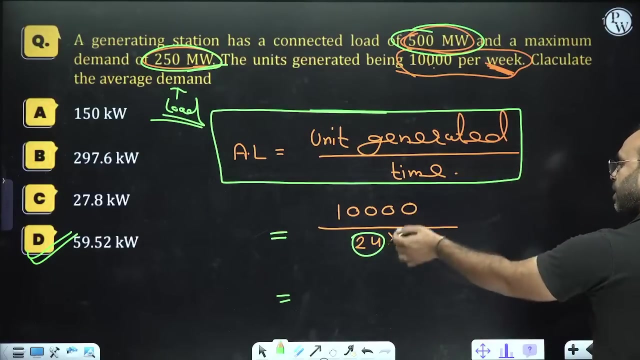 average demand or average load is one thing. if you are asked about the maximum demand or maximum load, then our answer will be correct, so the answer will be D. I am sure I am writing on your request so you can divide from here. 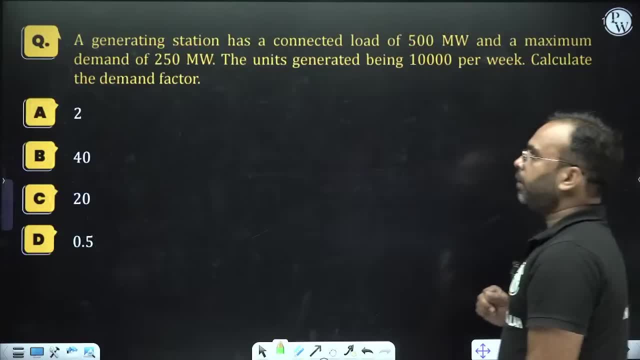 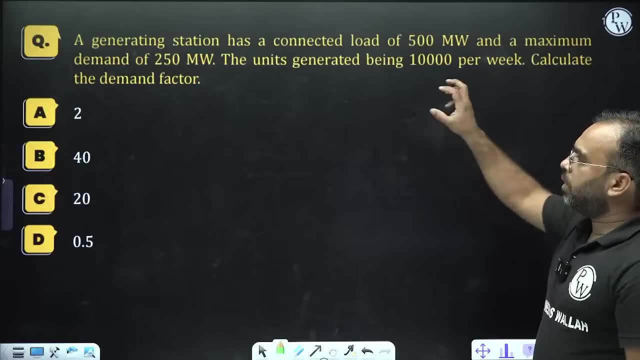 next. after this, let's do one more numerical, then we will move ahead. come on quickly, tell me what will be the answer to this question. what will be the answer to this question? I have asked you the same question. it is the same question. I asked you: how much will be the demand factor? quickly, tell me how much will be the demand factor. 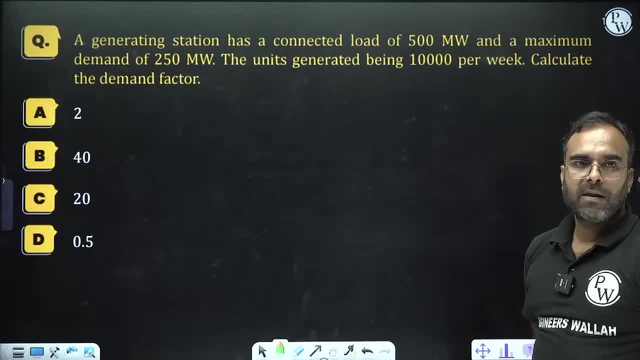 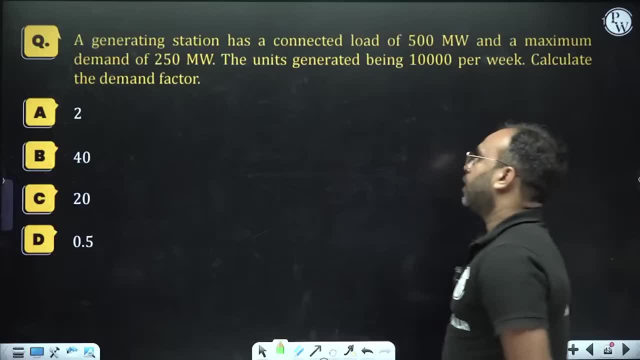 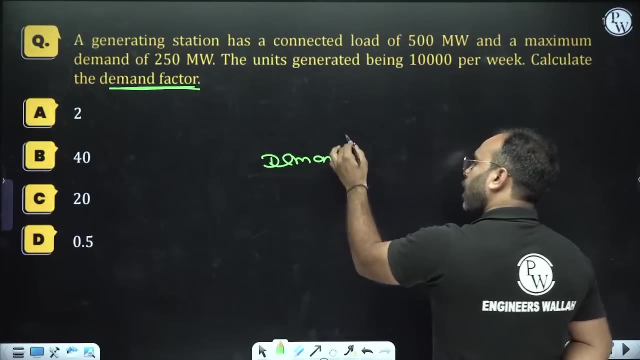 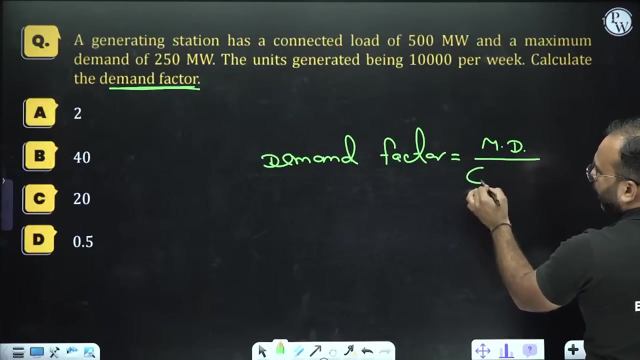 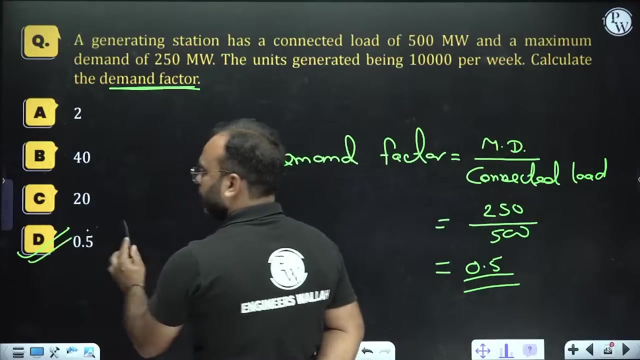 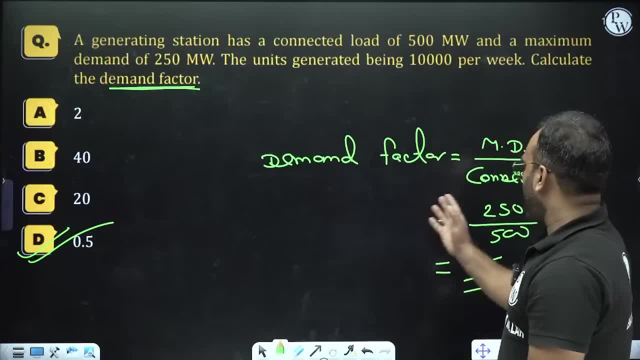 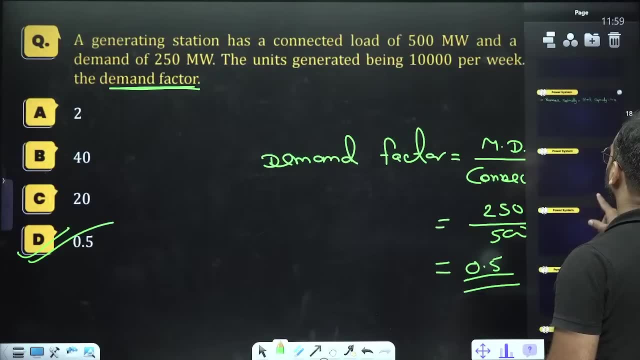 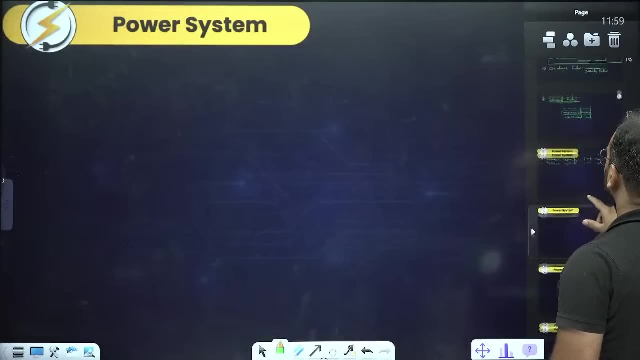 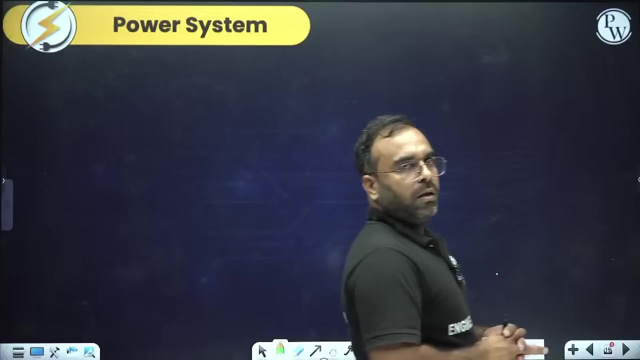 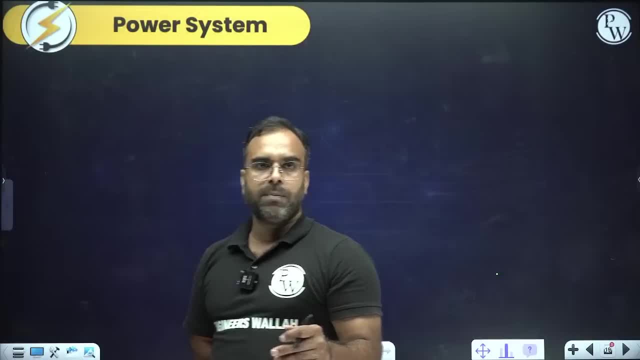 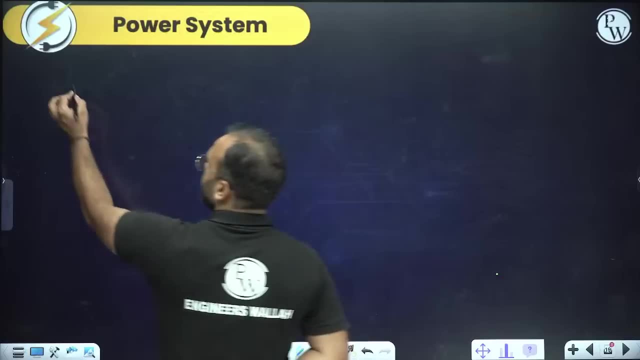 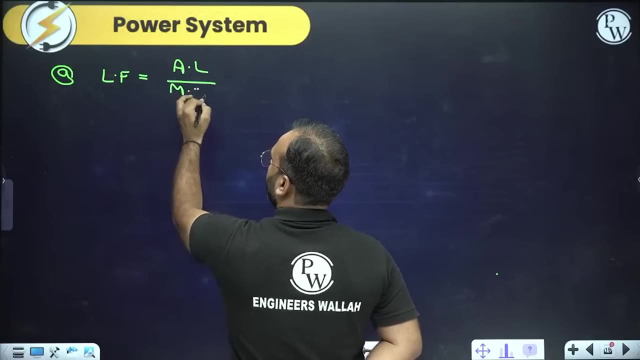 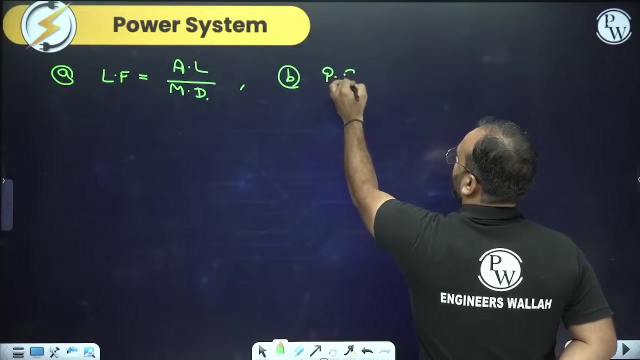 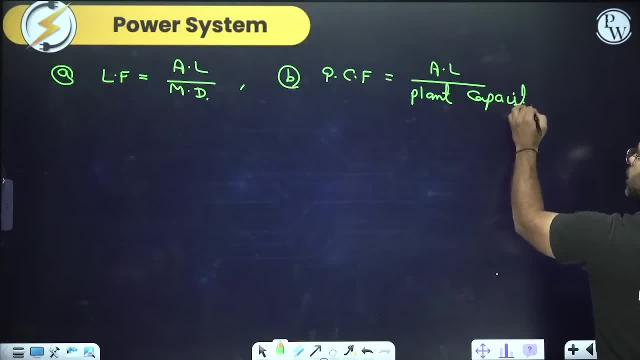 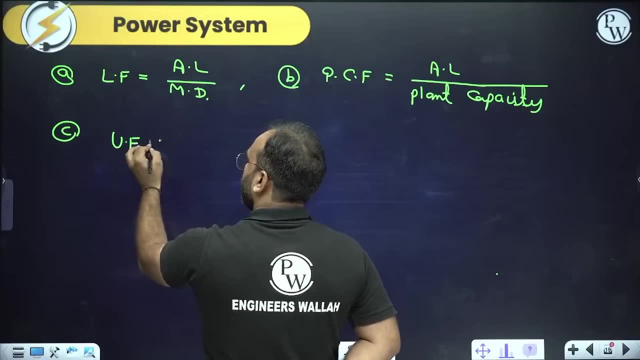 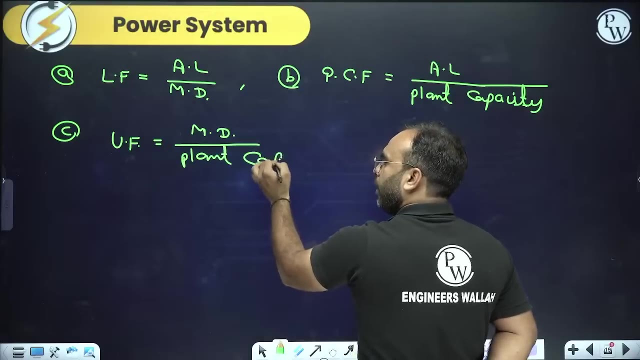 Plant capacity, Plant capacity. Just remembering this much, if your numerical is being made, then remembering is very good for us. Utilization factor will be with us: Maximum demand divided by plant capacity. Maximum demand divided by plant capacity. You must be thinking that we have read a lot. 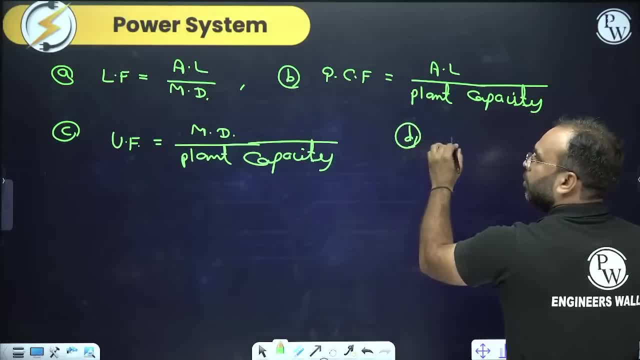 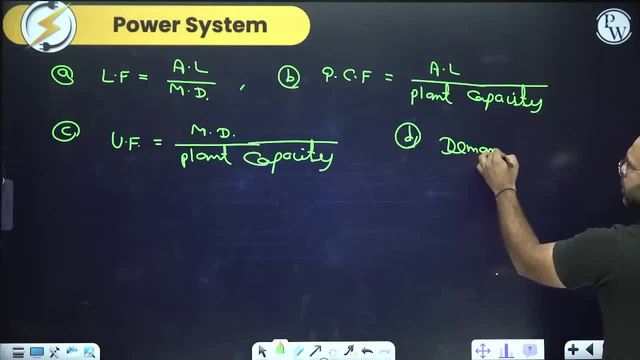 But, in summary, you will see that we have not read anything. We have read very little. Next, what will happen here, Next, after this, the load demand factor will come. Next will be demand factor, Demand factor. I have just told you Maximum demand divided by connected load. 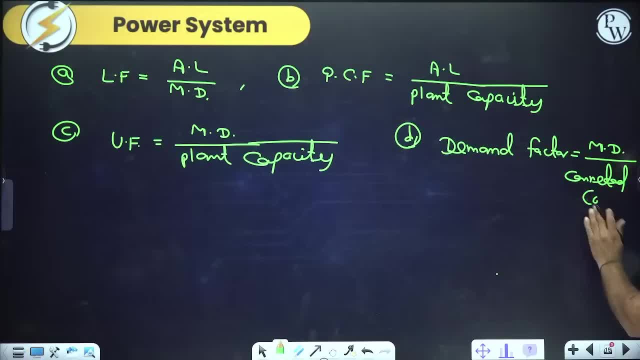 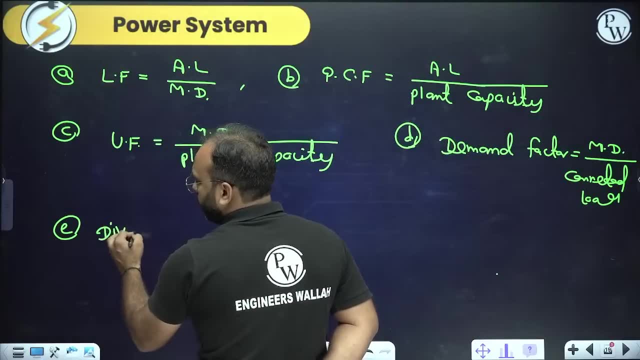 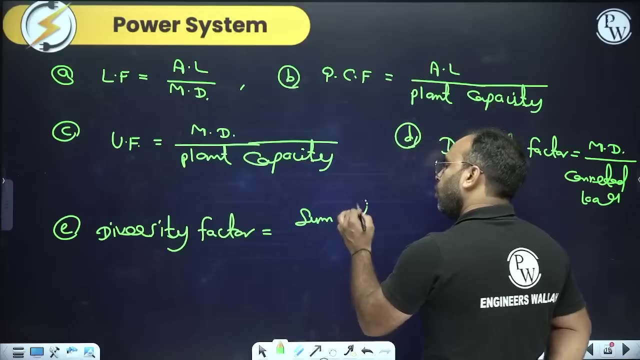 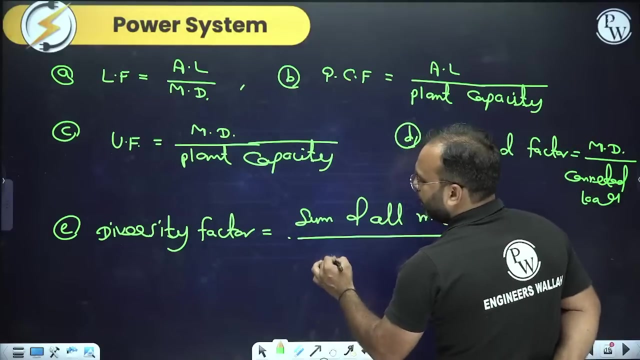 Maximum demand divided by connected load: Connected load. Next, after this E formula will be diversity factor. What will be diversity factor? And diversity factor will be with us: Sum of all maximum demand, All individual maximum demand Divide by maximum demand of system, Maximum demand of system. Take their ratio, you are a diversity factor. 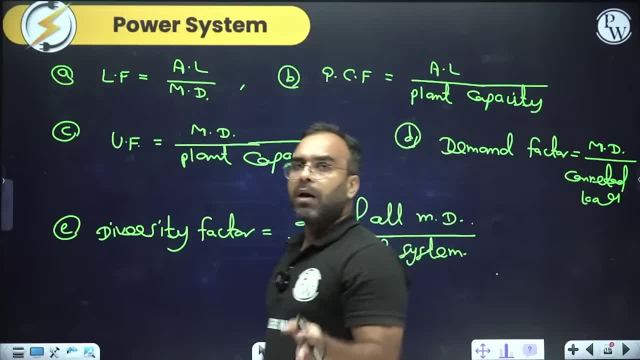 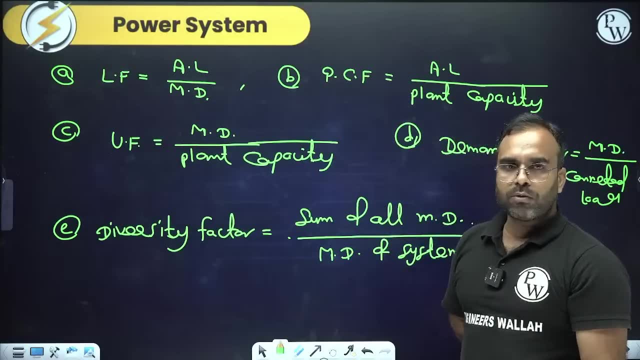 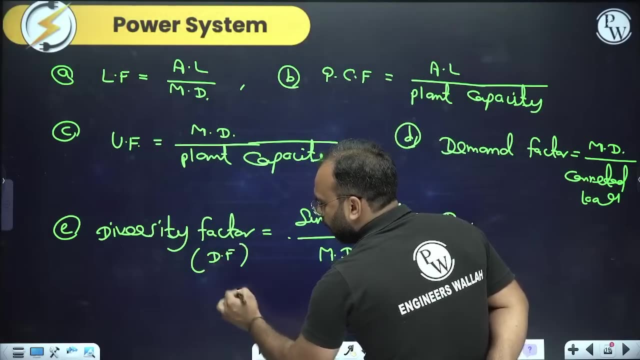 Ok, tell me the diversity factor will be near to 1. What will be the benefit from it? Diversity factor is: If it is near to 1, then tell me what will be the benefit from it. Diversity factor is DFA. Diversity factor is If it is more than 1 with us. 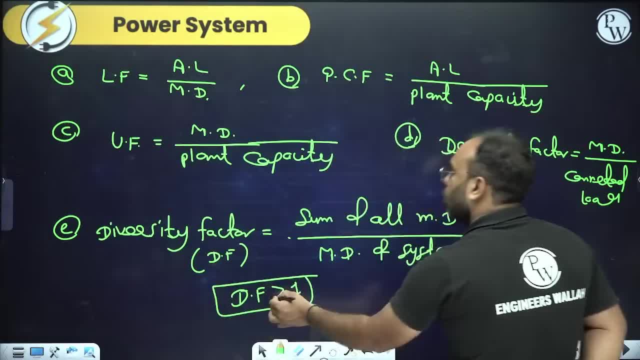 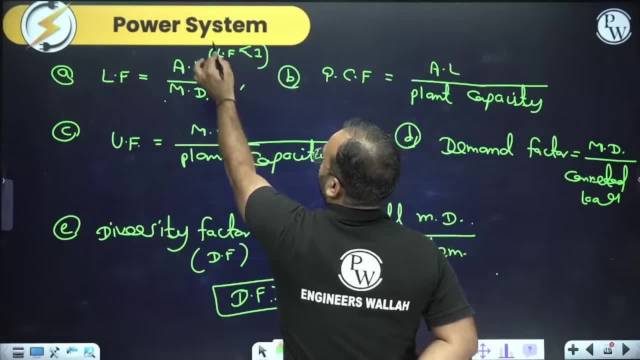 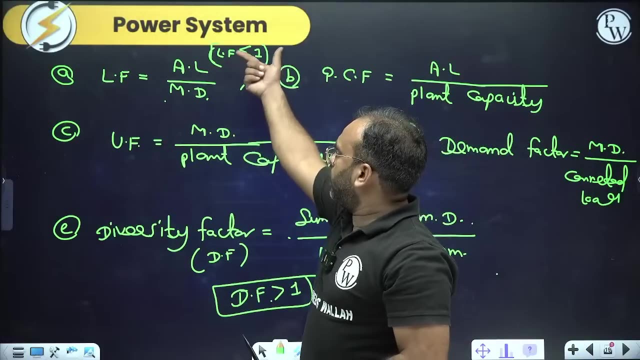 By the way, you know that it is more than 1, But if it is near to 1, then what will be the benefit from it? Average load factor is also less than 1. What will be the benefit from it? Cost will be decreased If its value, and its value is near to 1. 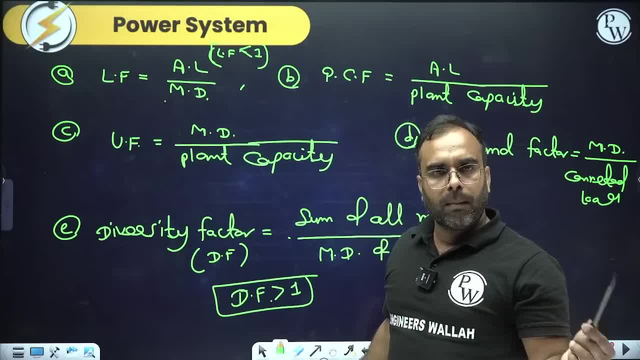 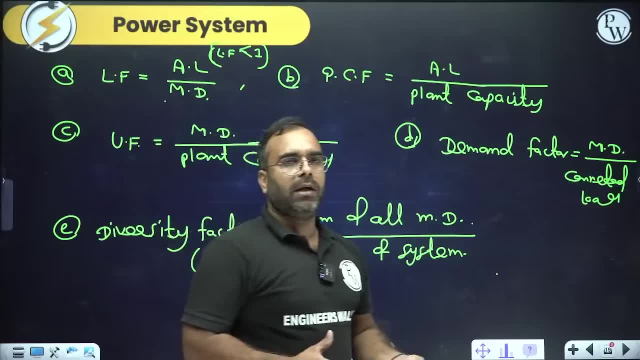 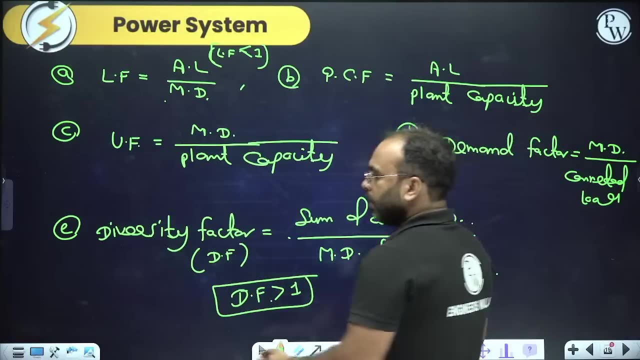 Then per unit generated cost will be low. So remember, if we ask the examiner To decrease per unit generated cost, What will we do Then? our load factor and diversity factor, Both values should be high, And after that I have written you the formula That here we had written, a formula. 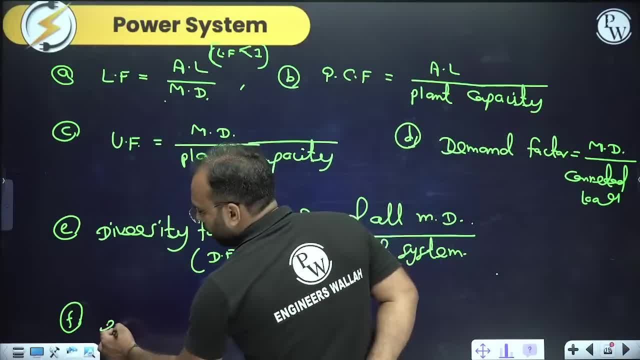 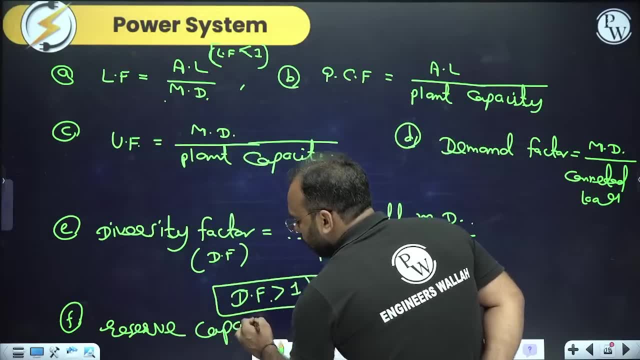 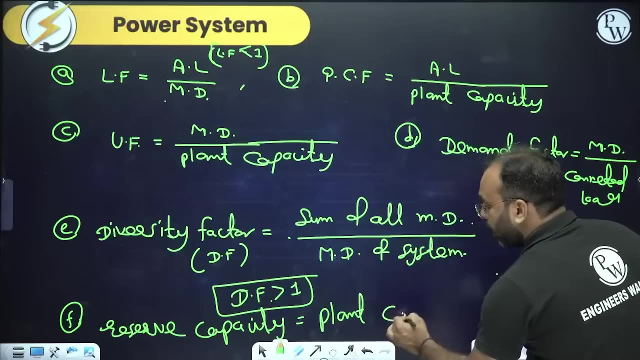 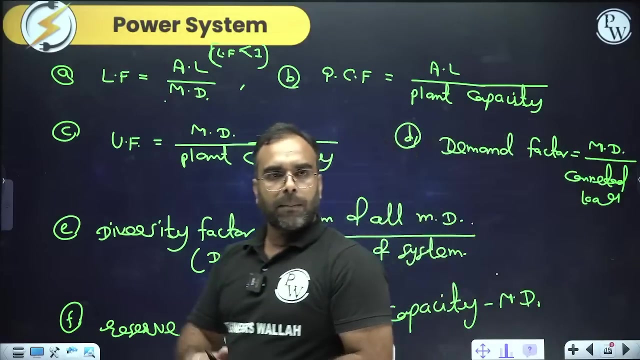 Reserve capacity. So what will come from here? Reserve capacity, So the reserve capacity will be with us. Plant capacity minus maximum demand. Plant capacity minus maximum demand. Tell me, I have told you so many formulas. Have we read too much? Tell me quickly, we had read this much formula till now. 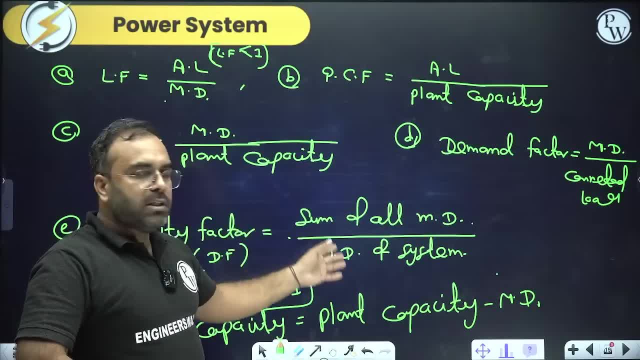 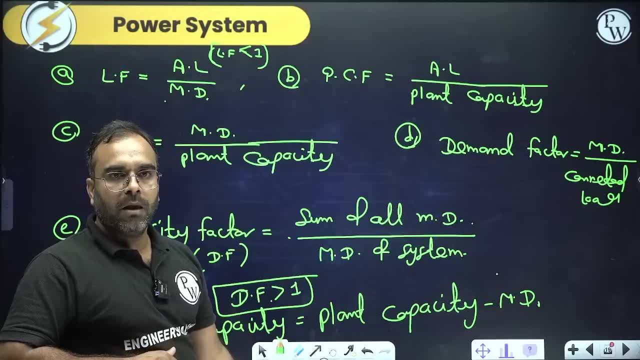 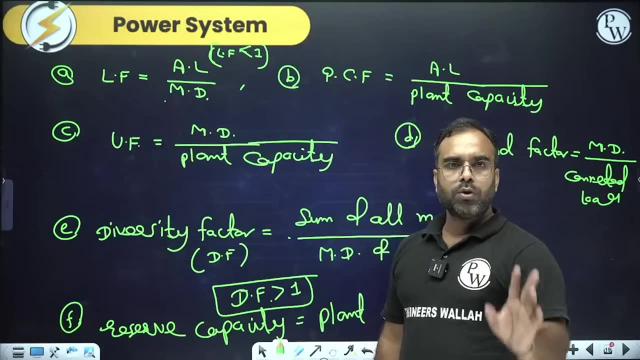 So this is what we have. You can remember it very easily. You can remember it very easily Understood. So you can see that we have read so many formulas. But keep in mind from here: Last year almost every paper had 2 questions. Means, if you have taken today's class, 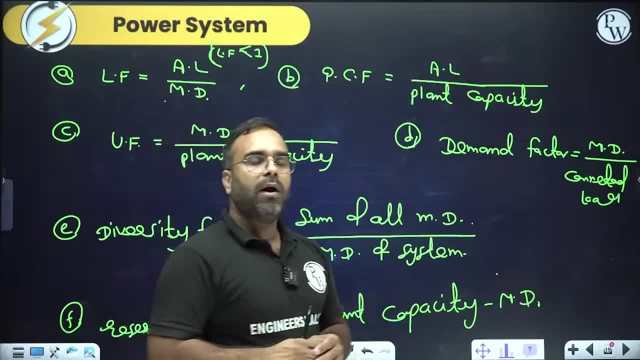 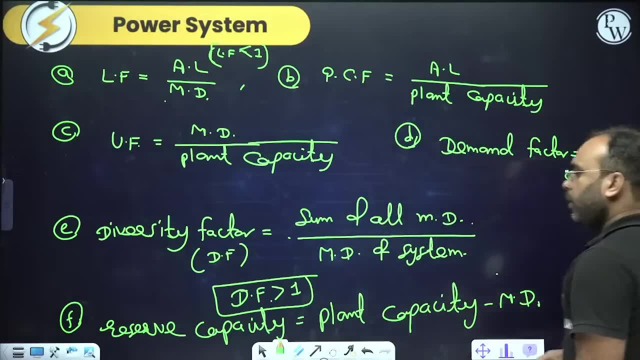 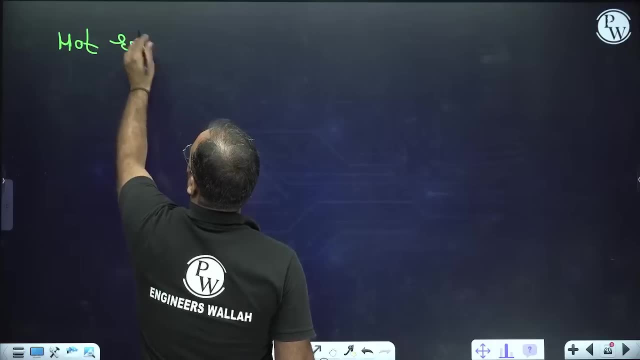 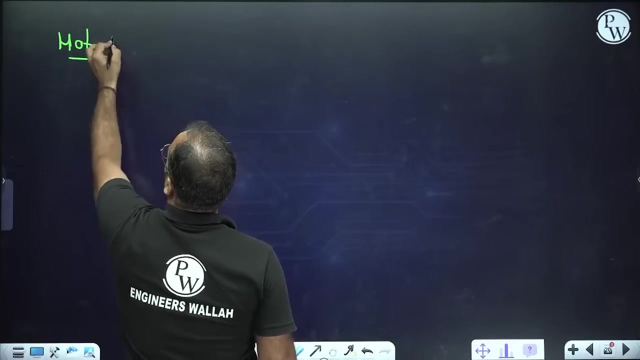 Then in today's class You have completed your 101% 2 marks. Now tell me quickly. Some definitions are asked to you here. It asks about HOT RESERVE, HOT RESERVE. Tell me quickly, If I ask you about HOT RESERVE, What is HOT RESERVE? 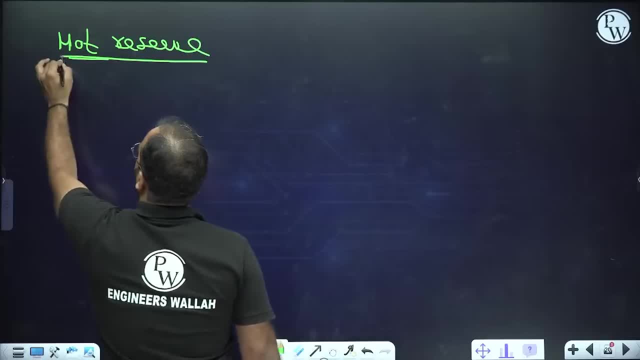 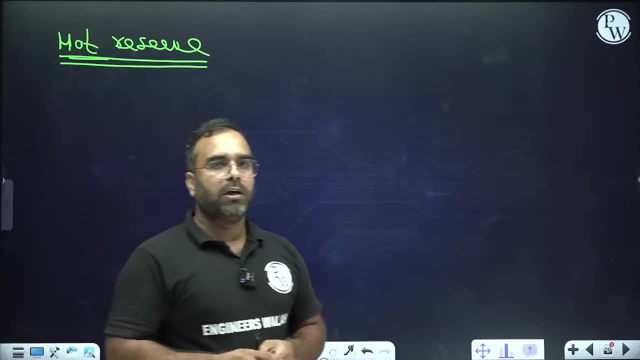 If I ask you, then what will be the answer? Tell me quickly What is HOT RESERVE? When will the class end? The class will end around 12.30- 12.30. You know that I teach almost 2 hours, So we- All of you who are new- 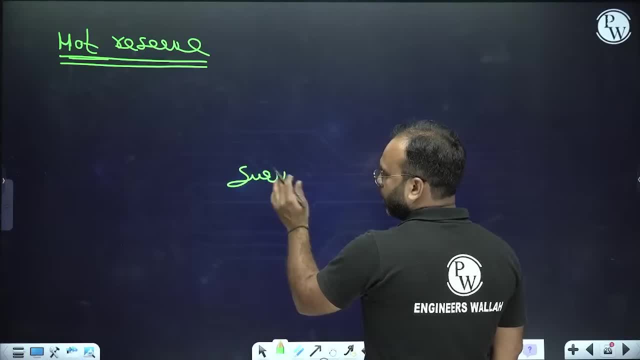 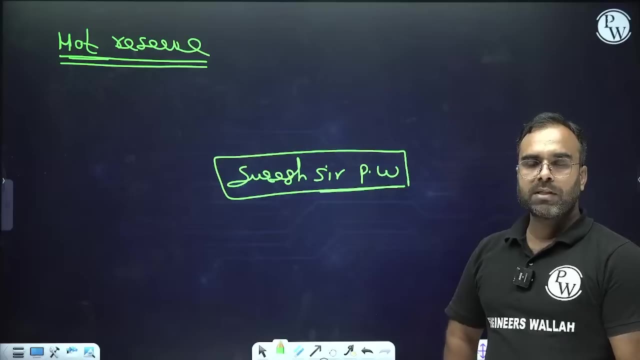 If you have any doubt while practicing any PowerStorm question, Then you can search on Telegram by the name of Suresh Sir PW And there, if you have any doubts, You can ask here. Power System Machine Measurement. If you have any doubt related to any subject, 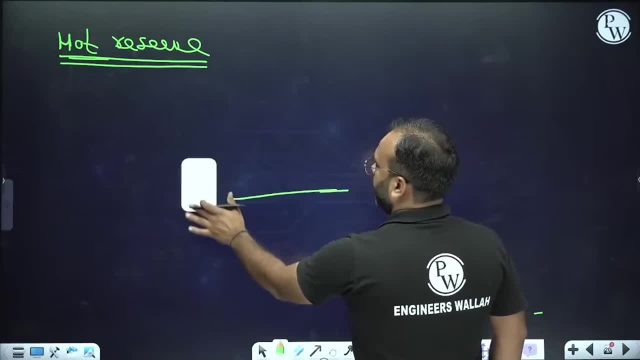 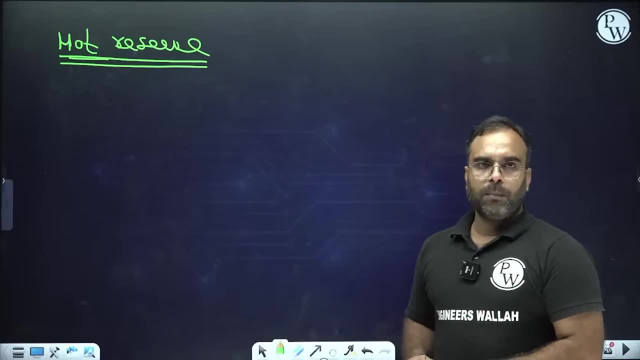 Then you can ask here And for PDF. You can download the application of PW from there, So you can join the group And you can download from there. Let's go Hot Pakode. So see here What is HOT: RESERVE: HOT means HOT What is HOT. 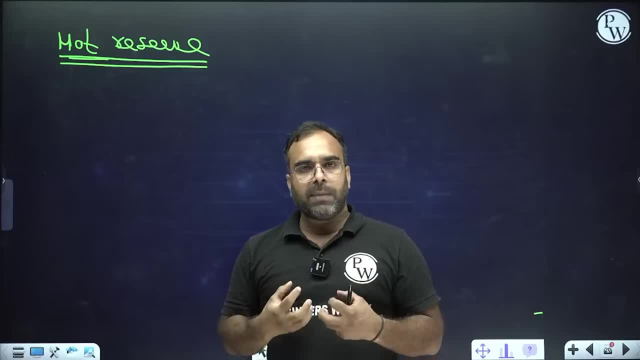 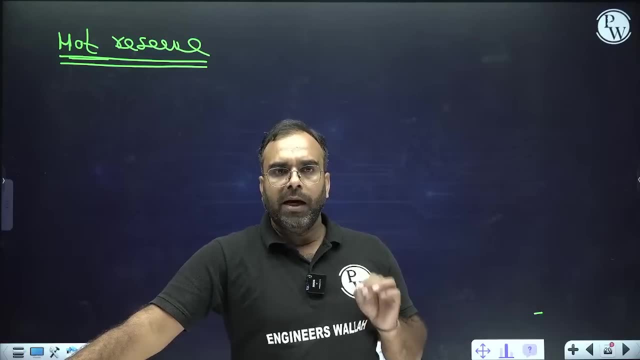 We have HOT and RESERVE. RESERVE means we have access. So what is HOT RESERVE? That means The excess of power which is ready to use, near boiler. Ready to use? How much is the excess available in our body? Ok, you will get it there. 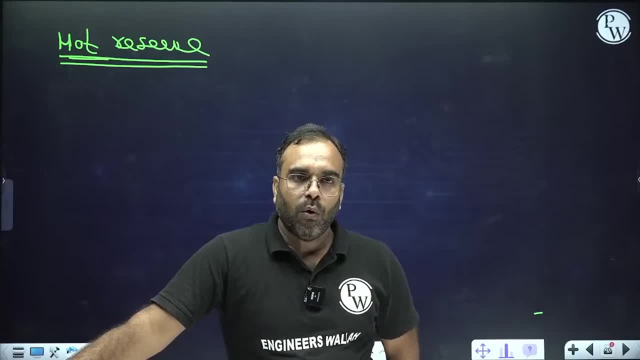 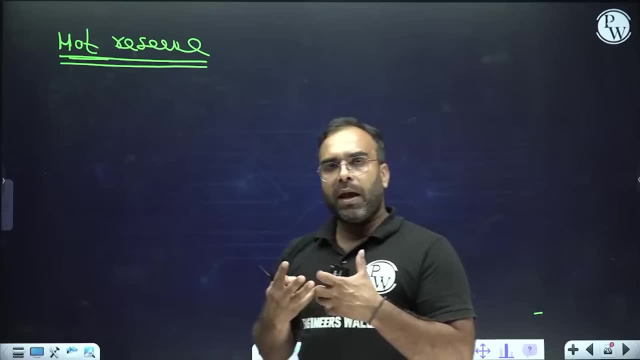 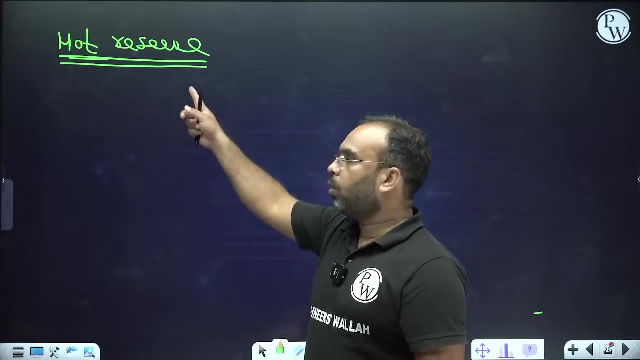 No problem, Let's understand What did I say. What is HOT RESERVE? That means If my load increases immediately, So the excess of power near boiler. If you have energy or power available which can supply the load, we call it hot reserve. It can be used on immediate loading also. 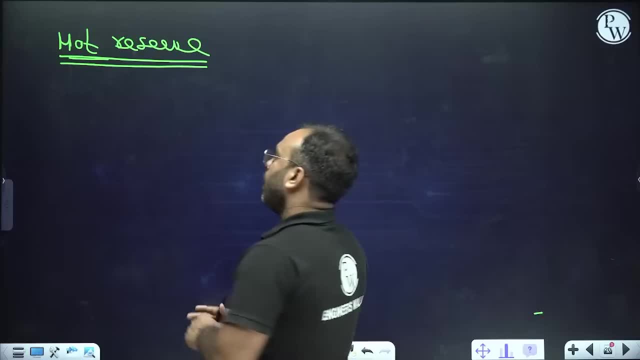 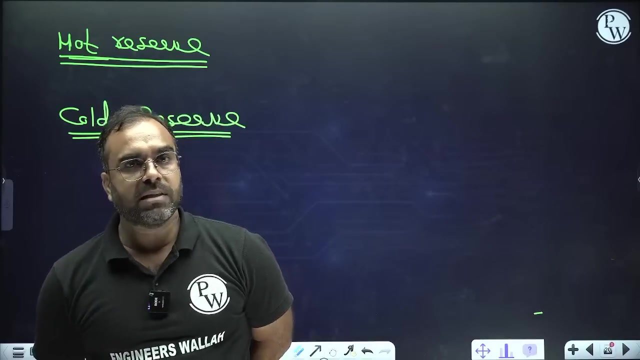 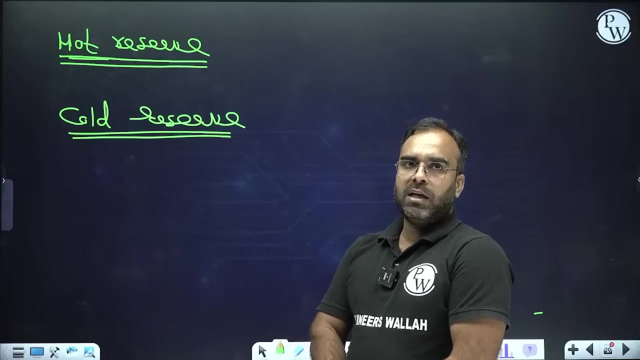 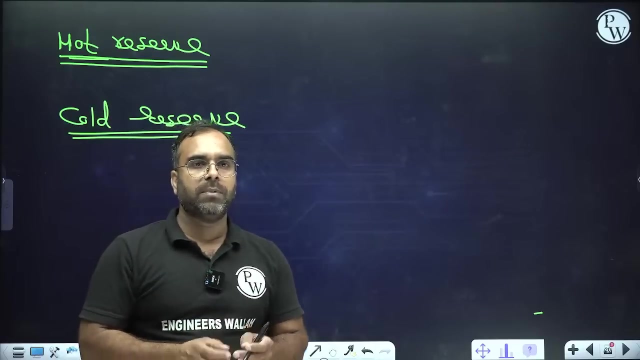 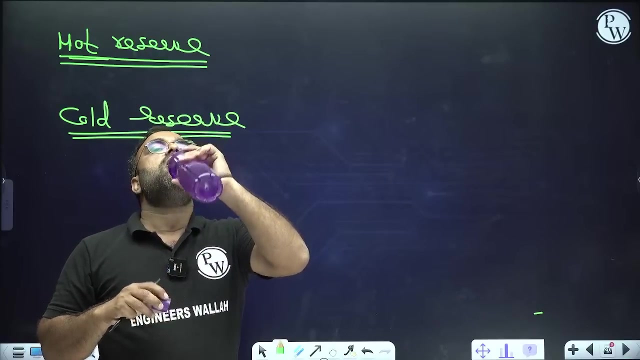 I will leave it on 12.30, no problem. Next, what is cold reserve? What is cold reserve? Yes, Rohit is correct, It is boiler capacity which is ready to take the load. What is hot reserve? It can be used on immediate loading also. 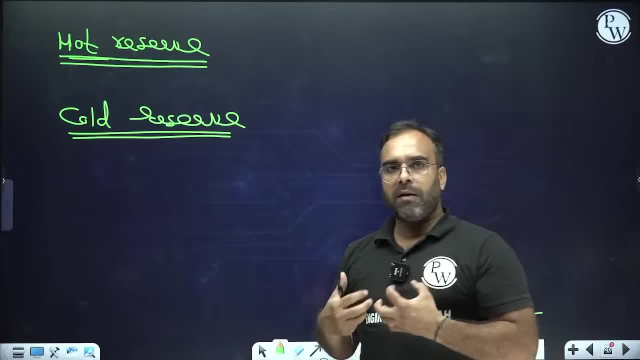 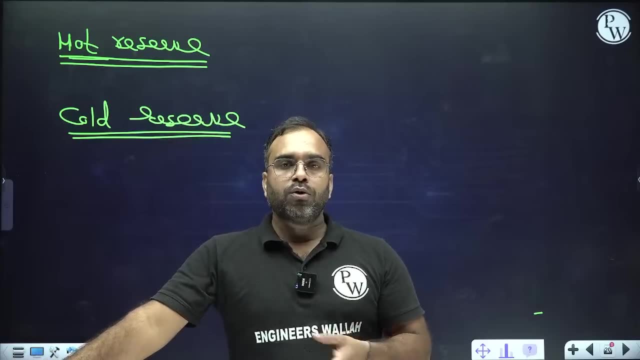 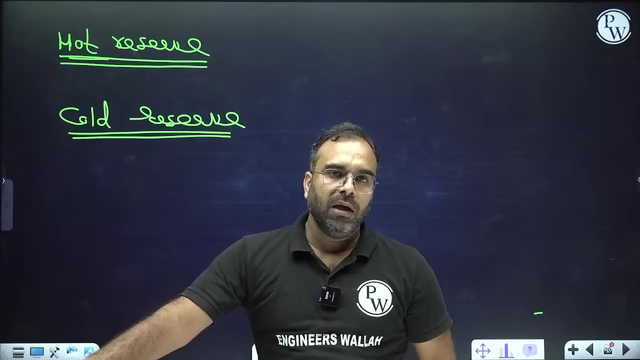 What is cold reserve? It is available. It is available, but I cannot use it immediately. I cannot use it immediately. To use it first, I have to take it to boiler and heat it there. After that we can use it. We call it cold reserve. 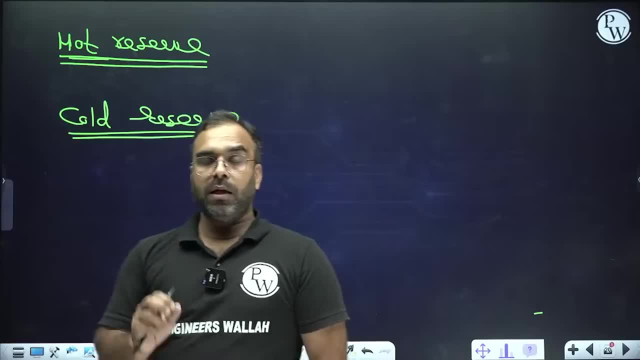 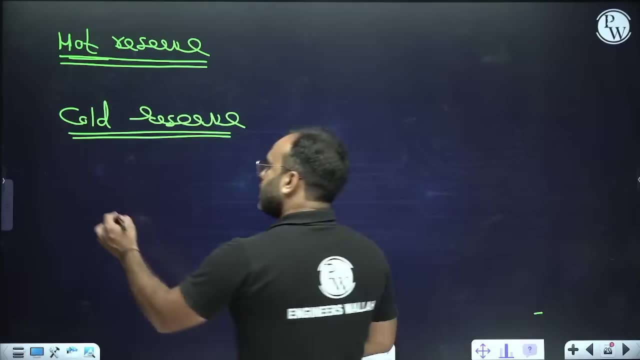 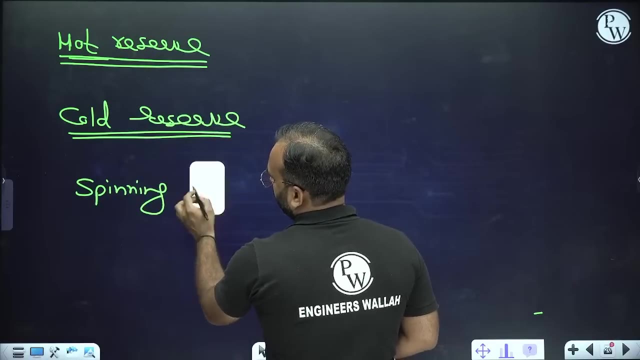 What is cold reserve? It is available, but not available for immediate use. So what will be available? It will be cold reserve. Next, What is spinning reserve? Tell me quickly What is spinning reserve. Tell me quickly What is spinning reserve. 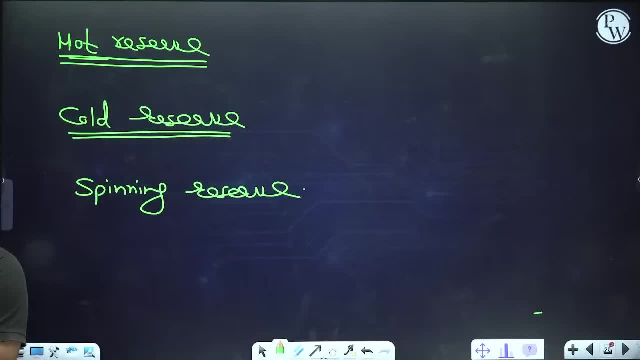 If you ask examiner what will be the answer. There are three answers. No problem, Join only three answers. Tell me quickly What is spinning reserve. What is spinning reserve? Tell me quickly The answer is: What will be spinning reserve. 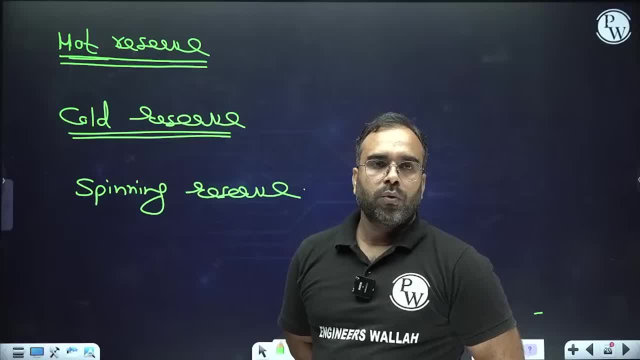 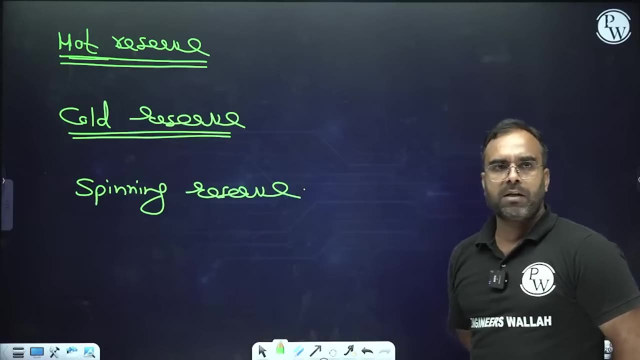 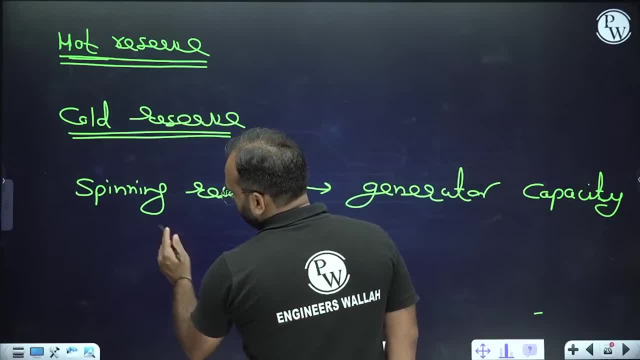 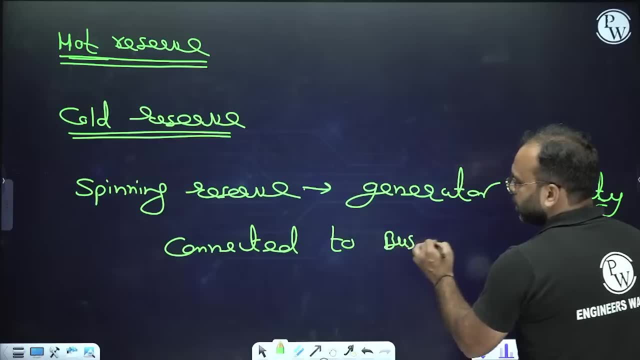 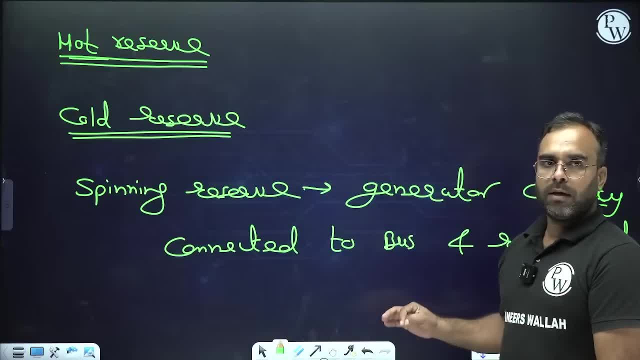 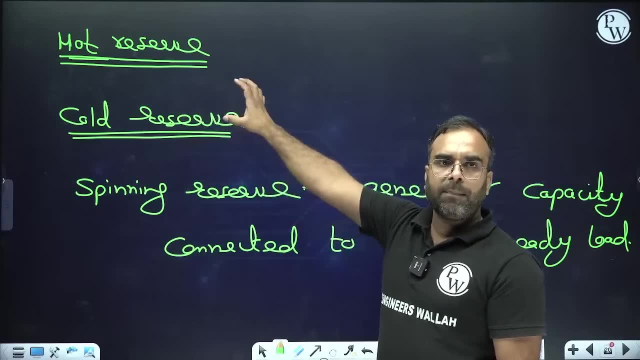 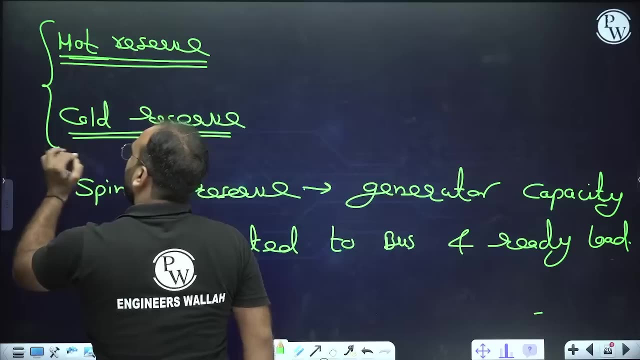 the generator's capacity? yes, it is in Alexa 3, correct. so this you can write. you can know something. what is spinning reserve? it is near the cold reserve, and hot reserve is near the generator or near the boiler. so here, keep in mind, it is near the boiler. 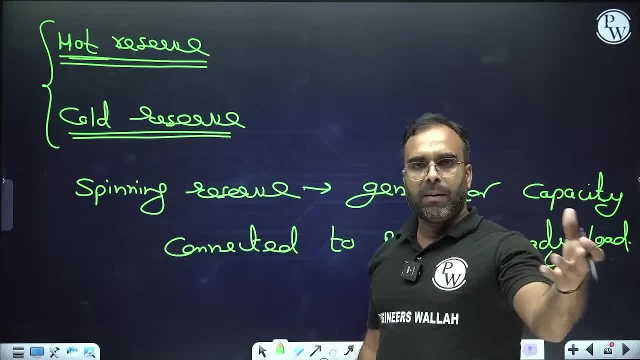 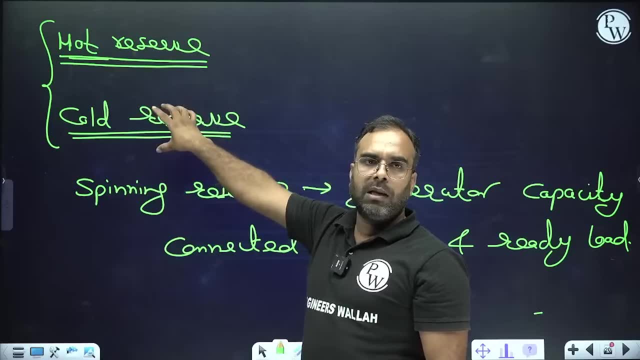 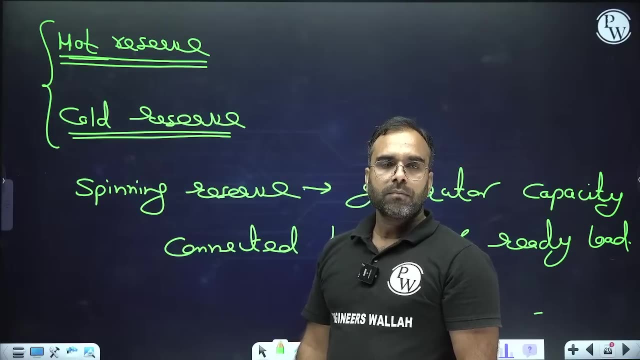 there is available capacity in the boiler or our available capacity in the plant, which has access near to boiler, which is ready to take load, but it is not available for immediate use. This is spinning reserve near the generator. understand, Yes, what is firm power? Emergency power? absolutely correct. 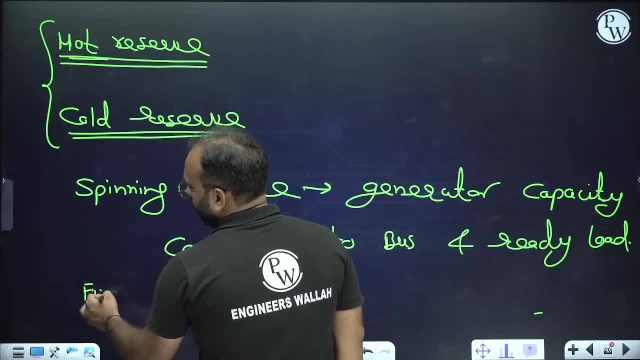 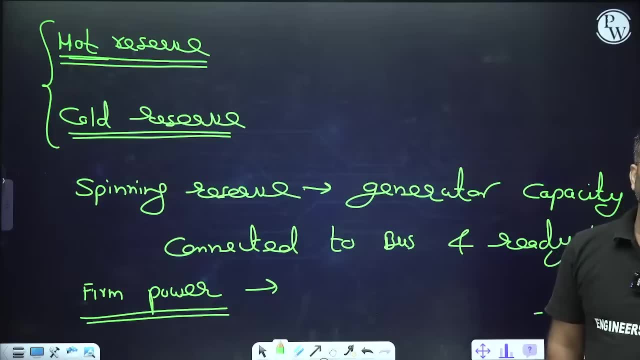 What is firm power? Tell me that too quickly. what is firm power? If the examiner asks you, tell me what is firm power, what is firm power, then what will be the answer? What is firm power? Tell me quickly what is firm power. If you are told that, what is firm power? 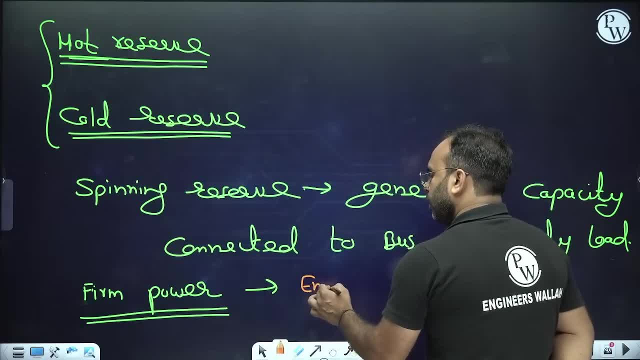 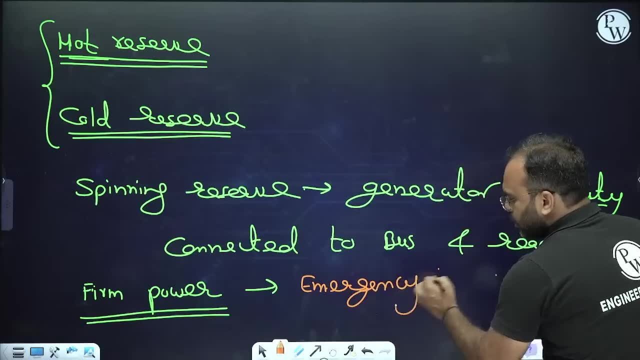 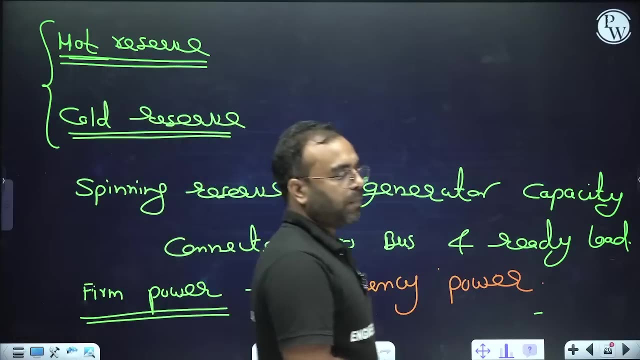 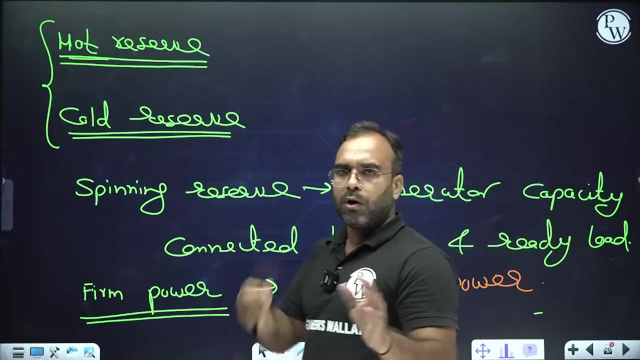 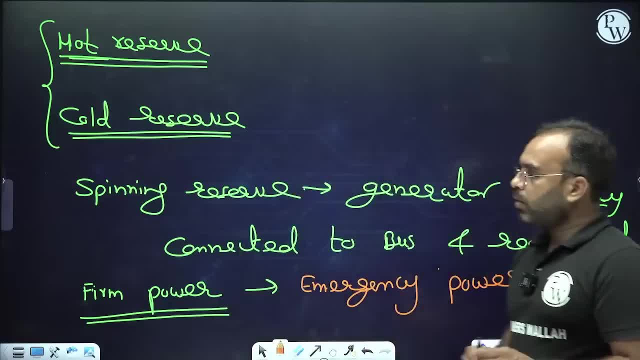 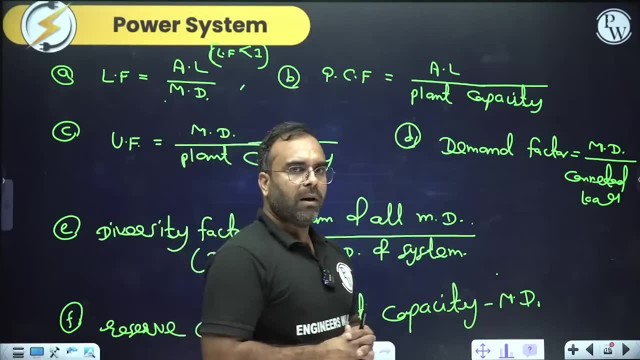 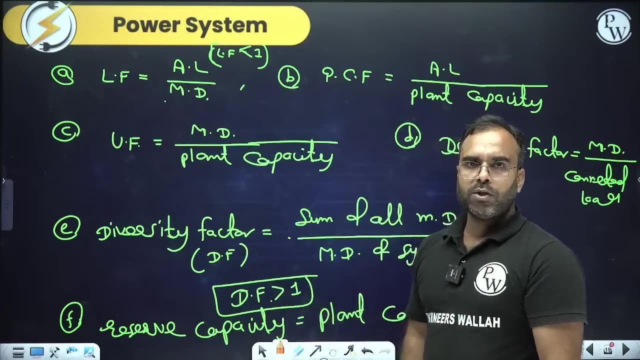 So if he will ask you, then according to me you will tell all the answers from here, And I am assuming that if you have given 2 hours, then if you have given 2 questions strong in 2 hours, then that is good, very good that you are securing 2 numbers 100% from here. 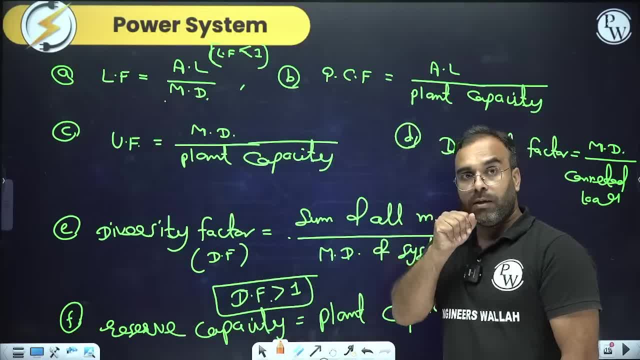 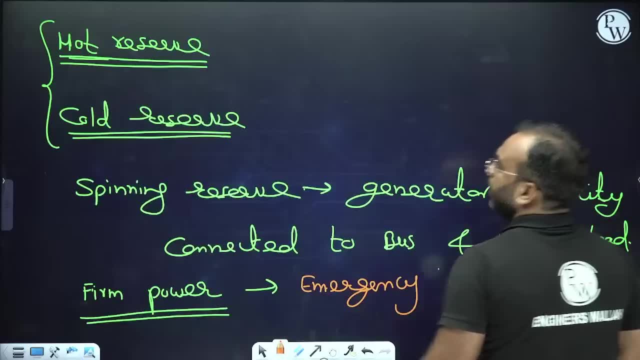 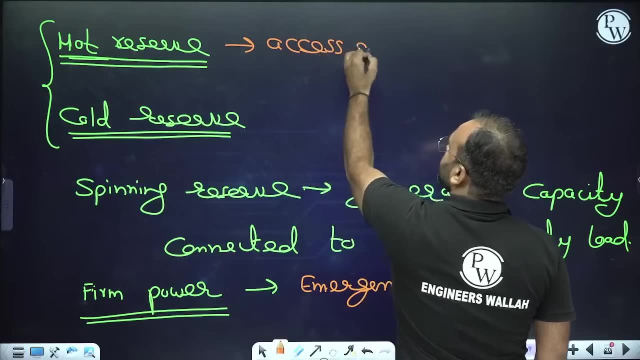 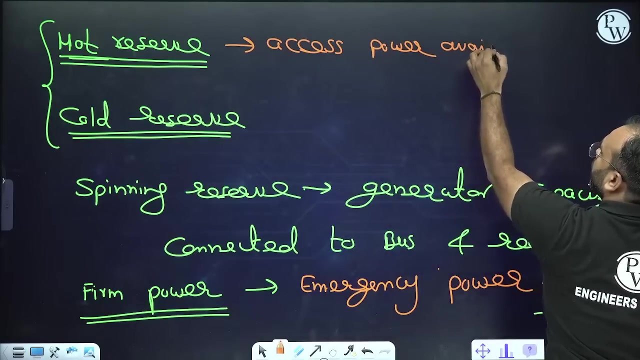 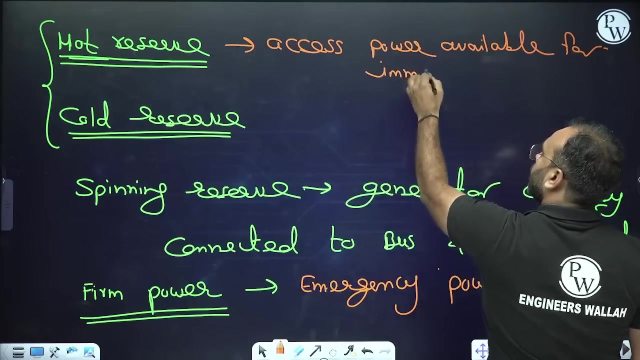 So I will teach PowerStorm in the same way. sorry, where most of the questions are asked in exams. Sorry, where most of the questions are asked in exams, So I will teach PowerStorm in the same way. sorry, where most of the questions are asked in exams. 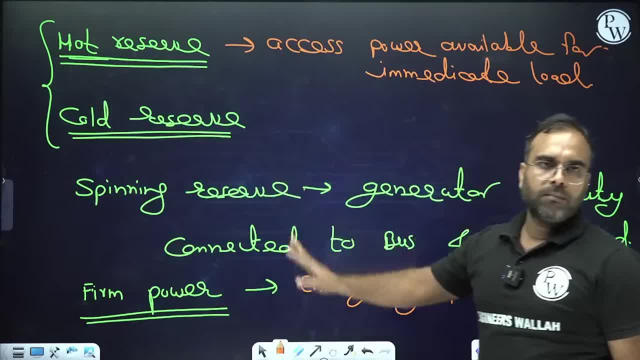 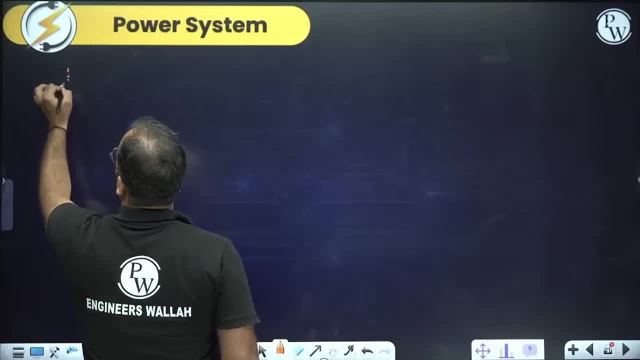 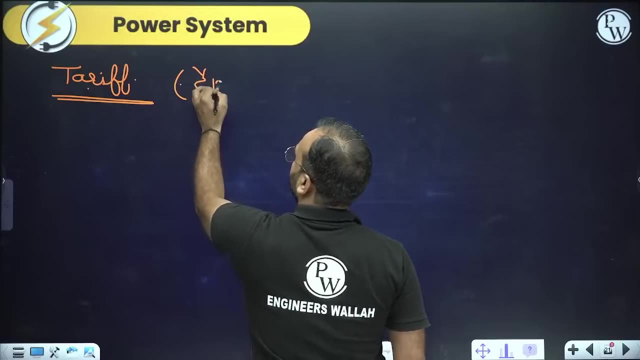 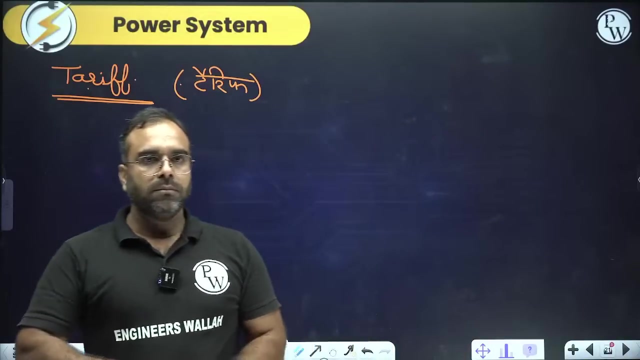 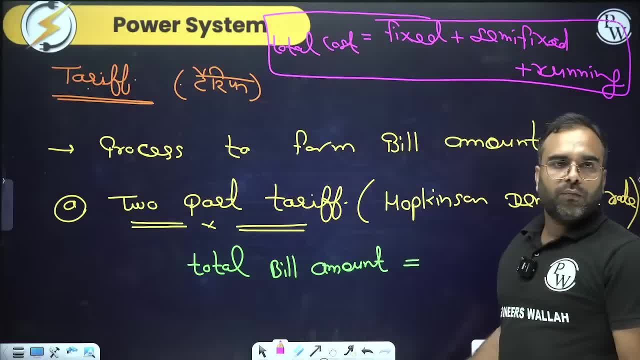 So I will teach PowerStorm in the same way, sorry where most of the questions are asked: in exams. So I will teach PowerStorm in the same way, sorry, where most of the questions are asked in exams. What are the two cost summations of two part tariff? 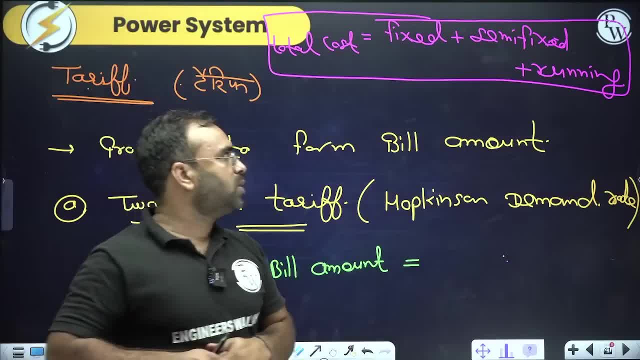 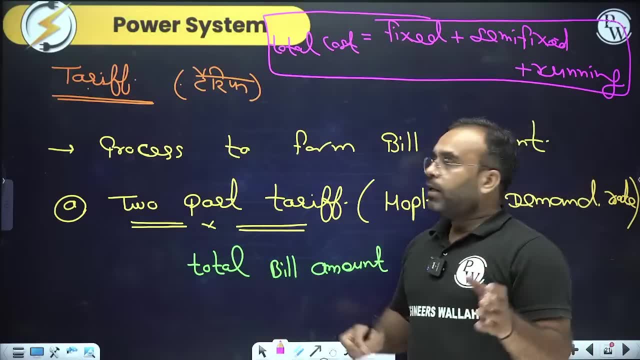 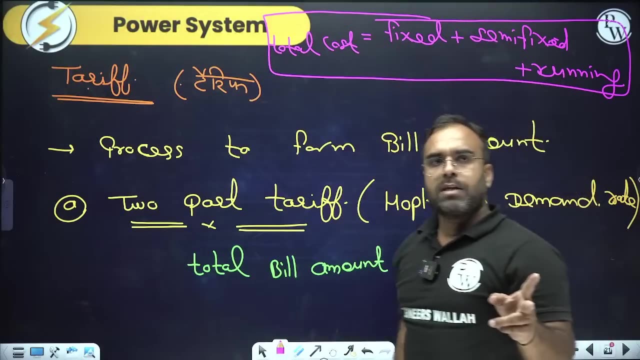 The answer is fixed and running cost. Tell me quickly: fixed and running cost or semi-fixed and running cost? Here the answer is some variation. These three are total cost, But I am talking about two part tariff. What are the two cost summations of two part tariff? 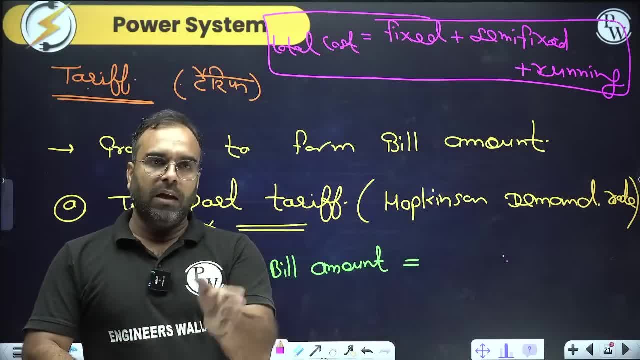 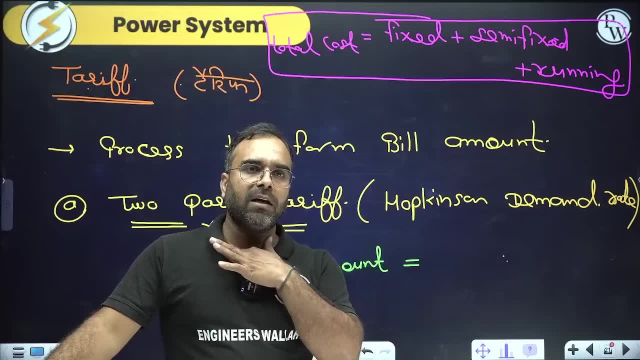 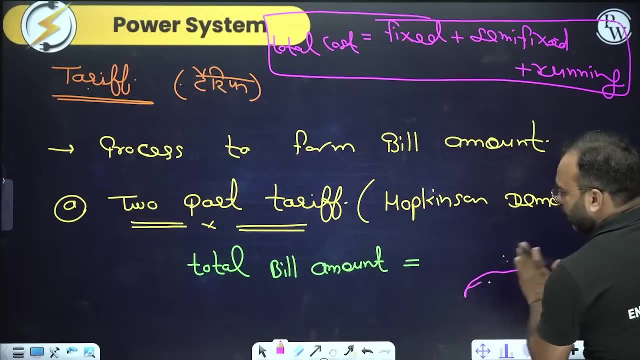 Fixed cost or semi-fixed, Or fixed and running Or semi-fixed and running. What is the answer? Because half of the answers are fixed and running, So the answer is semi-fixed and running cost. What are the two part tariff, Semi-fixed cost plus running cost will be the summation of both. 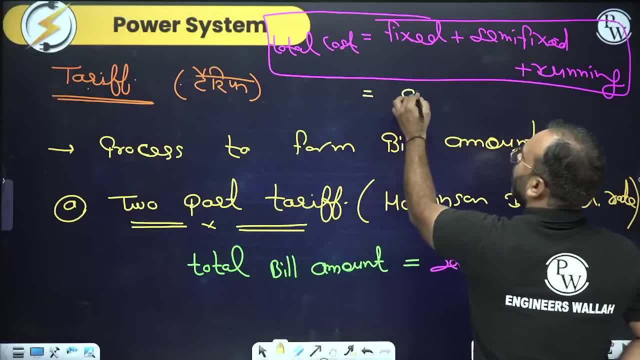 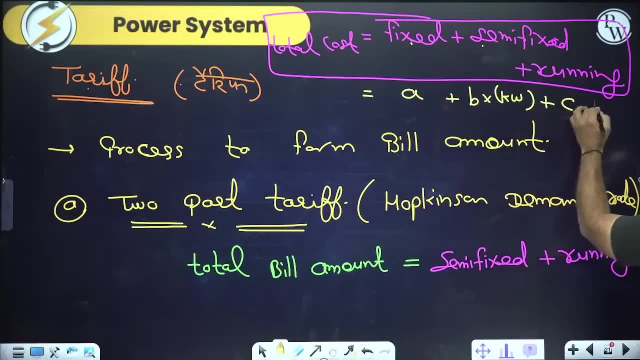 And you may know that the total cost of these three is: We write fixed cost and semi-fixed cost, We write B into kilowatt And here we write C into kilowatt hour. Keep this formula in mind in your SSE JEE last year also. 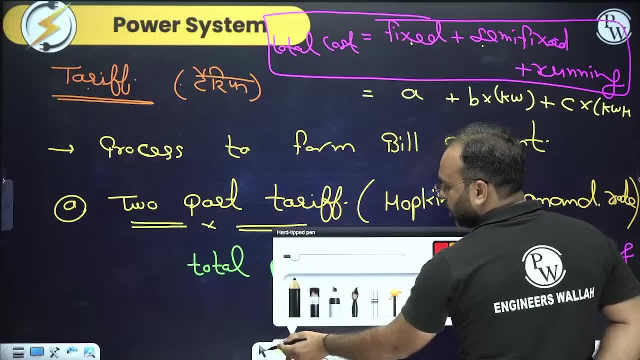 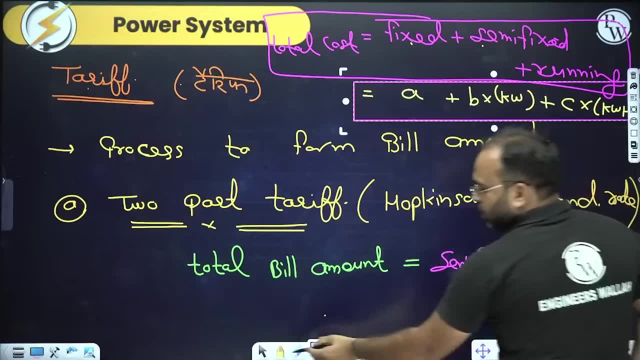 Last year also, SSE JEE had a question from here From this formula: Put this formula in bracket. This is an important formula. This formula is important From where the question came last year also in the exam: A plus B into kilowatt, plus C into kilowatt hour. 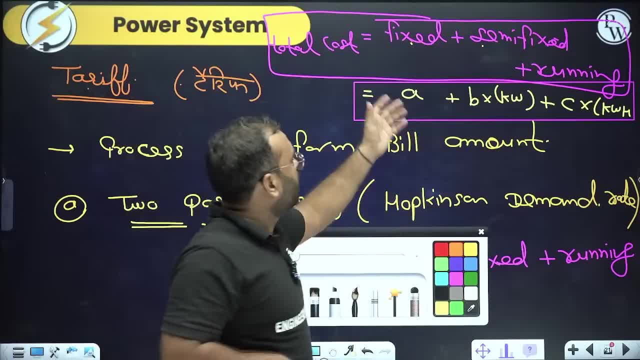 Now, what is this? A, B, C? So last year they did not ask anything. That the total cost is this much. Tell me how much will be the unit of B Or how much will be the unit of C. Tell me quickly what is the unit of B. 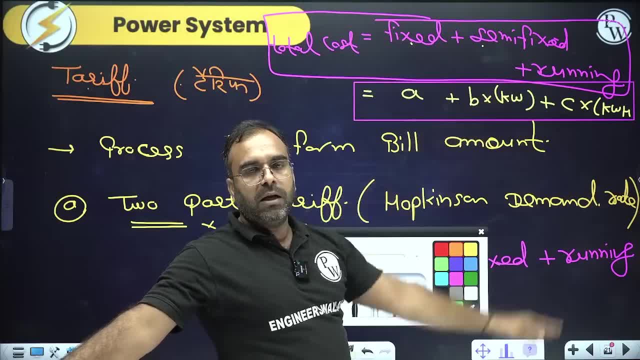 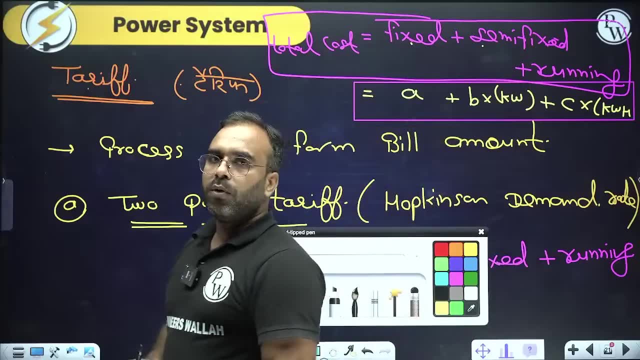 The examiner will ask you the unit of B or C in the exam. What will be the answer? Here I have written B or C. What will be the unit of their unit? What will be the unit of B? So keep in mind that this is in money. 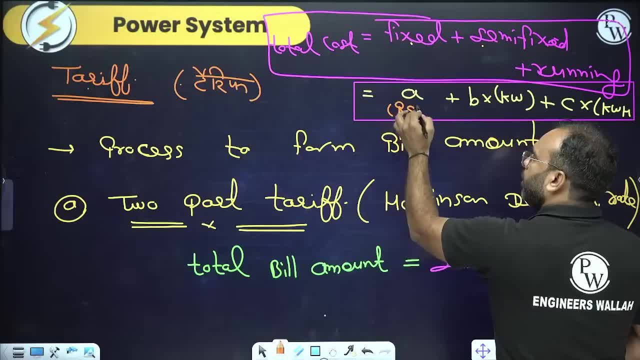 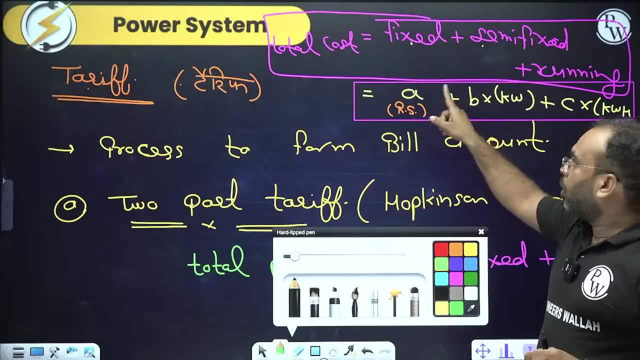 In Rupees Money, Because you know that you have to give money in the bill. So the unit of B here. See, I can add Rupees in Rupees. This should also be Rupees in Rupees. So what will be the unit of B? 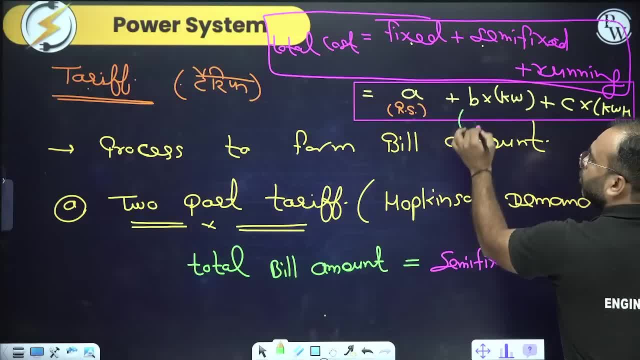 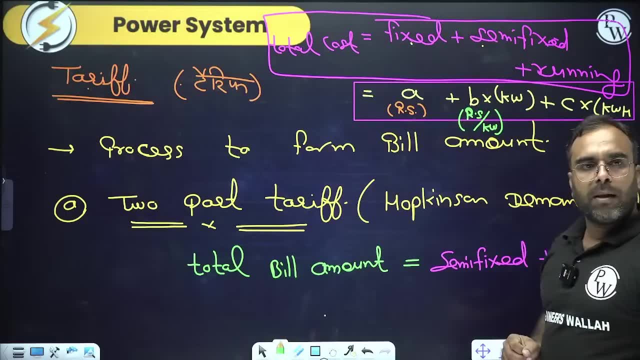 Rupees per kilowatt. So kilowatt will be cancelled from kilowatt, So the unit of this will be RS Rupees per kilowatt. So when you multiply it by kilowatt Then our Rupees will be saved. 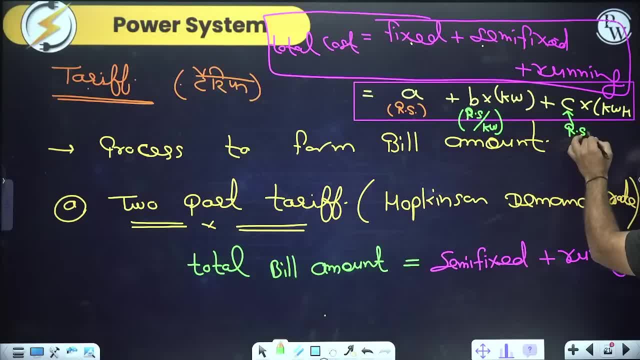 What will come in C here. So keep in mind that the unit of C will be Rupees per kilowatt hour, Because here we are multiplying by kilowatt hour, So the energy of kilowatt hour will be cancelled. Okay, 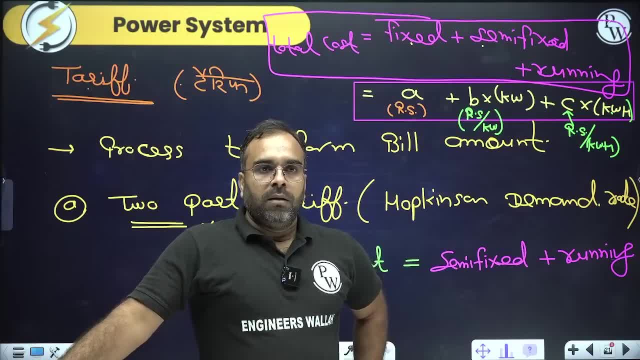 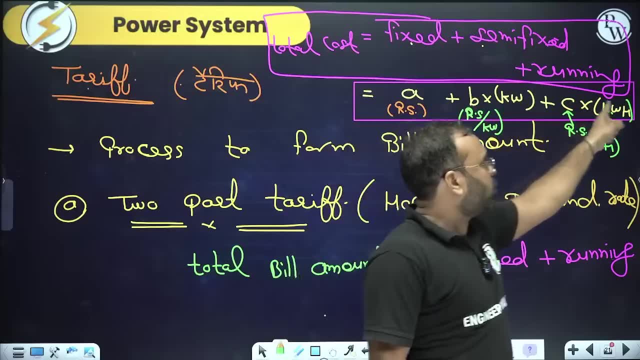 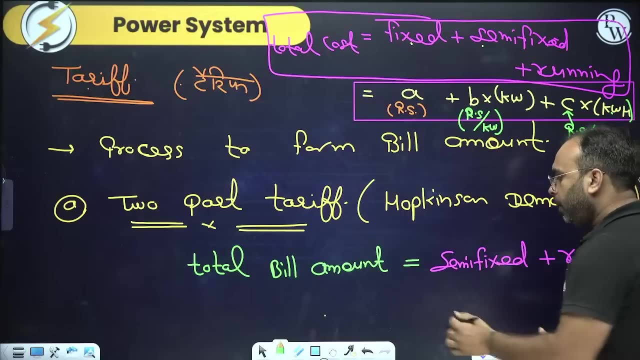 Understood. So see here this unit. Remember that A is B into kilowatt And C into kilowatt hour. But here we have two part tariff. In Hopkinson demand rate tariff The total bill that is made. That bill is our B into kilowatt. 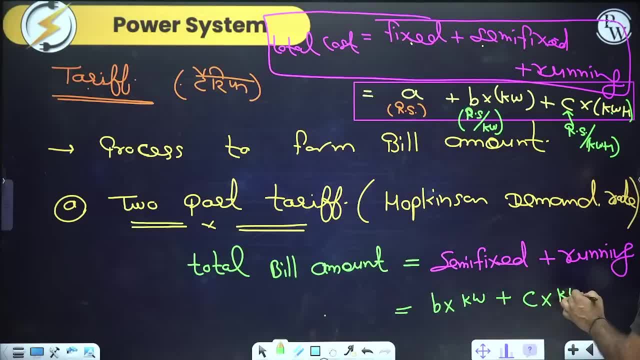 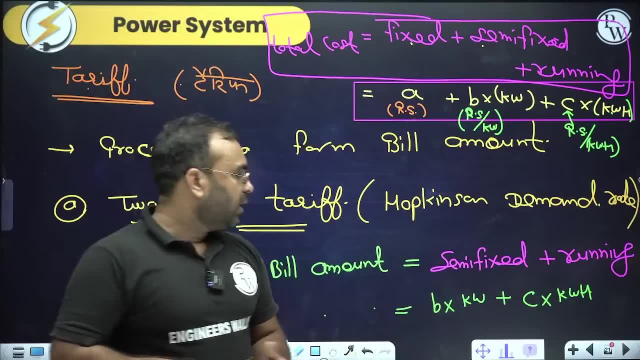 Plus C into What will be with us- Kilowatt hour That will be made with us. So this will be our total bill. Total bill amount. What did I say? This will be our total bill. amount B into kilowatt. 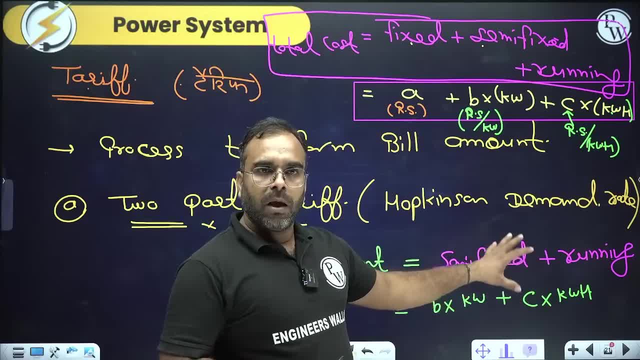 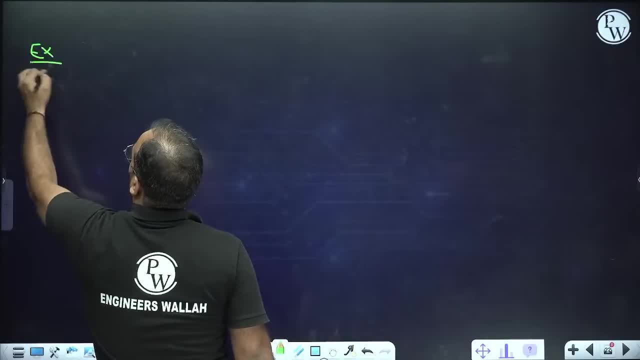 Plus C into kilowatt hour. Now see what numerical will ask. What numerical will ask. Numerical examiner will ask you such a question here. You will be told in a two part tariff. You will be told in a two part tariff. 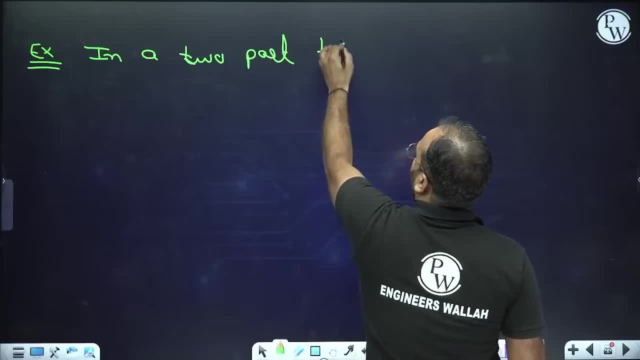 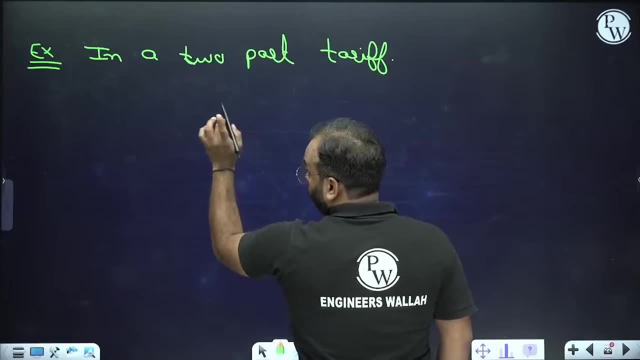 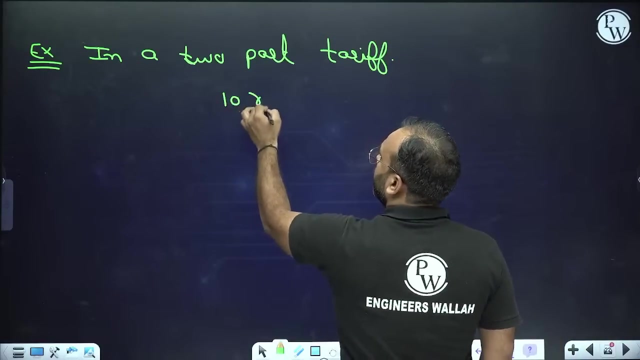 Two part tariff. Two part tariff is Two part tariff. You will be told in two part tariff, biblical tariff is That we have two constants. We will decide the bill with respect to two. cost ten rupees per kilowatt. 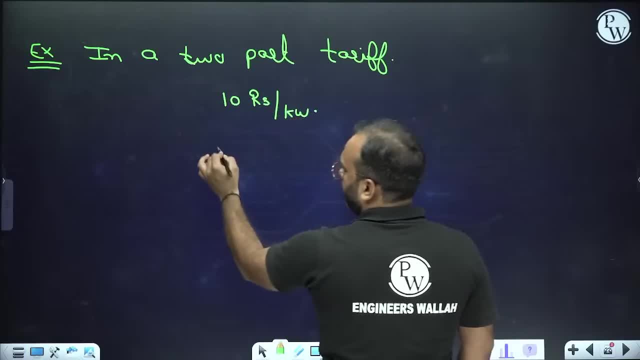 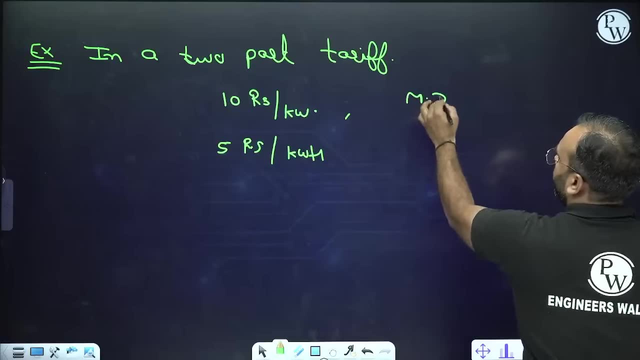 And five rupees per kilowatt hour And it will be told from you. Maximum demand of our system is that hundred kilowatt And the unit that we consumed. we have consumed 200 units. Tell me how much will be the bill. 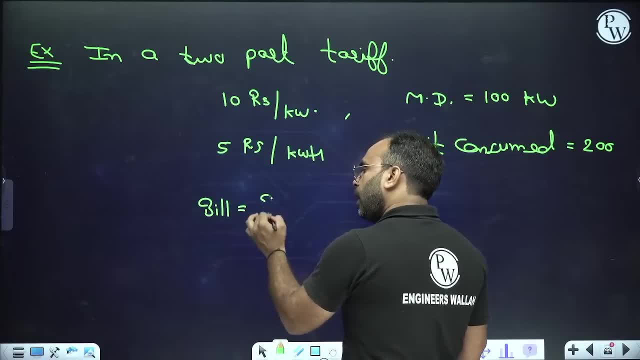 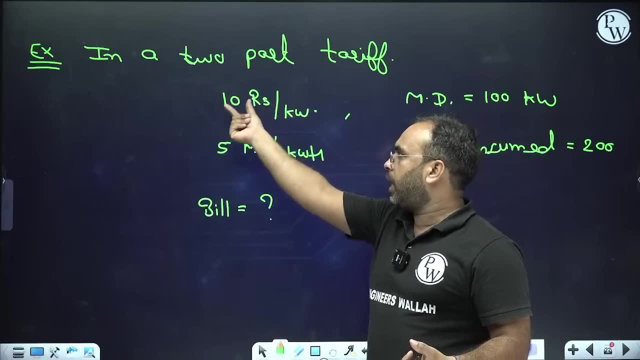 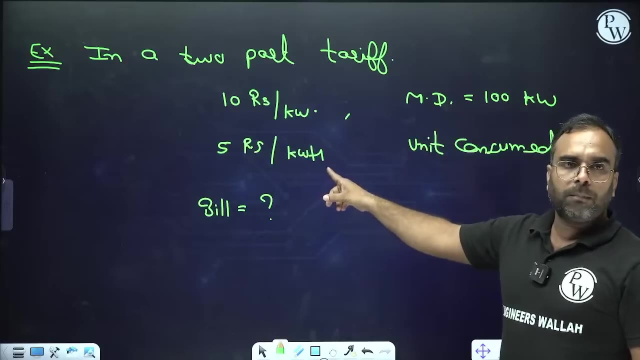 You will be asked an examiner question. I have written in short language. The examiner will tell you that in two-part tariff we will decide the bill amount. in this respect, We will take 10 rupees per kilowatt, per kilowatt of maximum demand and 5 rupees per kilowatt hour. 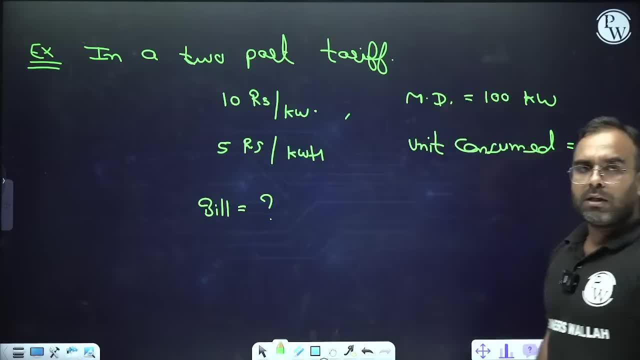 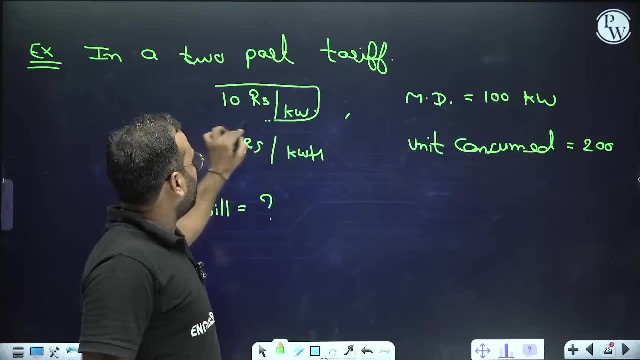 And he will tell you that the maximum demand is this much and the unit is this much. So he will ask you: tell me how much will be the bill. If you ask such a numerical, then keep in mind that I said that this unit is B and this unit is C. 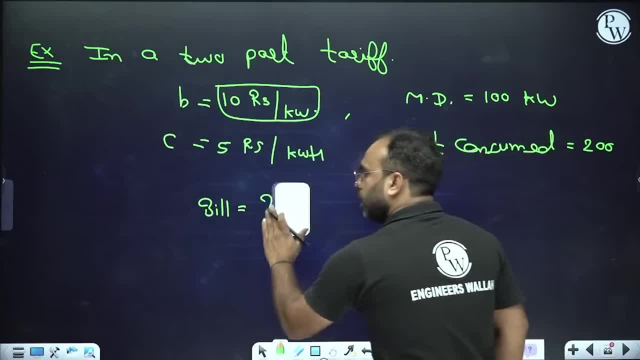 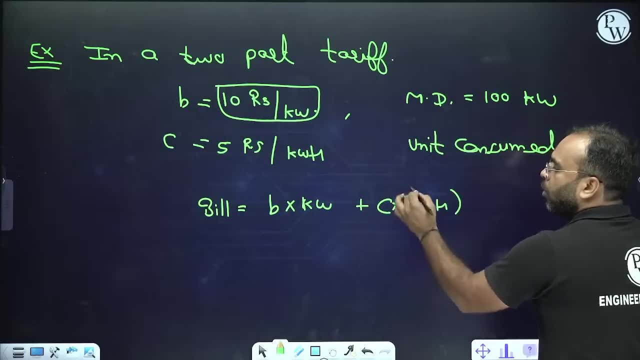 So if you want to decide the bill, then to decide the bill you will do B into kilowatt and plus C into kilowatt hour. This is what I mean to say. Kilowatt hour means unit energy. So what will be here? How much is B? We have 10 B. 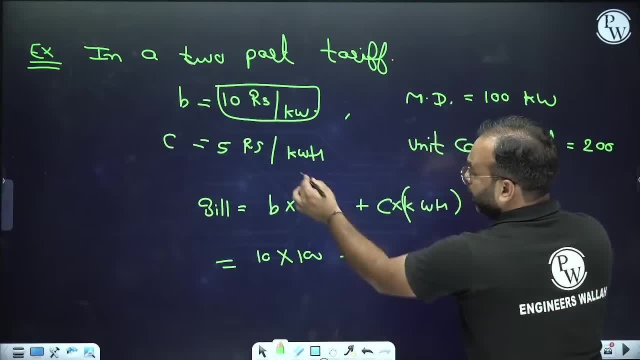 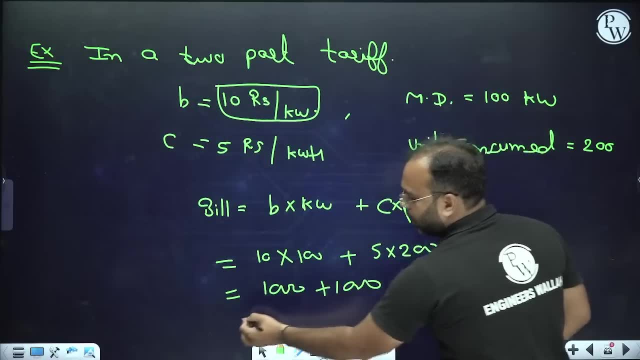 And kilowatt hour. How much is kilowatt 100.. How much is C 5.. And how much is kilowatt hour 200.. So from here, 1000 plus 1000, that is the bill of our house of 2000, will come, which is almost this much. 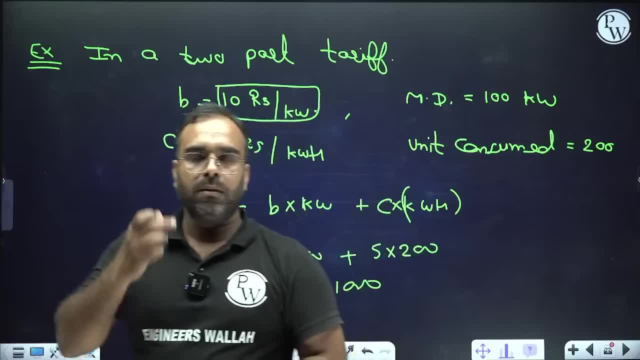 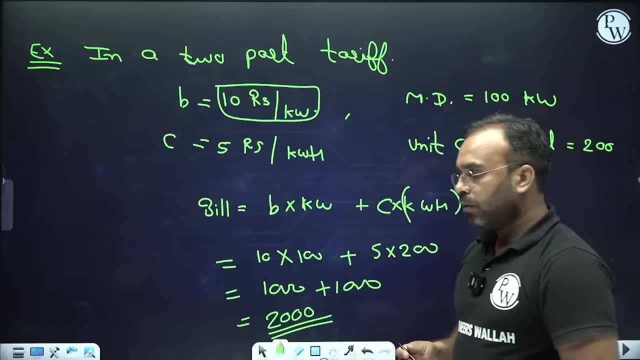 Got it, Ram. there is a software through which you can change the background. I will share its link in the group today. I had shared it earlier, So you can change the background. It will be white instead of black. Then you can print it out. 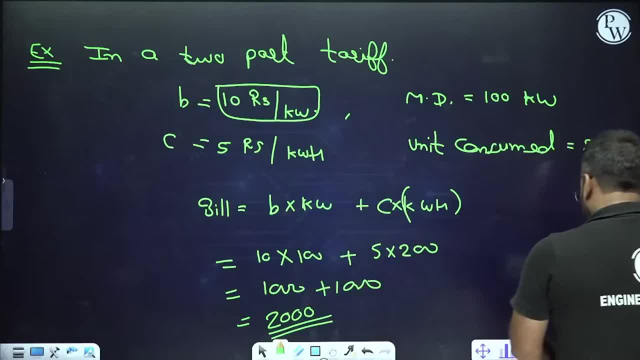 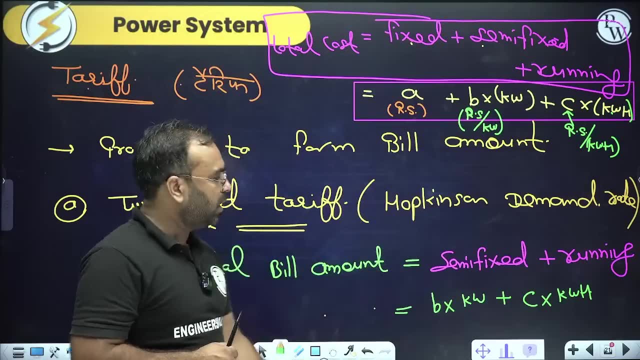 So what will we have? The answer will come: If you ask such a numerical, you will do it. If you ask such a numerical, you will do it. So sometimes, if you ask that Hopkinson demand rate tariff or two-part tariff, what is the sum of the costs? 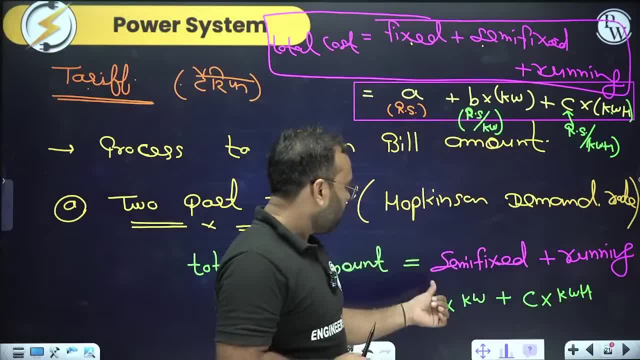 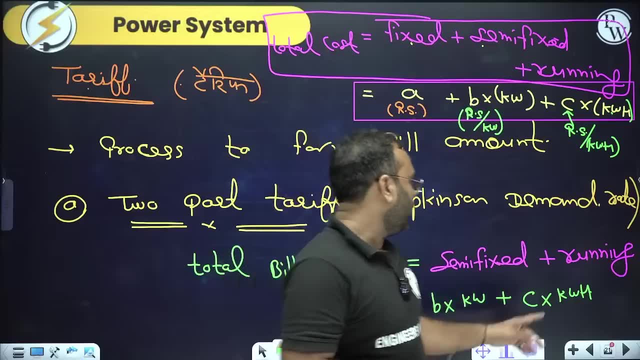 So there is a sum of family fixed and running cost in which we write B into kilowatt plus C into kilowatt hour. Okay, Kilowatt hour, Kilowatt hour. Kilowatt hour is written: See Here in the numerical. write it in this. 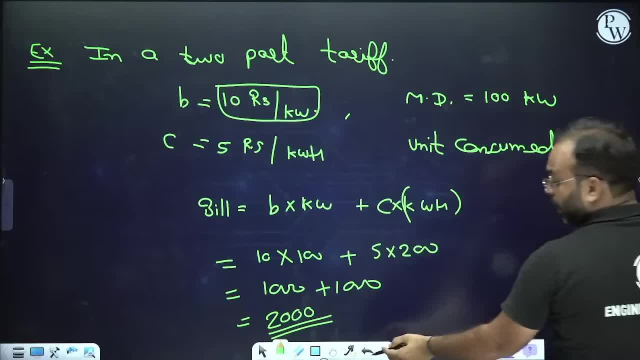 This kilowatt Here. it is said that I did not write it here in C. See, the unit is written here. Unit means one kilowatt hour. One kilowatt hour. Come on next. After this we will talk. 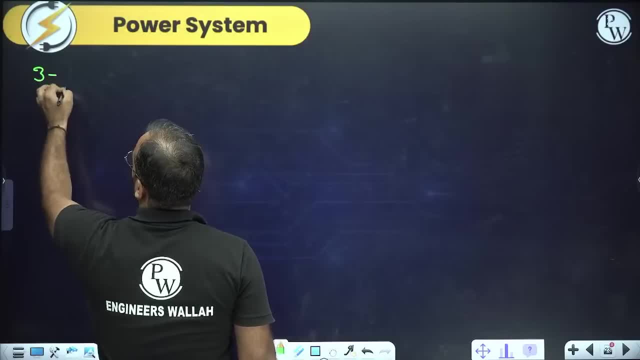 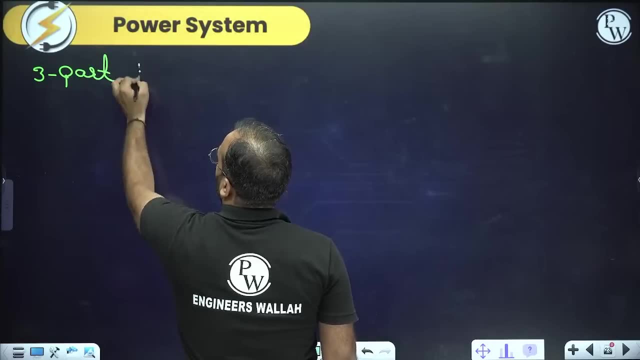 Next will be three-part tariff, Three-part tariff. Come on, tell me quickly What is the sum of three-part tariff. So here three-part. So here three-part tariff will be. Three-part tariff, Three-part tariff will be. 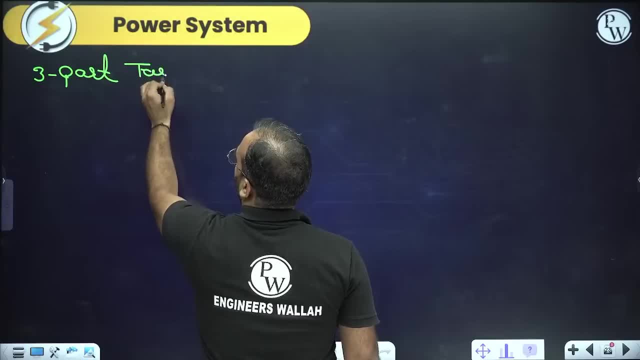 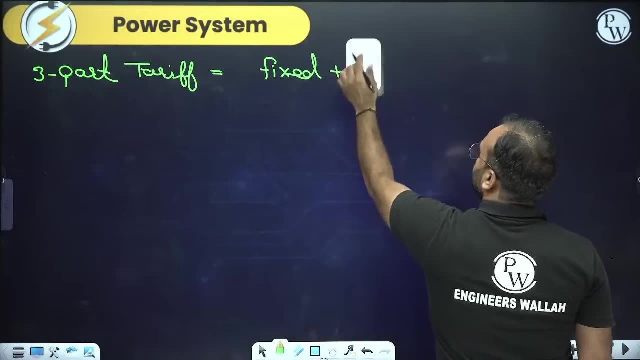 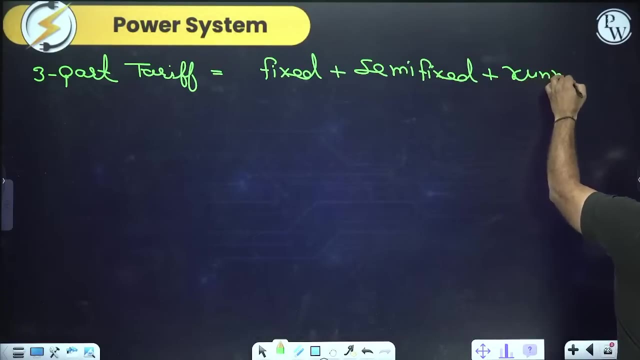 Three-part tariff will be The sum of three-part tariff will be three cost: One will be fixed, The other will be semi-fixed, Semi-fixed and the third will be running cost- Running cost. So what will we have? This whole overall formula is made. 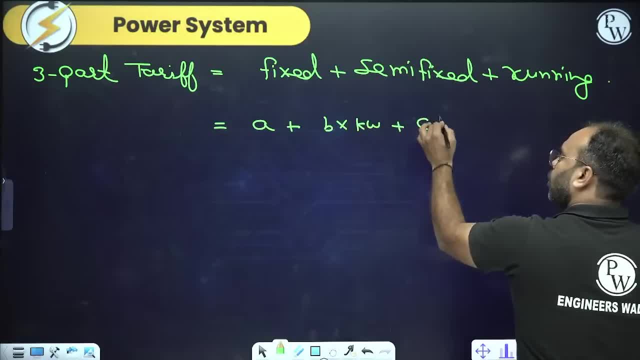 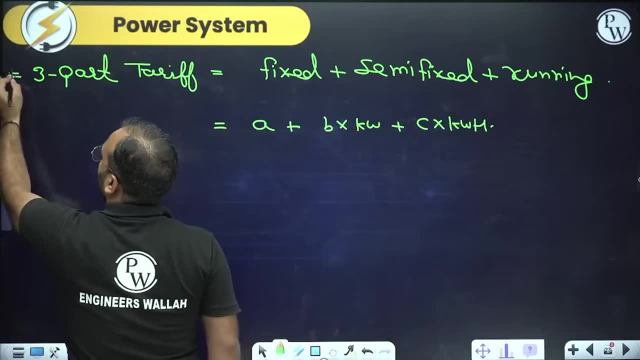 A plus B into kilowatt, plus C into kilowatt hour, and this is the formula of 3 part tariff. this is the formula of 3 part tariff, but keep in mind what is the other name of 3 part tariff? tell me quickly. 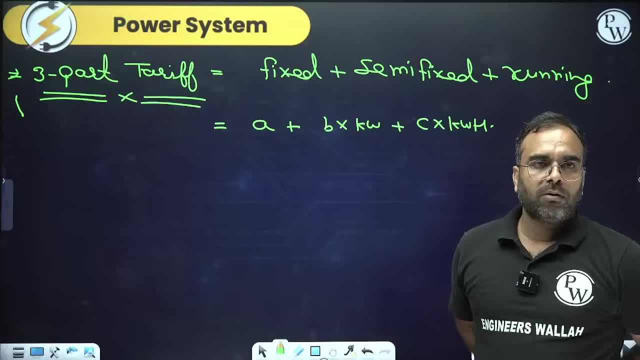 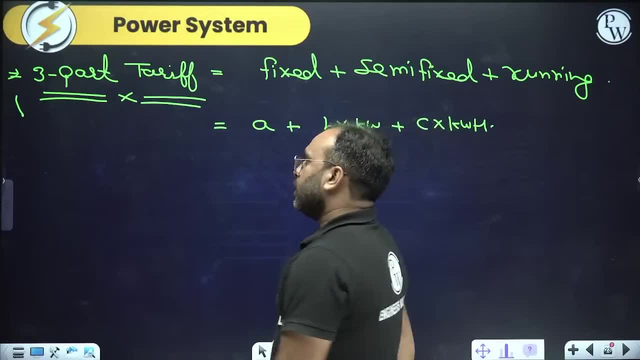 what is the other name of 3 part tariff? what is the other name of 3 part tariff? before asking me, you have told me you know my feeling, dotty rate is correct. so write here that one more name of this will be dotty rate, dotty rate. 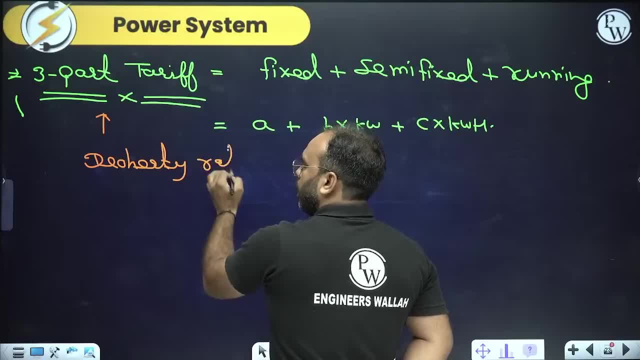 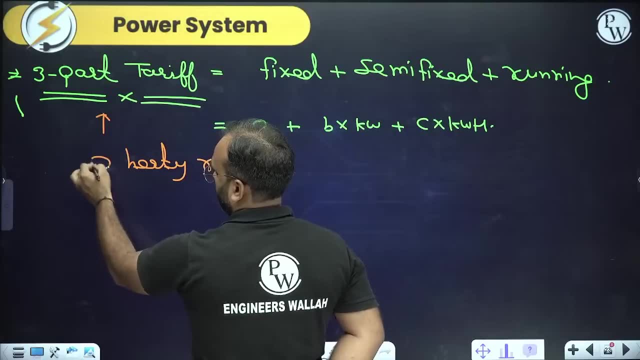 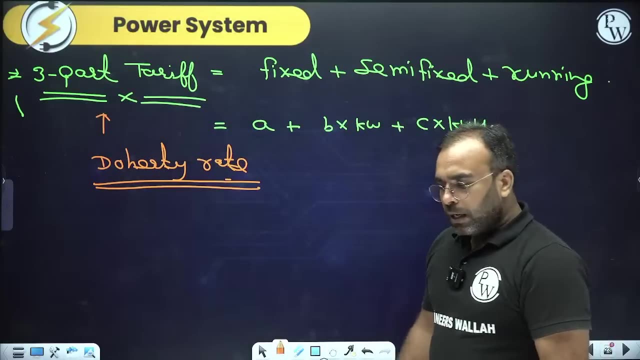 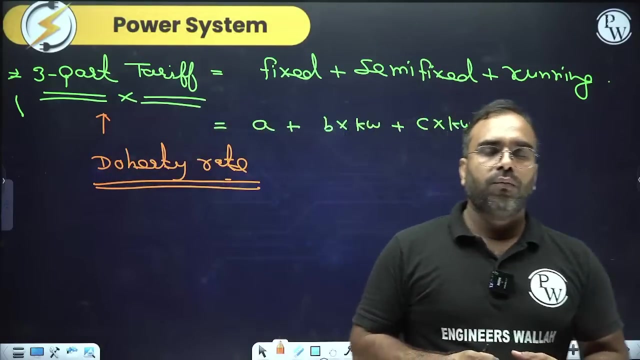 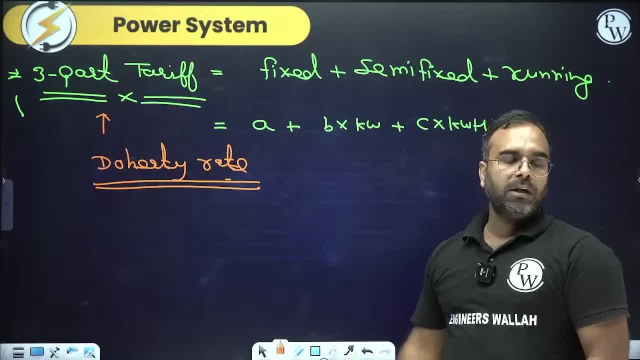 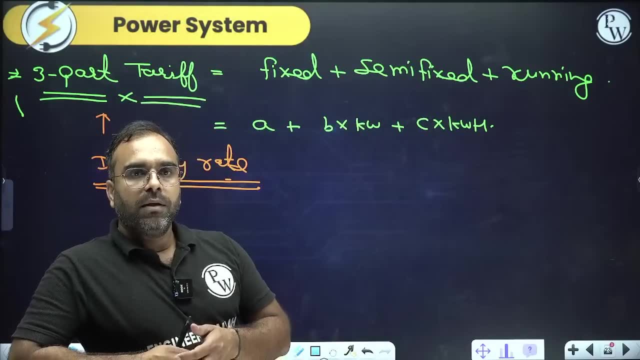 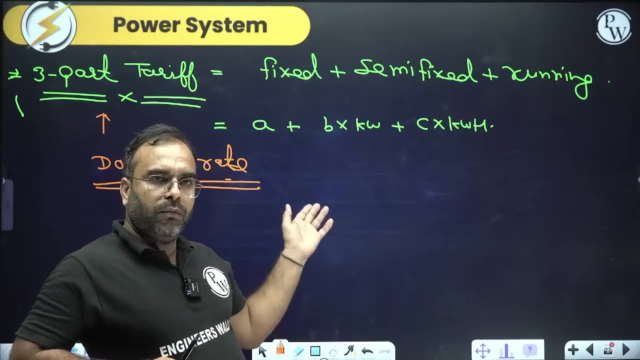 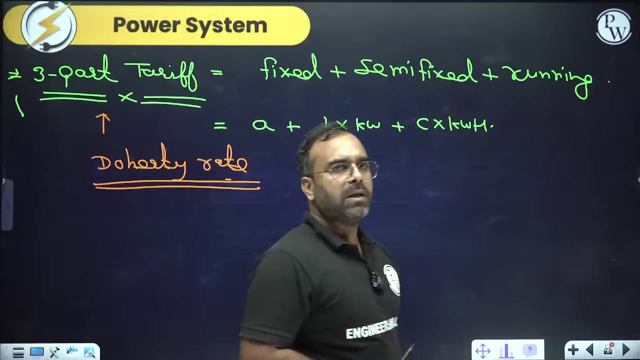 If there is a three-part tariff in the option, then you will put the three-part tariff there first because we are using the three-part tariff mostly we are using this. so see here till now we have more tariff in it: flat rate tariff, flat demand tariff, block rate tariff, KVA demand tariff, power factor tariff. there are many tariff, but all the questions that are asked to us, examiner asks all the questions. he still asks two and three-part tariff. 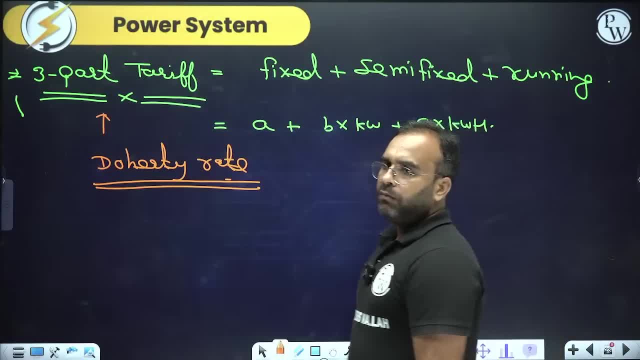 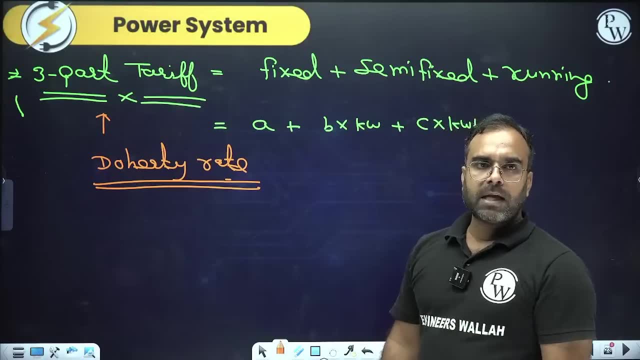 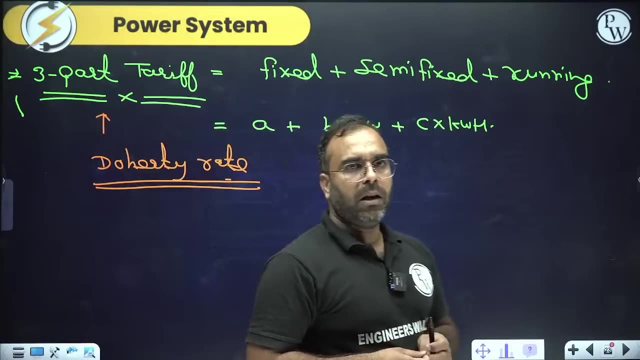 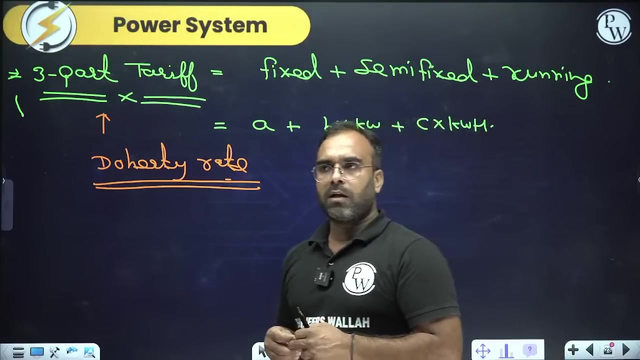 Now we will talk about block rate tariff and I will tell you: we will talk about KVA demand tariff, we will talk about power factor tariff. so in respect of different loads we decide different tariff. but for now- someone is saying that we use block rate tariff at home. son, they used to use it earlier. now almost all the states have changed theirs and a few days ago in UP block rate tariff was cancelled. they said that we will not take money according to block rate tariff. so in different states we will have different tariff. 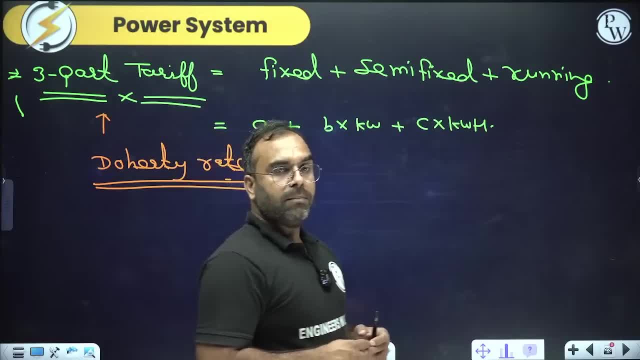 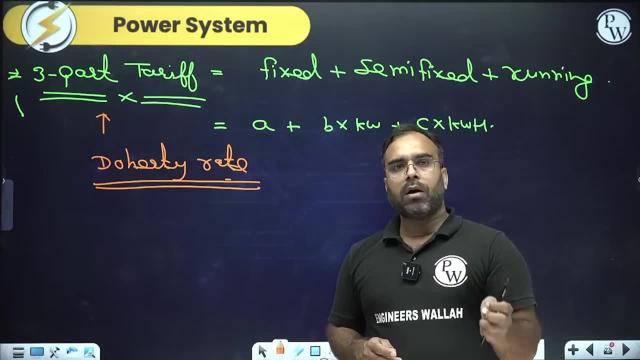 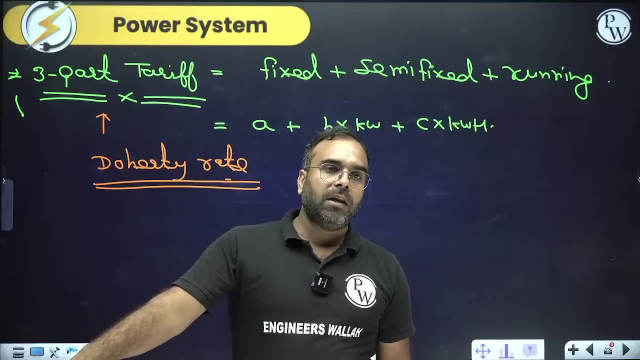 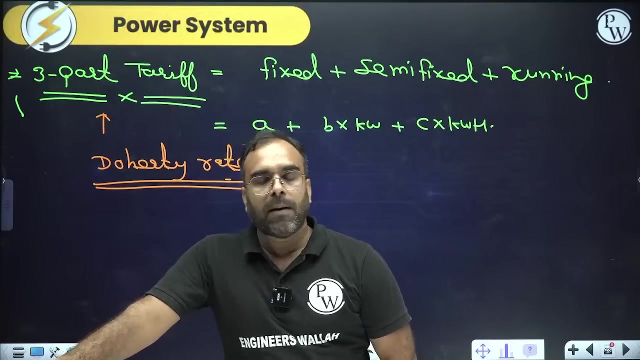 So see here till now what we have revised today. today you must be feeling that we have revised a little bit, but we have read a lot. cost has been done, depreciation has been done, load curve has been done. after that, all the important formulas have been completed. and here we have come to tariff. tomorrow we will complete the tariff part. after that we will read: hydro power plant, steam power plant, nuclear power plant, etc.